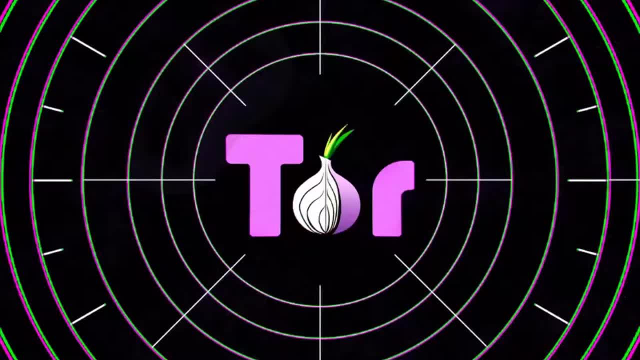 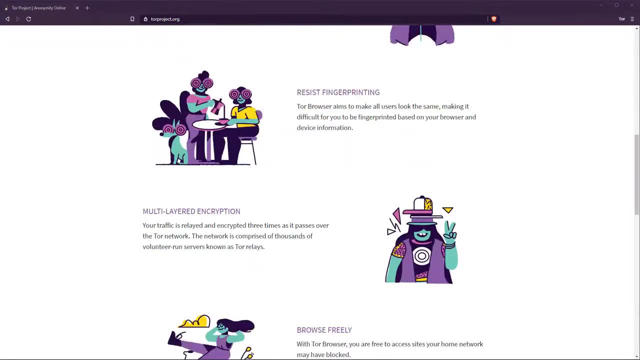 What is the tour and how does it work? What is the tour? The tour project is an intelligent solution developed by the United States Navy to protect the United States' intelligent communication online. Nowadays, however, it continues to serve as a non-profit, open source organization that promotes privacy online and is open to the masses. 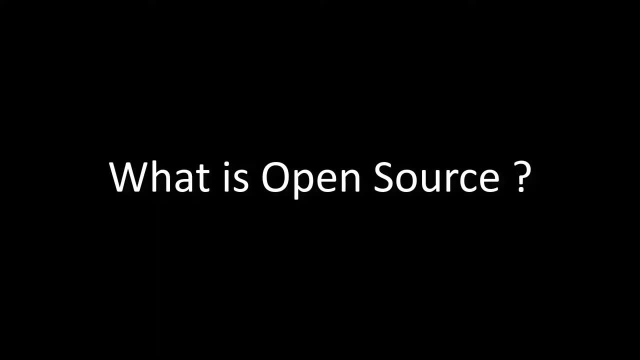 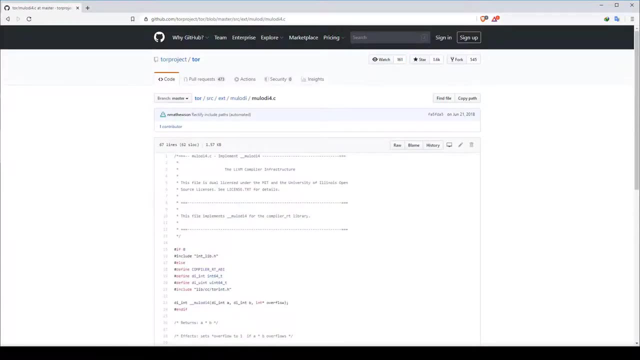 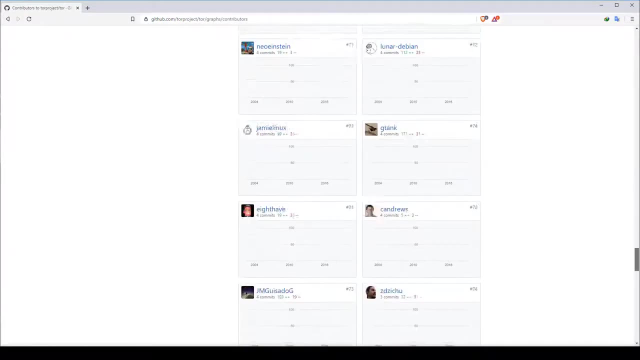 If you don't know what the expression open source means here. open source means that all source codes of the project is shared publicly. Since all source codes of the project are shared openly, the project can be developed much faster by many volunteers. ensuring the absence of the malicuse code. 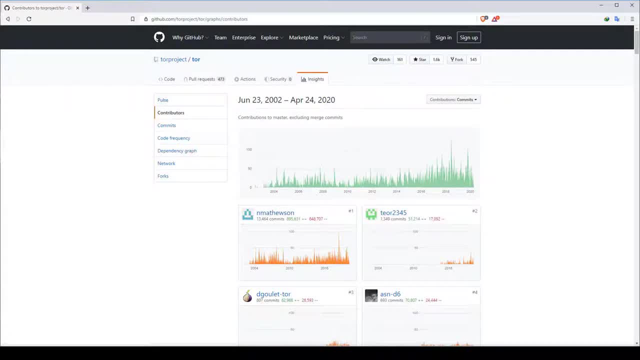 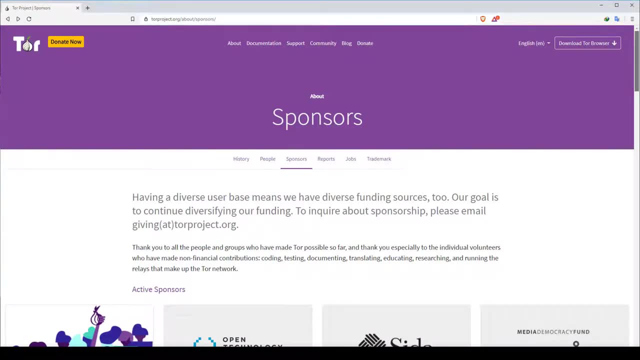 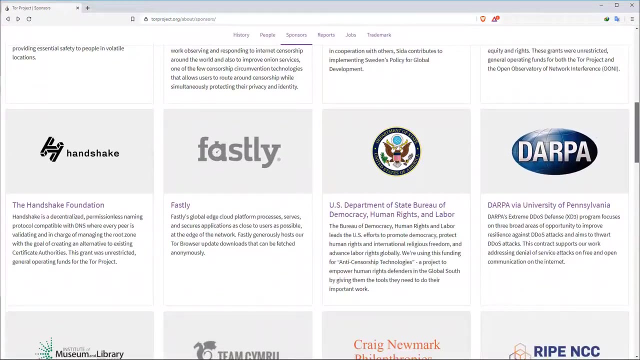 To sum up, if any project is open source, that project is under everyone's control. The main sources of funding for the tour project come from donations collected from volunteers, As well as a large amount of support received from many sponsors, including the American government. 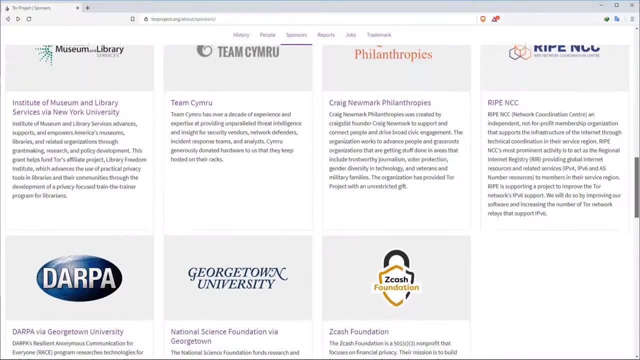 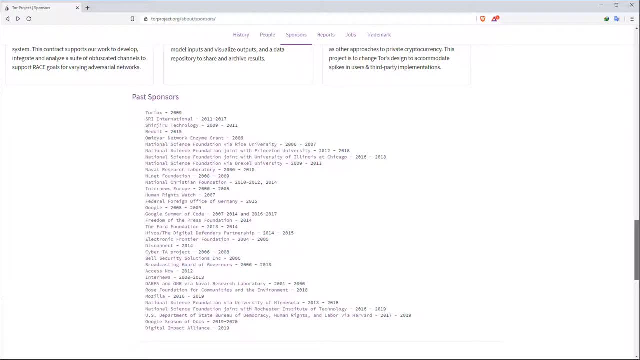 Interestingly, while some agencies of the United States governments provide substantial support for development of the tour project, others routinely spend a lot of resources to bypass the security of the tour network. In other words, a lot of funding is provided by the United States to the tour project at the same time. 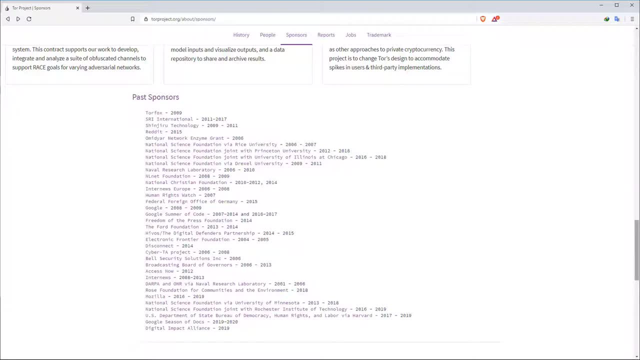 for both development and exploitation of the security. This is interesting because tour is not only available to the United States government. It is free and easy available to people all over the world. Government support is true to have different political and strategic reasons, And the tour independent organization is working to improve its founding base by taking these criticisms into account. 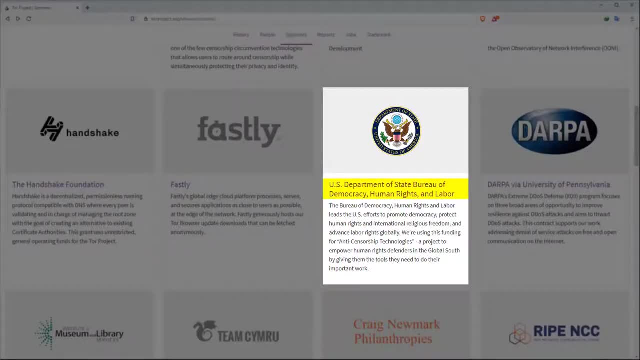 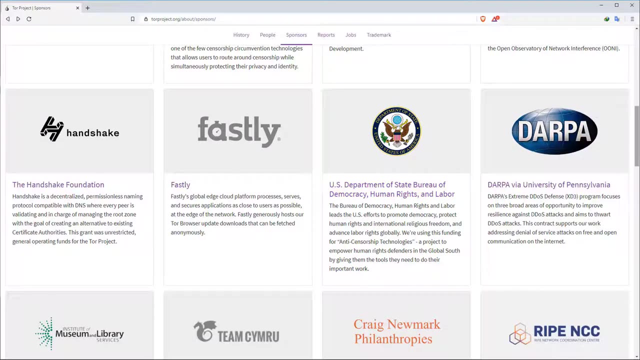 Nevertheless, considering the current situation, the United States Department of State Bureau of the Democracy, Human Rights and Labor is the main supporting institution. It is claimed that the aid is not malicuse. It is aimed at human rights. If you are curious, you can browse the tour project websites for more sponsorship information. 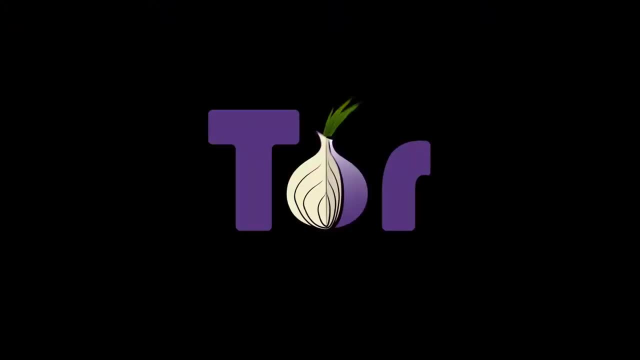 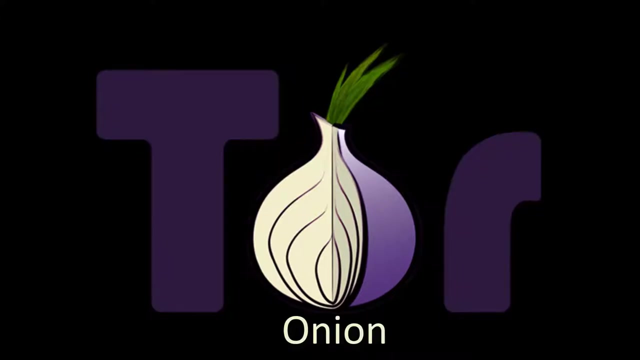 The name of tour comes from the expressions the onion router, which describe the multilayered encryption and routing to ensuring privacy. Since tour project was multilayered, this structure was likened to the onion, So the name onion comes from here. 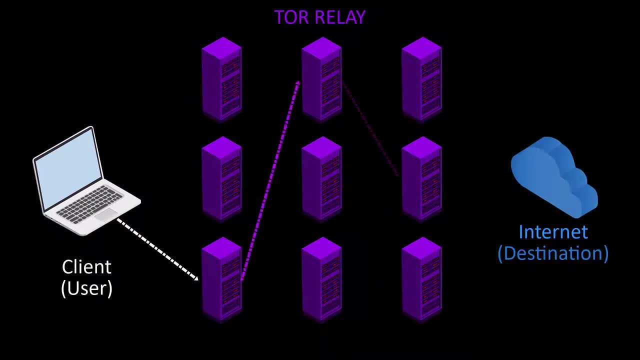 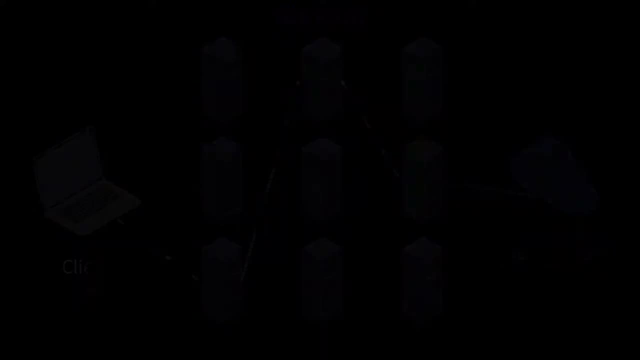 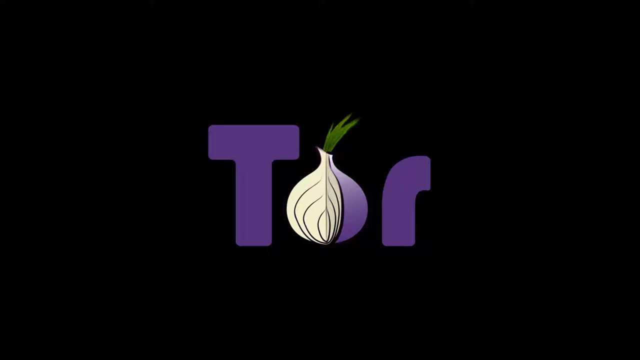 Tour's main goal is to distort our footprints on the internet, allowing us to access the internet anonymously and uncensored. How does tour work? Tour is basically based on obfuscation principle In order to better understand the working structure and see what kind of the system we actually rely on. 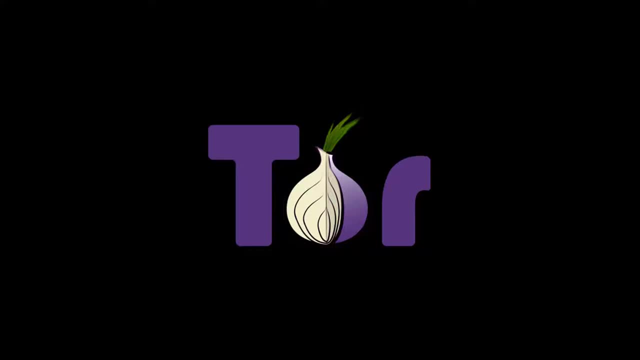 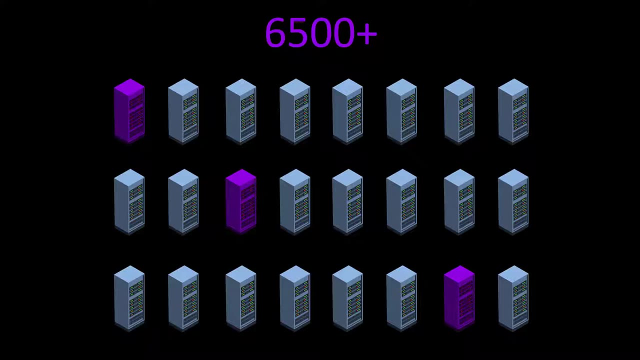 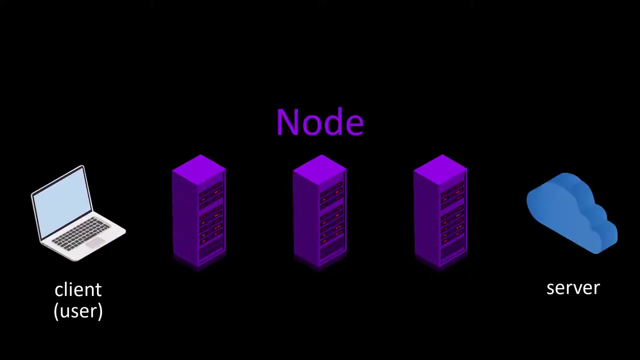 let's start by talking about the general working structure For the process of anonymizing the user. three of approximately 6500 voluntary servers are selected randomly. These selected servers are called nodes. While connected to tour network, data packets are encrypted and transmitted through these three nodes to the target server. 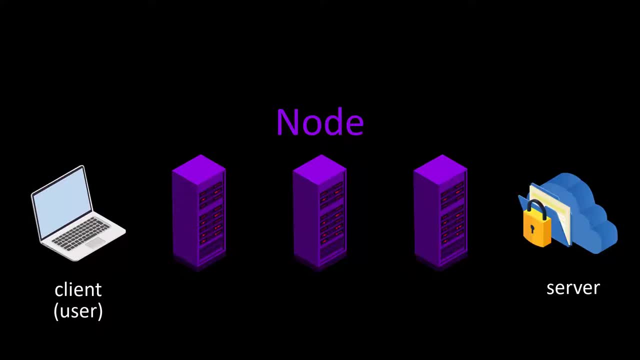 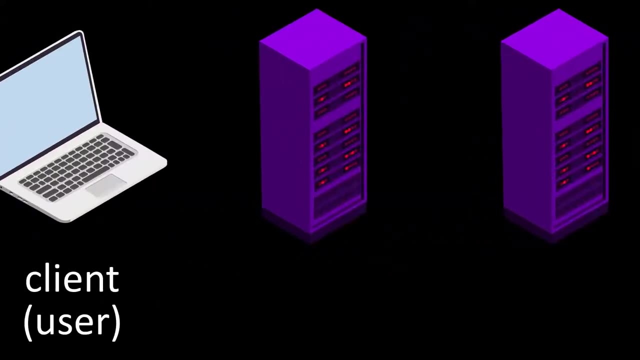 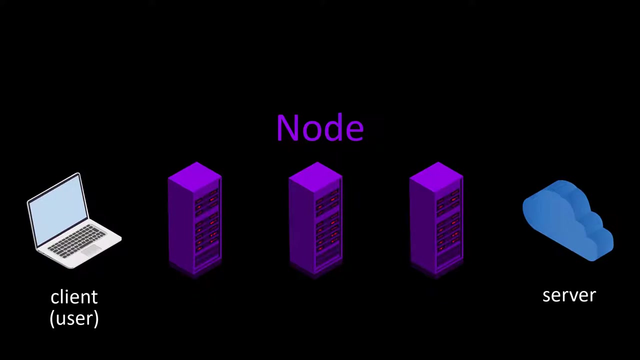 The server's response packet is encrypted in the same way and transmitted the user over three nodes. In this way, all traffic between the website and you is anonymized. Quite generally, this is the way the tour network works. However, let's continue to explain, as it will make us more secure. 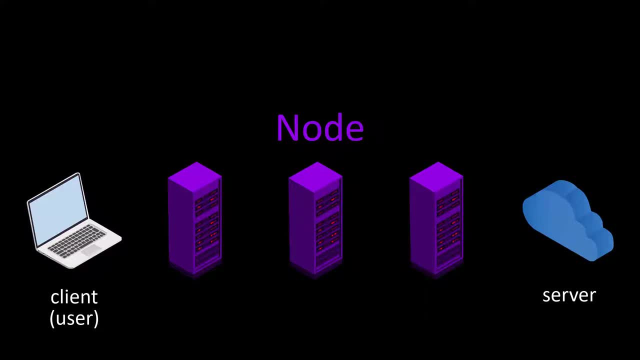 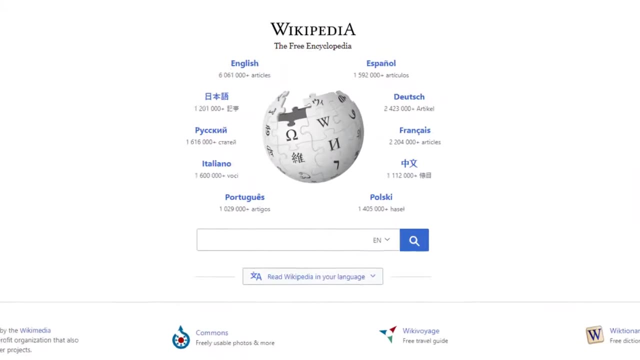 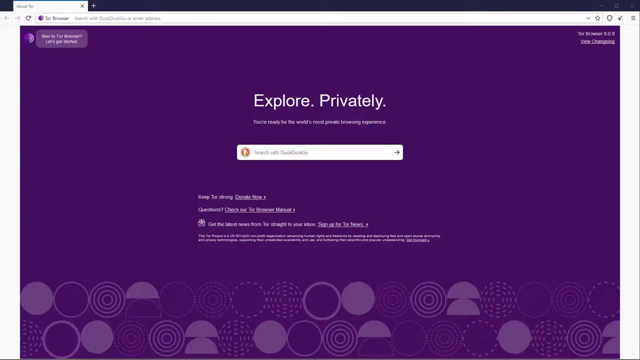 to know in a little more detail how our anonymity is provided through this structure. In example scenario, let's visit wikipediaorg via tour and explain all the process steps that take place during our visit, one by one. Firstly, for use, the tour network: 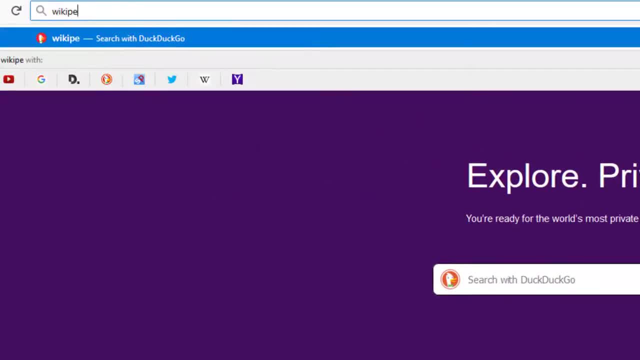 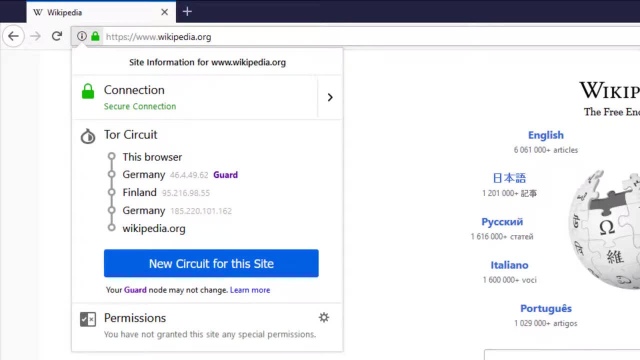 I opened the tour browser and typed the addresses I want to go to. Tour first selects the three random nodes from around 6500 active tour servers. Tour servers work on the voluntary basis and, in the selection of the voluntary servers, servers that can be provided high bandwidth and remain open for a long time are preferred. In other words, the number of these servers- which are certainly around 6500, may change over the time, and the list of all servers is publicly published After the nodes points are selected randomly. my request packet is encrypted in three layers. The request package here is the package that states I want to go to wikipediaorg. 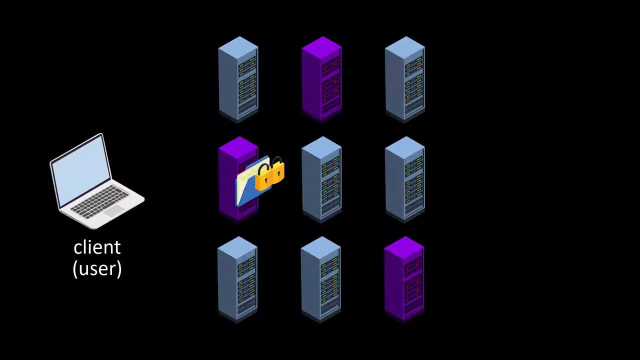 The first node of the encrypted layer is decrypted by key in the starting node, and the decrypted layer only gives information of the next node, Those the first nodes. only knows to which nodes is the will forward the request package. Likewise, the middle node decrypts on the second layer with its own key. 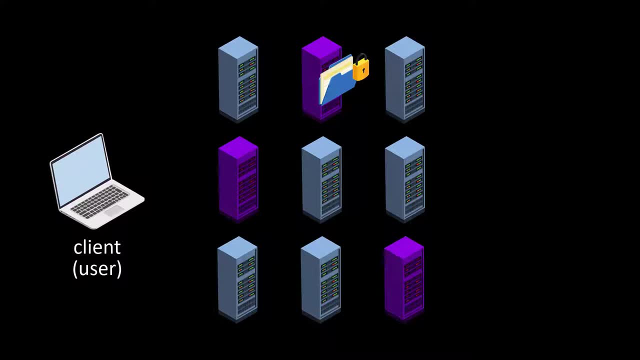 In this way, it learns which nodes to redirect packets to and it redirects it to The last encrypted layer in the packet. reaching the exit node is also decrypted, and which server this packet should be transmitted to is learned by the last node and the packet is transmitted to the relevant server. 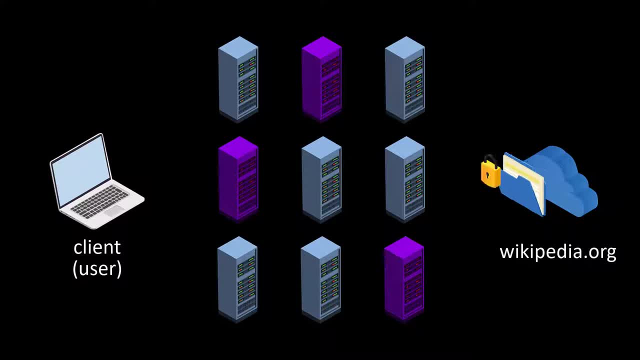 In response to the package reaching the server. the response packet of the server follows the same route and reaches the user, namely by client. In addition, in order to ensure anonymity of the user in long-term use, the selected nodes are changing randomly every 10 minutes by default, except for the first node. 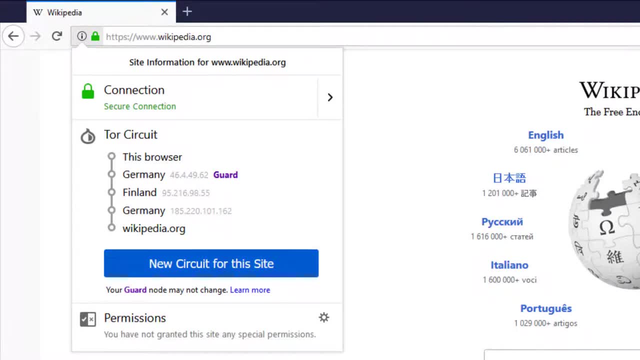 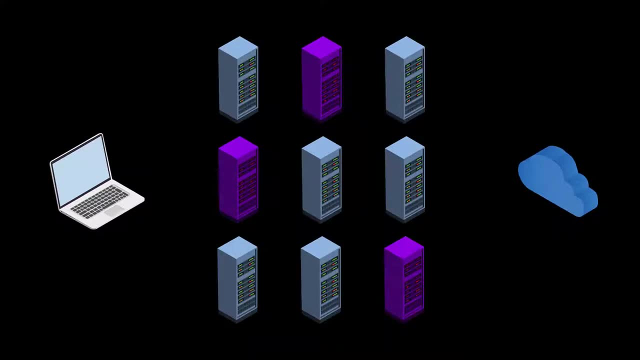 In addition, users have the opportunity to manually change the nodes randomly whenever they want. This much information is enough for now, as going into much deeper and technical issues will not make you safer on the Tor network. This is how the Tor network generally works. 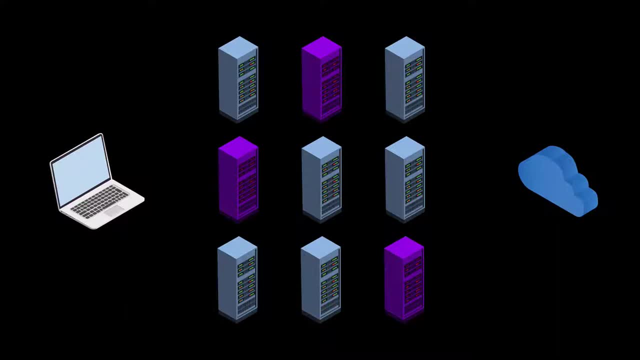 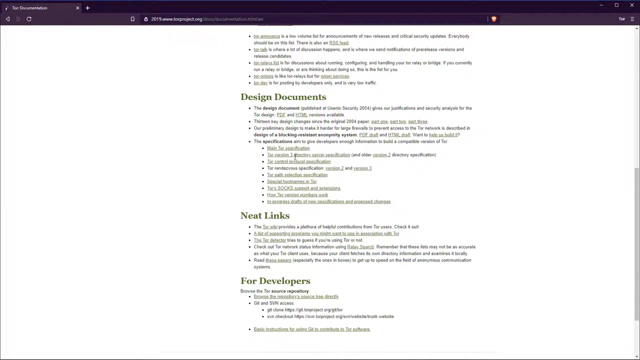 We'll be talking about this working structure in more detail in the following sections. If you are curious about the technical and scientific detail behind the Tor network, there are many articles on the subject. You can easily access the detailed information on the Tor official website. 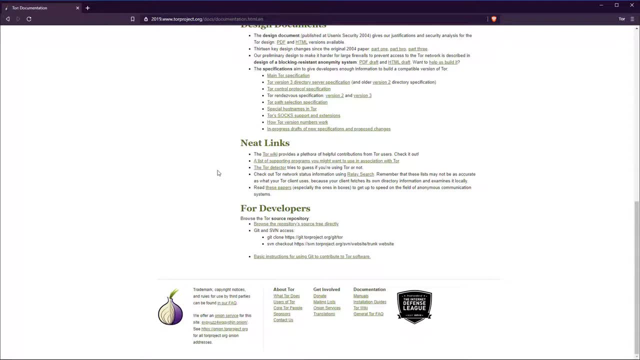 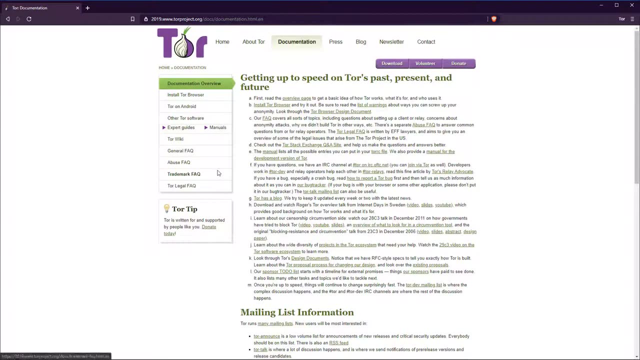 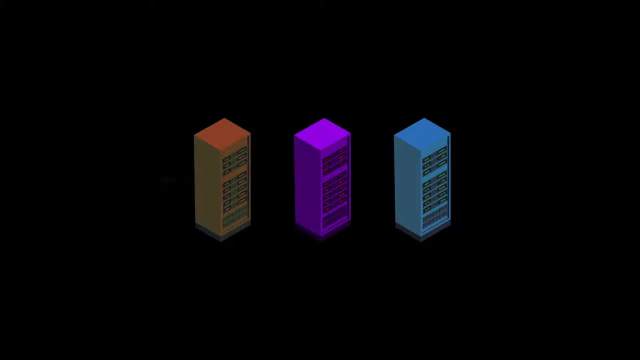 or if you do a short internet search. However, you can be sure that in this course I will talk about everything you need to know about anonymity and privacy. What makes the Tor network secure? In structure of use, the Tor, only the first node, knows the real identity of the user. The exit node only knows which server should forward the packet. Thus the first node doesn't know to which exit node the packet is sent to, while the last node doesn't know from whom the packet, Since the task of the middle node is only to transfer between the first node and the exit node. 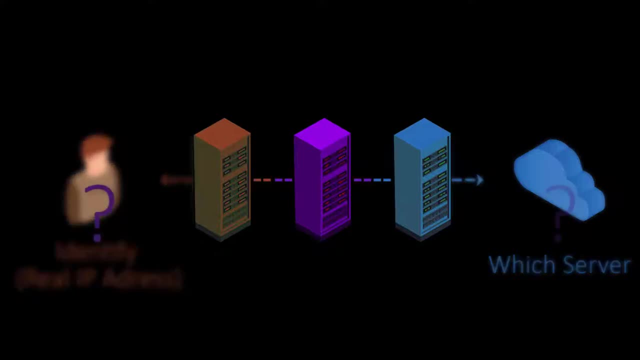 it cannot know the sender of the packet and which web server the packet will reach. In this way, anonymous communication between client and the server is provided. However, the structure used by the Tor is not that perfect in the real world. Now let's talk about the weaknesses of the Tor network and the solutions to these weaknesses. 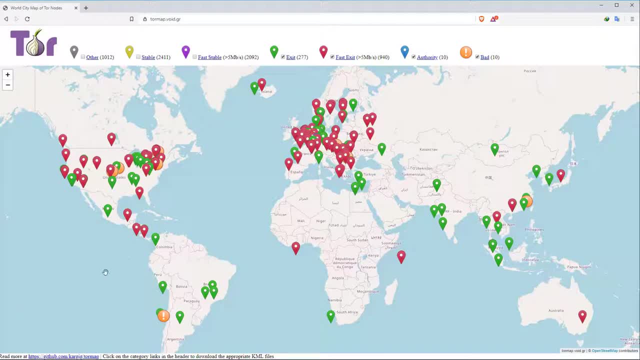 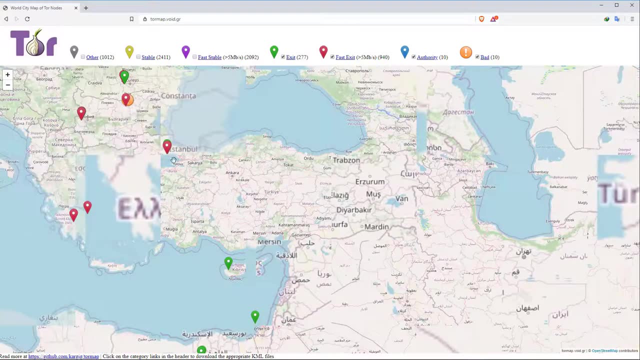 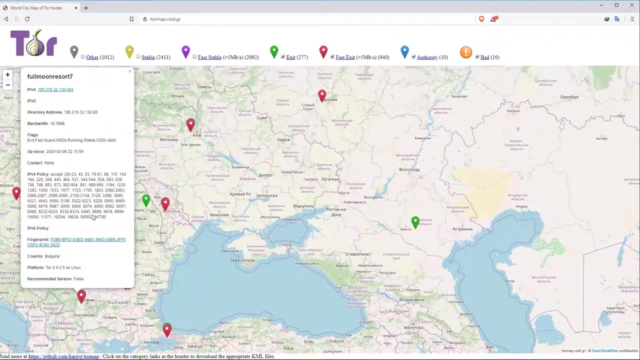 Fundamental Weakness 1. First of all, since the list of node servers you can connect to through Tor is published publicly, Any authority, such as government, internet service provider, network administrator, etc. can easily restrict your access to the Tor network by blocking each of these servers. 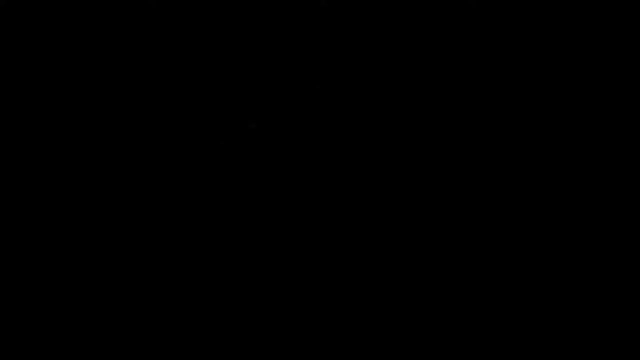 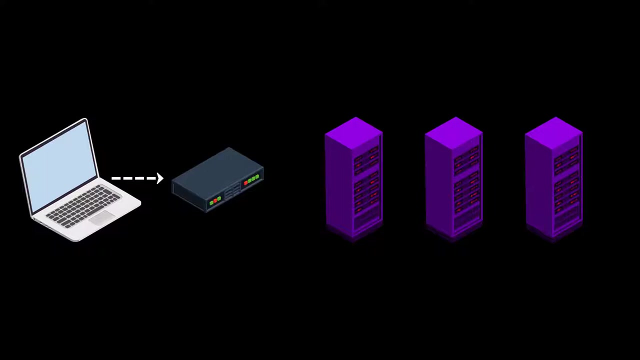 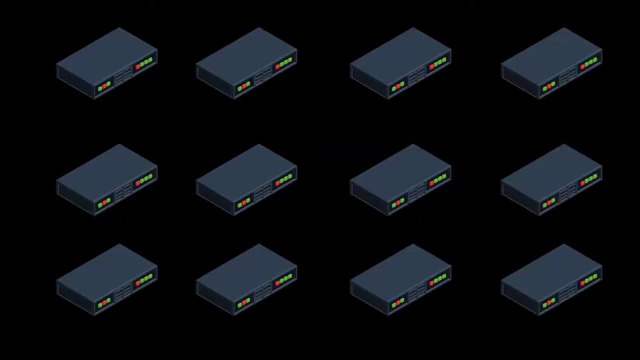 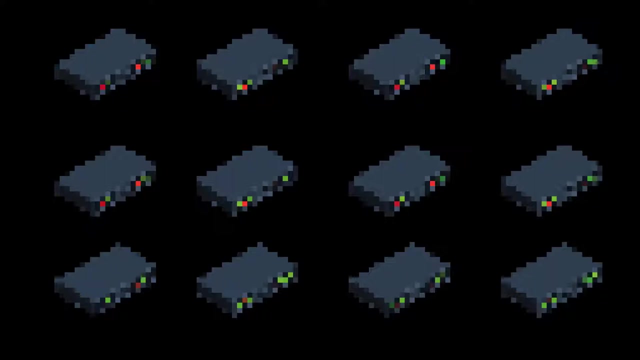 As a solution to this situation, Tor provides bridge connections. With the bridge connections provided to you before accessing the Tor network, you can bypass existing districts and gain unlimited access to the Tor network. Moreover, since all these bridge addresses are keep confidential, it is prevented from blocking all of them in possible situations. 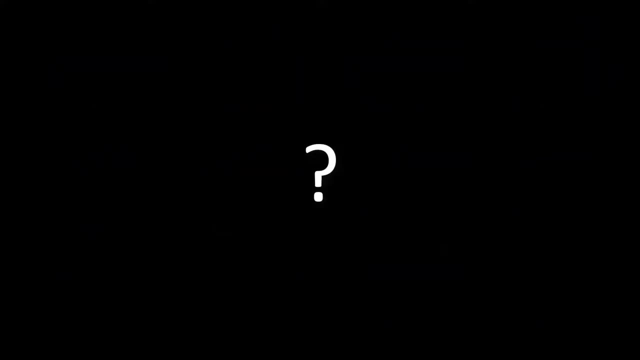 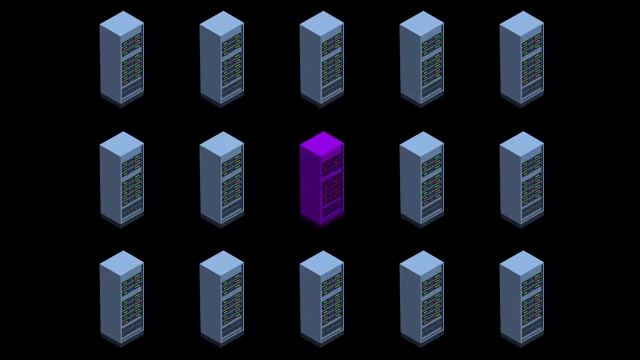 But if its Tor can keep bridge connections private, why doesn't it keep the list of node servers private? Essentially, there is no point in trying to keep the server's information private, Because anyone who owns one of the voluntary servers can obtain and publish the list by running a client. 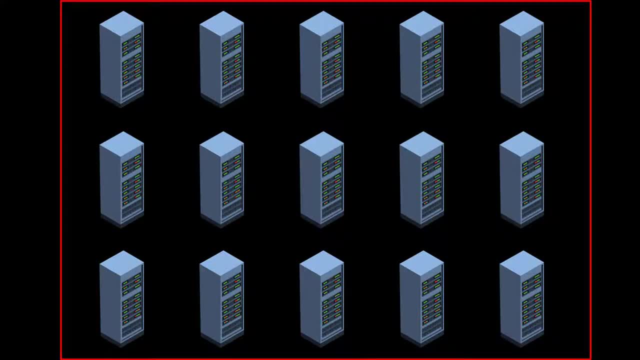 Since all the servers are located the common Tor circuit, it is not difficult for any servers to reach the list of other servers. In other words, due to the working structure of the Tor network, it is very easy to get information about which servers on the Tor network are active. and which servers are inactive. So keeping the server list private is pointless. Fundamental weakness 2: When transferring your packet to the entry node and when you packet reaching the destination server from the exit node, your privacy can be breached by those who listen or control the entry node and exit nodes. If observers are only observing between you and entry node, in other words listening to your network, they can only see that you are connecting to the Tor network. In some cases, even this may cause you to be under a deeper follow-up by becoming a suspect. On the other hand, if they are listening to both your connection with entry node and the connection between the exit nodes and the servers with greater effort, by looking at the correlation between the time of sending your packet and the time of the packet reaching the server. 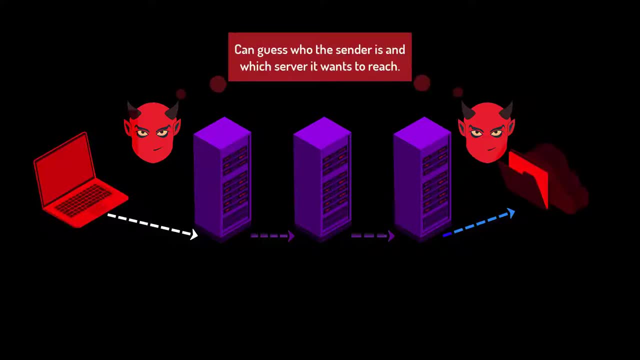 they can conclude that you are interacting with this server and deepen the tracking. Although it is low probability that this situation will occur, it may violate your security when it does, And this weakness is unacceptable when we speak of real privacy and anonymity At this point. 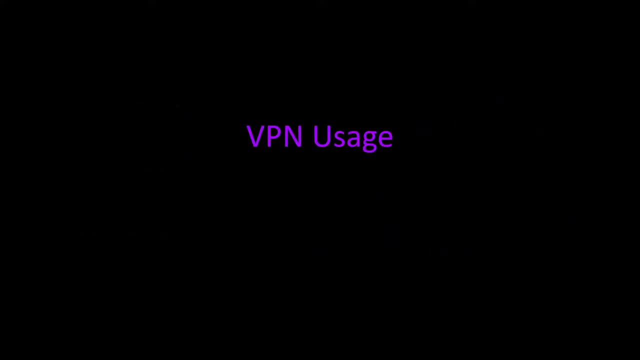 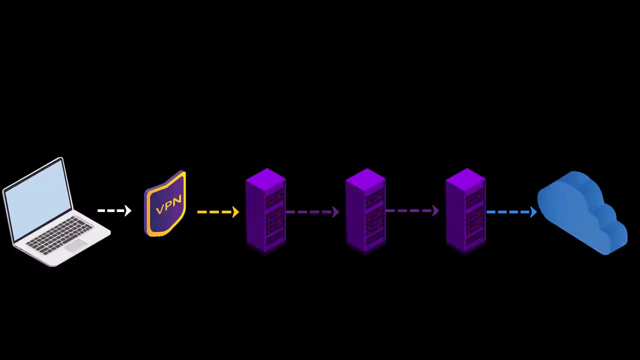 it is must to use VPN in addition to Tor and prefer HTTPS web addresses with SSL certificate. We'll deal with these issues one by one in the course, but let's try to explain briefly for now If you use VPN before accessing the Tor network. 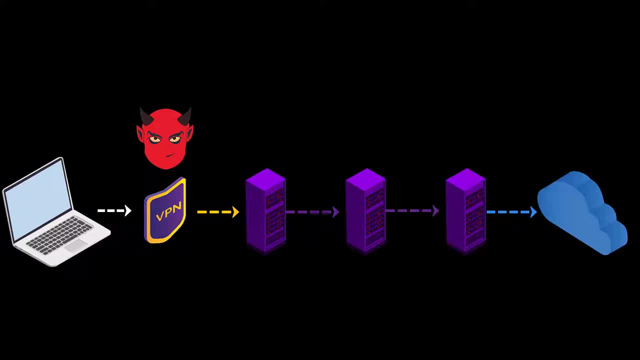 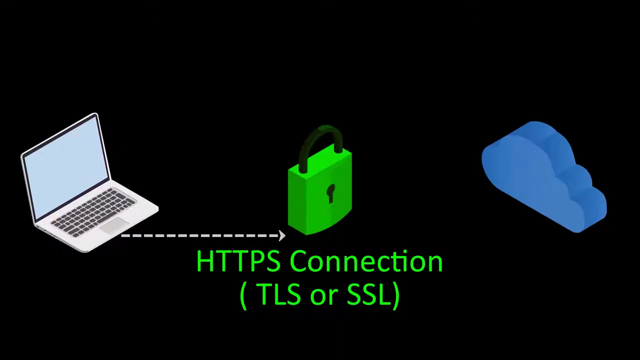 observers won't be able to see that you are accessing the Tor network, as they will only see your VPN connection. This usage is called the Tor over VPN, Also communicating only with servers' SSL certificates will encrypt communication between the server and you. 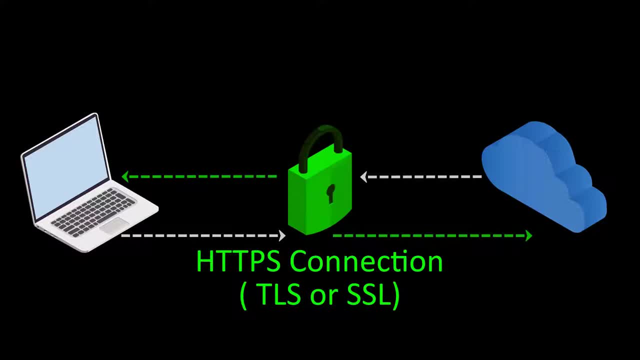 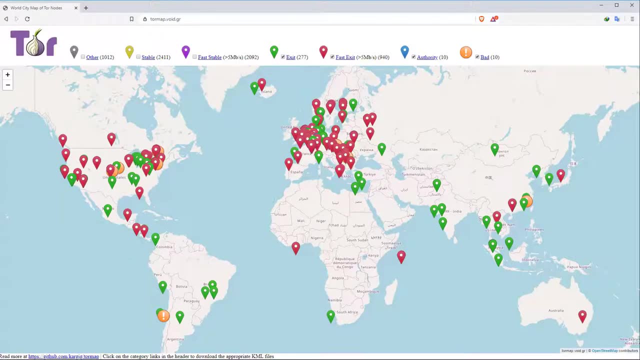 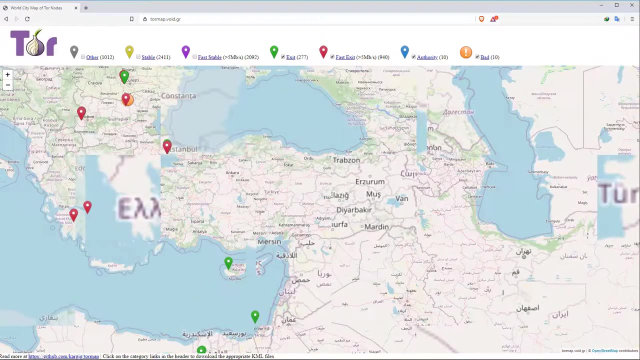 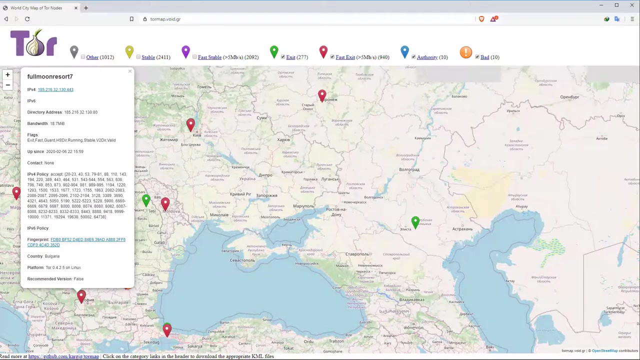 keeping sensitive information away from observers- Another point of risk- that the server used as nodes and transferring your packages are provided by volunteers around the world. It is not surprising that among these volunteers there are various intelligent agencies and individuals or organizations intending to monitor the Tor. 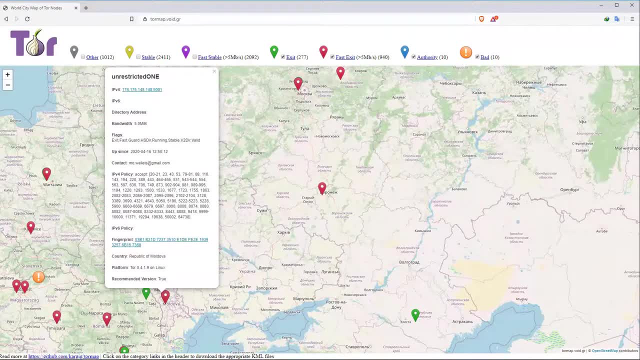 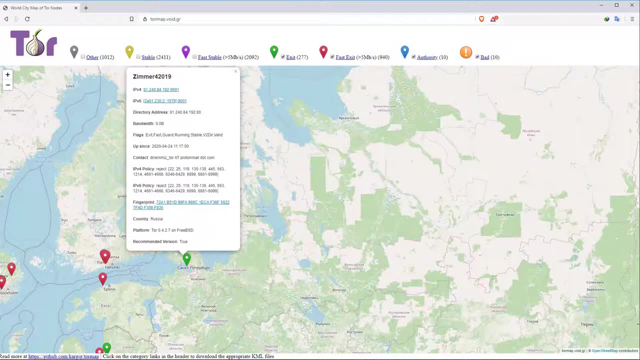 In particular, the requirements that the preferred server's high bandwidth and long active working time are conditions that are not easy for every volunteers to provide for free. Moreover, the possibility of dealing with copyrights and various lawsuits due to traffic generated through their own servers makes people question the interests of people. who endure such a terrible many times. When this is the case, you don't know which nodes to trust. However, the probability of this insecurity by the Tor community is considered very low, Considering there are about 6500 nodes on the Tor network. 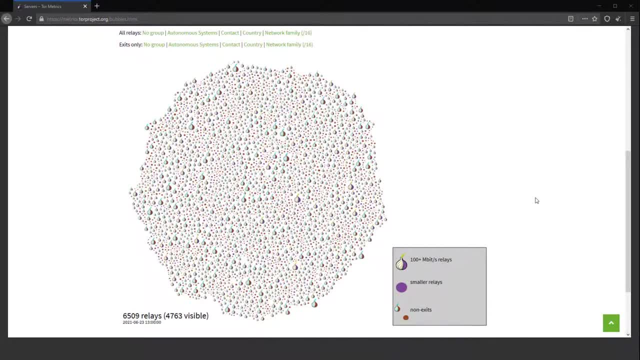 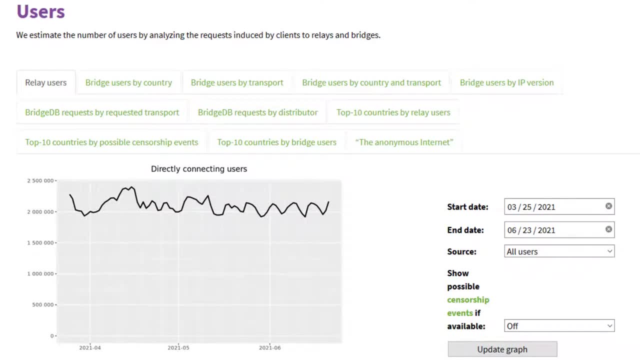 and the server selection is made on randomness and it servers many users at the same time, it is considered low probability to make a problem. This is a point-by-point traffic analysis. However, probably this is a very innocent expectations, Because we don't know the limits and potential of the resources. 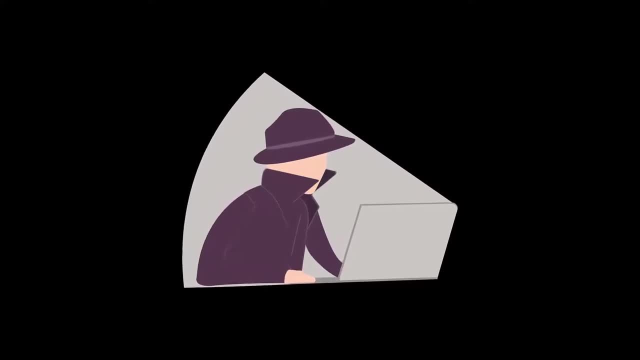 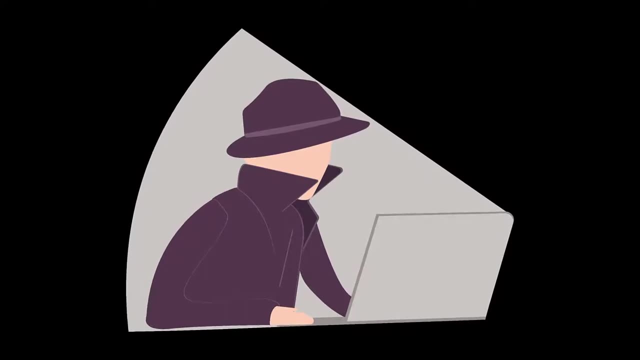 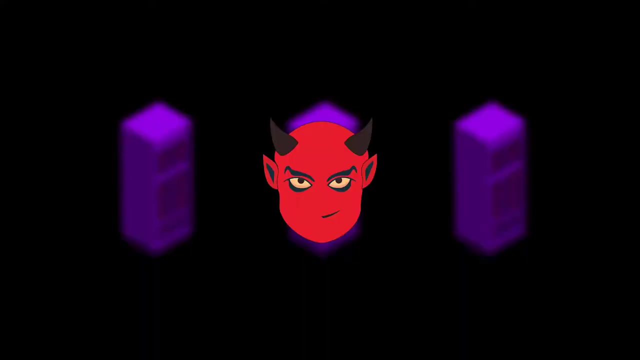 in the hands of an intelligent agencies or any formation that has a high motivated to follow you. this danger always seems to be present. There are even some successful attacks on the Tor network itself. Even so, since any observer is expected to be able, 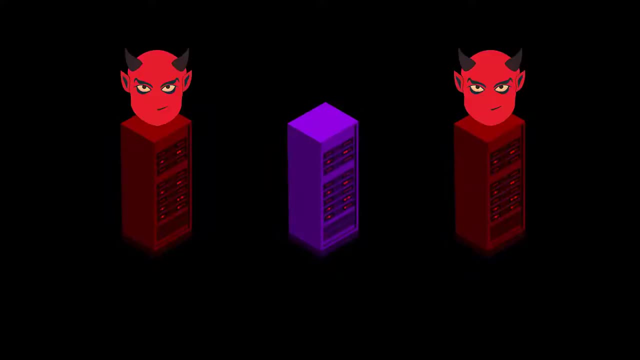 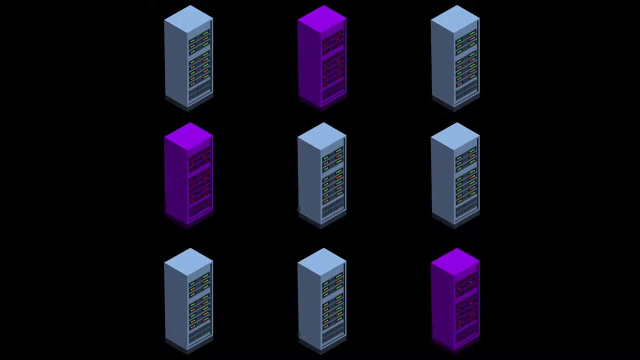 to check both entry and exit nodes' tangible evidence: it is highly unlikely that the entry and exit nodes of three randomly selected servers belong to the same observers. Moreover, since the Tor changed middle and exit nodes every 10 minutes by keeping the entry nodes constant, 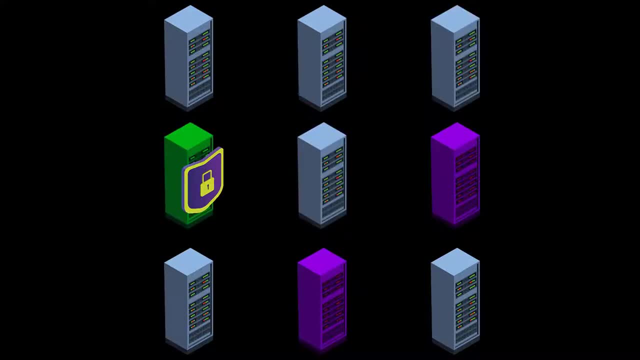 it significantly reduces the probability that both the entry and exit nodes are being managed by the same observer. In addition, as a result of the attacks on the Tor network, it is the general expert opinion that it is more precise to expect the target people to make mistakes. 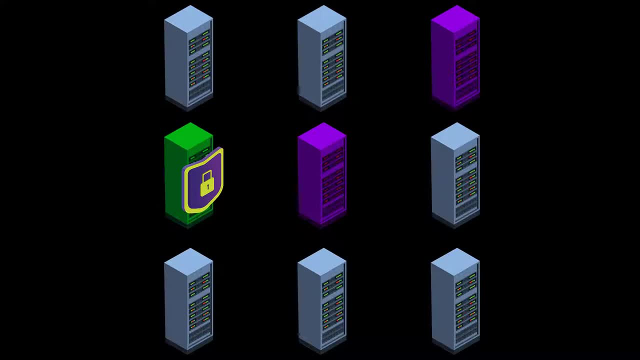 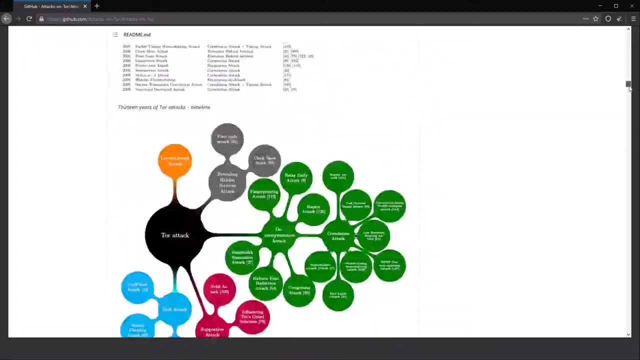 that will reveal their privacy, rather than focusing on the imperfect structure of the Tor network. In short, it is not easy to achieve anonymity. Tor never guarantees 100% anonymity either, But in retrospect, even well-founded, sophisticated attacks on the Tor network haven't yielded definitive, useful results. 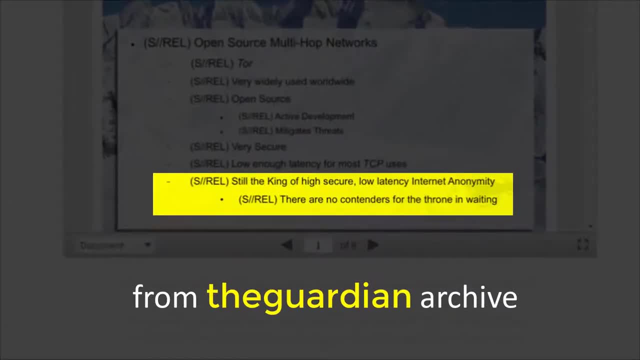 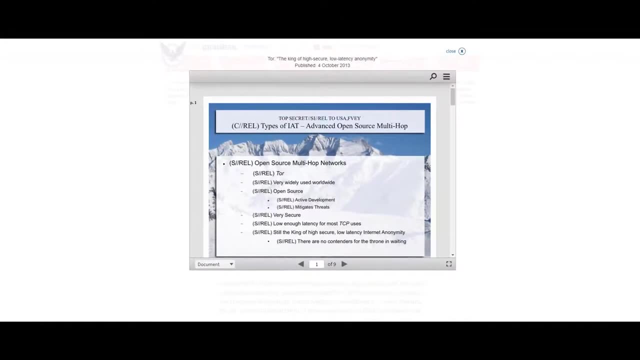 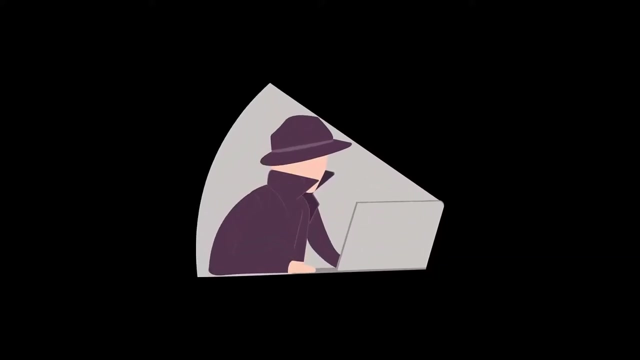 Documents published by Edward Snowden also report the NSA has major problems in monitoring the Tor network. However, Tor can never guarantee 100% anonymity, As we don't know the potential power of today's organizations and the potential newly developed attack techniques. we don't know what the future holds. 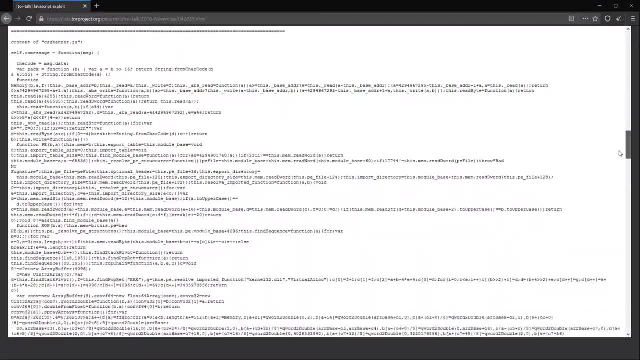 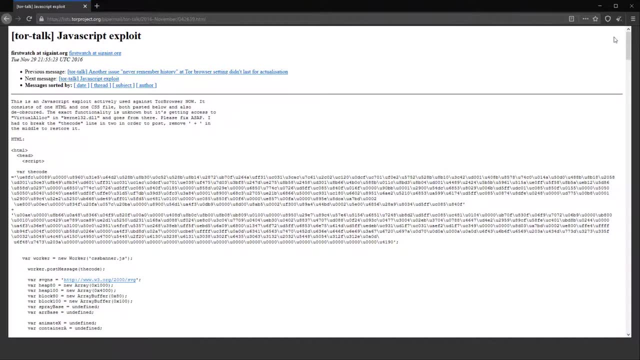 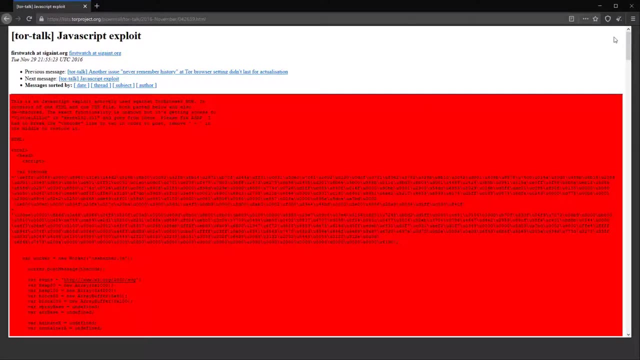 As a proof of this, zero-day vulnerabilities found on Tor in recent past can be cited. Zero-day vulnerabilities refer to vulnerabilities that haven't been noticed or, even if noticed, vulnerabilities that haven't yet been patched, Although there are many published and closed vulnerabilities. 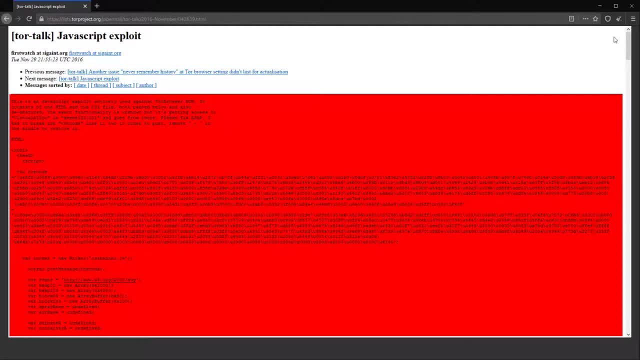 it is thought that there are many vulnerabilities that haven't yet been closed and predicted to be actively used by organizations such as intelligence services. These vulnerabilities are often critical vulnerabilities of the type that will expose your real IP address. However, as far as we know, 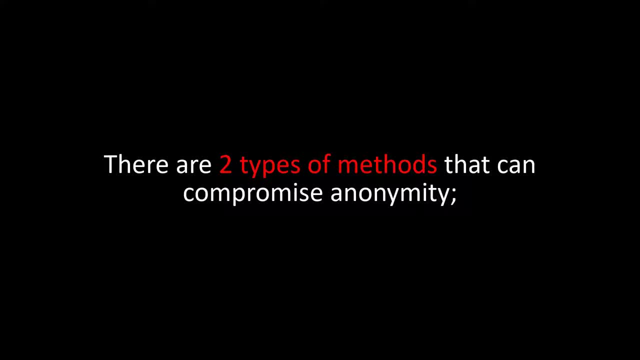 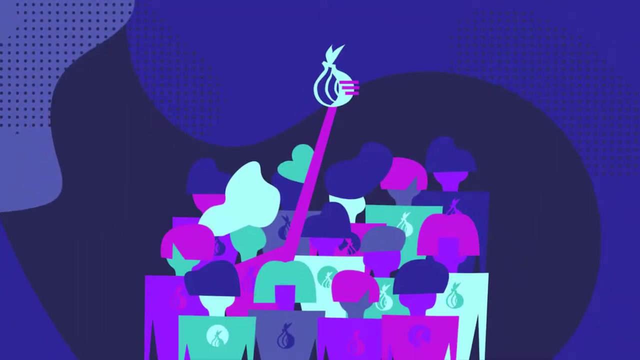 there are two most common types of the methods that compromise Tor network's privacy, rather than technical attacks: Malequeues- exit nodes and timing analysis. Malequeues- exit nodes: As we mentioned earlier, the servers of the Tor network are based on the volunteering and for what purpose they are providing this server resource. 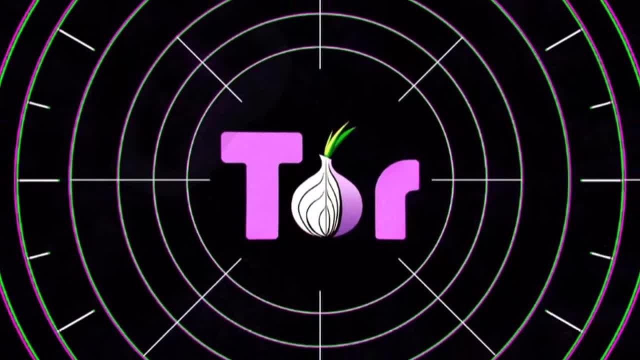 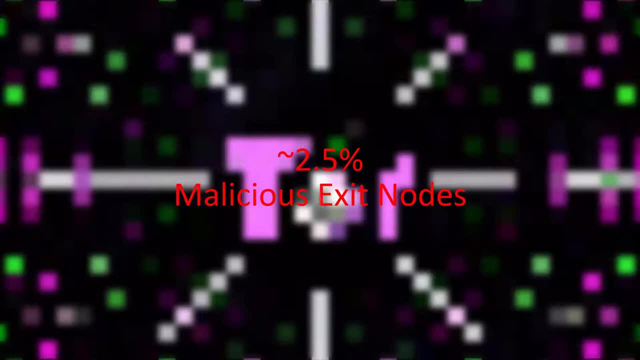 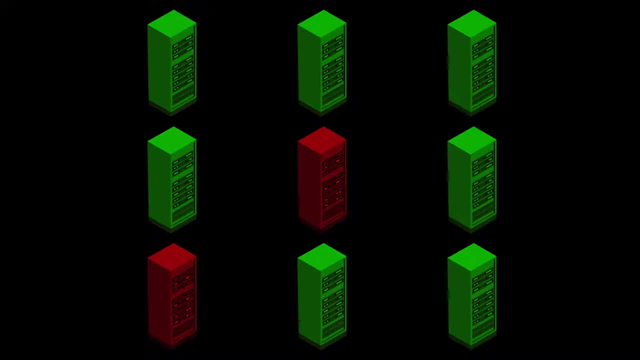 As a result of the Vorius test, it is estimated that approximately 2% and a half of the exit nodes of the Tor network are provided by Malequeues people, Although regular tests are carried out to detect Malequeues servers and remove them from the Tor network. 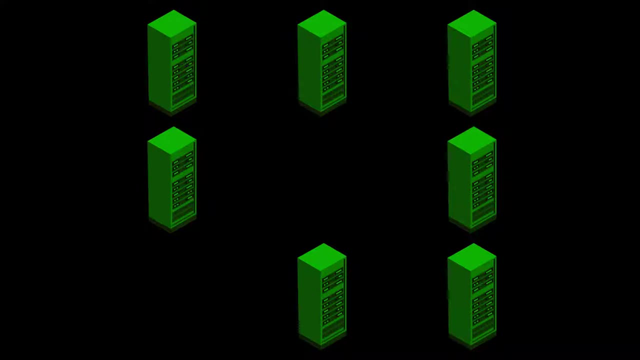 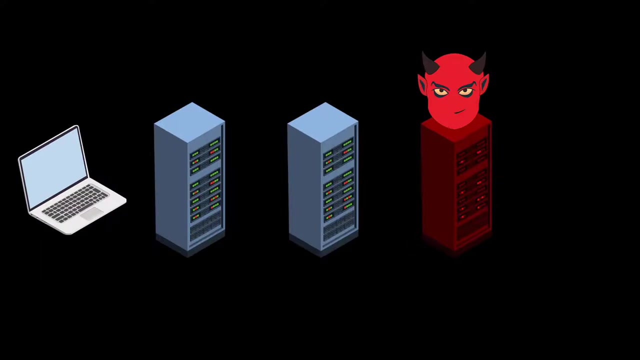 it is a fact that this method doesn't provide definitely solution. What can Malequeues exit nodes do? Since it is the exit nodes, it doesn't know directly who you are, but it knows which web addresses you want to reach. However, you run the risk of revealing your real identify, directly or indirectly. 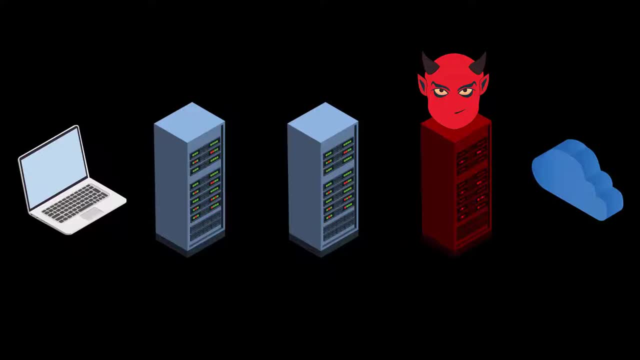 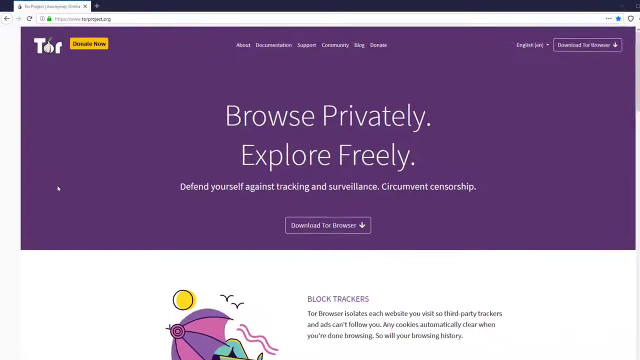 Through your communication and your internet behavior. In addition to spying on your data, Malequeues, Tor exit nodes can often perform a man-in-the-middle attacks that redirects your page request to fake website. How can we protect it As long as you connected to secure, SSL encrypted websites? 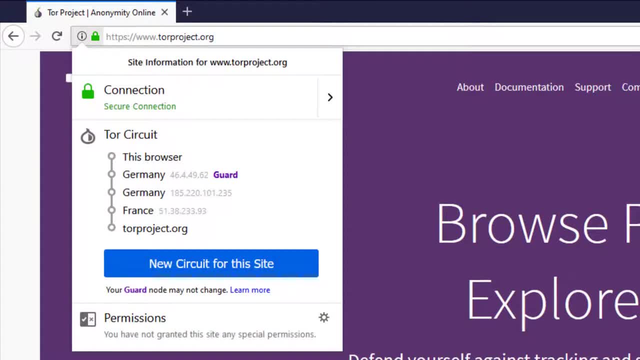 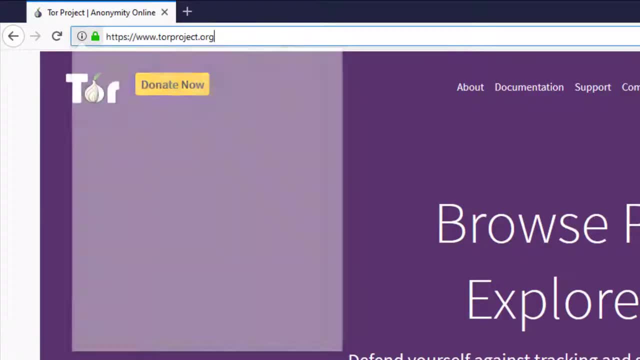 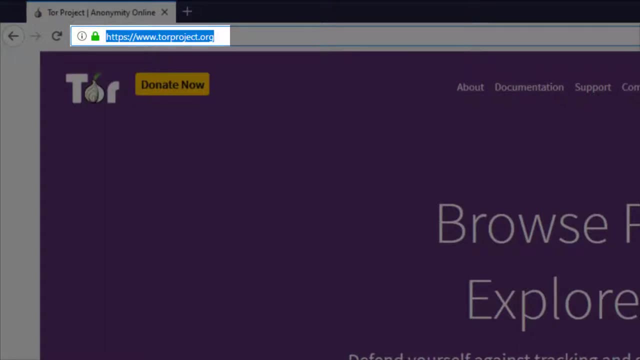 your data stays safe and cannot be compromised by a fake exit nodes And, being aware of the man-in-the-middle attacks, it is important for your security to check the addresses you want to go to and be aware of the sensitivity of the information you enter. 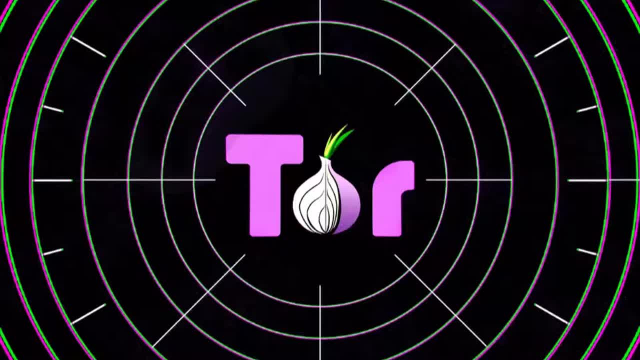 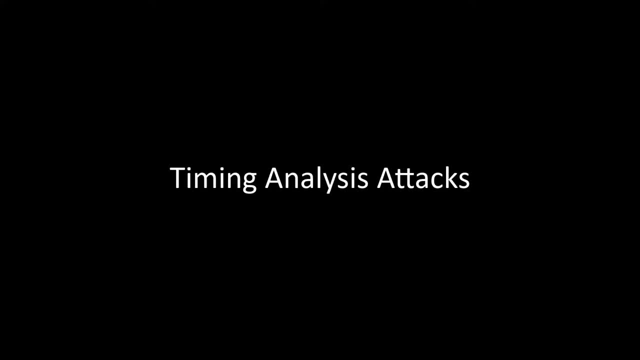 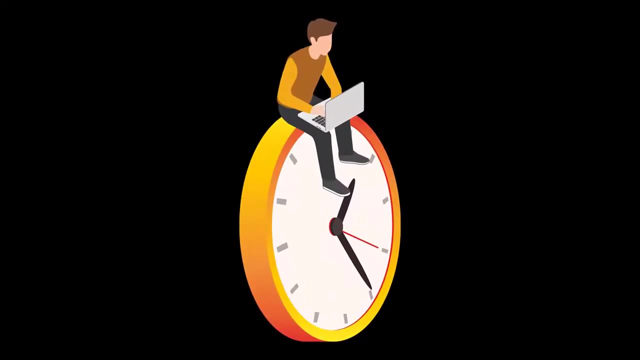 Since you are using the Tor network, you should always be in control of your steps, without thinking that you are completely safe. Timing Analysis Attacks: These are the attacks that the risk the most security. Essentially, timing attacks are attacks that can be created with a wide variety of scenarios. 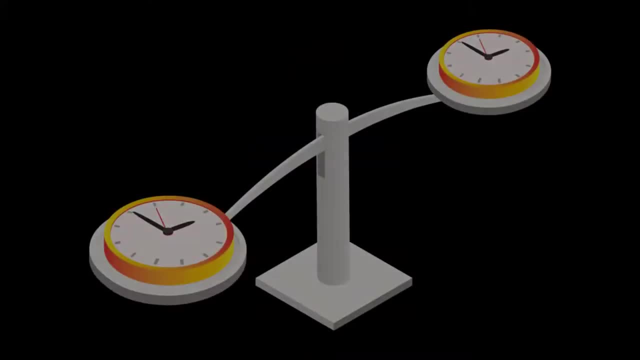 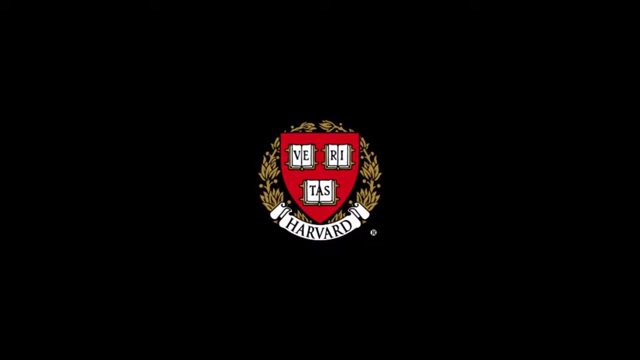 the ones that most security risk. The main purpose of the timing attacks is to determine the correlation between the activities performed and the time when the person accesses the Tor network. For example, in 2013, Harvard students made bomb threats to avoid exam. 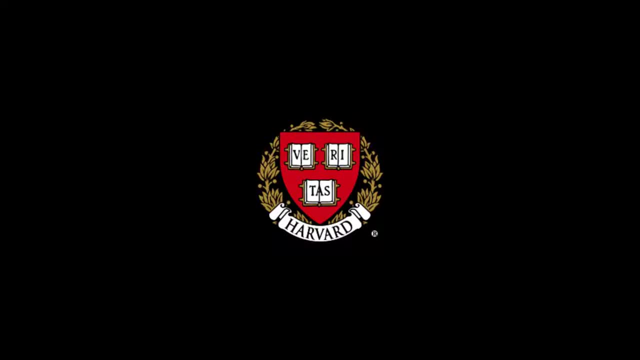 This bomb-huxing was sent over the Tor network after a certain period of time, using an email service that self-destructed. However, despite all these security measures, the person making the huxing was Kao. The main reason for his catch was that. 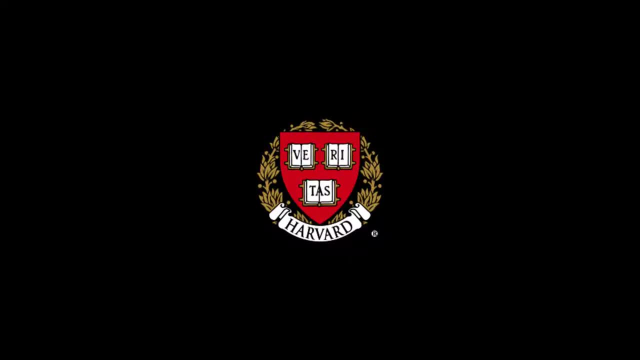 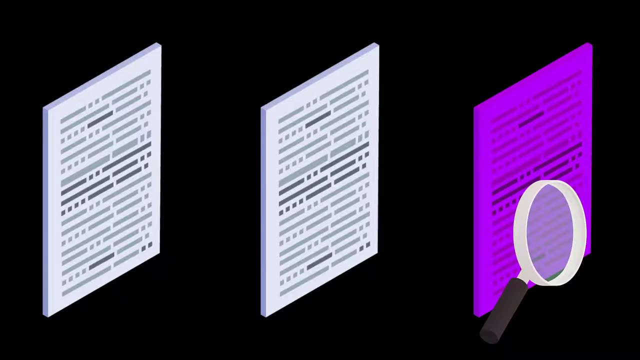 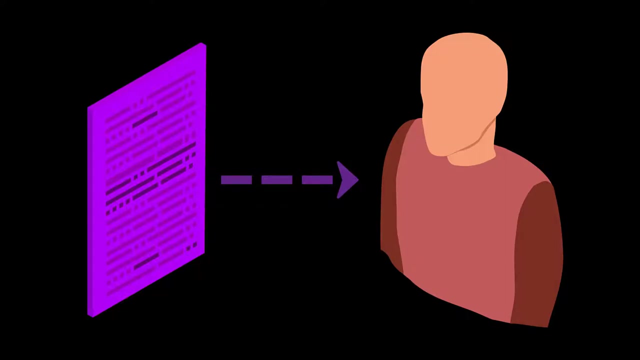 he sent the email over the Tor campus Wi-Fi network. The research team checked to see if anyone had accessed the Tor through the local wireless network. After all, this was only one person using the Tor network on campus And it turned out that was the person who sent the message. 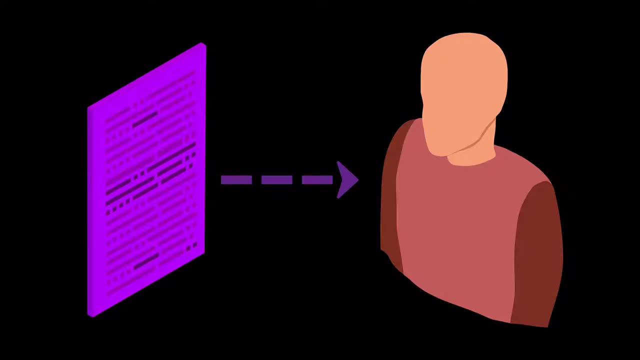 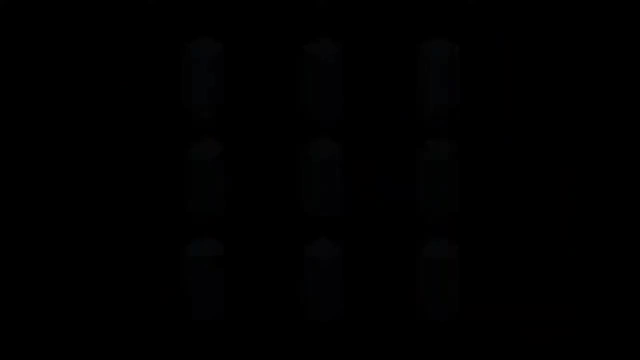 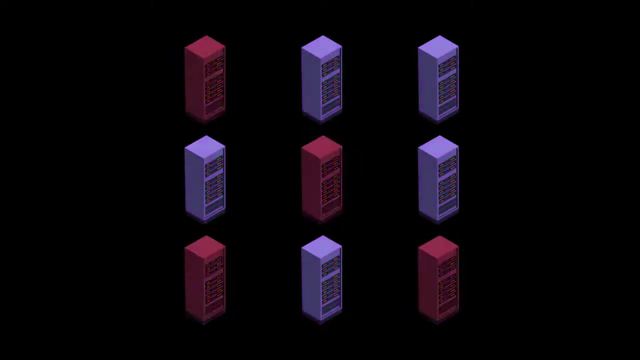 This is a fairly simple mistake of Kerne's, But basically the real identities of people can be revealed through such time matches. Apart from this, if the observer has a high number of the servers on the Tor network, it can identify the person by analyzing the incoming. 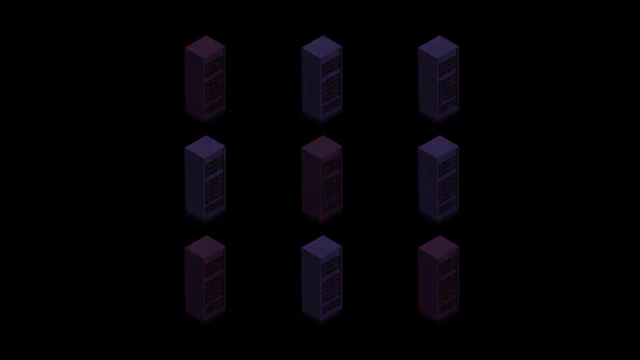 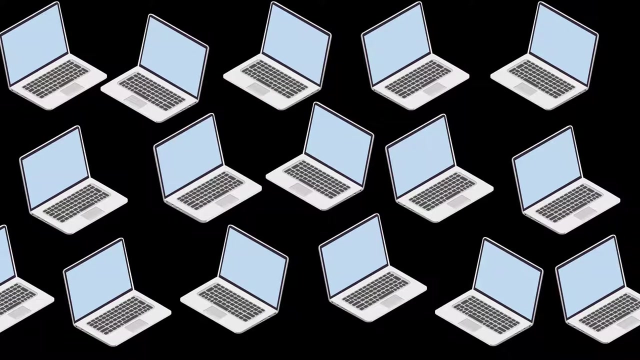 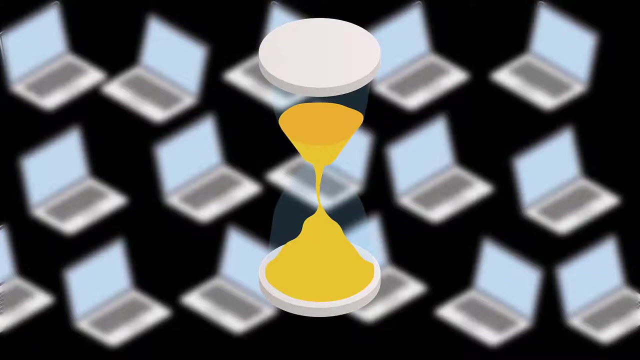 and outgoing data in a similar way. However, as there will be a large number of Tor users online at any given moment, such a correlation would require extensive and long-term statistical analysis, making it almost impossible to get definitive conclusions. However, of course, 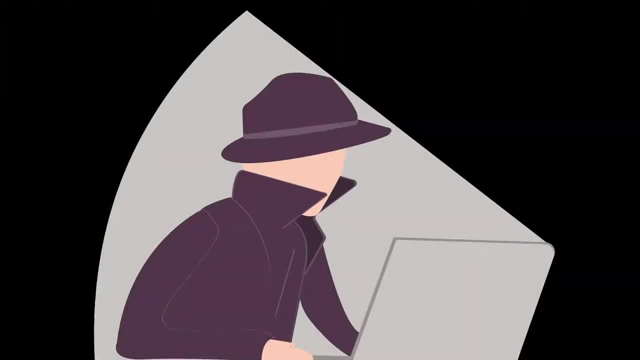 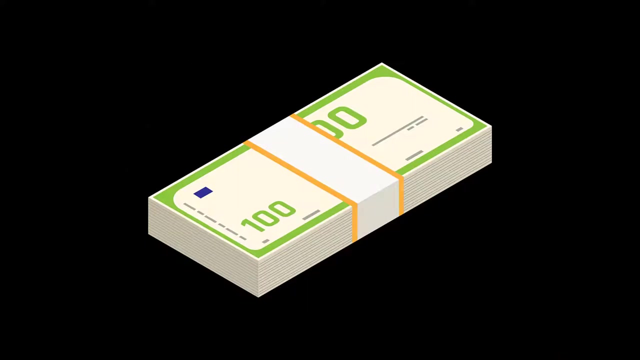 we have no way of knowing the potential resources available to various organizations that have virtually unlimited power and truly global reach. So, in theory, if the observer allocates enough resources for the target, there is always a possibility that the target might violate the anonymity and privacy. 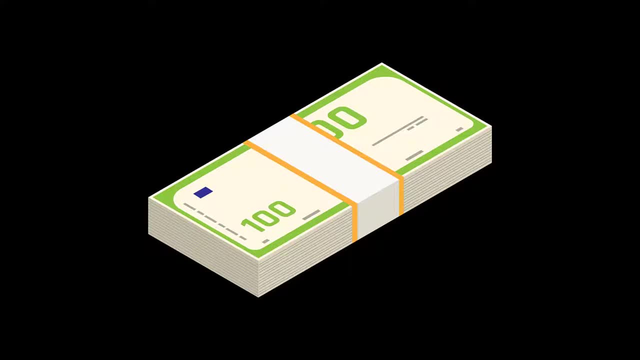 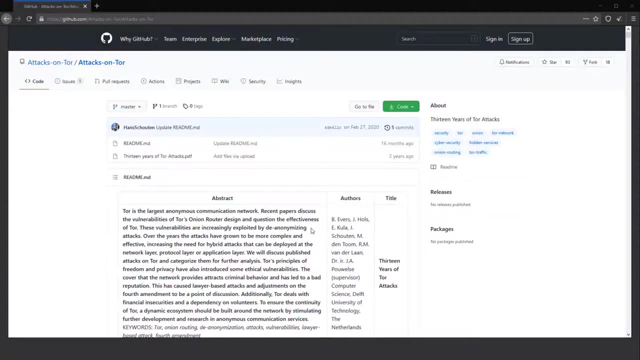 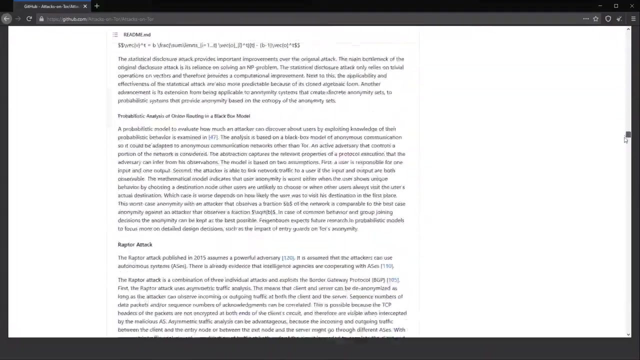 In addition, apart from these two attacks, many inattentions that a person can make directly reveal the identity of the person. However, if technical attacks other than inattentions are of interest to you, you can also take a look at the known attacks on the Tor network. 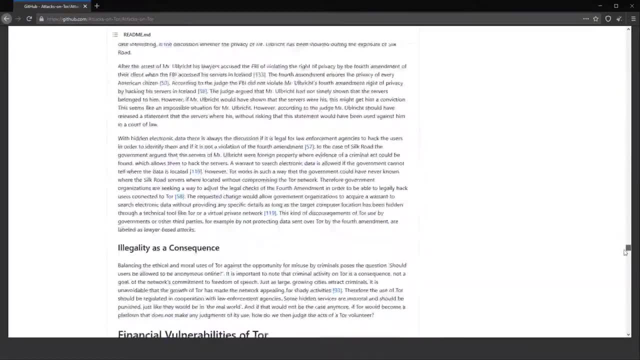 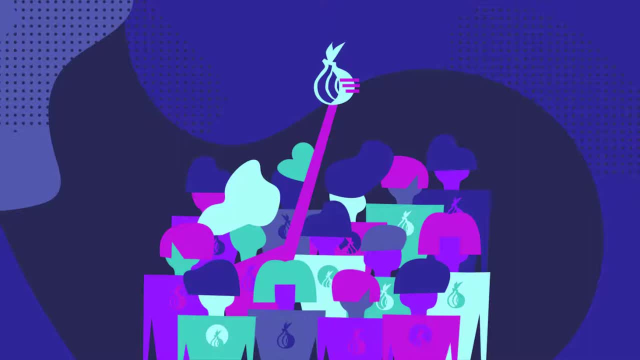 from the list in this lecture: resource Types of the attacks from the past to the present. If you are not going to participate as a developer to actively contribute to the Tor project, the detail of technical attacks are unnecessary for a normal user. Tor developers are responsible for resolving technical attacks. 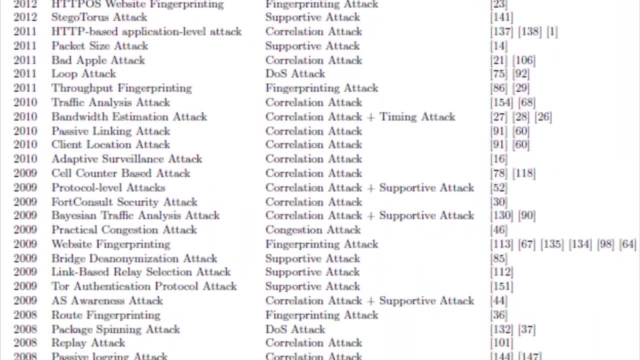 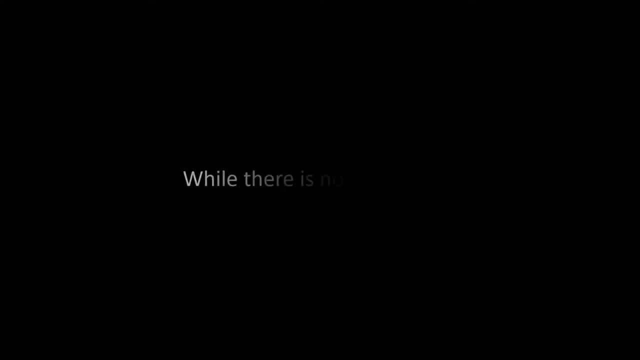 However, you can, of course, take a look at the attacks on the list in order to have general information. So how can we protect it? While there is no direct way to protect yourself from timing attacks, keeping your personal activities under control can provide security. 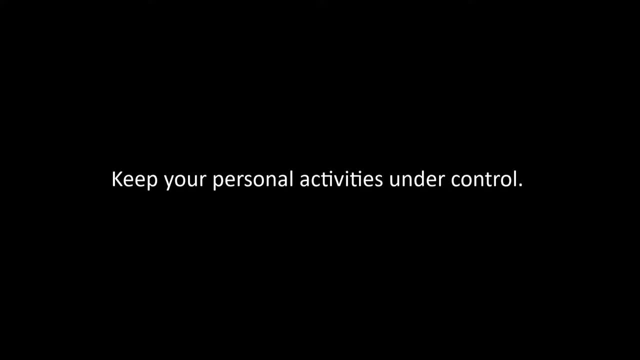 You need to act by taking all these parameters into account, including the internet you are connected to your location, the computer you use and whatever can be associated with you in real life. In short, you should be able to keep all factors required for operational security. 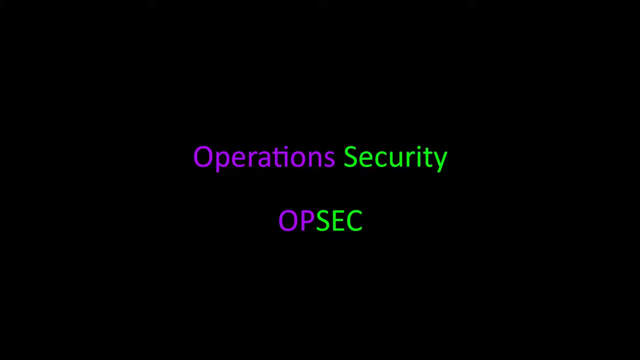 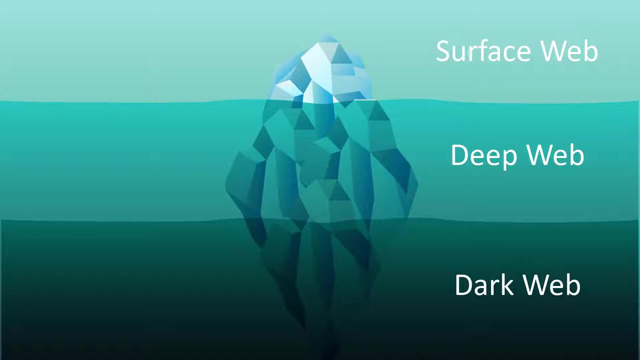 called OPSEC, under your control at all times. Tor, hidden services. Let's start by explaining a few concepts. You have probably heard of the concepts of deep web, dark web and surface web before. The iceberg example is often used because it represents concepts well. 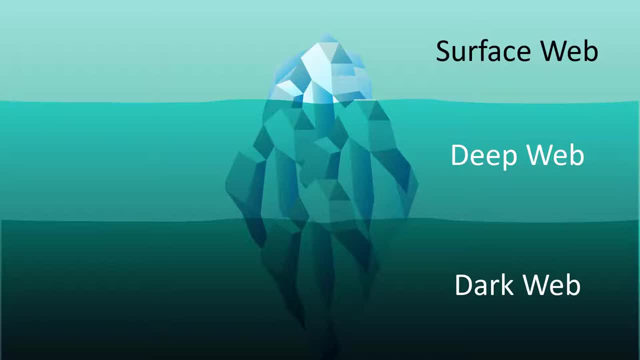 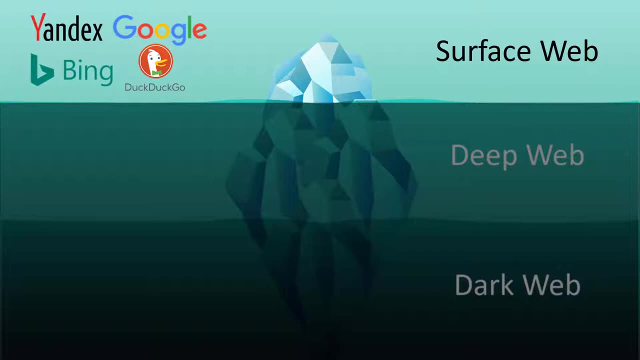 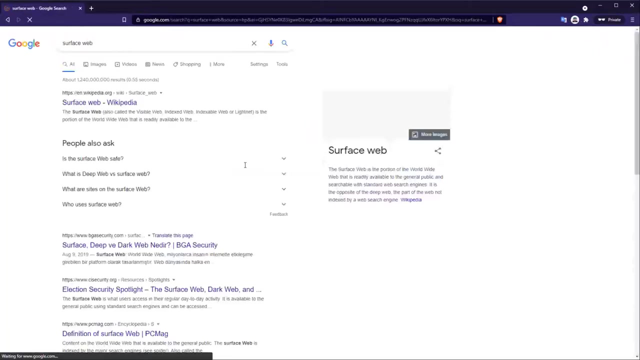 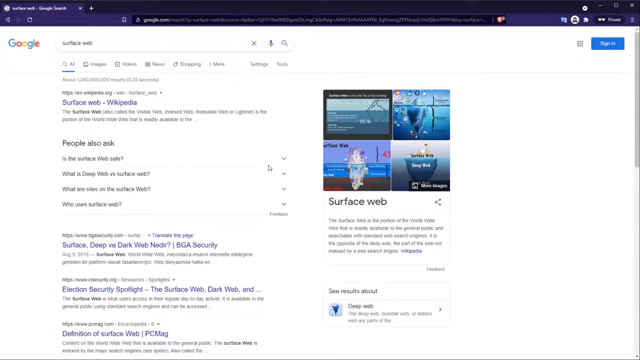 Surface web. As in the iceberg analogy, it represents the surface of the web network. that is, a very small fraction of the overall web network indexed by search engines. For example, when you search using a search engine such as Google, all the web content you encounter only represents those in the surface web area. 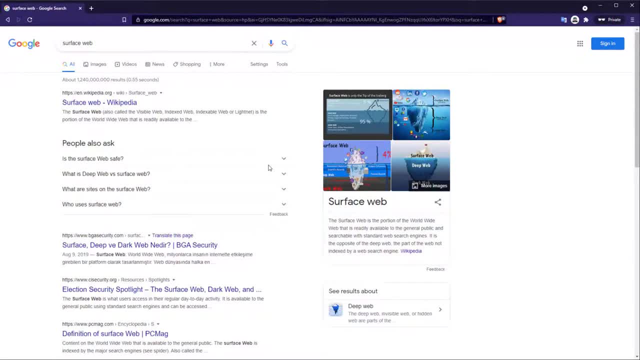 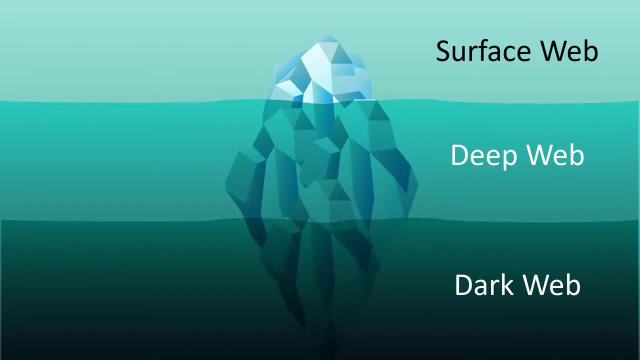 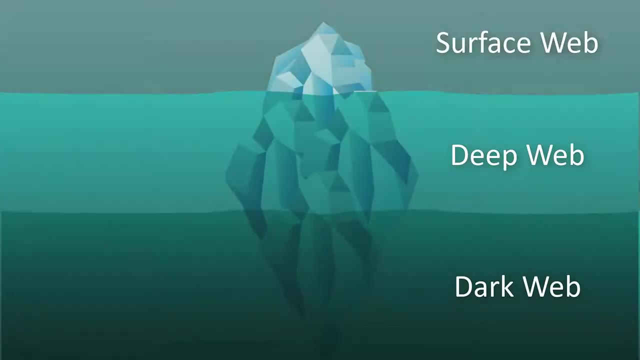 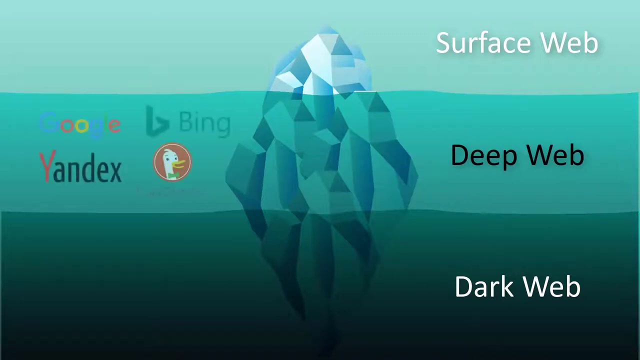 Are websites that have accepted to be able to be indexed by standard search engines such as Google, And they represent a very small fraction of the network when considering the entire web. Deep web, Unlike the surface web, it represents all kinds of web content that search engines do not index. 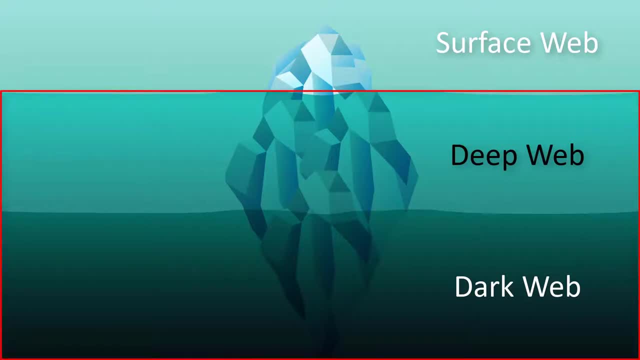 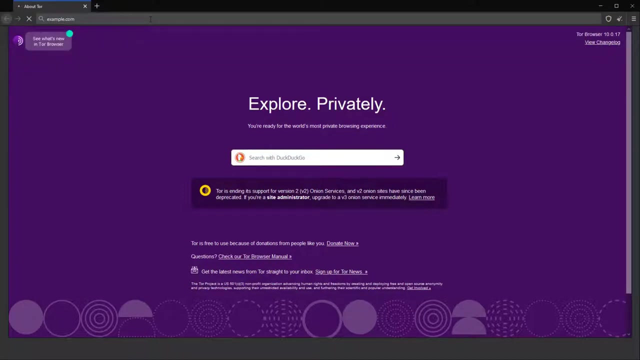 It usually represents the overall web area where search engines find it not worth indexing or where websites directly block indexing to escape search engines. So to access the website in this area, the web addresses must be entered directly and the conditions required for the connection must be met. 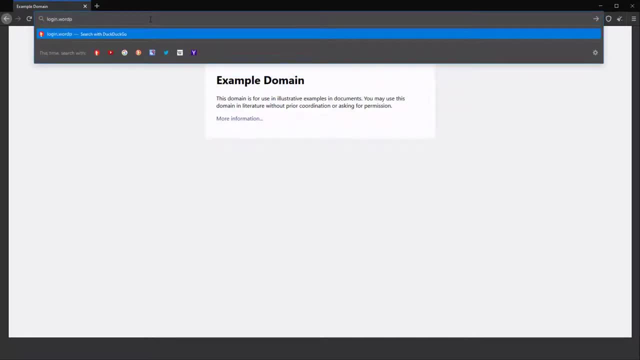 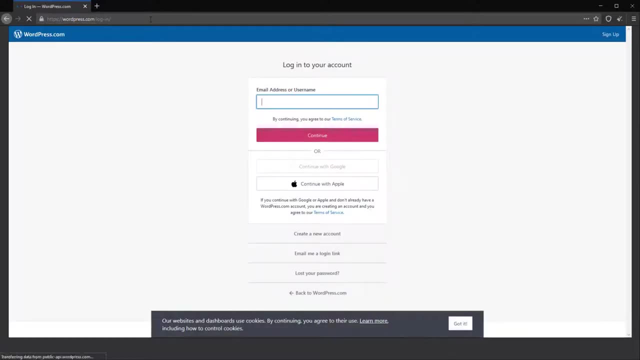 For example, the admin panels of the site are generally excluded from the indexing of search engines for security reasons. Those while the admin panel of the site can't be found through the search engine, If we know its exact address, we can access the admin panel. 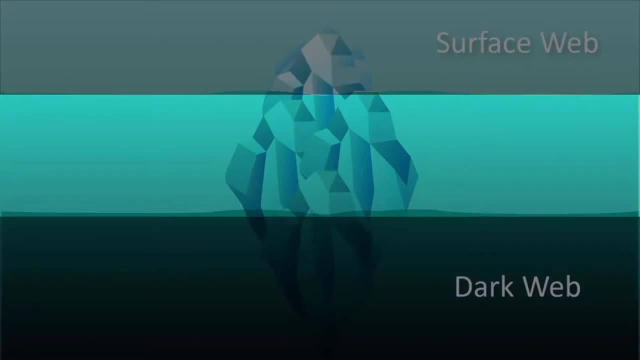 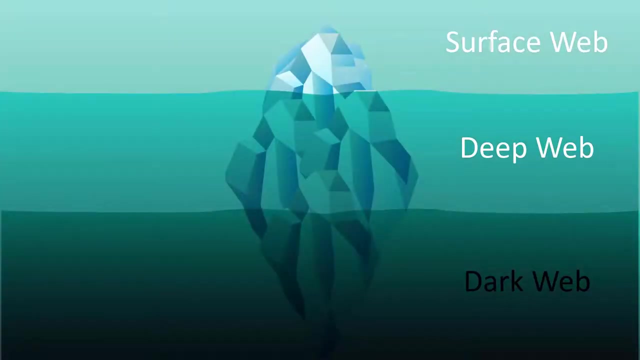 In other words, the deep web area which is excluded from the scope of standard search engines for this and many other reasons, is called deep web. Dark web, Similar to deep web. the dark web, on the other hand, is outside the scope of search engines. 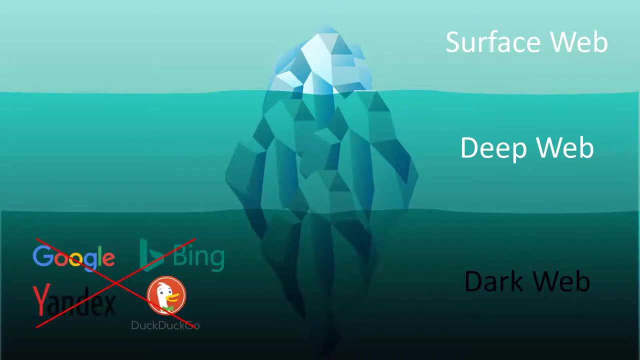 On the surface web and, since it's located on the Tor network, it is only accessible over Tor. Dark web is the general name of the web addresses with onion domains kept on the Tor network and where privacy is at the forefront- Websites with this onion domain. 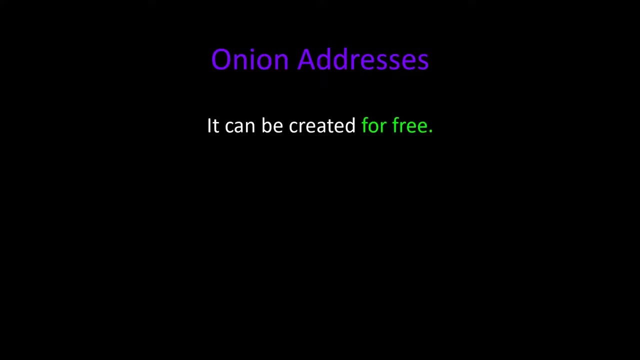 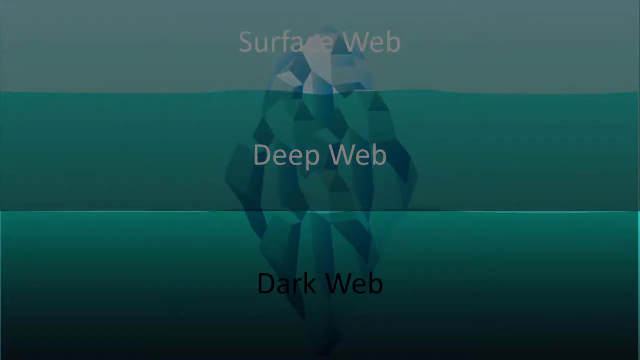 can be created free of charge by anyone and published anonymously. The fact that websites can be created anonymously and free of charge has made this web area more vulnerable to abuse. Since this web area is mostly used malicious purposes, it has been named as dark web. 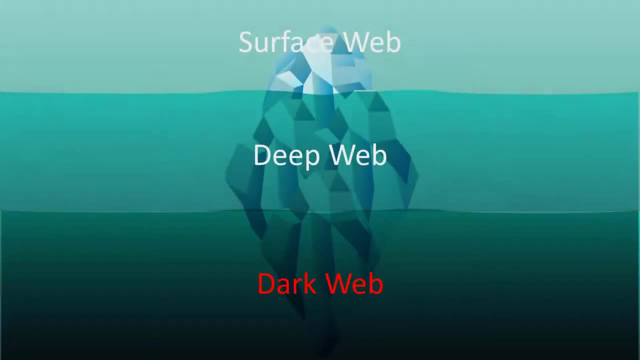 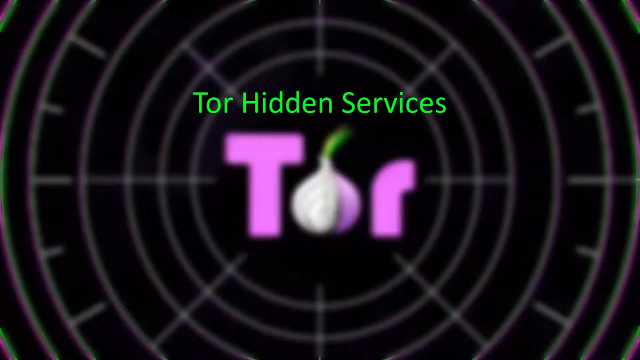 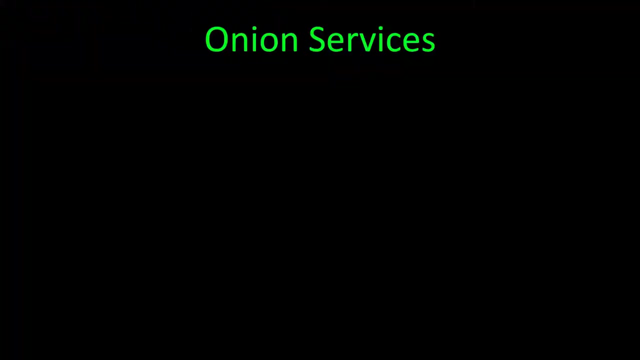 In addition, websites that are in the dark web, that is, can only be accessed through the Tor network, are also called Tor hidden services or, more modernly, onion services. If we need to talk briefly about onion services with the onion service, 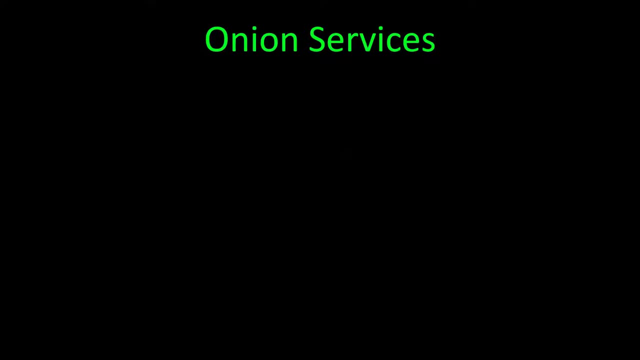 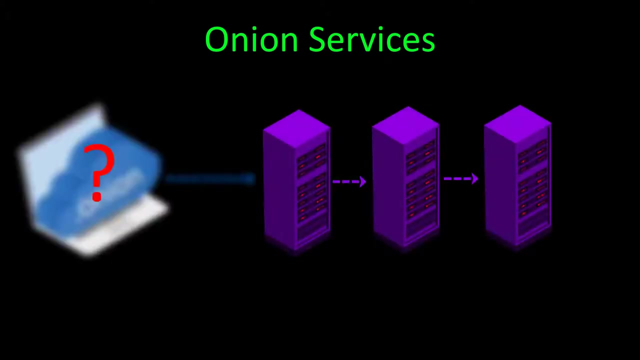 you can publish a website over the Tor network without any third-party service provider for hosting or domain service. Moreover, because the entire connection is routed through the Tor network and encrypted, you can remain anonymous while publishing over the onion service. In short, this is the working structure of the onion service. 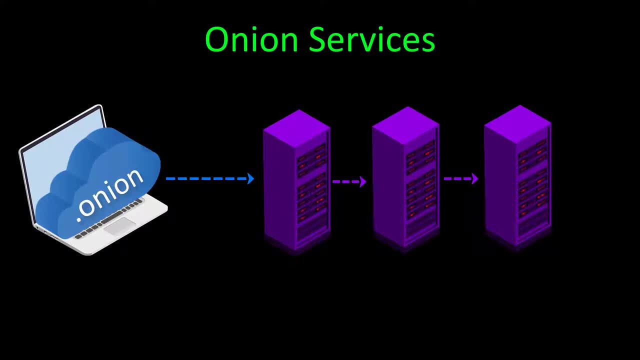 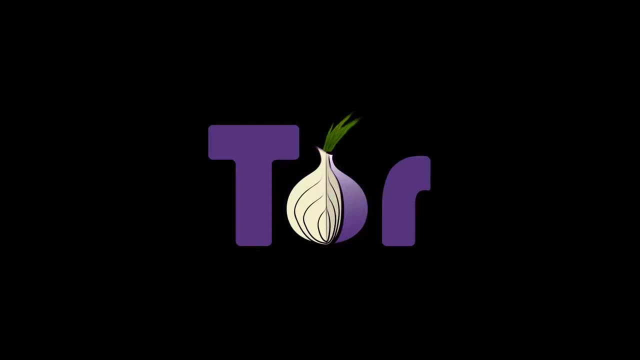 We will be talk about this service again in a part of the course. While explanation we have made so far, we have briefly mentioned many concepts that you need to know in general. In addition, we will be talk about these issues in more detail in the course. 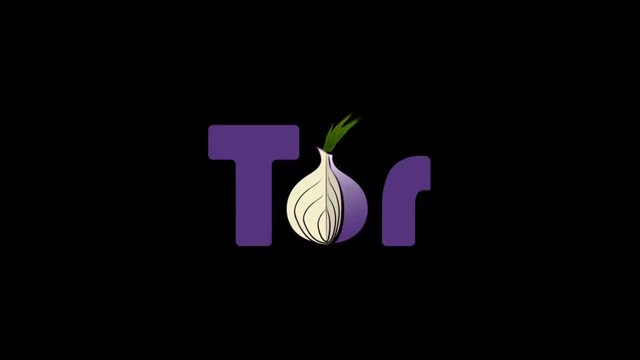 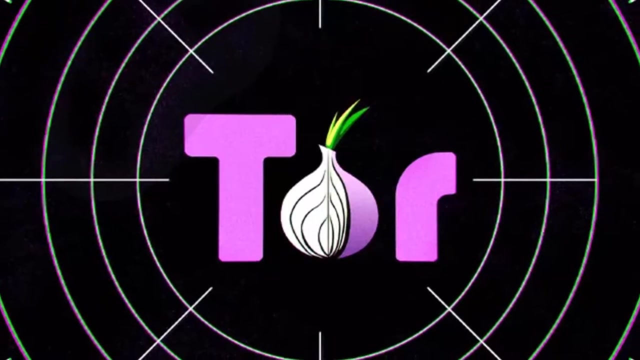 as the time comes. Now let's continue with the explanation by considering the various tools and methods by which you can access the Tor network. Accessing the Tor network: Although there are more than one method to use the Tor network, will be considered three different ways. 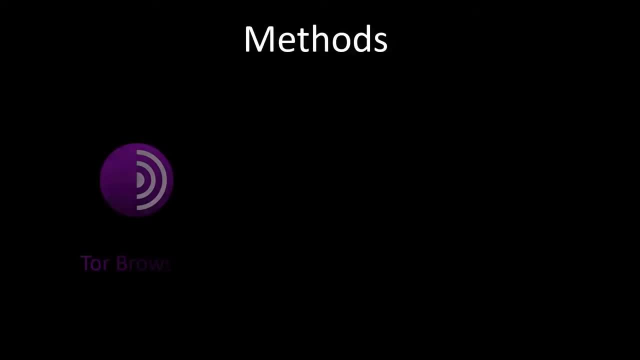 to securely access the Tor network. These are Tor Browser: TailOS. Honix via KubeOS Tor Browser: it is a simple but not very safe method. Tail Operating System: it is a good method in most situations. Honix via Kube's operating system. 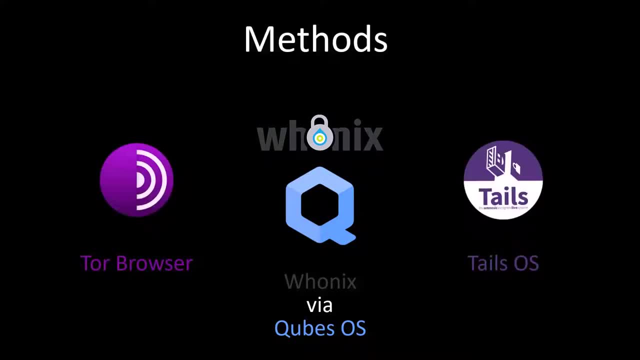 it is the method considered the safest. In the rest, of course, we'll be explain all these methods one by one. While explaining the methods, we'll be talking about the advantage and disadvantage of these methods. In this way, you will know which methods. 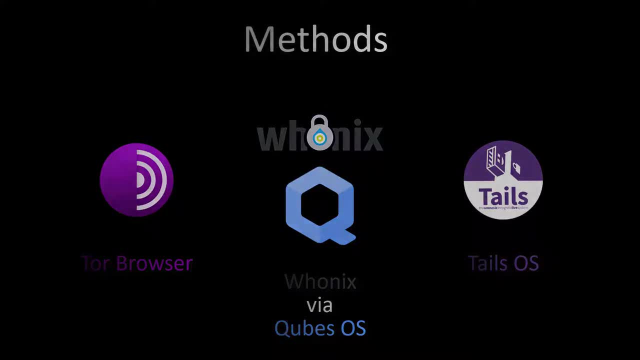 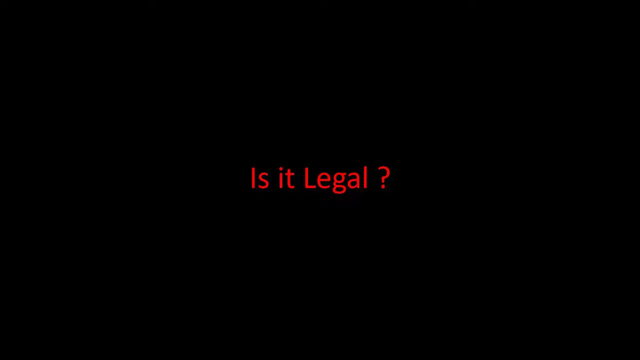 will meet your needs more accurately when you need it. Is it legal to use the Tor network? Finally, let's clarify whether it's legal to use the Tor network. In fact, whether it's legitimate depends entirely on what purpose you are using the Tor network. 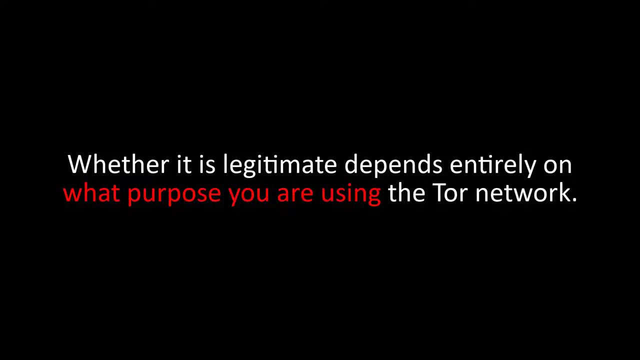 So in most cases you wouldn't be accused just for connecting to Tor network. Just being connected to Tor network is not a direct crime. However, you are responsible for all your activities on the Tor network. If you have criminal activities and you are caught. 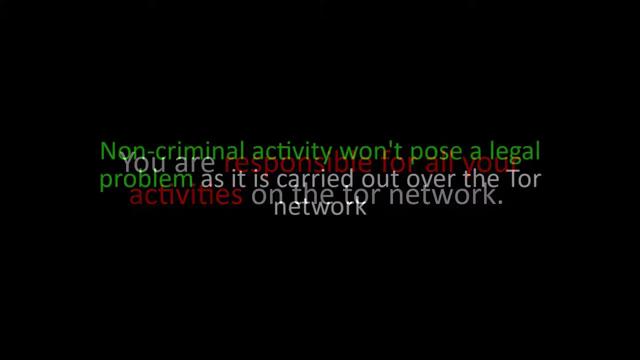 it is quite natural that you will be accused. In summary, any non-criminal activities won't pose a legal problem as it carried out over the Tor network. In this course, your aim is to gain the basic awareness that will enable you to protect your personal data. 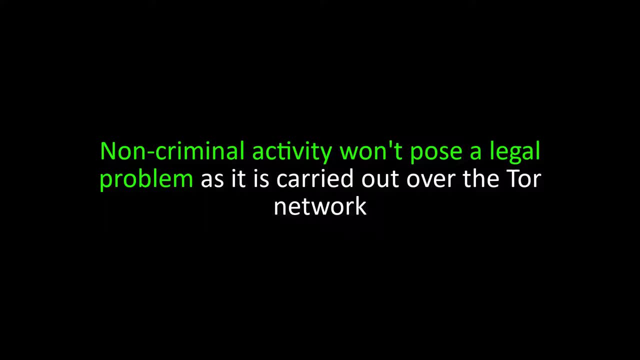 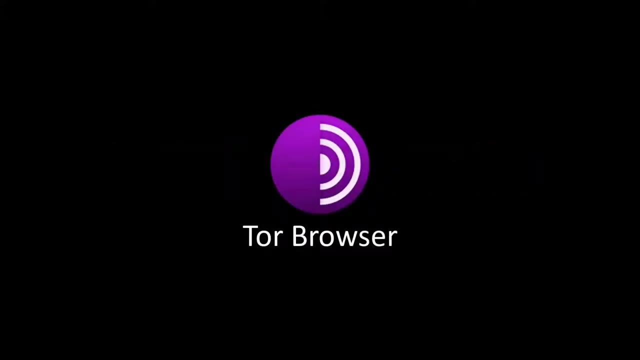 No one can promise you 100% anonymity. If it does, it is not true. You will already see the limits of anonymity and privacy in this course. In the next section we'll be continue with explanation Tor Browser, which is first use method. 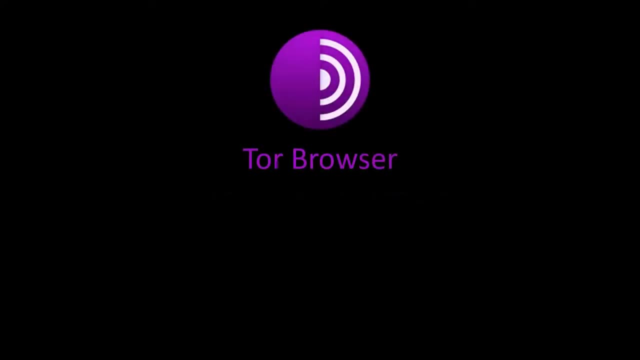 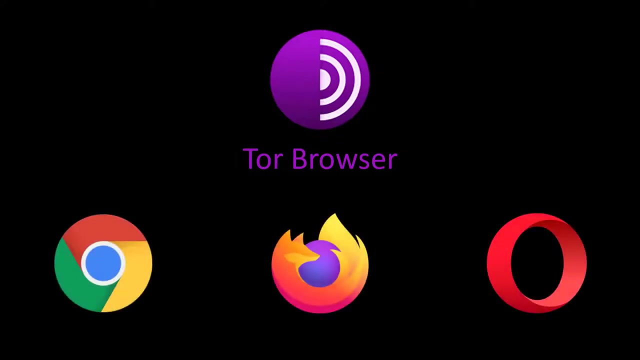 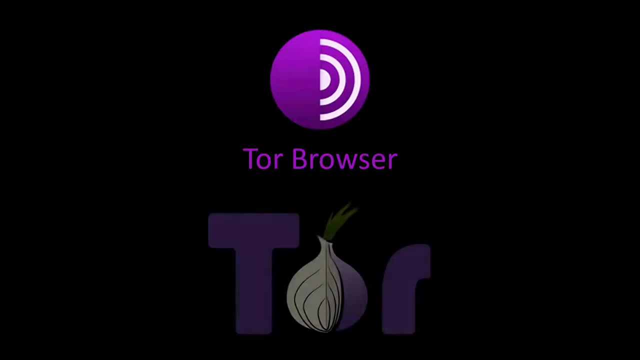 What is Tor Browser? Tor Browser is basically a tool that help us surf the web, just like Chrome, Opera, Firefox or any other web browser. However, unlike standard browsers, it throws all internet traffic through the Tor network, In this way bypassing all restrictions. 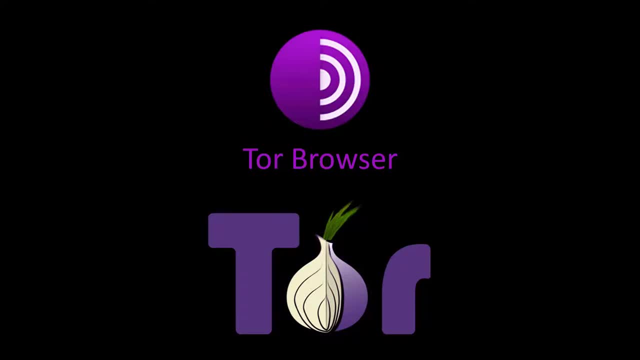 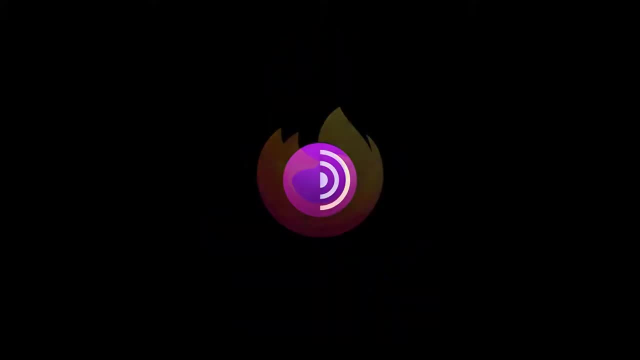 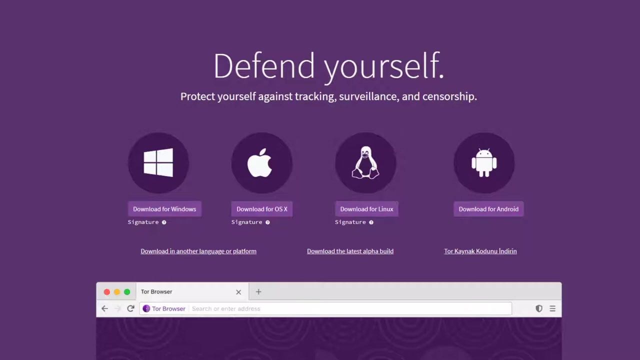 it enables us to securely access surface web and hidden services, called dark web, through the Tor network. Tor Browser was created by customizing the Firefox browser for the Tor project. It's a practical solution for connecting to the Tor network via various operating systems, Although there is no officially supported. 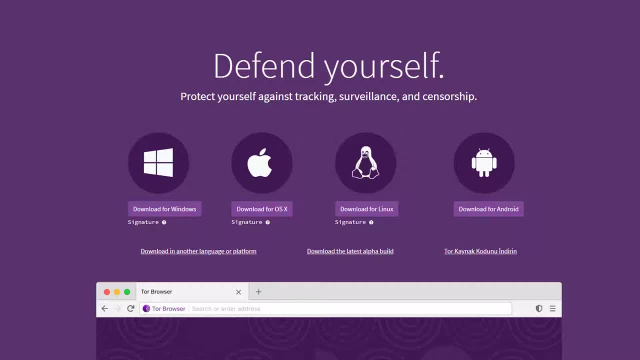 browser for iOS, yet there are browsers with officially supported for Android, Windows, Linux and Mac. Unlike regular browsers, Tor Browser come with various restrictions And security measures, apart from routing all internet traffic through the Tor network. So it is fully optimized. 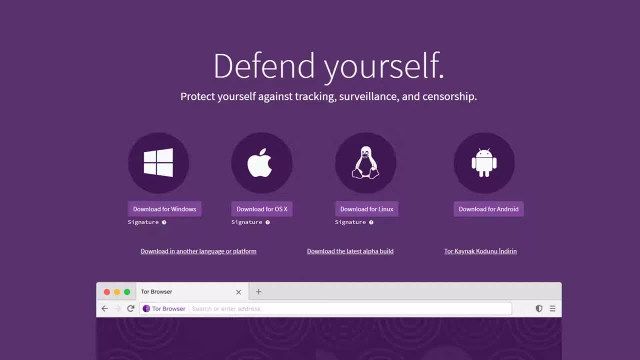 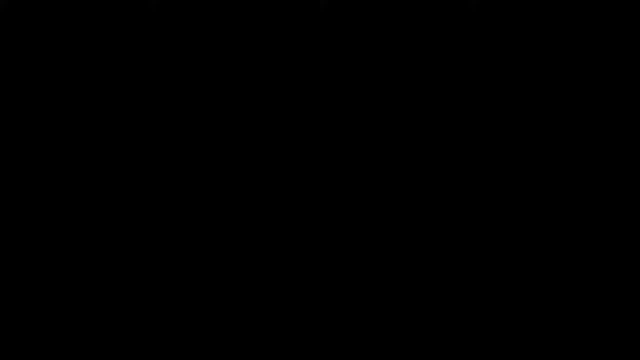 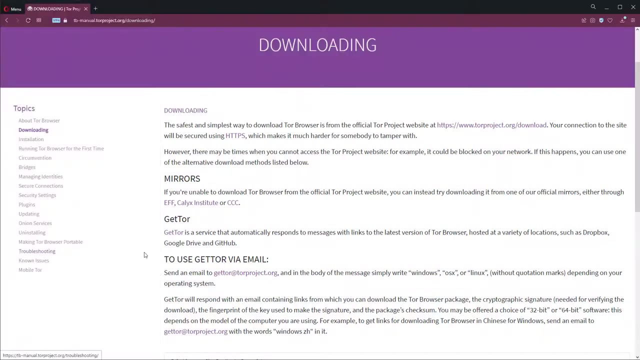 for security and privacy. Before going into the details of Tor Browser usage, you should first learn where and how to download Tor Browser. Downloading Tor Browser: You have multiple alternatives to download the Tor Browser. All these alternatives exist, so you can securely download the Tor Browser. 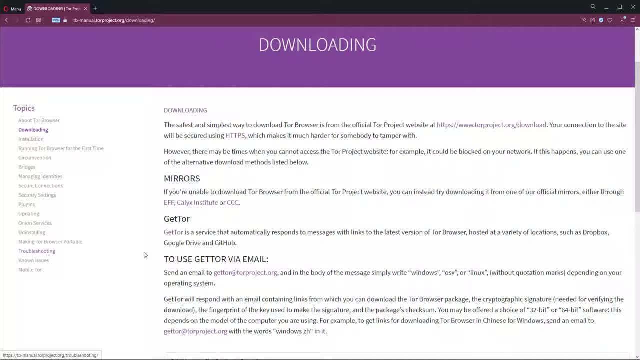 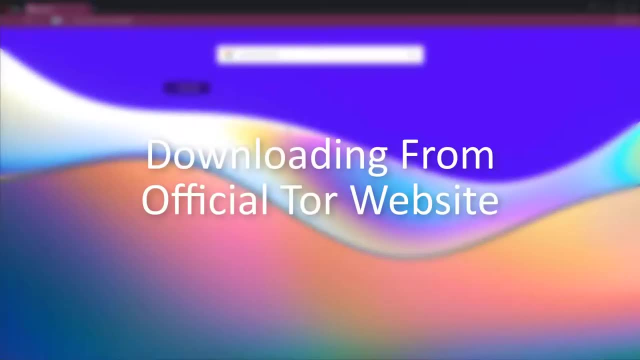 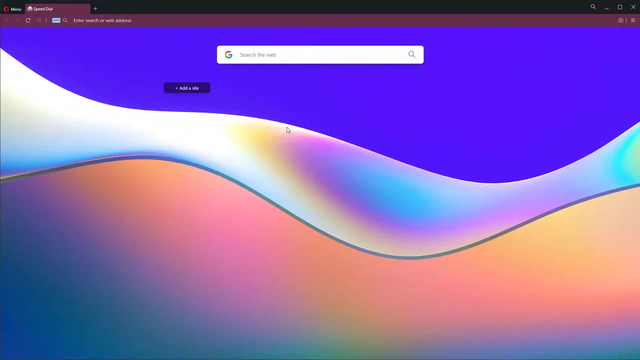 over any network where access is restricted. Let's take a look at the download alternatives in order. Downloading from the Tor official website. The most basic and common method used to download the Tor Browser is to download the versions suitable for your system from its official website. 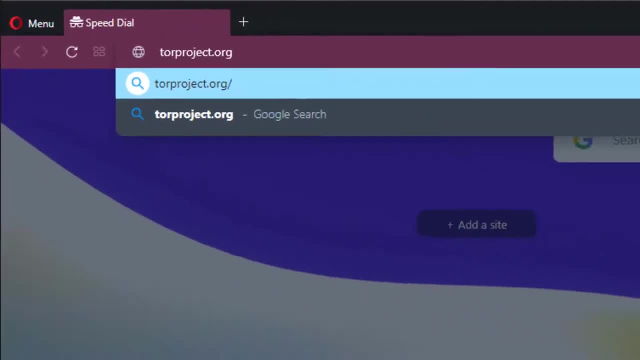 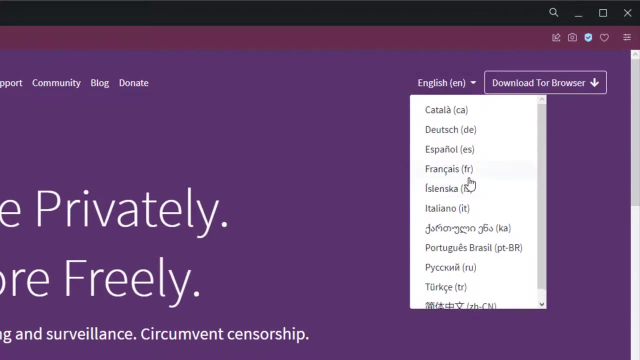 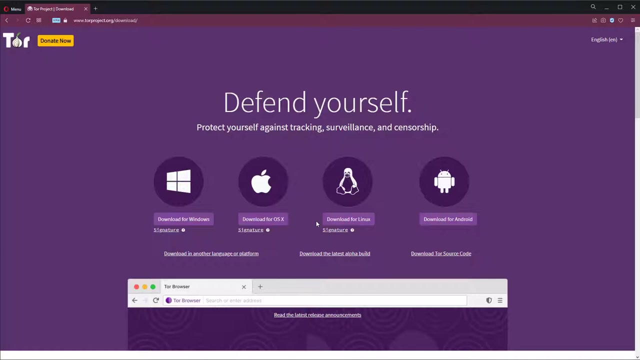 To download browser. firstly visit the torprojectorg. If you want, you can choose the language of the website as your native language and understand what is written more clearly. Click the Download Tor Browser button to see the download options, As you can see here. 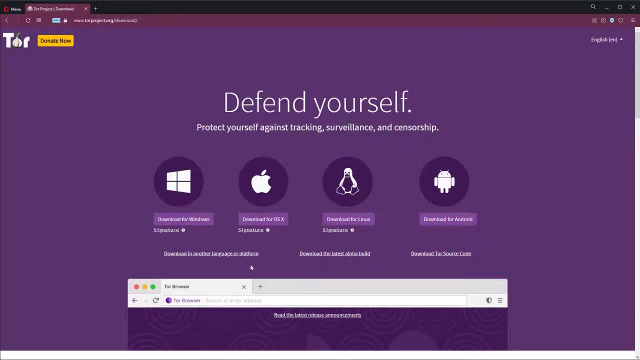 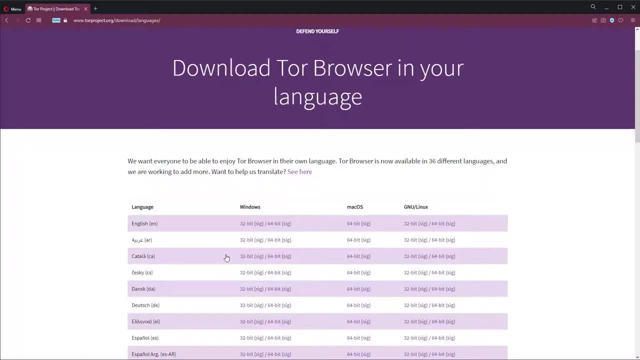 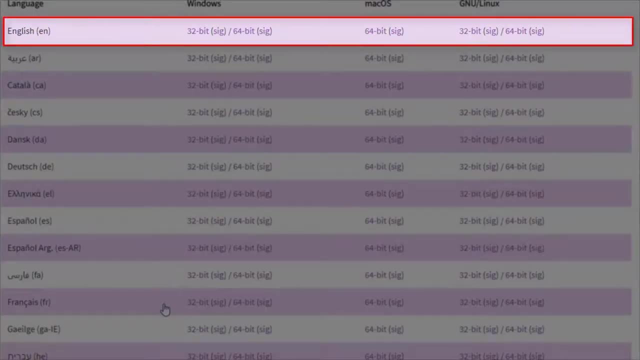 there are download links with multiple language options for multiple platforms From here, just click on the link to download the appropriate versions for your operating system. At this point, my suggestion to you is that you prefer the English installation package, which has a much more. 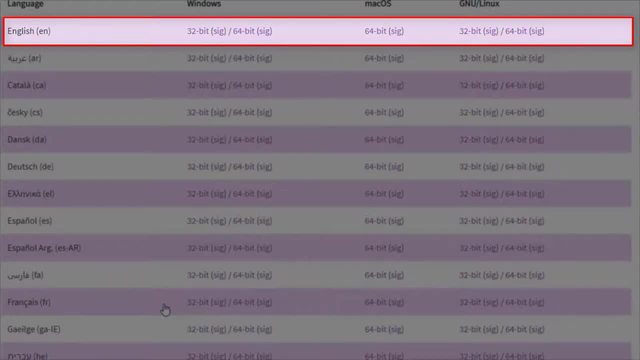 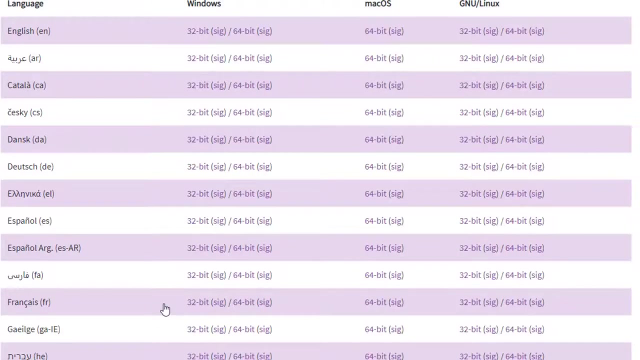 general use, rather than packages in other languages that you know or can be associated with you. In this way, you can make your real identity much more uncertain. with a much wider browser version, You can still choose the language pack you want If you think you have difficulty. 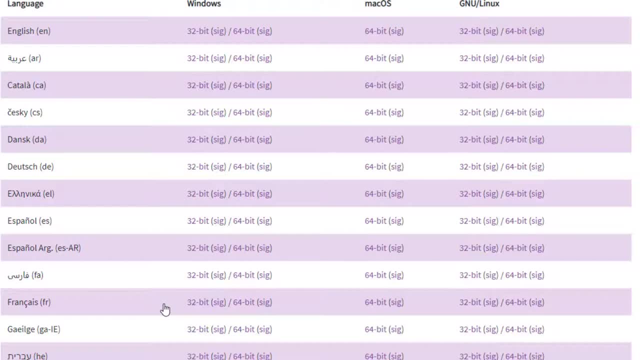 or, if you prefer, for use where your anonymity is not so important. Your native language can be preferred to use, at least until you get used the Tor Browser. Just click on the link to download the version suitable for the operating system. you will install the Tor Browser on. 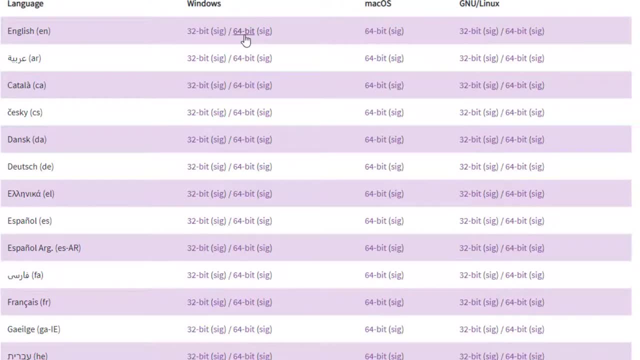 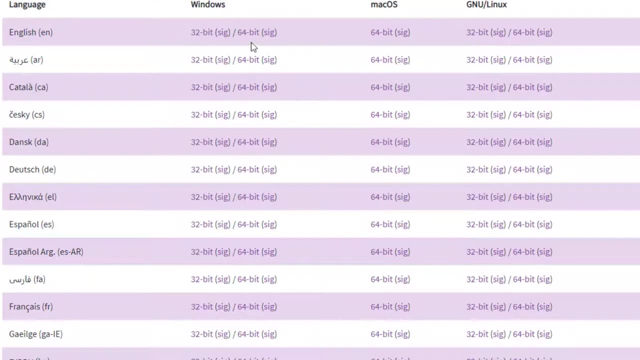 For example, since I will install on a Windows 64-bit system, I click the link here And also make sure to save the signature file of the installation file you downloaded by right-clicking on the link that sync and clicking as You will be using this. 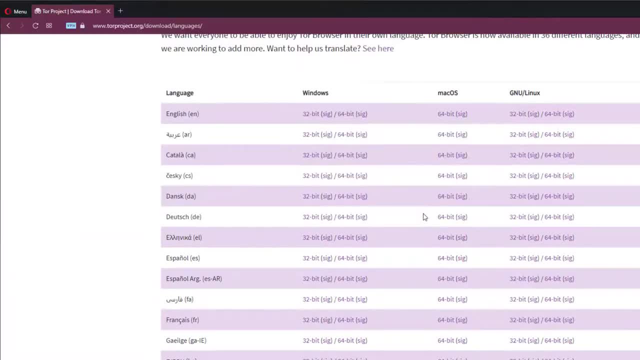 signature file during the installation phase to test the safety of the setup file. We discussed the first download alternative. However, despite being the first, this is actually most prevented alternative. The country you are in or the internet service provider you use may have blocked the. 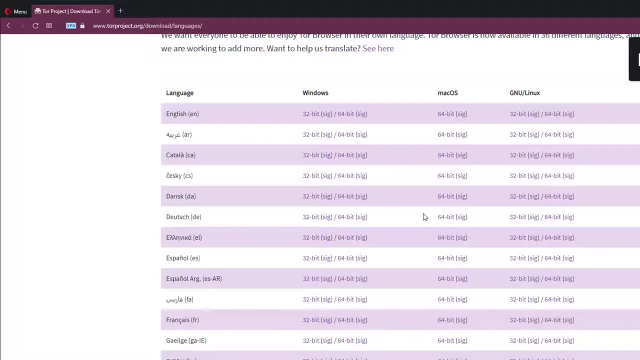 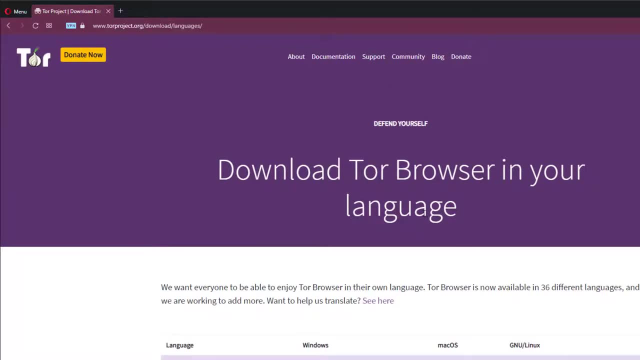 Tor project's websites, So you may not have been able to access the Tor websites while were you following this lecture. In this case, you can either use the second alternative download source or you can download from the websites by using VPN, As a matter of fact. 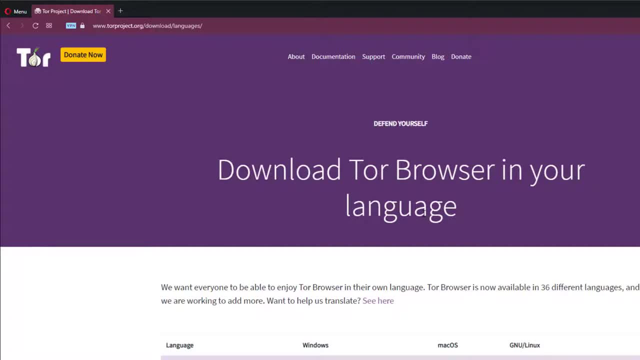 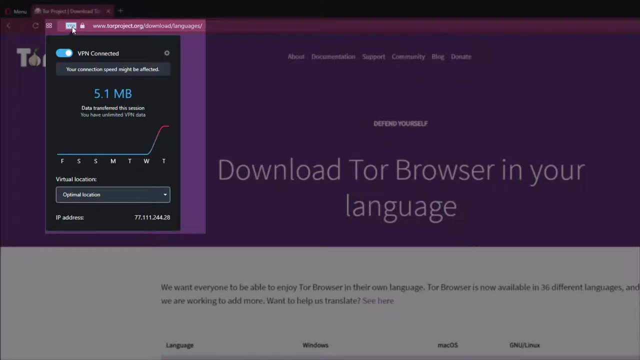 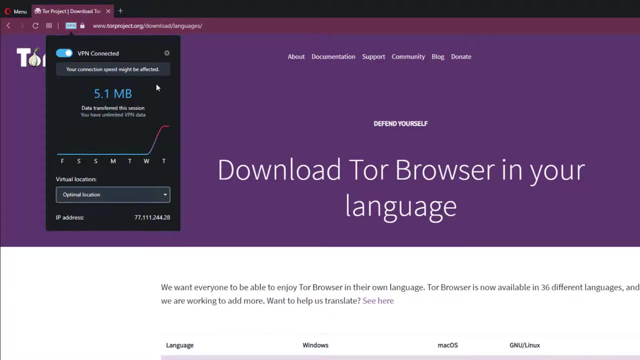 since I had trouble accessing the websites while preparing this guide, I was able to show the processes by accessing the websites through a simple VPN application installed in my browser. So if you wish only for downloads, you can use simple VPN extensions that can be installed. 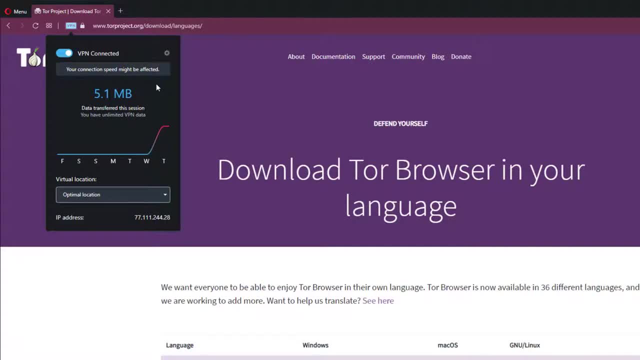 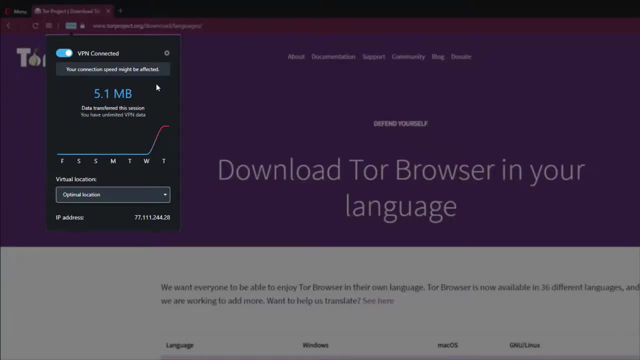 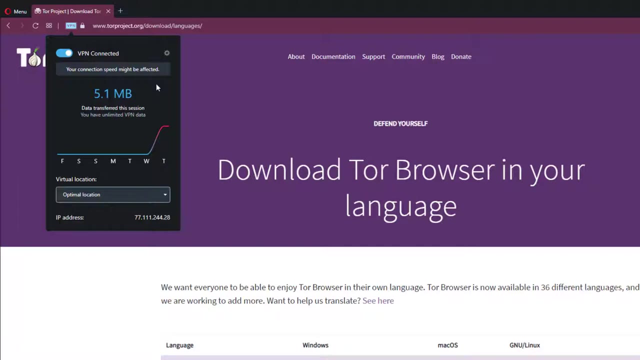 on browsers, or you can try second download method. Also, by the way, I would like you to know that such free VPN services running on the browsers are not secure and there keeps logs your personal data. Apart from this, I recommended you read the terms. 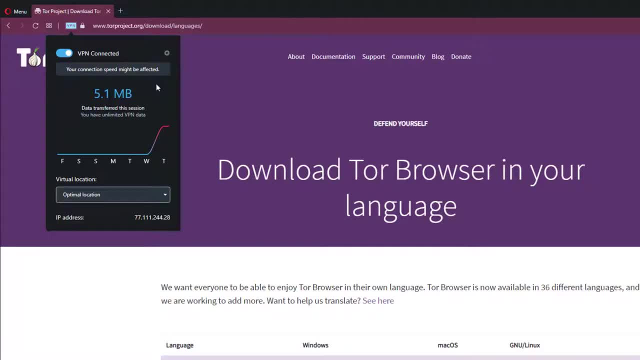 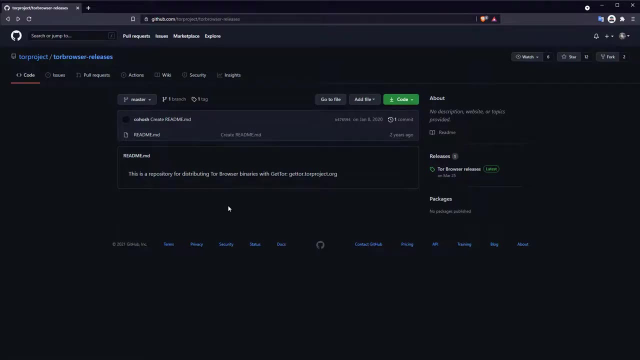 of the use before using such free services and find out what information they collect about you. Leaving aside the use of VPN for now, let's consider second alternative source: Download on GitHub. In this alternative, which provides a much more uninterrupted access compared to the first, it is possible. 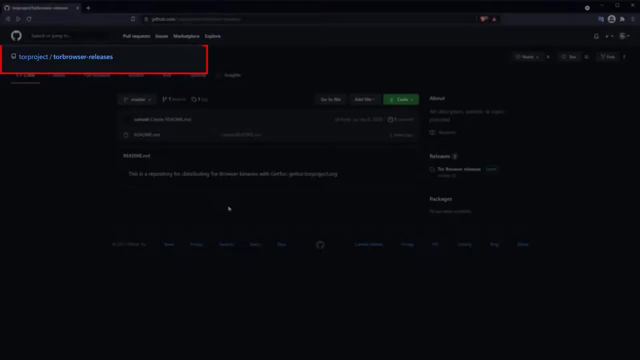 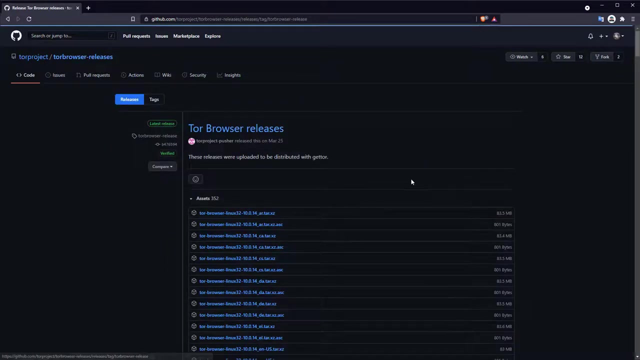 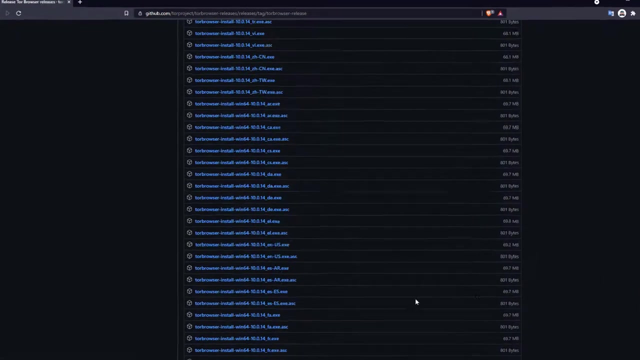 to access download files on GitHub. Firstly, you should visit to the Tor project's GitHub source. Click on the release tab to download the sources published on the GitHub. As you can see, all downloadable files are here. Here you can download the setup file suitable for. 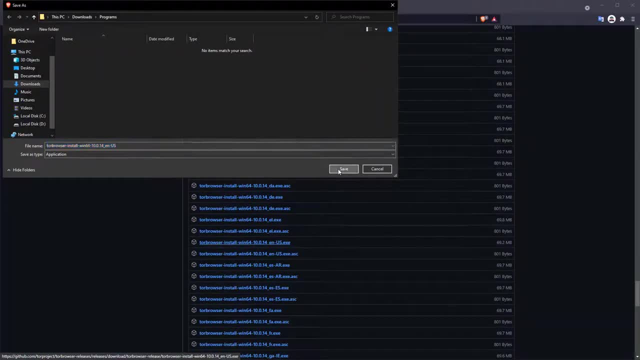 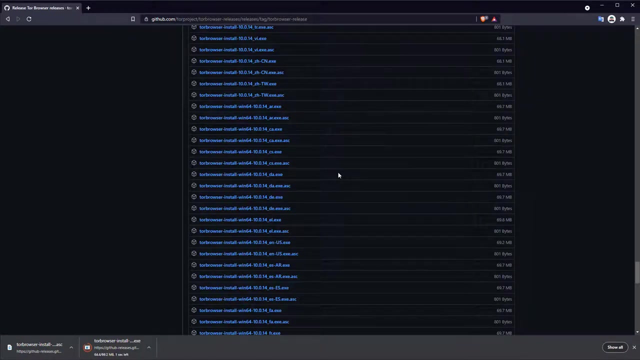 operating system you are using. Also, please don't forget to download signature files with ASG extensions along with the setup file you downloaded. As I said before, you will be using the signature file during the installation phase to test the safety of the downloaded. 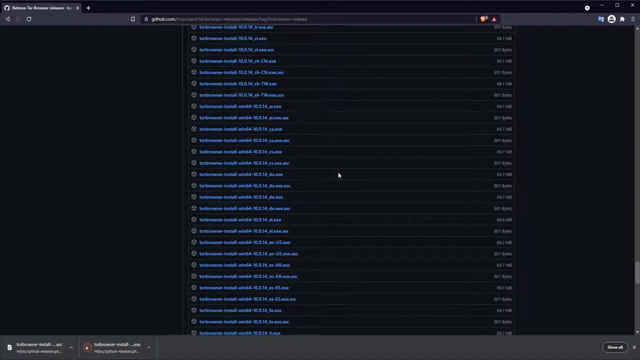 file. If the GitHub platform is blocked in your country or somehow you have lost access to the Tor installation files on the GitHub, you can download the files you downloaded from the Tor installation files using VPN or the next alternative method, Download via email, If in any way you can. 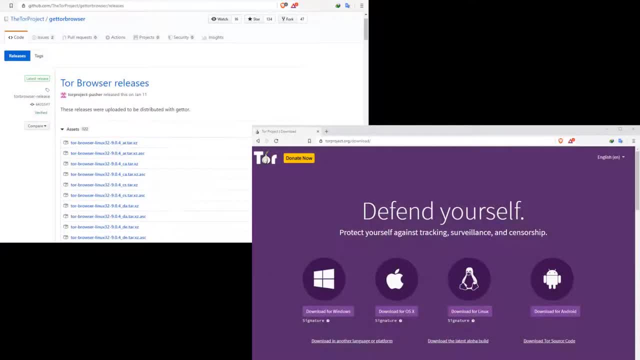 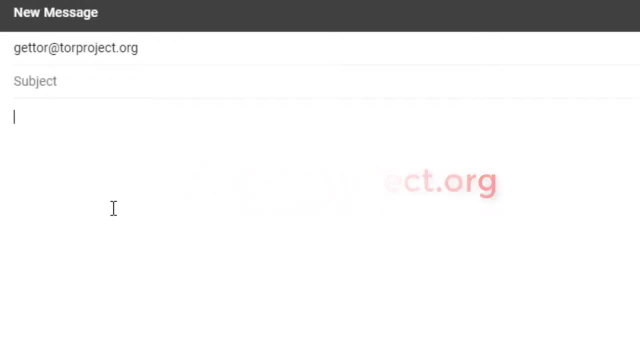 access the Tor browser download sources with the previous methods. just send an email to gettor at torprojectorg. For example, if I want to download the English version of the Tor browser for Windows, I just need to send to Windows and message You can. 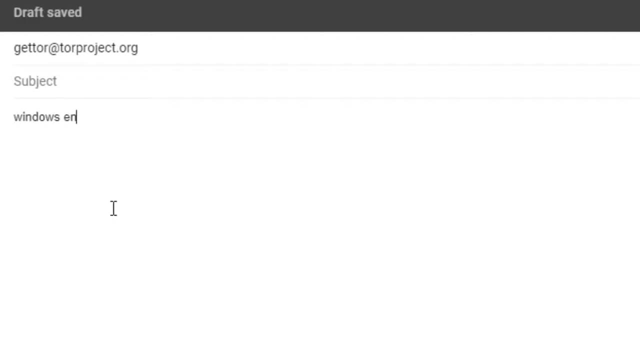 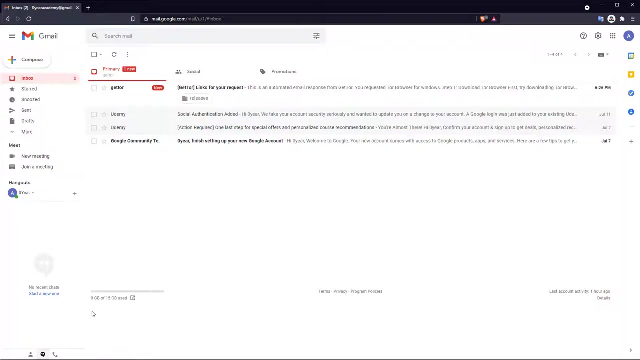 write OS X or Linux instead of Windows, and all of them specify the abbreviation of your preferred language pack. For example, if you want Tor browser for macOS in Arabic, you can send OS X R message. As you can see, I soon received the download links in. 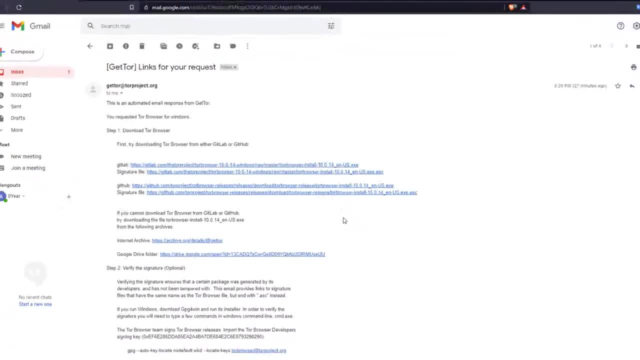 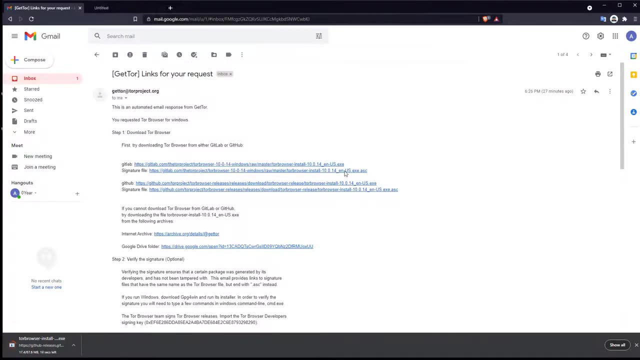 response, including many alternative ways. Now all I have to do is to download the setup file and signature file from here. Depending on the density, the response message may be slightly delayed for you. So even if don't get an immediately response, it's. 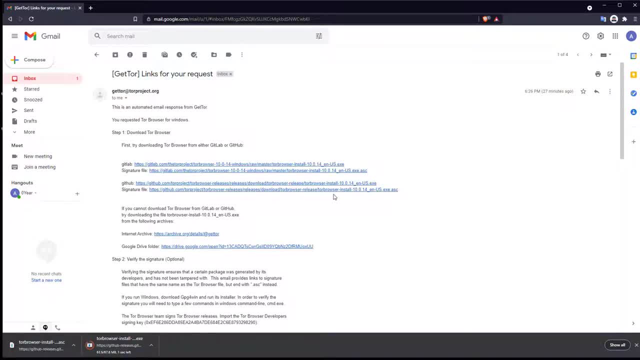 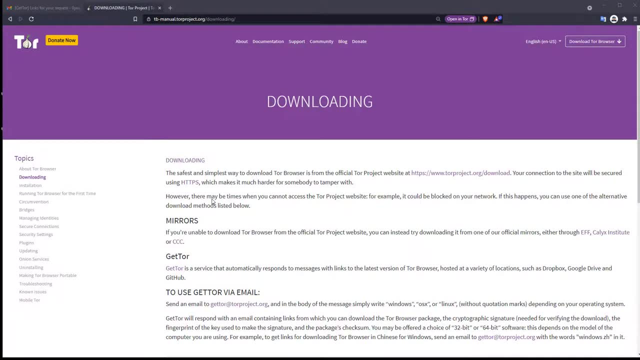 okay, All these methods and addresses that I have explained so far may change over time for different reasons. In such a case, you should check out the download guide on the Tor official website. You can easily read many documents and guides, as it already has. 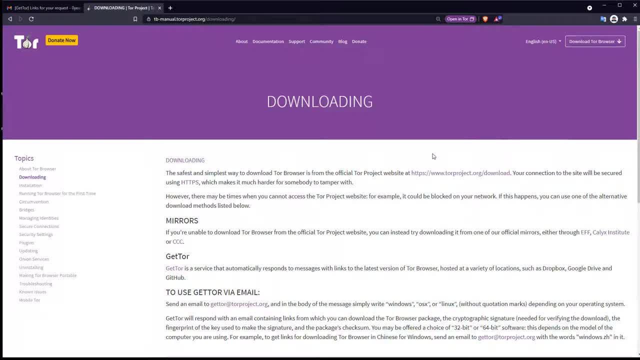 It has your native language support. There may be some of you wondering, or even critic, why I have just explained a simple download at such length. The reason for this situation is in the structure of the Tor project, Since the Tor project has always struggled with censorship by nature. 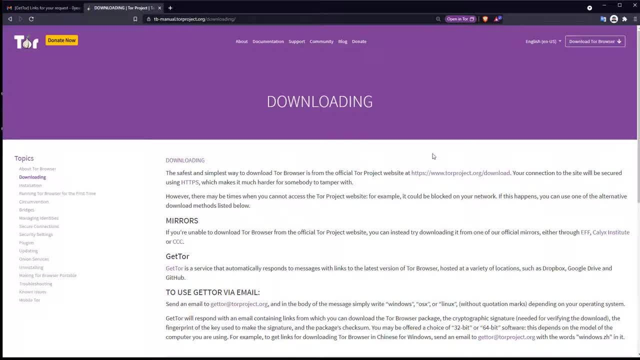 it has always had to create alternative ways. I've explained it this lengthy because I think will be useful for the known alternative ways to access sources in all situations. Ultimately, you learned how you can obtain the files you need to download for the installation process, including alternative. 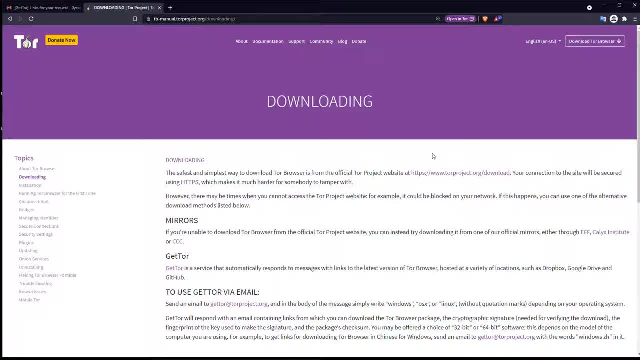 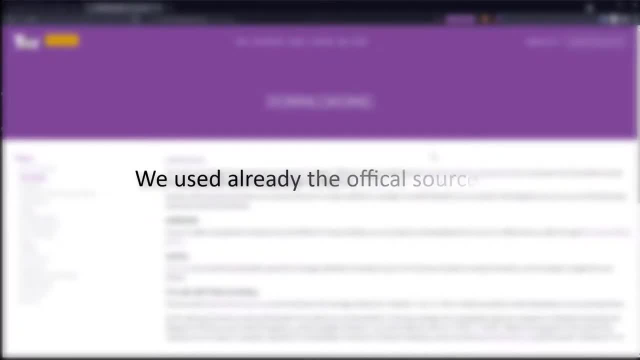 ways. Before installing the Tor browser, you need to verify the setup file. But why do we need to verify setup file? Were the sources we used not already the official sources of the Tor project? Let's answer this question in the next lecture. 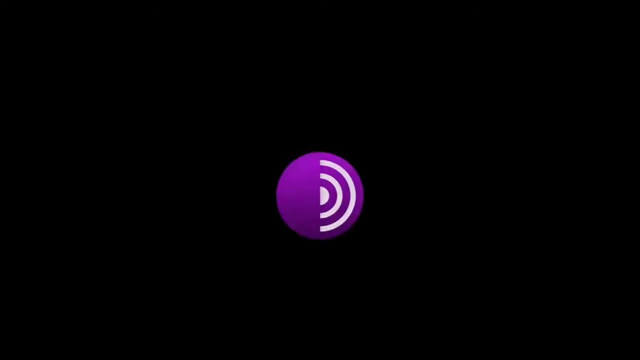 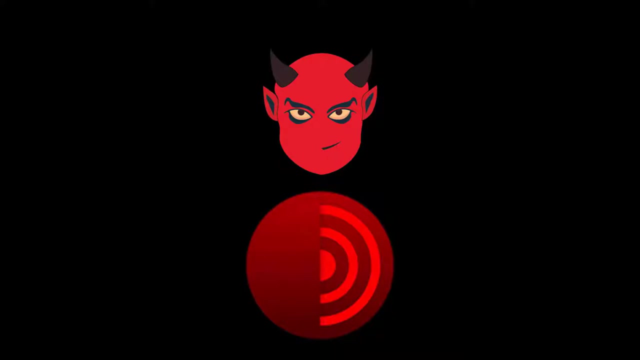 Verifying the installation file. Regardless of where you downloaded the installation files, the contents of the installation files may have been changed by attackers before or during the download process. For example, a file you downloaded from the Tor project official websites may have been replaced by a malicious. 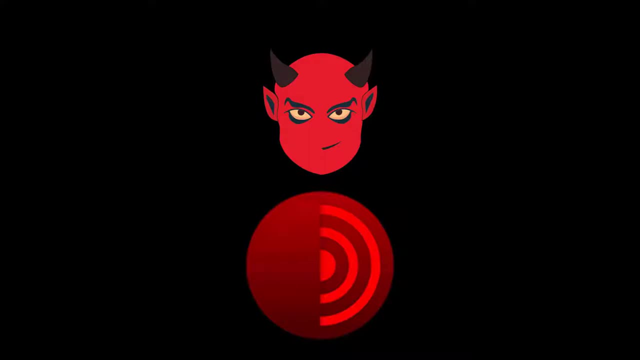 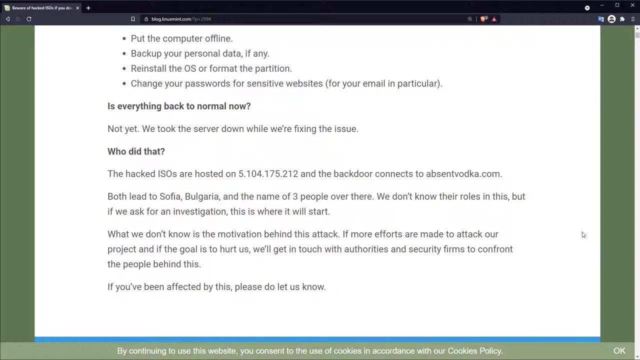 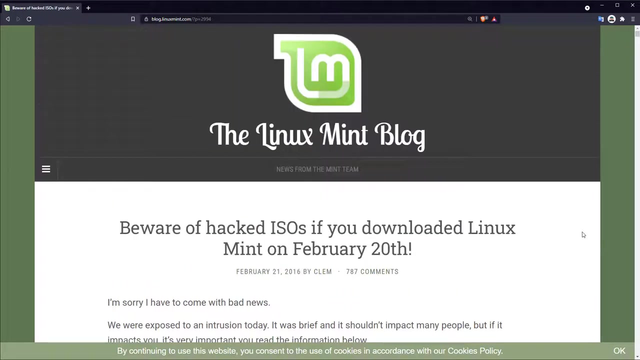 version by attackers, Although such a possibility seems unlikely to many. I would like to remind you that in 2016,, Linux Mint servers were hacked and installation image files were replaced with malicious files, and many people downloaded and installed malicious files of Mint. In addition, even 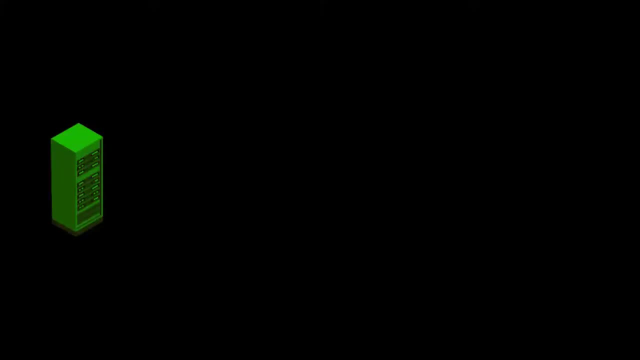 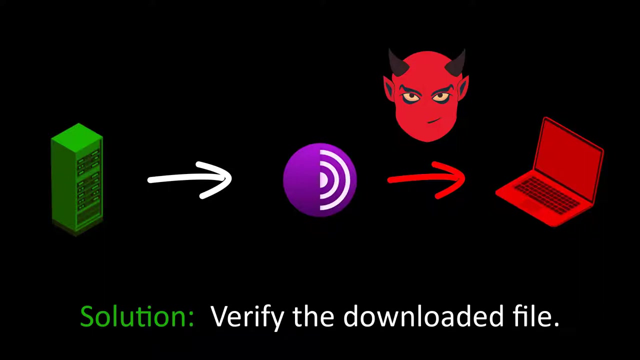 if the direct download source is not hacked at any time during your download process, the files have been changed with the malicious version by the attackers who control your internet connection. The surest solution to these and similar scenarios is to verify the downloaded file For verification. 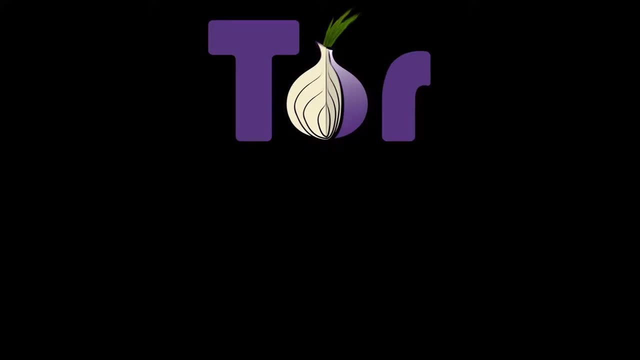 you need to compare the digital signature published by the developers of the Tor project with the signature of your current installation file. Digital signatures are unique signatures only assigned by developers to the respective version of the program, Since even the slightest change in the content of installation. 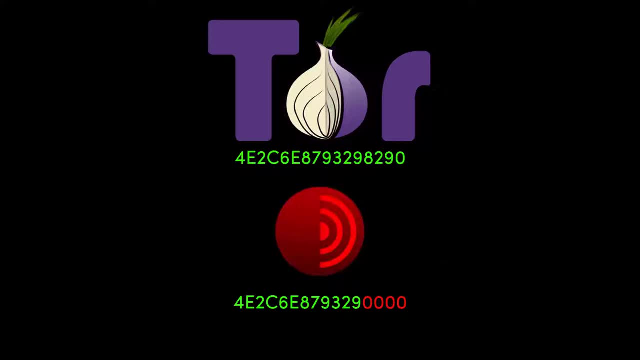 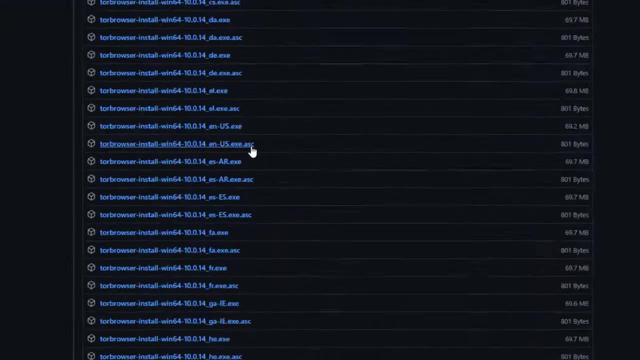 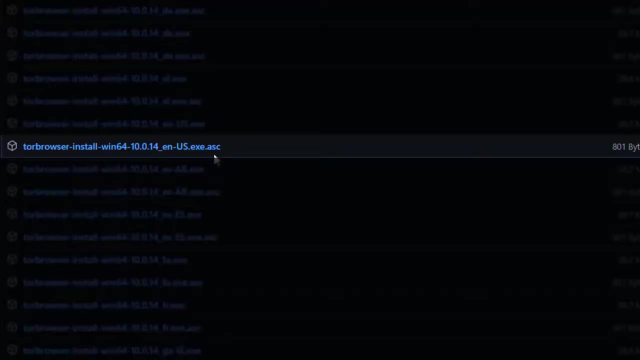 files will cause the signature to change. you can easily test whether the file has been changed or not through the signature When you downloaded the setup files. remember I mentioned that you need to download signature files with ASG extensions in addition to setup file. These: 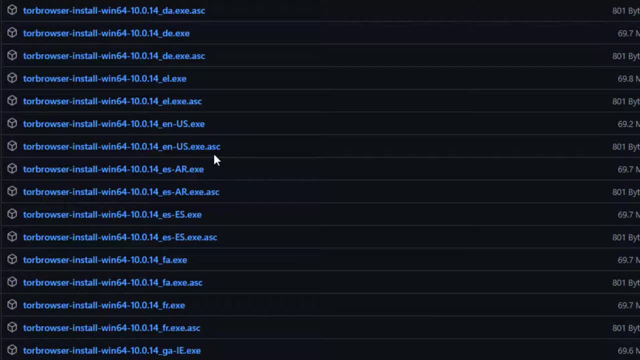 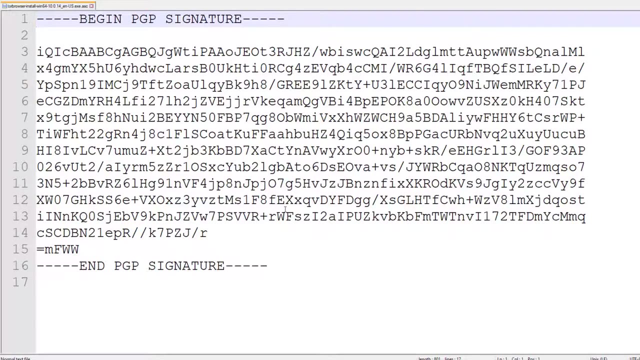 ASG files are actually signature files created with PGP encryption protocol. This file contains a uniquely generated key. Thanks to this file, we can test whether the content of the program has been changed or not. If you haven't downloaded this signature file, go to. 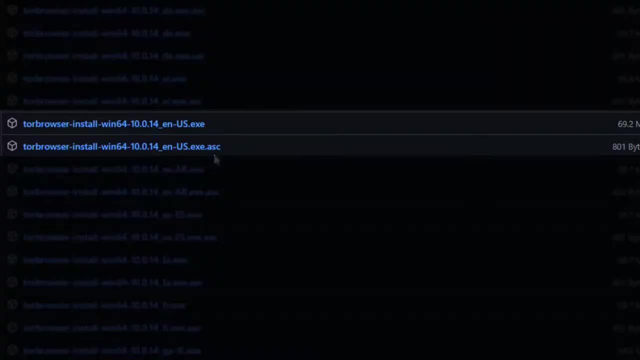 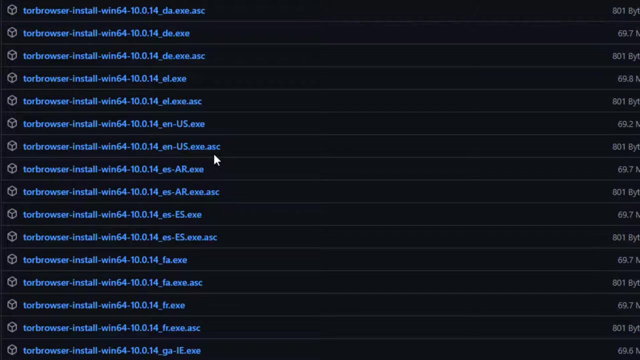 download source and download the signature files of the Tor browser version you downloaded. To avoid problems during verification phase, make sure download the signature files of the exact Tor browser versions you downloaded earlier. Otherwise the verification will fail. Please don't worry if the terms I 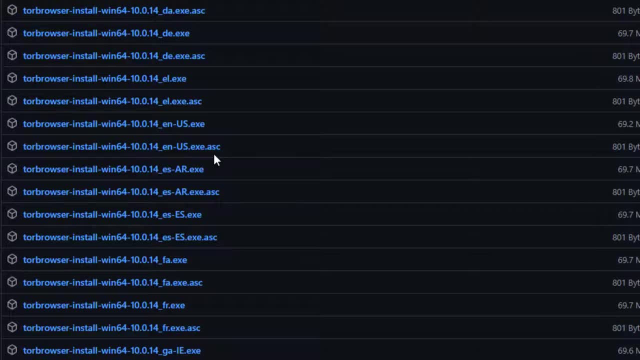 use seem unfamiliar and incomprehensible to you. When you come to encryption section in the rest of the course, I will be talking more about these terms separately. For now you only need to focus on verification process When this process is quite simple. 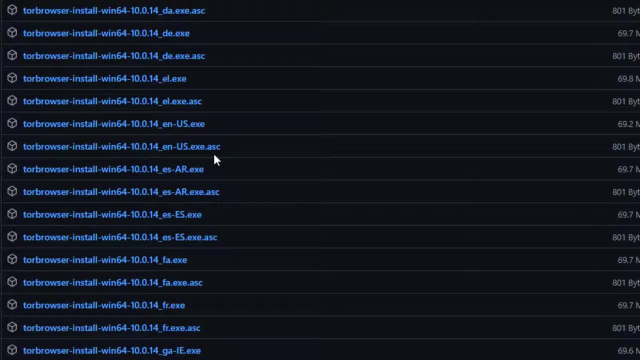 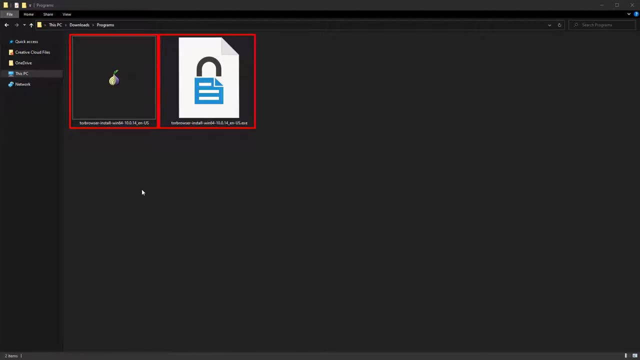 you shouldn't have any problems if you follow the guide carefully. After obtaining the setup file and signature file, you need to use a separate tool to test the setup file, Although this tool differs according to the operating system used, the functions and uses of them. 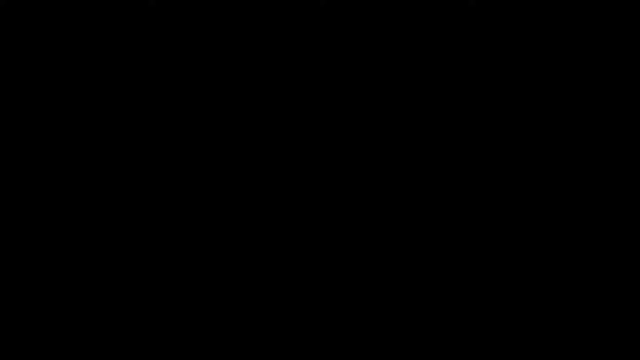 are basically the same. For example, we'll be use gpg4win tool to verify signature files on the Windows. On macOS, we will verify the signature with the tool called gpgsuite. Finally, we will test the signature on the Linux using 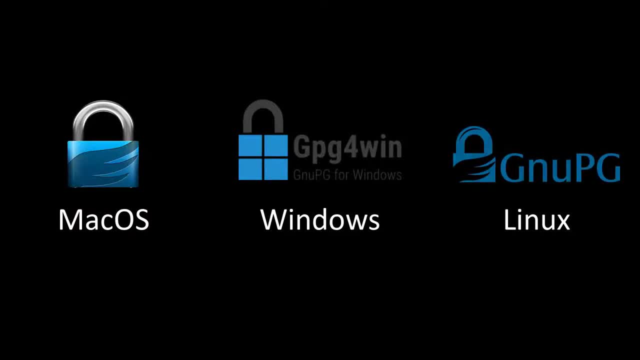 a verification tool that is already installed. We will be handling the verification and setup processes one by one, specifically the operating system, so you can directly throw the verification and installation video for the operating system you are not using. We will already be discussing how you can implement same process. 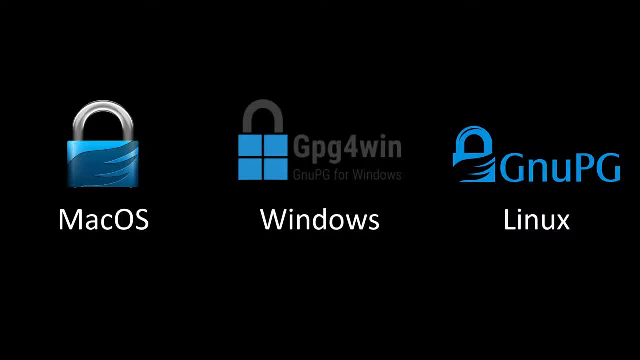 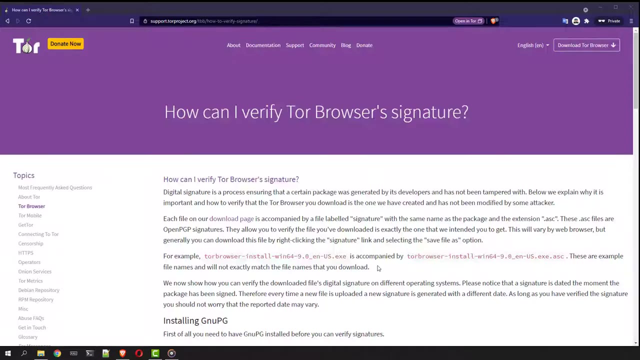 in each of them on the current operating system. Without further ado, let's start by discussing how you can verify and install the Tor Browser installation file on the Windows system. Tor Browser Verification and Installation Windows installation process. you should perform signature check to verify. 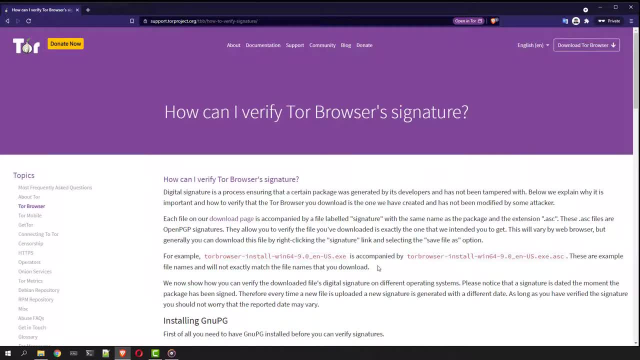 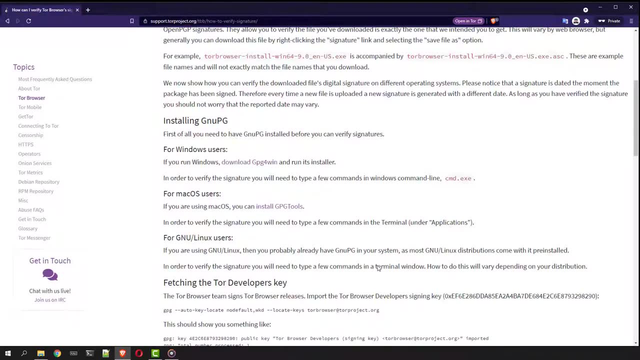 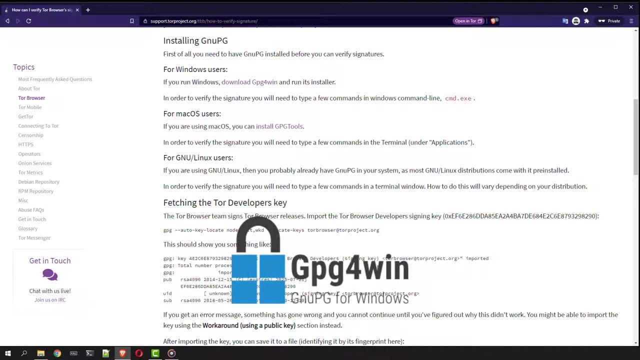 content of the setup file you downloaded. You can use the official guide to follow the verification steps easily. I added this verification guide link in this lecture sources Since you will use the gpg4win tool, as I mentioned before, to check the signature on Windows. 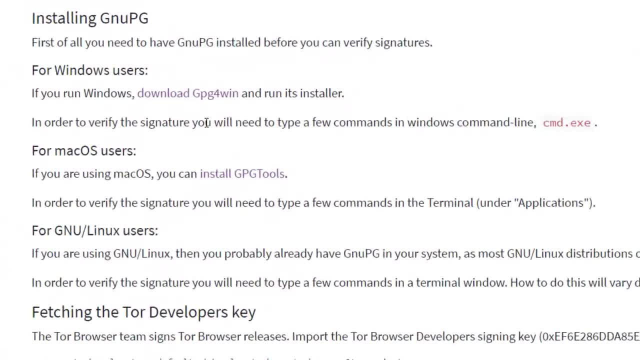 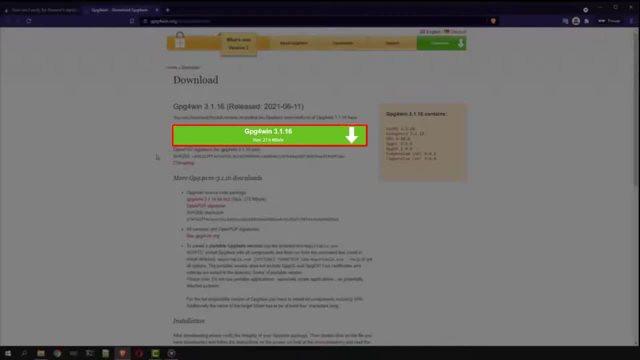 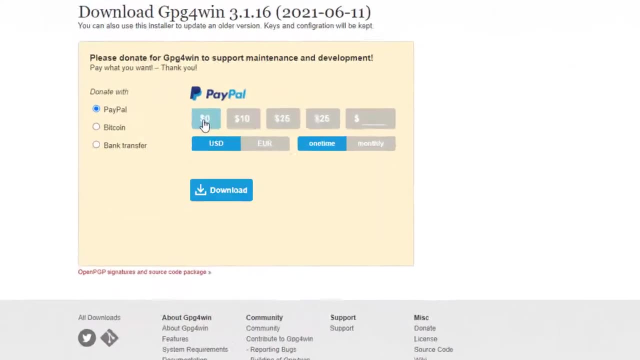 you need to get this tool first. To download the gpg4 tool, open the download page by visiting gpg4winorg. If you want to donate, you can specify the amount you want here. If you are not going to donate, 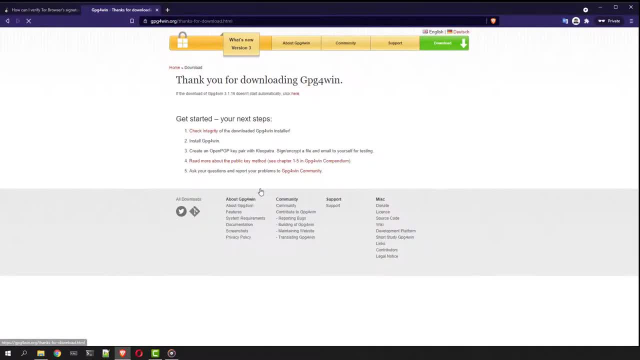 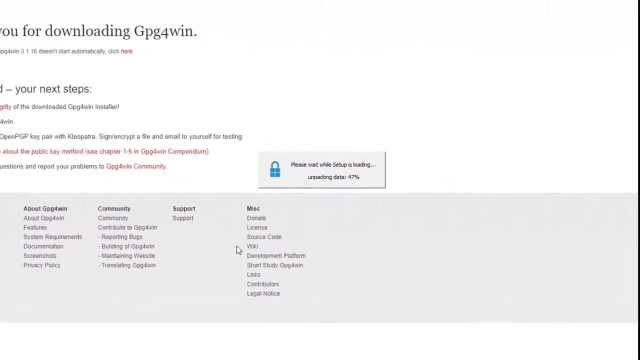 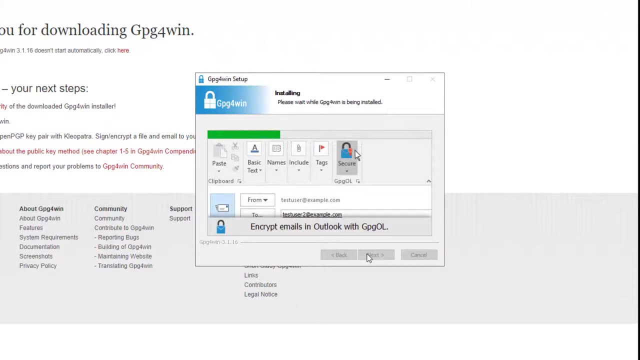 select the zero amount and click the download button. Now you can install the tool quickly. after the download, During the setup process, you can complete the steps without changing the default settings. That is how easy gpg4win tool is to install. 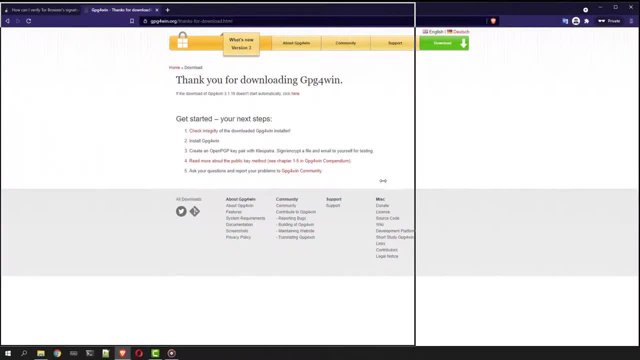 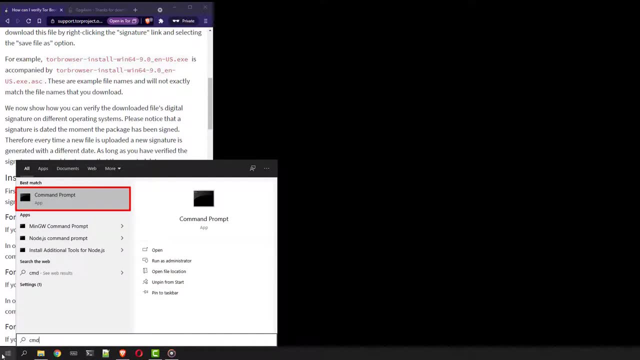 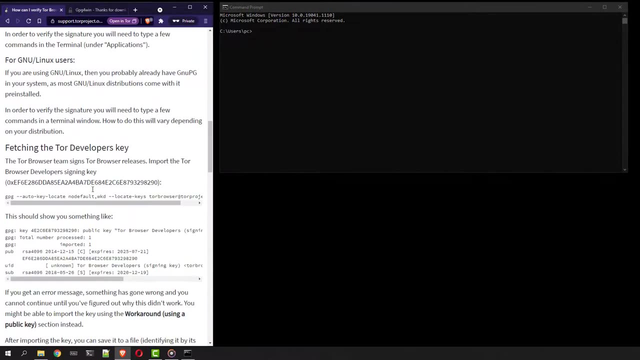 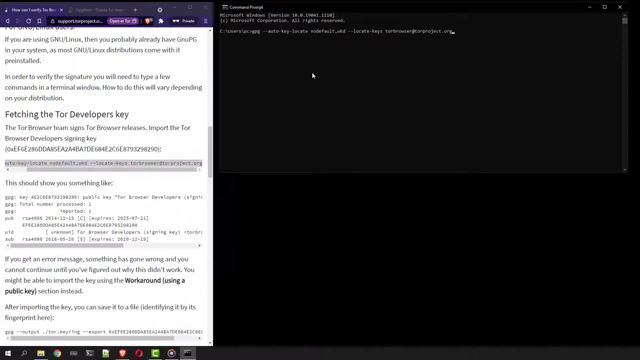 In order to verify the signature, you first need to import the developer key. For this, let's run the cmd tool, which is the command prompt on Windows, And enter the command. When you enter the command correctly, the developer key is imported, as you can see. 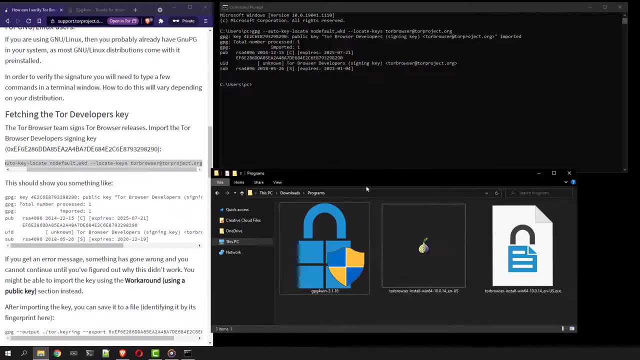 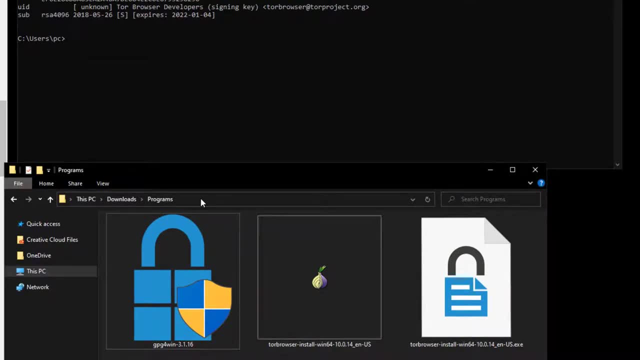 After this process, let's enter command by specifying the location of setup file and signature files downloaded. Since the files I downloaded are in the downloads folder, I enter command in this way. When entering the command, it's important that you first specify the signature file. 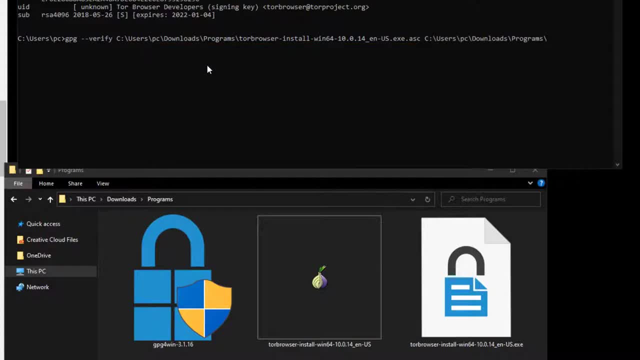 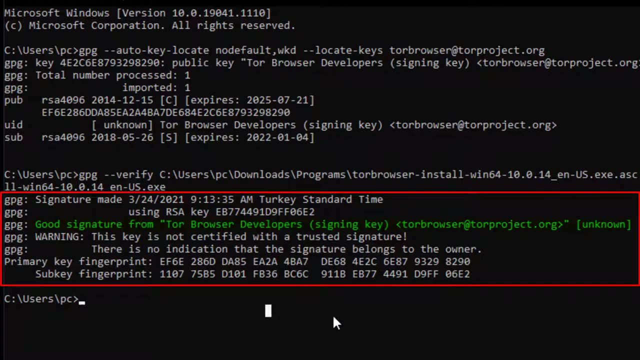 that is, follow the command order And, as a result, the output I got match with the developer key I imported, proving that my file is signed by the Tor developers and has not been modified. If your file was a modified file, you wouldn't be able. 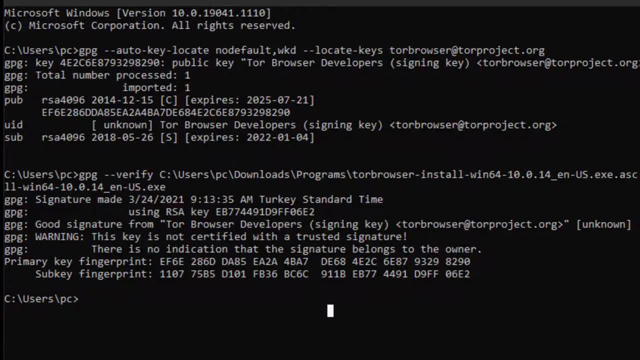 to get this output, as the signature match wouldn't be provided In this case, you need to download the setup file and verification key from an alternative download source again and try this verification process again. Now that we have verified the setup file, we can start the Tor browser. 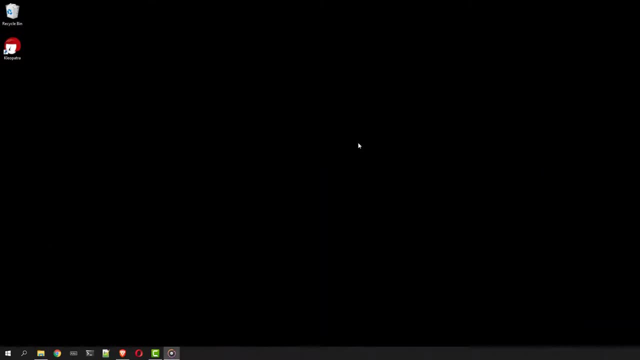 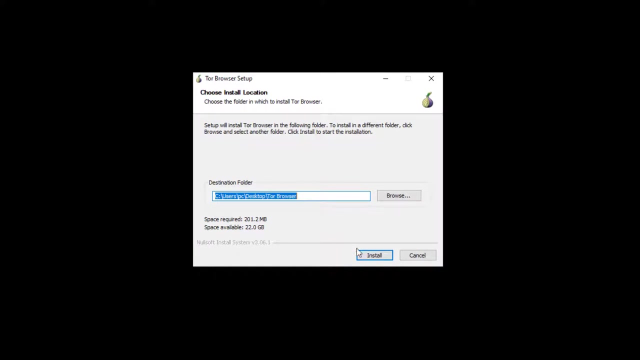 installation. by clicking the setup file, You can select the language to be used during the installation process here. Unlike many programs, when the Tor browser is installed it doesn't spread throughout the system. It maintains all files in a single file location, so you can choose where the location. 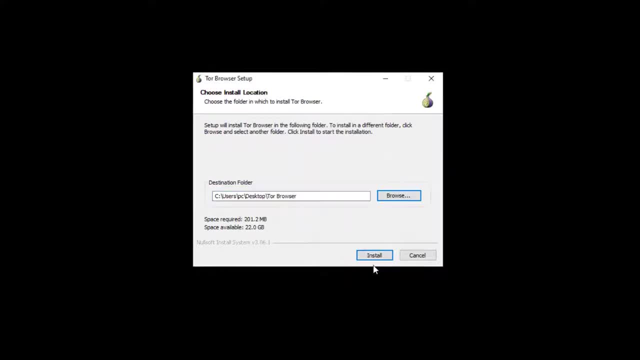 the file from the window that opens. I'm not changing the default file location. If you wish, you can specify a different location. The installation process is completed in a short time. If you want to create a shortcut to start menu and desktop, you can click finish. 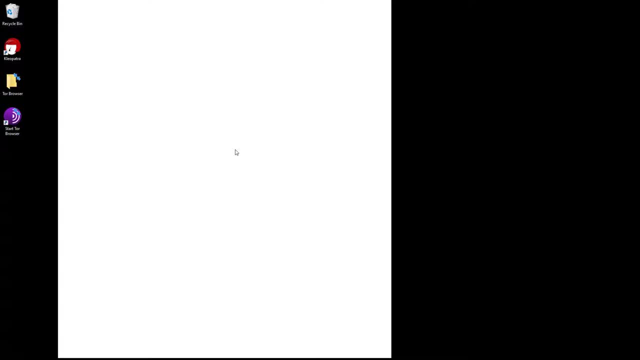 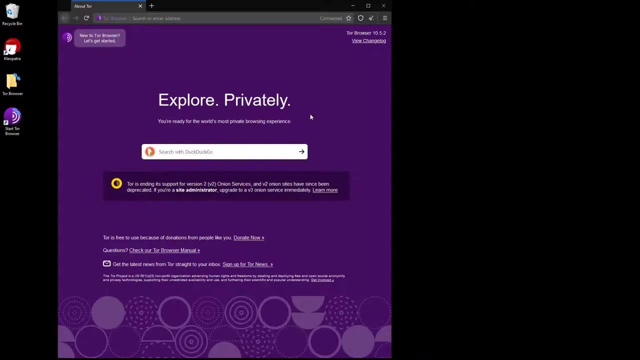 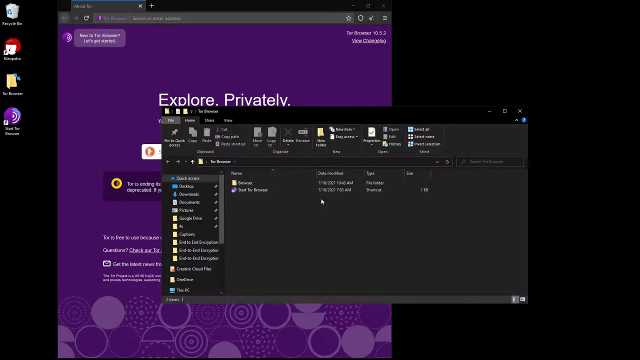 without unchecking. In the window that opens, I click the connect button to connect the Tor browser to Tor network. After a short while the connection is ready and Tor browser is opened without any problems. Also, when you check, you can confirm: 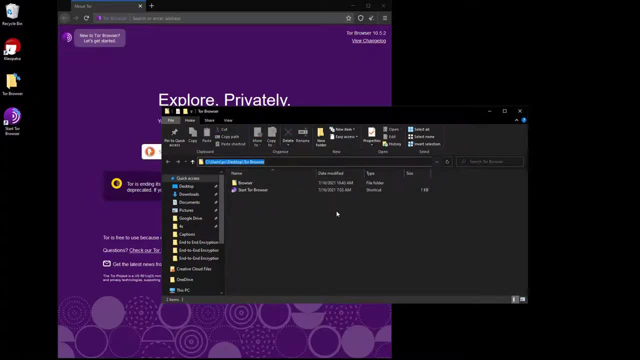 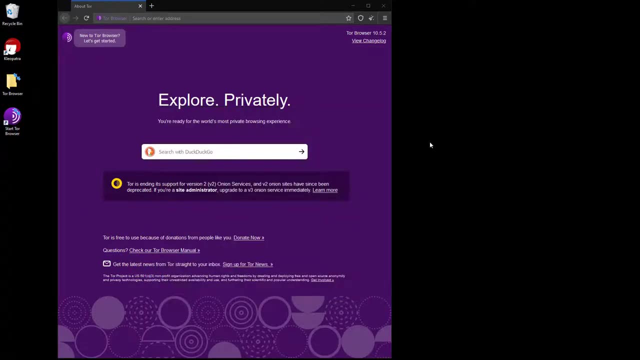 the Tor browser is installed in the folder named Tor browser on the desktop. This is how we safely downloaded and installed the Tor browser. We will discuss its use in detail in the next lectures. Finally, I would like to point out that isn't have to perform. 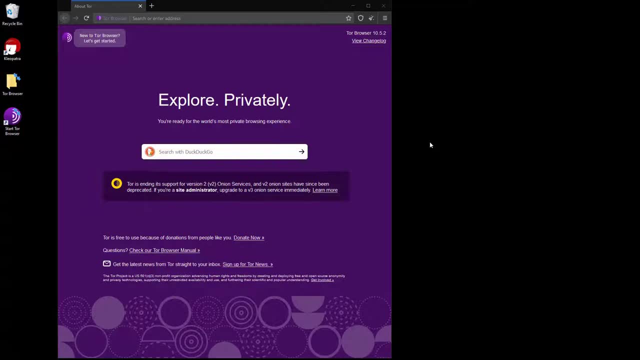 the verification process, but it is an extremely important detail for your security. As there is no difficulty at verification steps, I strongly recommend that you verify before the installation process. In the next lecture, we will perform the same verification and installation process, this time for the Mac. 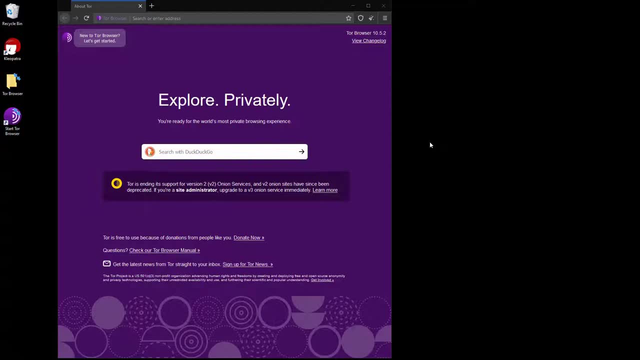 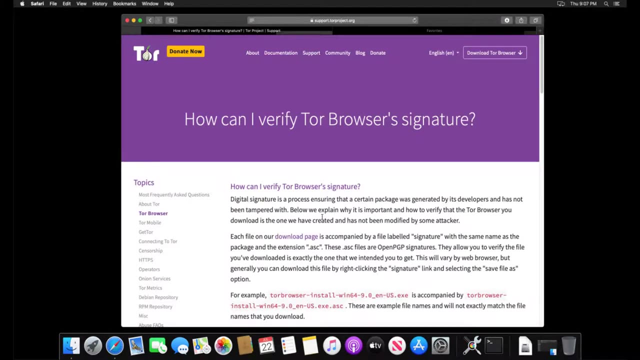 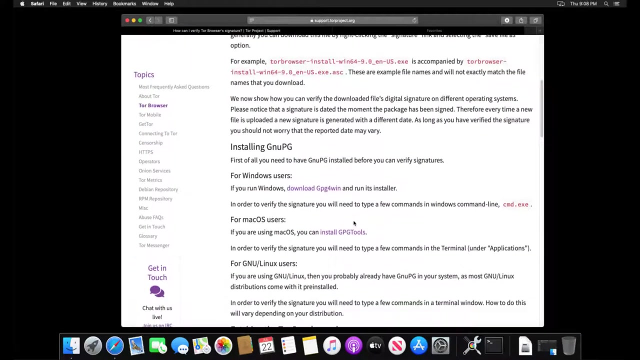 operating system. So if you are not using Mac OS, you can skip the next lecture directly. Before the installation process you should perform signature check to verify the content of setup file you downloaded. You can use the official guide to follow the verification. 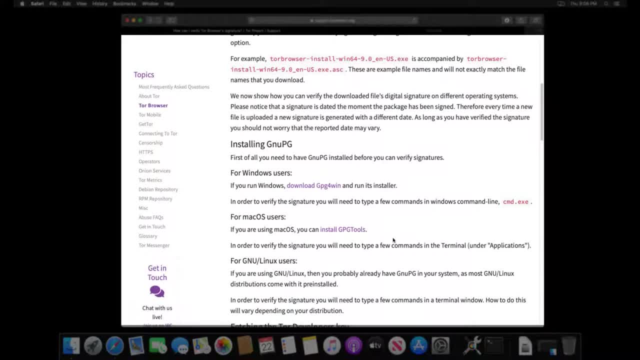 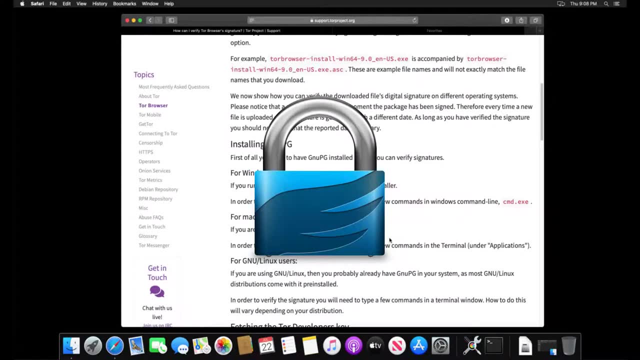 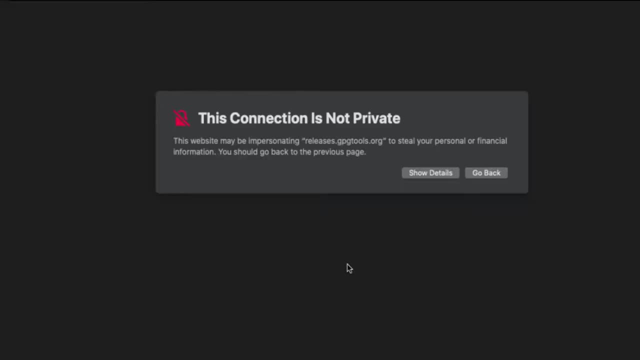 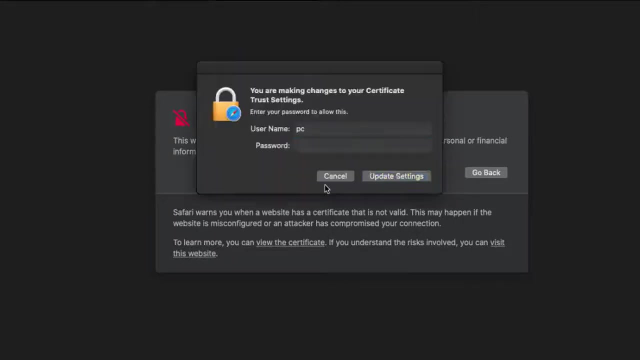 steps easily. I added this verification guide link in this lecture's sources. You will use the GPG Suite tool to verify the setup file before installing. To download tool, go to gpgtoolsorg and click the download button. After the download, you can start. 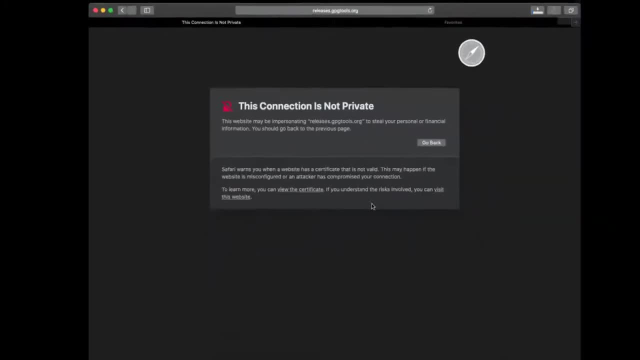 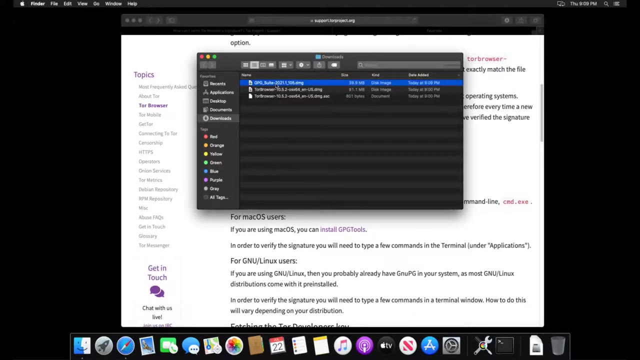 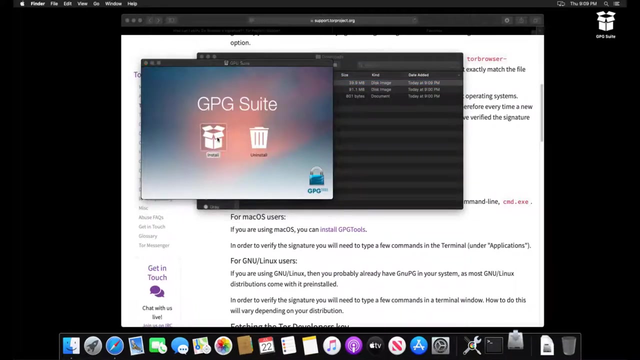 installation by double-clicking the setup file And click install in the window that opens. Let's complete the installation process in a short time by giving all the necessary approvals for installation. The installation process will start in the next lecture. Thank you for watching. 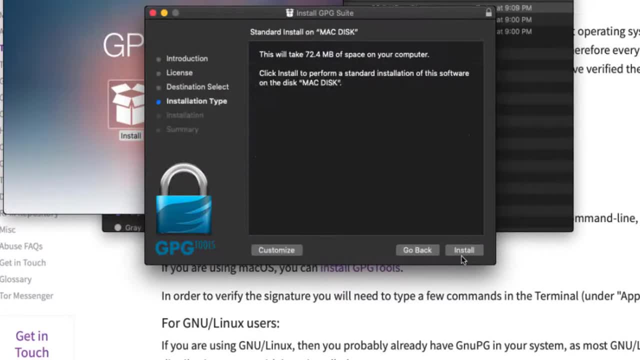 Have a nice day, Bye-bye. Now that you have installed the verification tool, you can verify the signature by opening the terminal. If you don't know how to open terminal, you can access it by searching terminal from application section or the search bar. 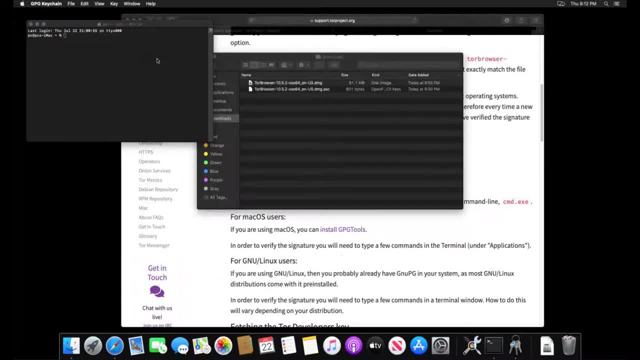 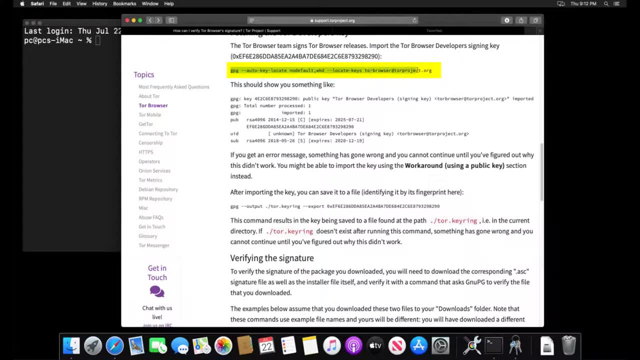 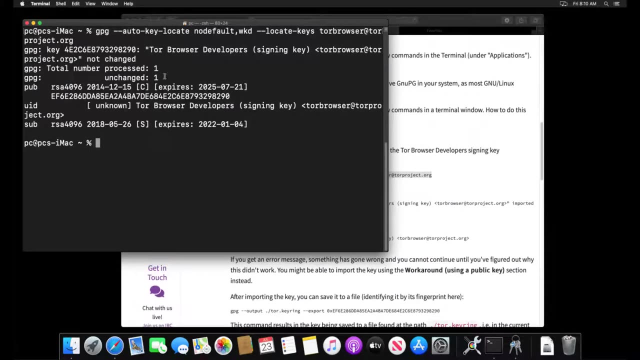 In order to verify the signature, you first need to import the developer key. Enter the command to import the developer key. When you enter the command correctly, the developer key is imported, as you can see. After importing the key successfully, let's enter command. 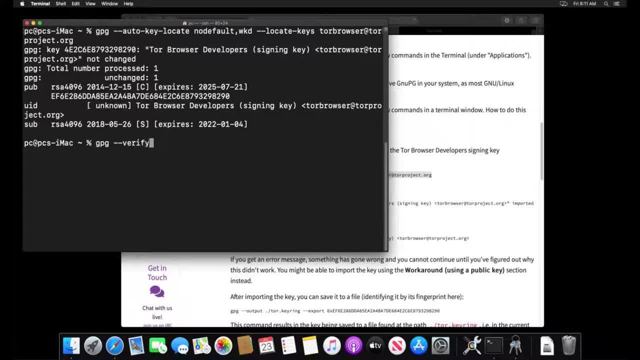 by specifying the location of the setup file and signature as downloaded. Since the files I download are in the downloads folder, I enter command in this way. When entering the command, it's important that you first specify the signature file that is follow the command. 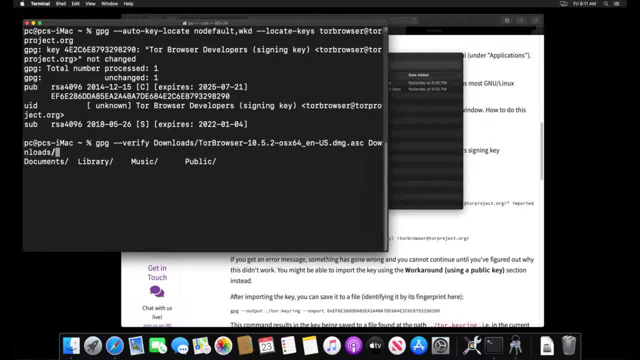 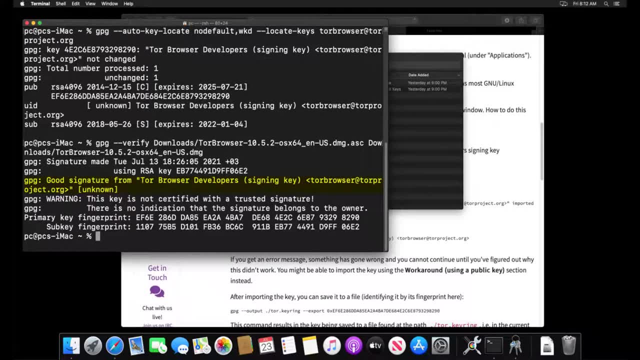 order. When you click the tab key while typing the file names, the name will be completed automatically And, as a result, the output I got matched with developer key I imported, proving that my file is signed by the Tor developers and has not been changed. 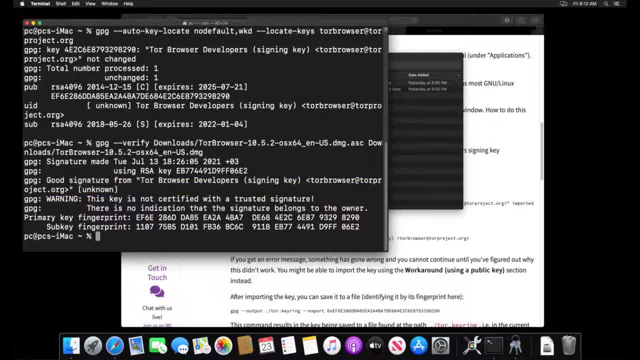 or modified. If your file was a modified file, you wouldn't be able to get this output, as this signature match wouldn't be provided. In this case, you need to download the setup file and verification key from an alternative download source again and try this verification process again. 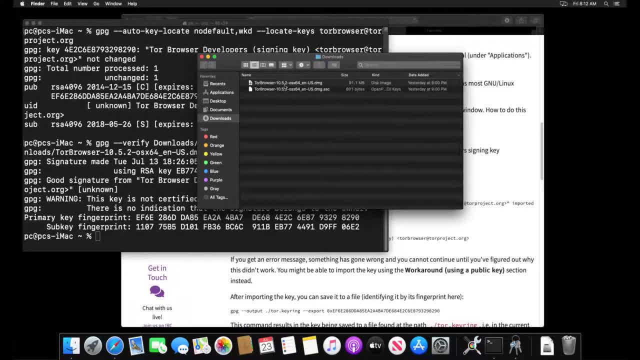 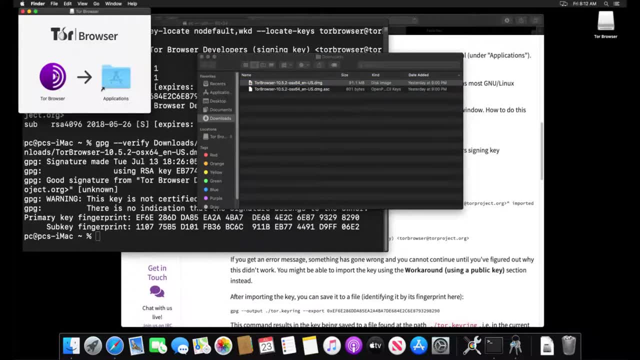 Now that you have verified your file, you can start the Tor browser installation by double-clicking the setup file. You can drag and drop the application icon onto the application icon to install the Tor browser on your computer. You can run it smoothly by clicking. 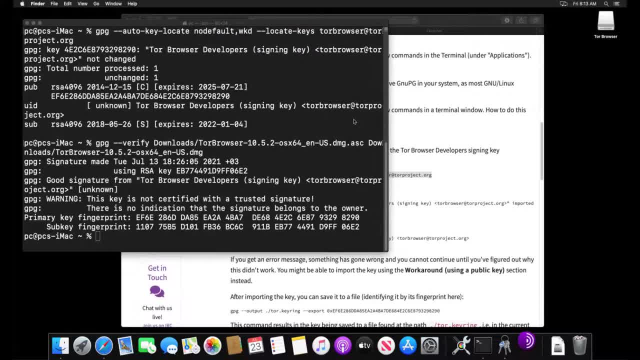 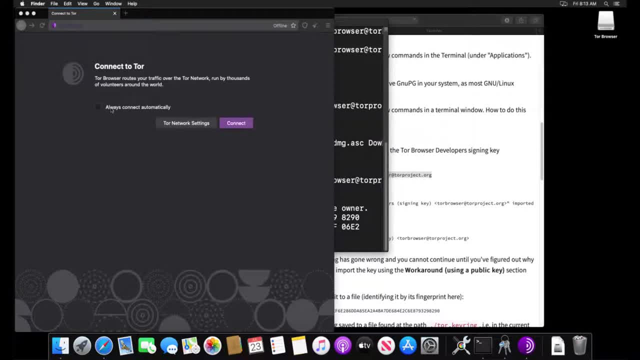 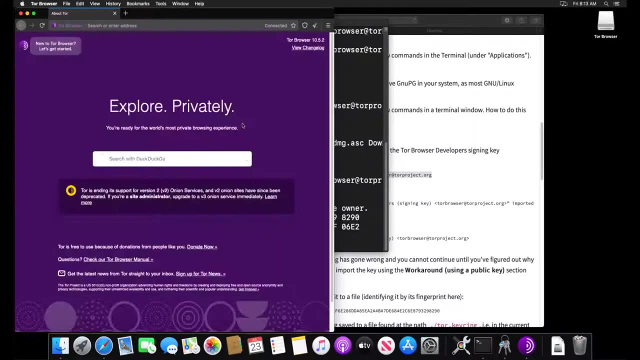 the Tor browser icon from the application section. In the window that open, you should click the connect button to connect the Tor browser to the Tor network. After a short while, the connection is ready and Tor browser is opened without any problems. Thus you have installed the Tor browser. 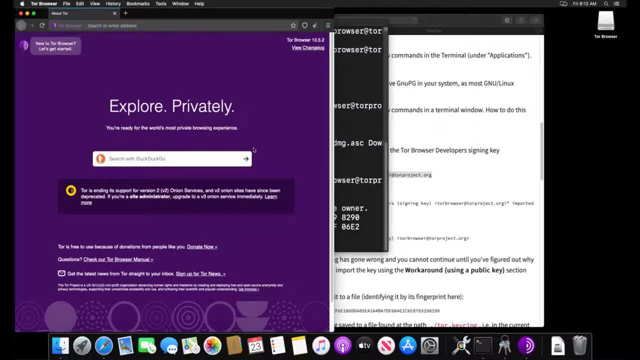 very easily. We'll be talking about its use in detail in the following lectures. Finally, I would like to point out that it does not have to perform the verification process, but it is an extremely important detail for your security, As there is no difficulty at verification. 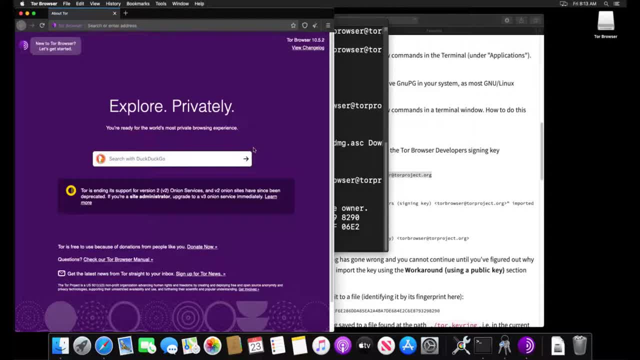 steps. I strongly recommend that you verify before the installation process. In the next lecture we will perform the same verification and installation process, this time for the Linux operating system. If you are not using the Linux, you can skip the next lecture directly. 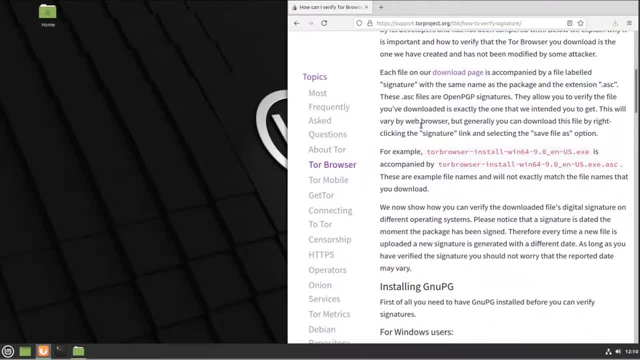 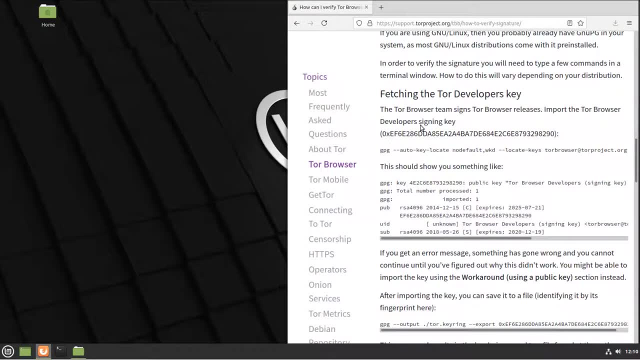 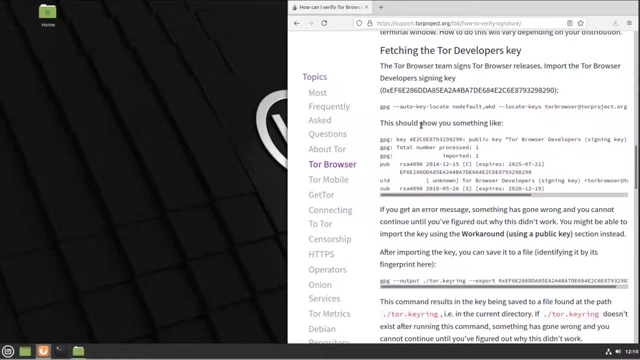 Before the installation process you should perform signature check to verify the content of the setup file you downloaded. You can use the official guide to follow the verification steps easily. I added this verification guide link in these lecture sources. You don't need to install an external tool for 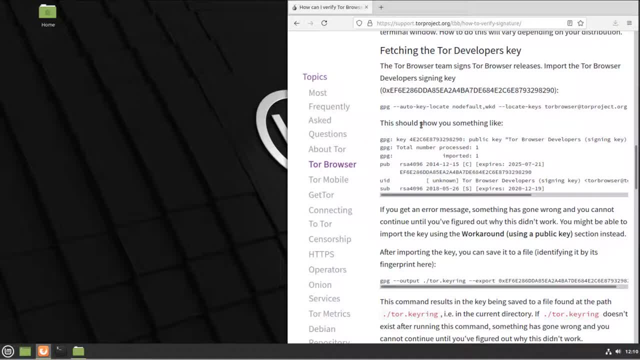 file verification as it is in other operating systems. Most Linux distributions usually come with a GPG tool. If there is no verification tool in the Linux system you are using, you can reach me from the question and answer section In order to verify the signature. 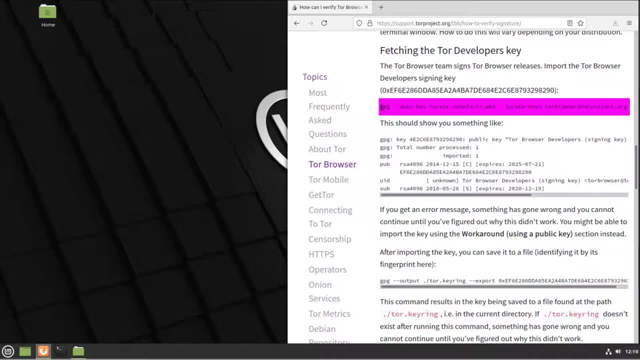 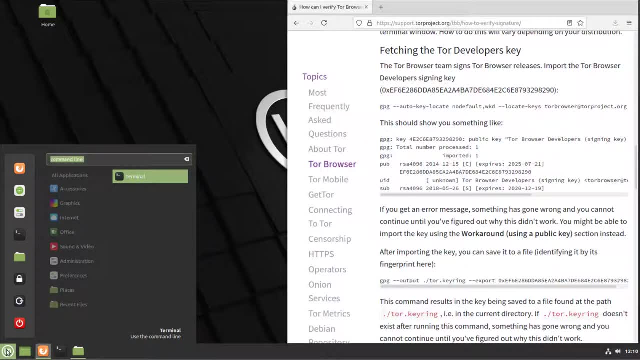 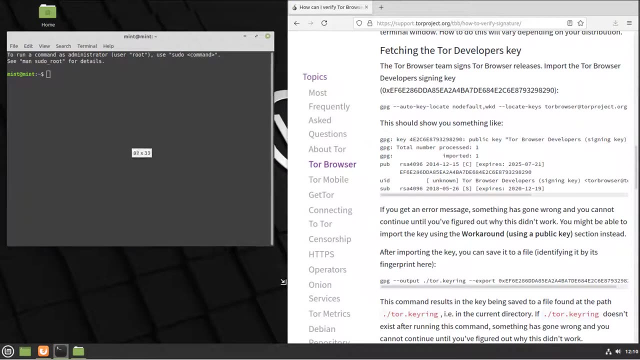 you first need to import the developer key. If you are using Linux but have never opened the command line before, you can open it by searching for command line or terminal or finding it from the list of application. After opening your terminal, let's enter command to. 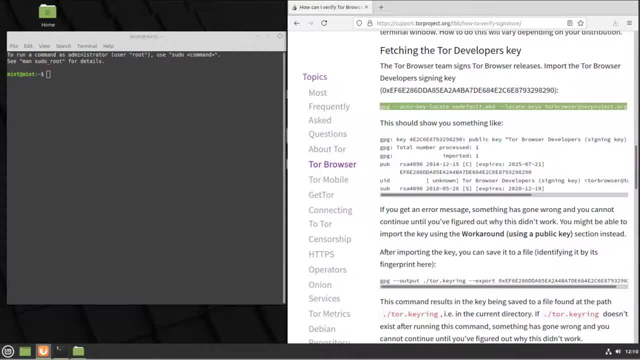 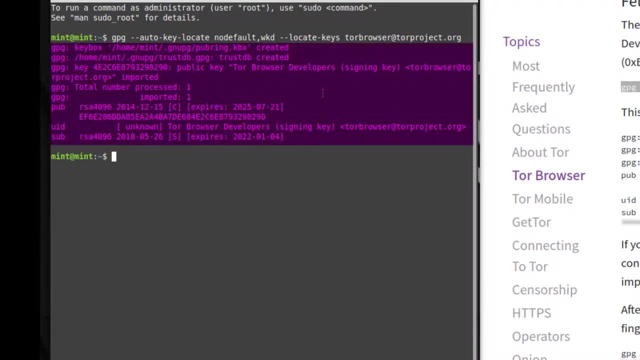 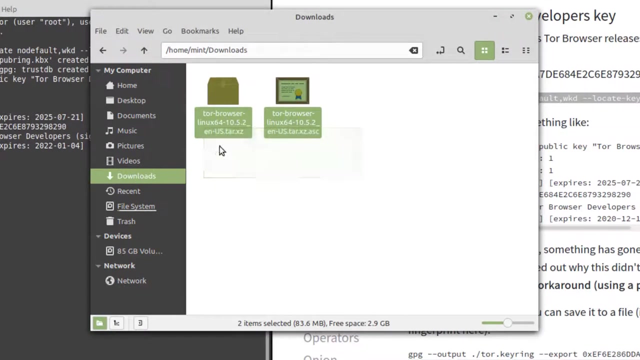 get developer key. When you enter the command correctly, the developer key is imported, as you can see. After importing the key successfully, let's enter command by specifying the locations of the setup and signature files downloaded. Since the files I download are in the download folder, I enter. 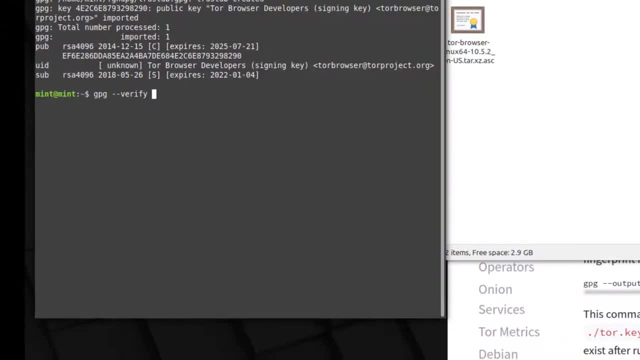 command in this way. When entering the command, it's important that you first specify the signature files. that is, follow the command order. When you click the tab key while typing the file names, the name will be completed automatically And, as a result, 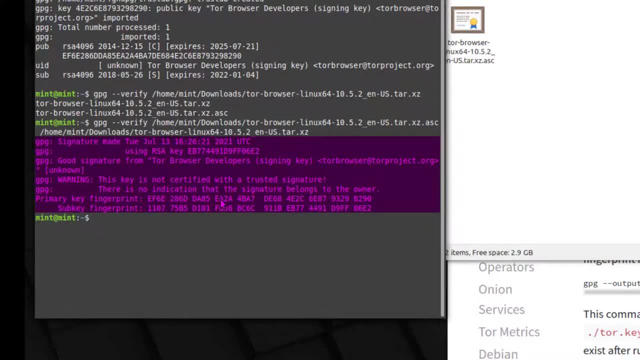 the output I got matched with developer key I imported proving that my file is signed by the Tor developers and has not been modified. If your file was a modified, you wouldn't be able to get this output, as the signature match wouldn't be provided. 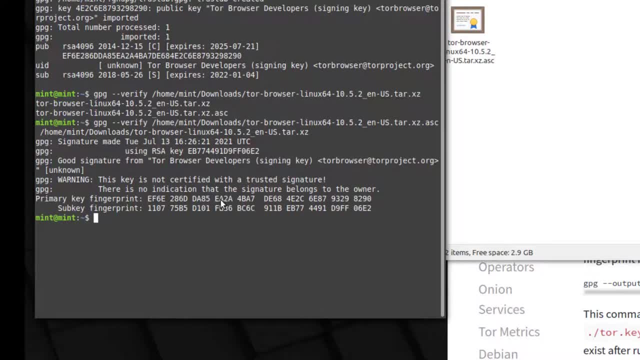 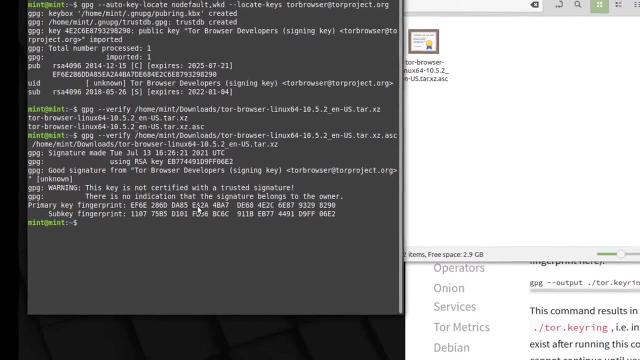 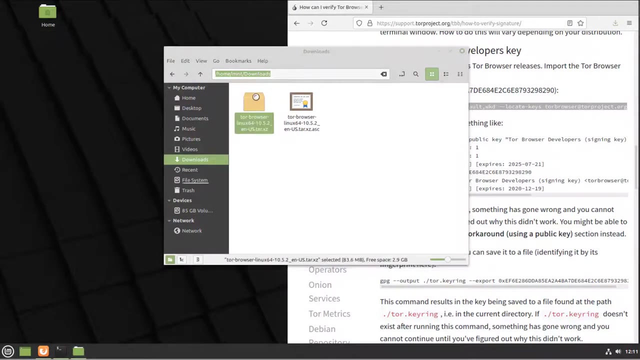 In this case, you need to download the setup file and verification key from alternative download source again and try this verification process again. Now that you have verified setup file, you can start using Tor browser by extracting it from the archive file to a location you want When. 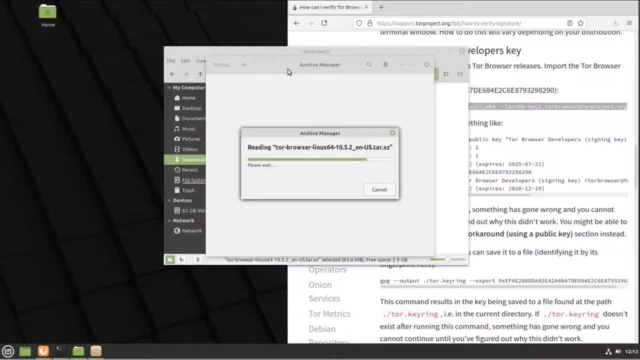 you using Tor browser. on Linux it comes pre-installed without the need for installation. All you have to do is decide where you want to locate this file. I extract the contents of the archive to my desktop location. To run my browser, I go to the file location. 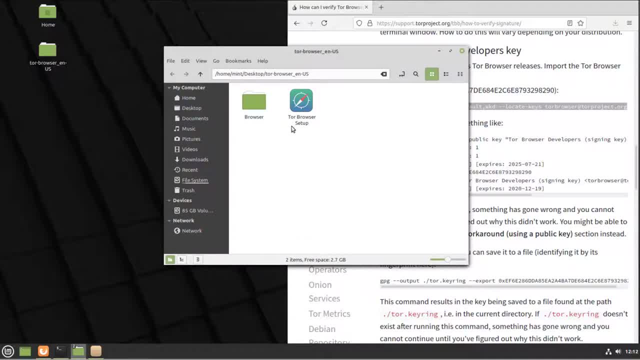 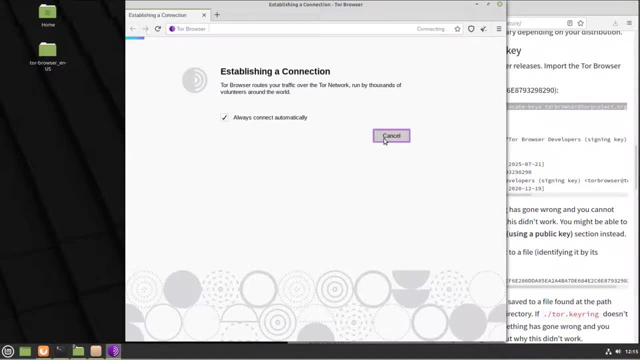 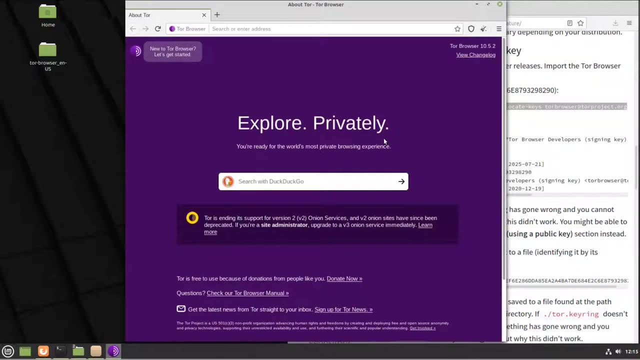 I extracted and double click on its icon. In the window that's open, I click the connect button to connect the browser to the Tor network. After a short while, the connect is ready and Tor browser is opened without any problems. though we have safely. 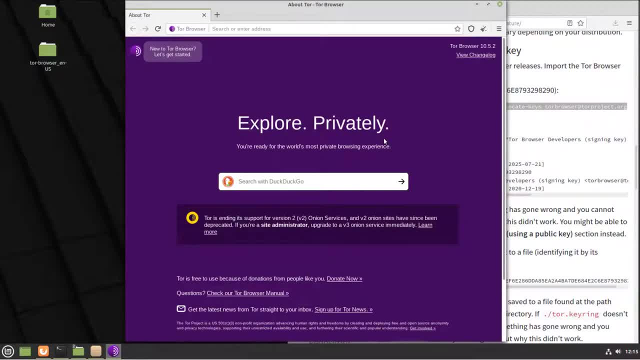 downloaded and installed Tor browser on the Linux system. We will be talk about its use in detail in the following lectures. Finally, I would like to point out that is not have to perform the verification process, but it is an extremely important detail for your security. 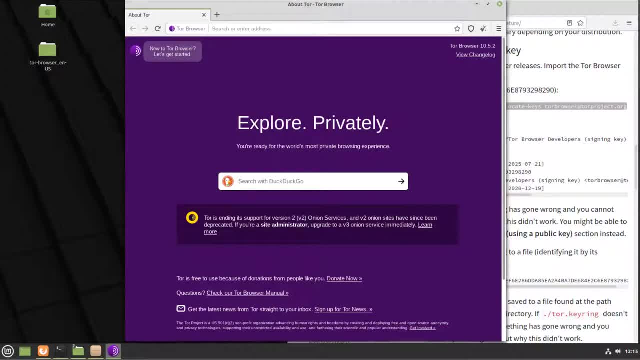 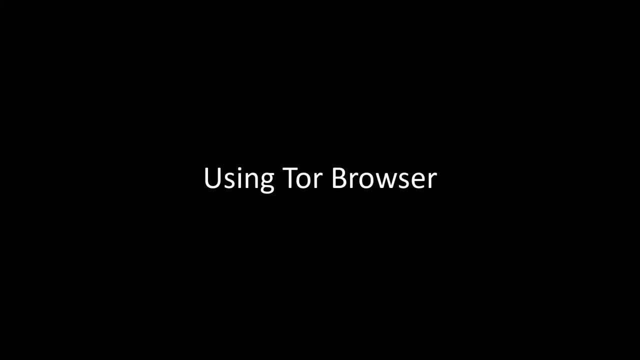 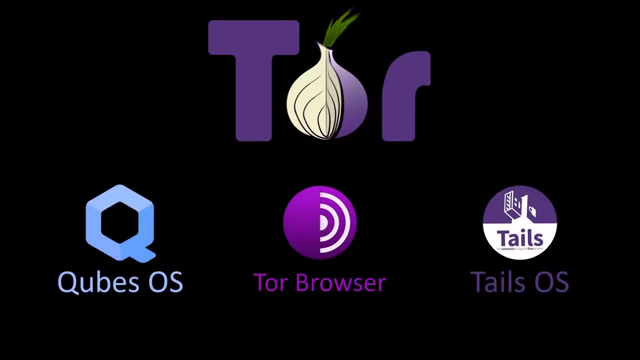 As there is no difficulty at the verification steps, I strongly recommend that you verify before the installation process Using the Tor Browser. When I talk about the structure of the Tor network, I have listed the methods you can use the Tor. If you remember, I mentioned 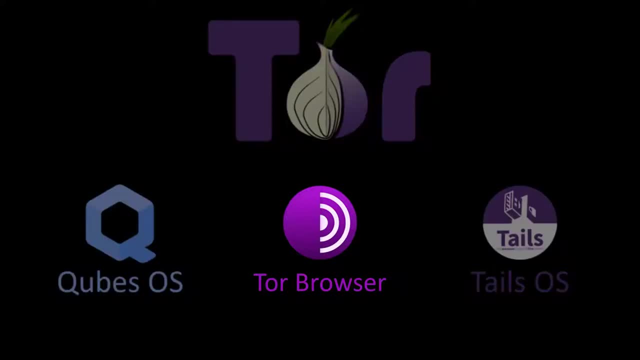 that using the Tor browser is not the best way among these methods. The reason why using the Tor browser is not the best method is because the operating system we use the browser is not strictly security oriented. So, in fact, we will be using the Tor browser in other methods. 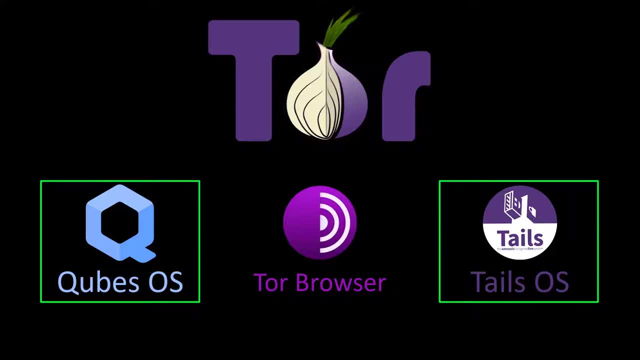 that we consider safer in the continuation of the course, Since operating system that we will use the Tor browser for in the methods we consider safe, are fully configured for privacy, they will provide a much more secure environment than any other operating system. So actually using the Tor browser. 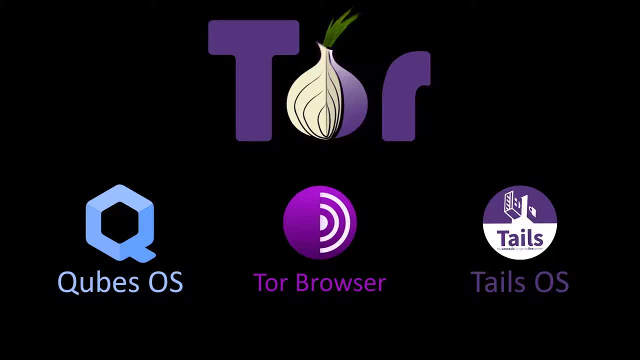 on Android, Windows, macOS or a standard Linux distribution is not a completely inefficient way, But it is not the best way for security and privacy. The vulnerabilities that may occur in operating system or software on the operating system may cause the anonymity and privacy features provided. 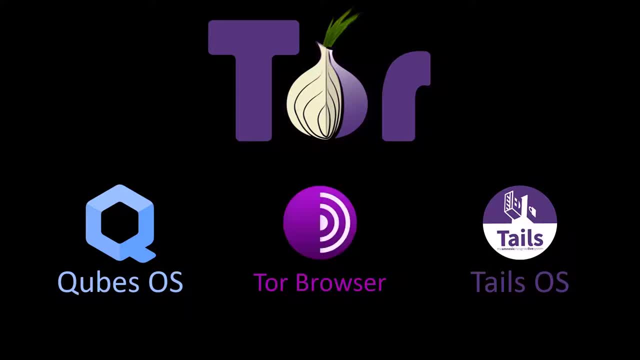 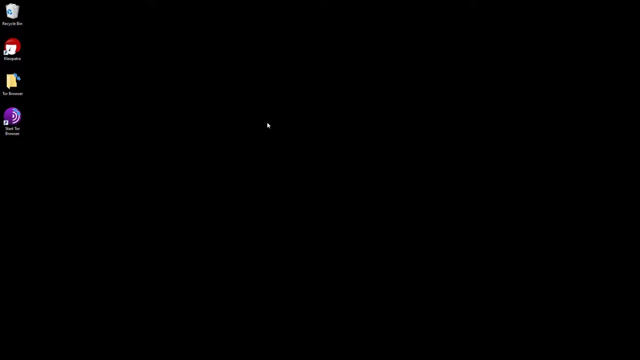 by the Tor browser to become meaningless. In short, using the Tor browser on standard operating system is practical, but alone is insufficient for security. Without further ado, let's continue to explanation by talking about the use of the Tor browser and its various settings. Although the 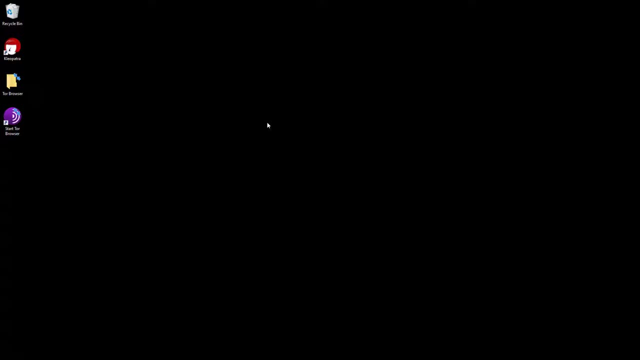 installation and verification process differs slightly for different operating system. the use of the Tor browser after it is installed is very similar for all system. In other words, all system user can easily follow the instruction here. I will perform the lectures on Windows operating system for now. 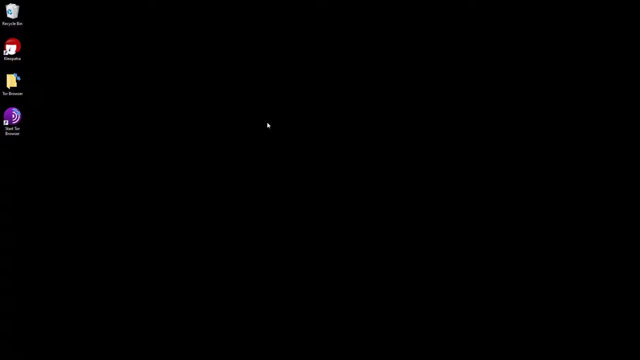 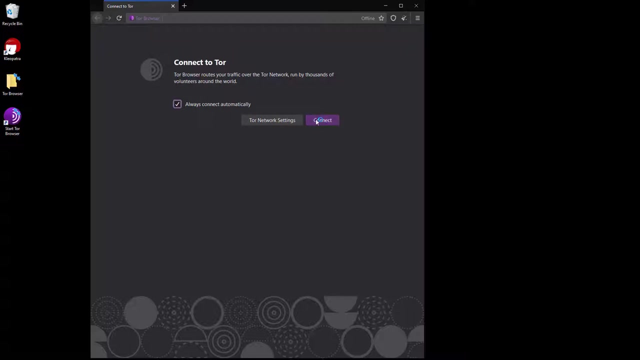 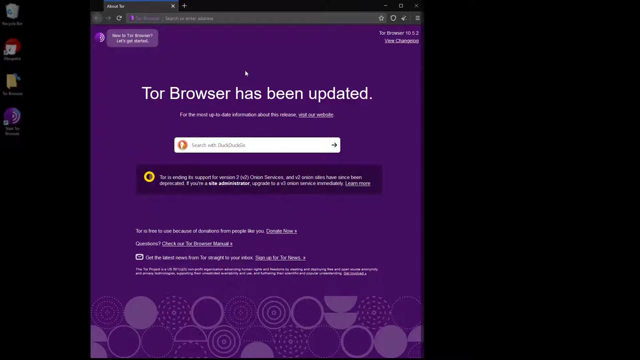 You can follow it on any operating system you want. I double click on the application to open the Tor browser. As you can see, a simple browser interface doesn't look much different from the standard Firefox browser. welcomed us. Now let's check our connection. by going to checktorprojectorg to test whether we are properly connected to Tor network. On the page that opens, we can confirm that our connection is routed through the Tor network, as it should At this point, if you haven't encountered this. 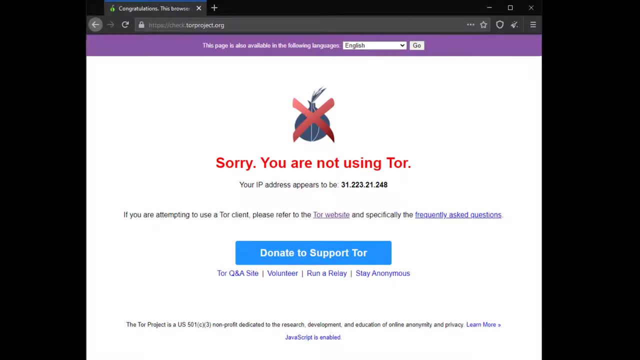 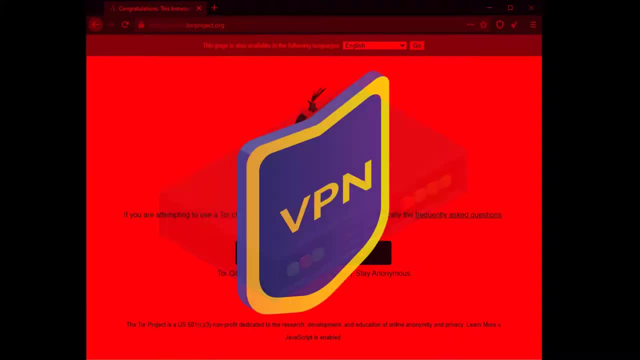 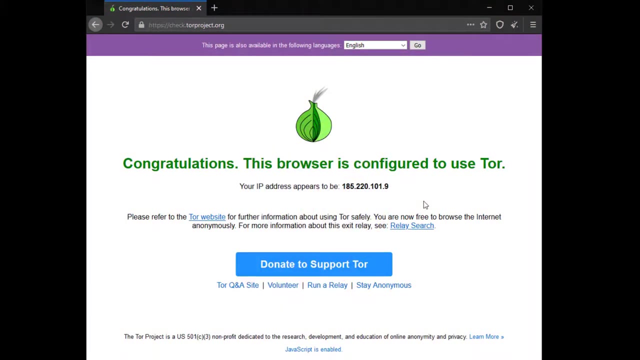 confirmation statement. you may have an internet connection where the Tor network is blocked. In such cases, you can choose to use the Tor bridge connection or VPN to bypass the block. We will talk about VPN usage in the following lectures. For now, let's continue. 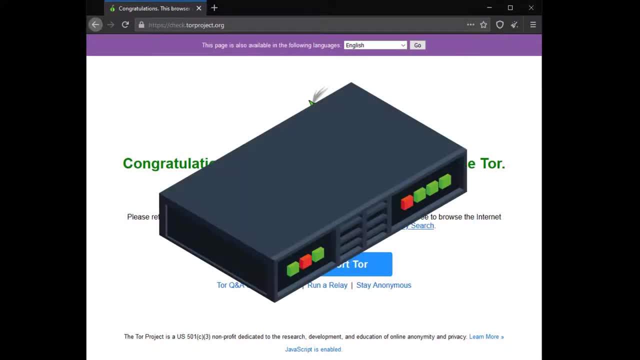 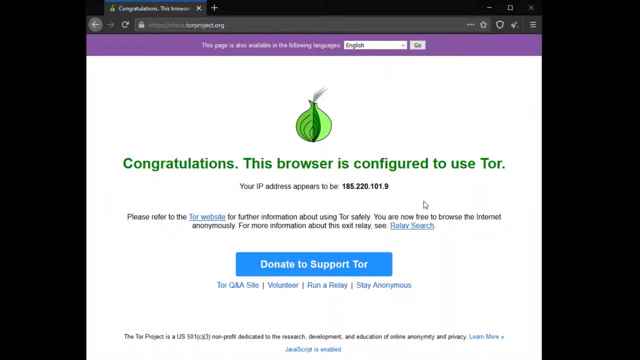 with explanation by talking about the Tor bridge connections. In addition, even if you can access the Tor network smoothly, while you follow this lecture, it will be useful to learn how to use bridge connection in case you encounter a potential block. So even if your Tor connection is fine, 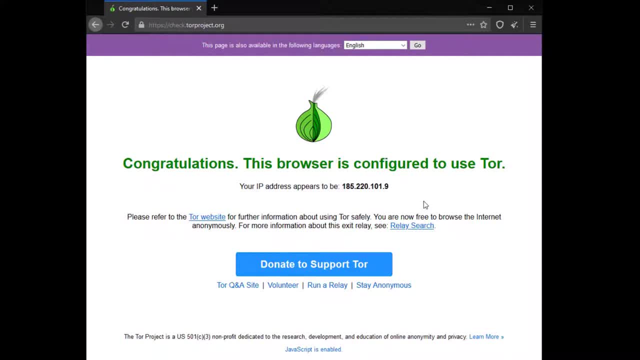 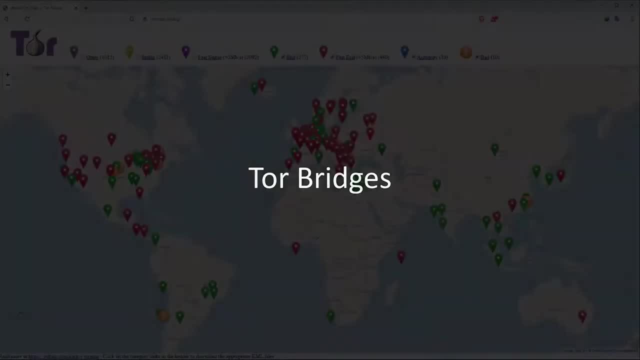 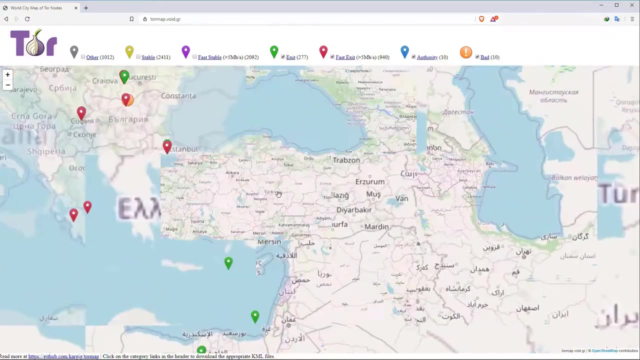 please continue course without leaving the curriculum layout, When I talk about the working structure of the Tor network. at the beginning of the course I mentioned that the list of the server in the Tor network is publicly published and therefore the Tor servers can be easily blocked. 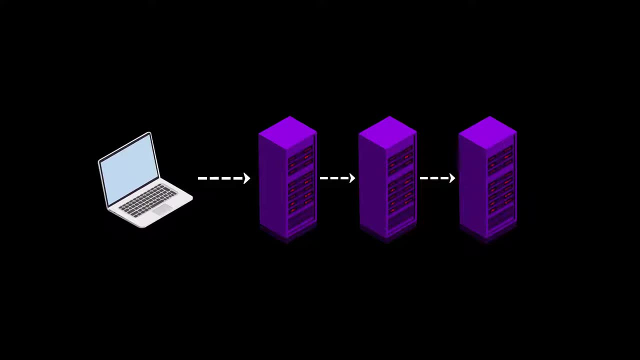 Authorities such as a government, your service provider or your network administrator can easily block the Tor network through this publicly published list of servers. It's possible that you will often encounter situations where the Tor network is blocked, because it is easy to block In such 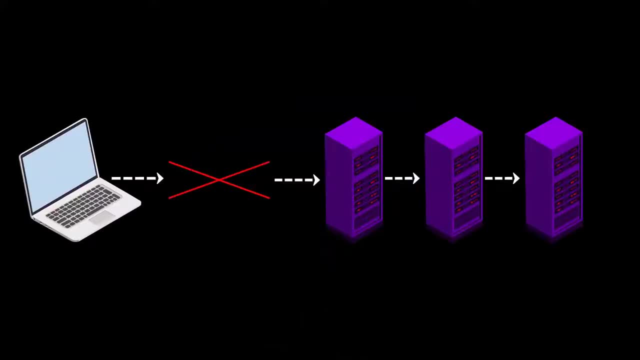 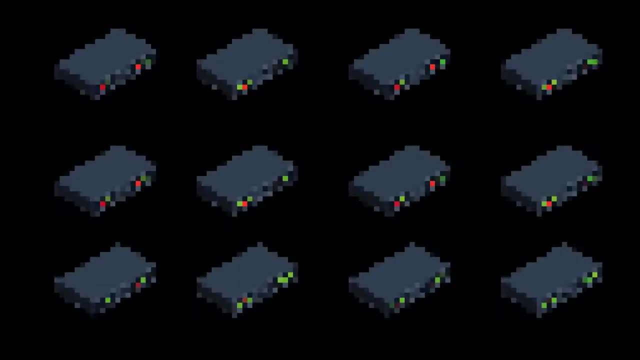 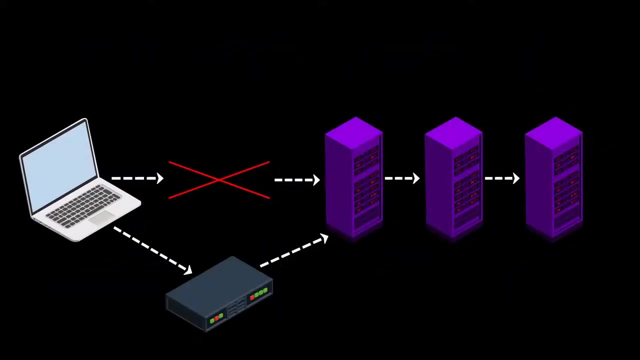 cases, you can use the bridge connections provided by Tor project to overcome the obstacle. Since the list of bridge routers is keep confidential. all bridge connections cannot be blocked at once, So even if the servers are blocked, access to the Tor network can be achieved. 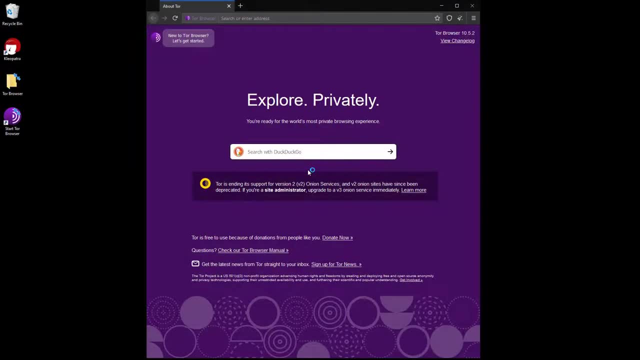 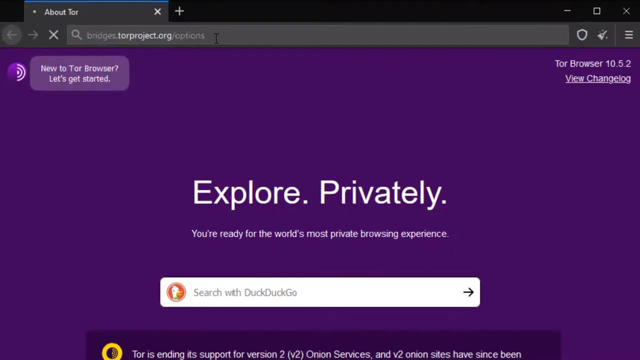 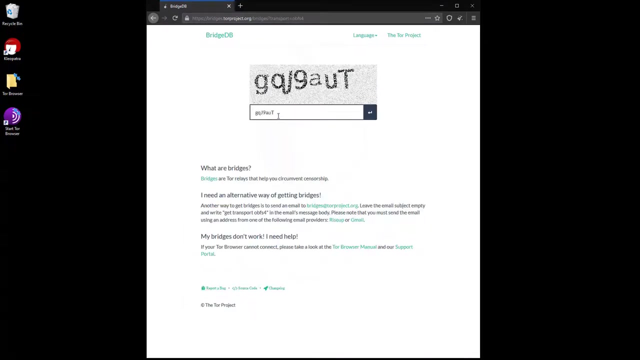 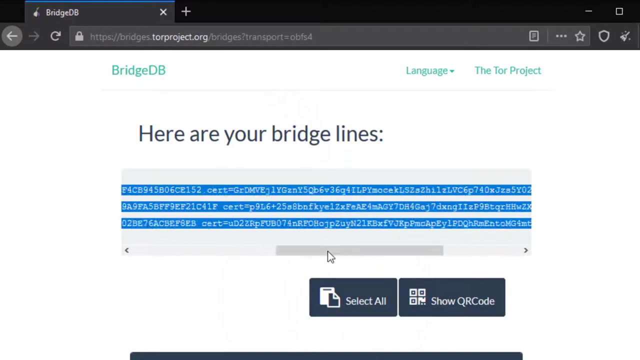 over the bridge connections. So establish the bridge connection. you need to visit the bridgetorprojectorg slash options. After entering the security code you can see address information required for bridge connections. You can copy these addresses from here If Tor is. 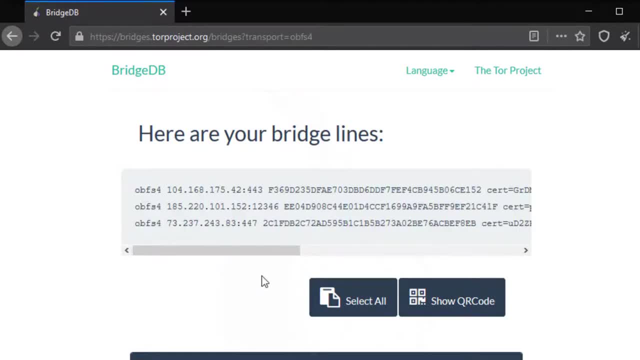 blocked on the internet you are connected to, this website is probably also blocked. If you haven't been able to obtain bridge addresses in this way, you can access these websites using any VPN service. You can also get these addresses from within the Tor browser, as. 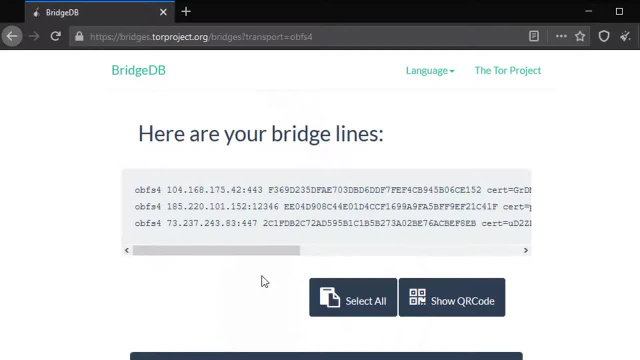 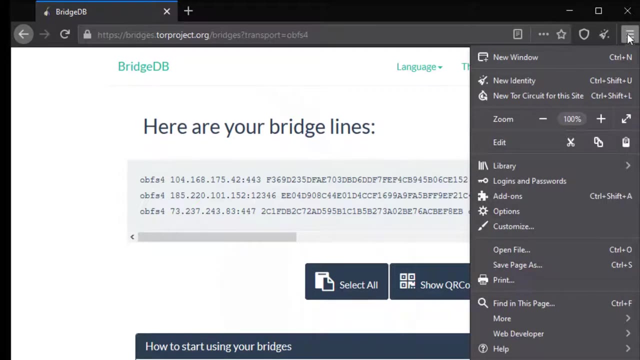 an alternative to VPN option. When we talk about the Tor browser settings, you will see how you can get bridge addresses from within the Tor browser. Now let's click the three line icon on the right side of the browser to open the menu. to make the necessary. 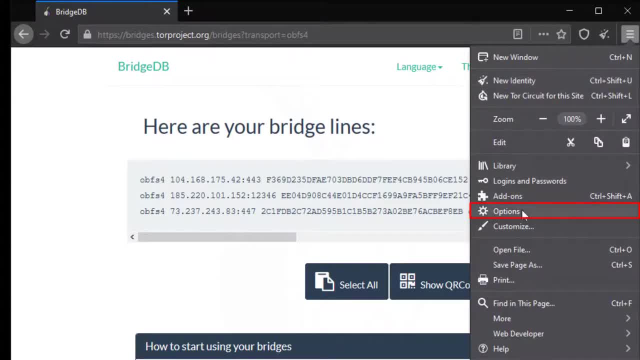 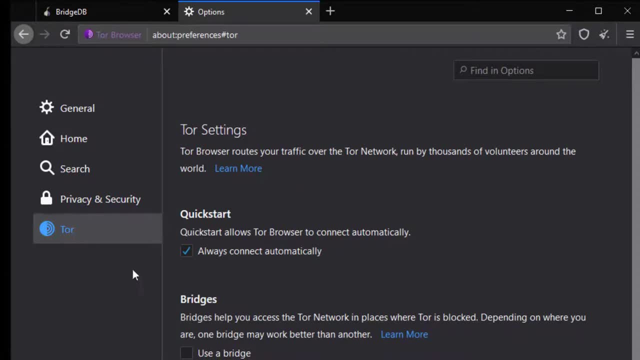 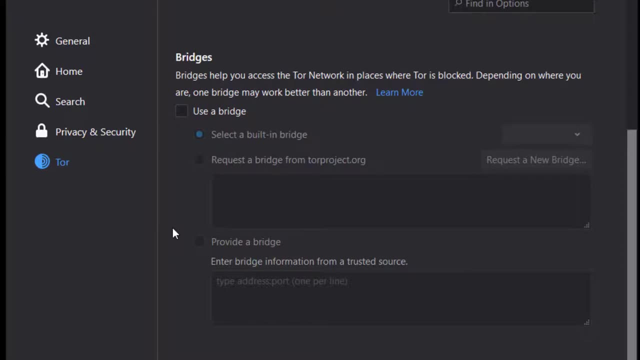 settings for the bridge. Click on options from the menu that's open. After the options window opens, click on the Tor tab on the left. Here we will make the necessary settings for the bridge connections. To configure the bridge first, let's check in the use bridge. 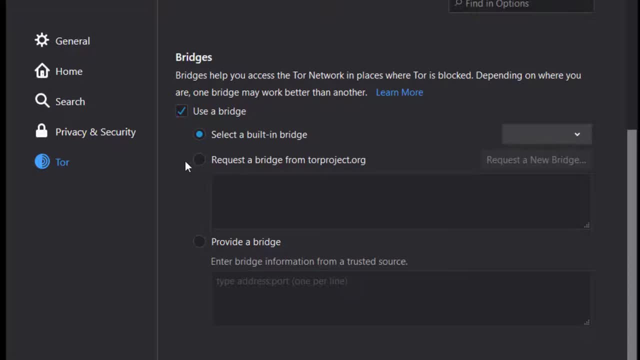 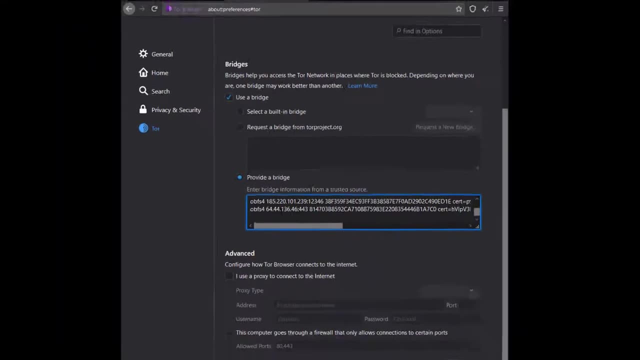 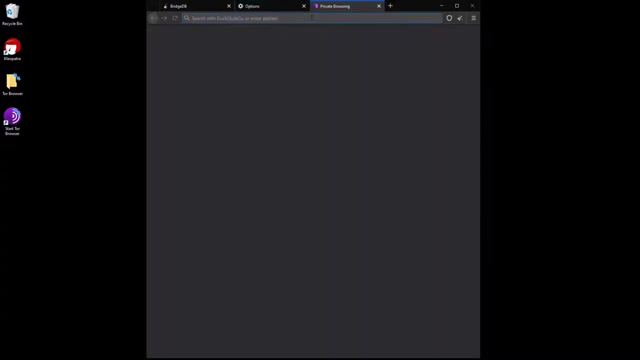 box. If you have bridge addresses, you can click on the provide a bridge option and enter the bridge address in this field, Those. the Tor network will be provided over the bridge connection you have specified. To test whether a bridge connection is available, let's go to. 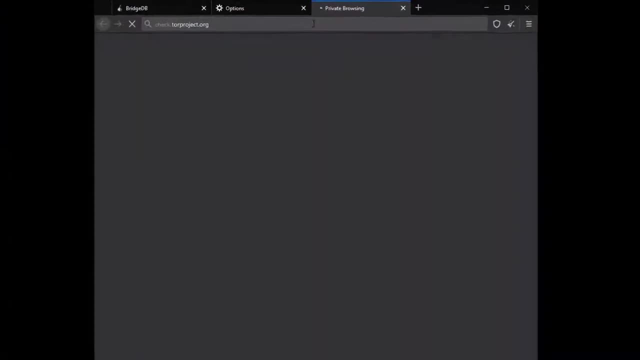 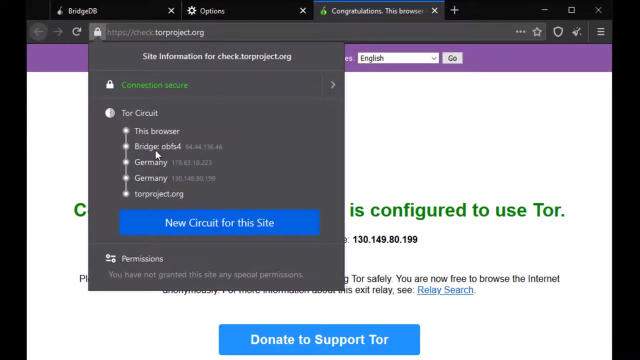 checktorprojectorg again and check the nodes used to connect to this address. As you can see, the first node is the bridge. This means that you were able to successfully establish the bridge connection. In addition, if you don't have addresses for the bridge, 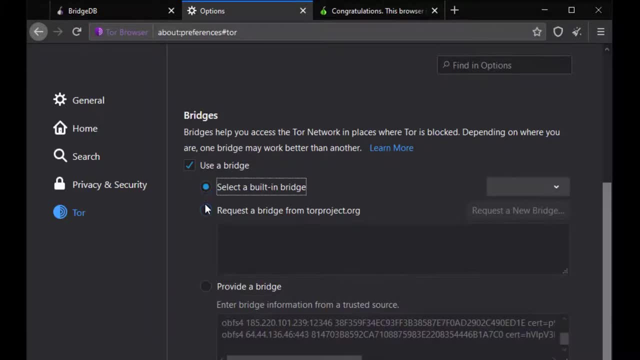 connection. you can also use the select a built-in bridge or request a bridge from torprojectorg options from the bridge section. If you use the select a built-in bridge option, select the OBFS4 option. here a built-in bridge will be used In addition. 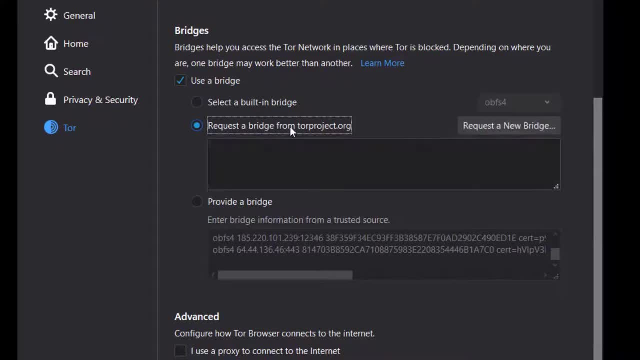 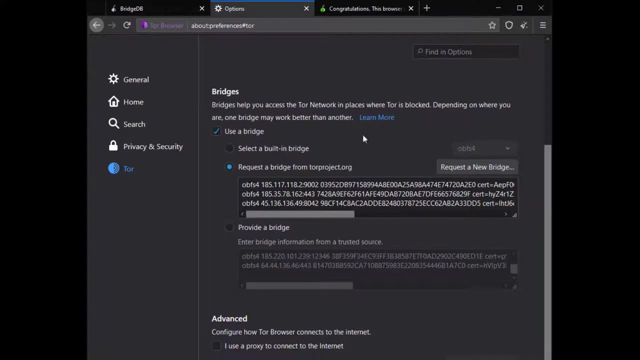 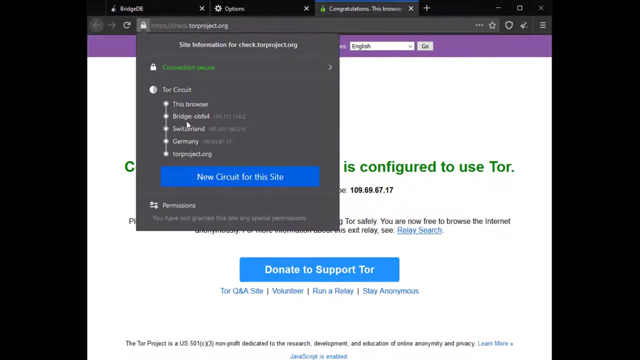 the bridge addresses can be defined automatically with the request a new bridge option. You can easily overcome situations where the Tor network is censored by using all these methods. If you are using the bridge connection and still have problems with the access, you are probably 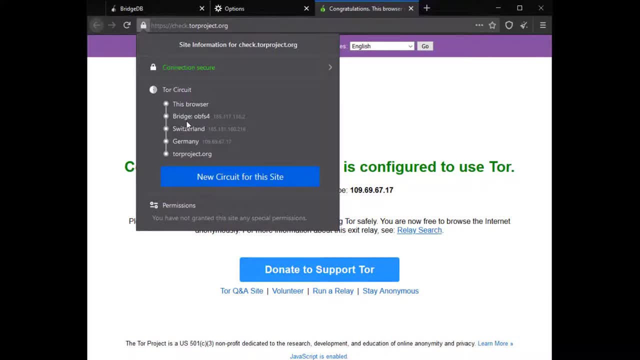 dealing with a censorship mechanism that detects that you have accessed the Tor network by truly analyzing your network traffic. As a simple solution to this situation, you may prefer to use the Tor network over VPN. Moreover, using VPN will may provide you with much more security measures. 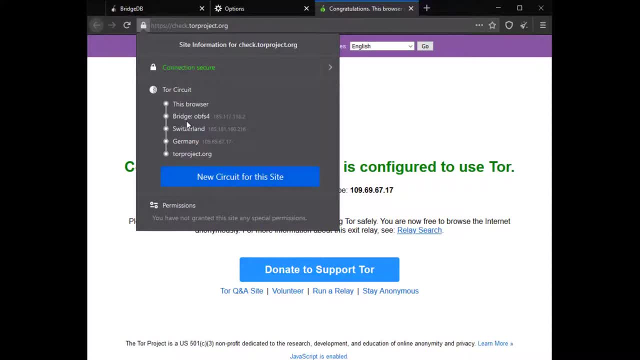 as well as bypassing the censorship. If you don't have access block to the Tor network, using a bridge connection won't make sense because won't provide you with extra security. Please note that the purpose of the bridge is only to bypass censorship, not to 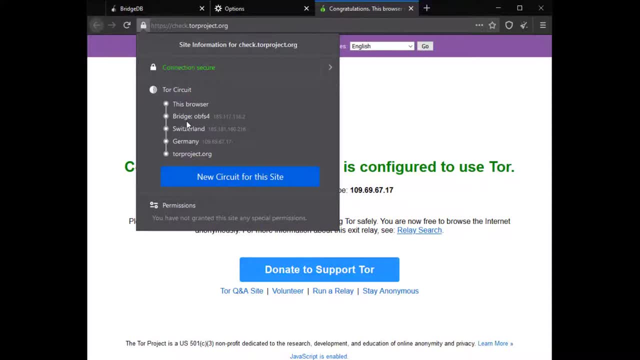 provide extra security. However, in some cases you may want to use a VPN even if you don't have access block to the Tor network. To better understand why, let's explain the effects of the VPN usage on the Tor network by handling Tor connection over VPN. 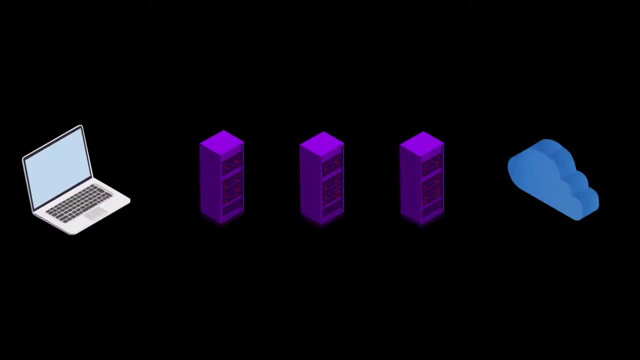 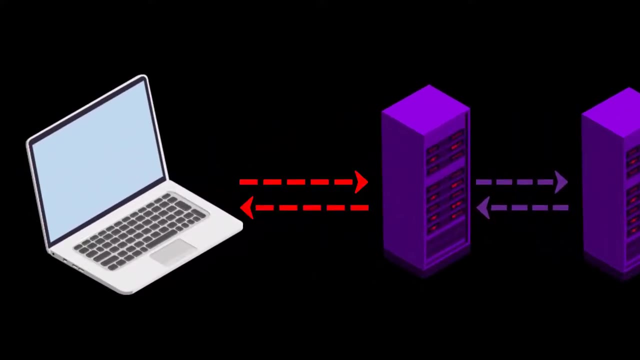 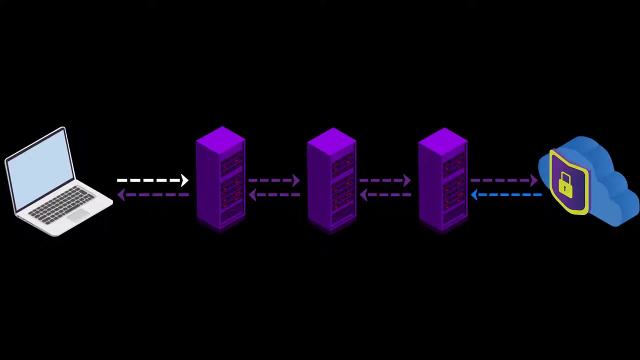 Tor over VPN. When you want to access the internet through Tor network, the traffic between you and entry node assigned to you can be monitored by malicious observers If the website you are visiting to doesn't have SSL or TLS encryption layer, in other words, the encrypted connection. 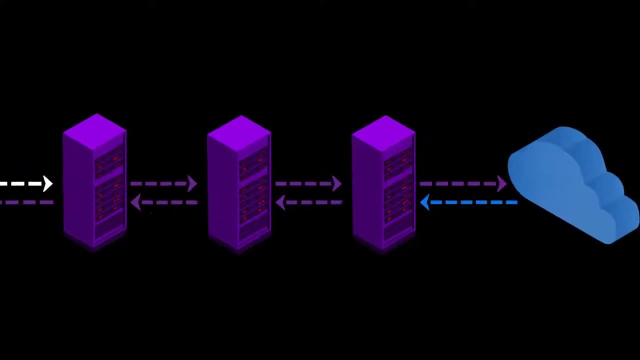 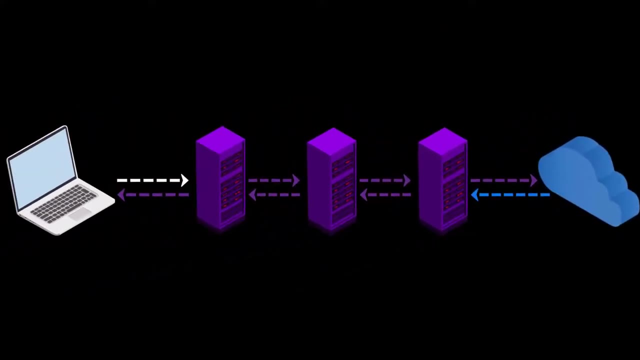 that appears as HTTPS. the traffic between the website and you won't be encrypted, so it can be monitored by observers. If the website you communicate with has a valid SSL or TLS certificate, the observer can't know about the content, even if they monitor the connection. 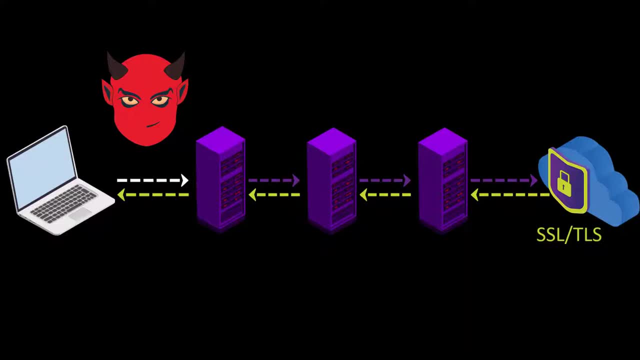 between them. Observer, can't only see that you have access to the Tor network. The SSL and TLS certificates mentioned here both encryption the traffic between you and website. Some the websites use SSL, others use TLS certificate. For the rest of the course, I will be referring the both. 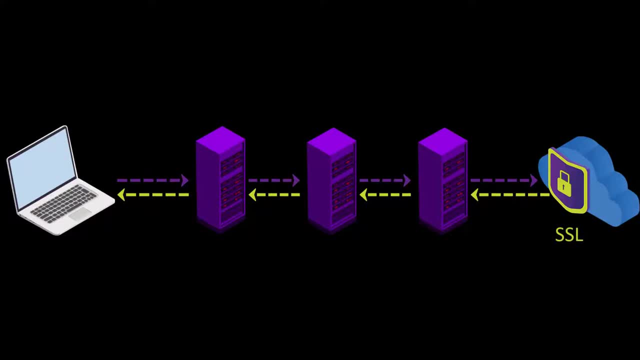 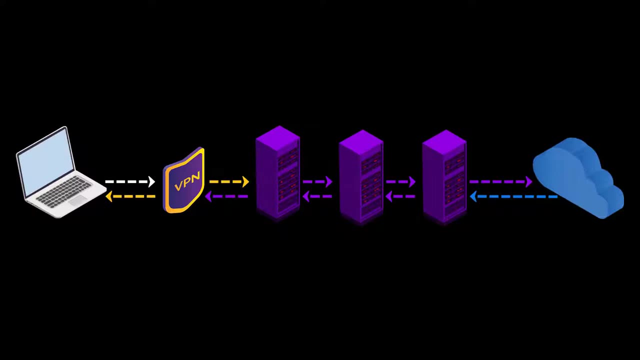 certificates by simply saying SSL. When you connect to the Tor network over VPN, your internet access appears as like that Advantages of connection to the Tor network over VPN. Your internet service provider or any observer on your network can't see that you are connecting to. 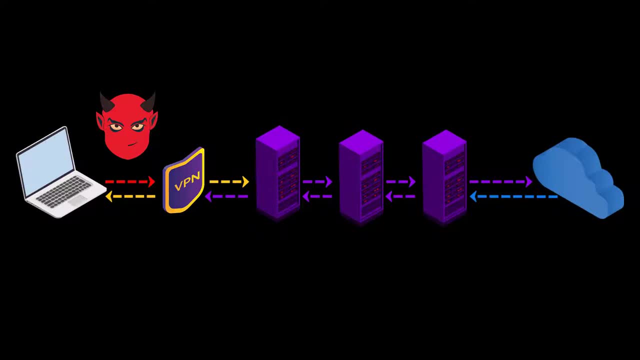 the Tor network. It only sees that you have established a VPN connection. Since VPN use is much more common than the Tor network, this creates relatively little doubt about your internet traffic, Because the communication between you and the entry nodes will be encrypted by the. VPN observers or malicious entry nodes on the network cannot breach your privacy, Since the Tor entry nodes will see the IP addresses of the VPN servers you are using instead of your real IP address. you will hide your real IP addresses even if the entry node 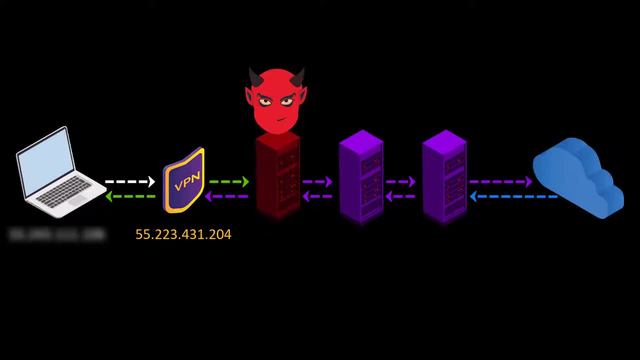 is malicious. However, for real anonymity at this point, your VPN servers shouldn't be keep logged. Otherwise, your anonymity may be violated by associating your real IP addresses with the IP address of the VPN servers. In addition to these advantageous features, there are also: 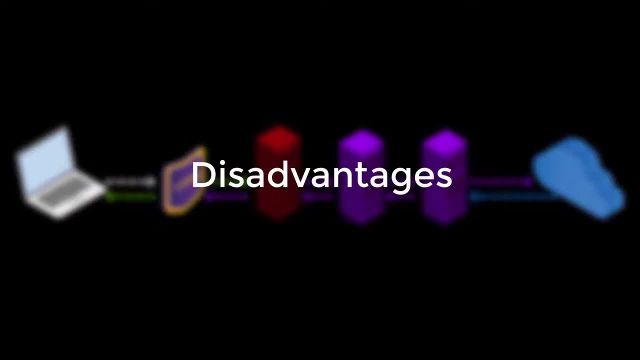 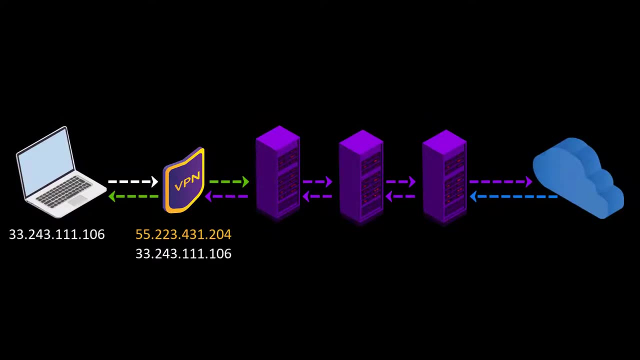 disadvantages we experience when connecting to the Tor network over VPN, Your VPN servers, known your real IP address. If it skips logs or is an unreliable service for any reason, it can reveal your true identity. At this point, it is very important to choose the reliable service. 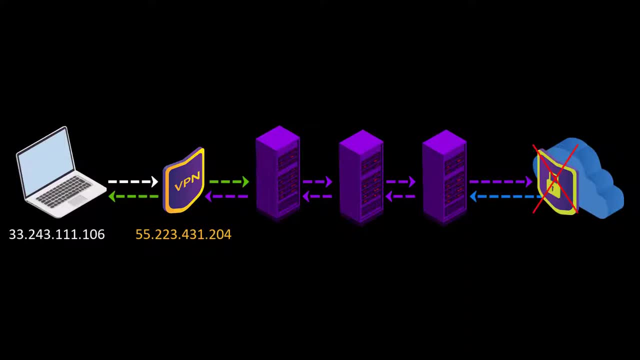 If the web addresses you are visiting doesn't contain SSL protection, malicious exit nodes may read by the website response to you. Although it isn't associated with your real IP addresses, there is a possibility that your data, in other words, your privacy, may. 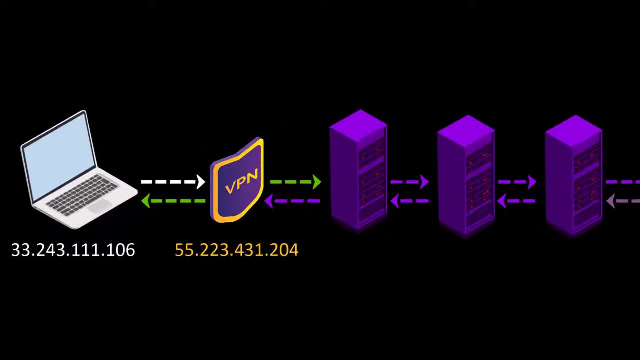 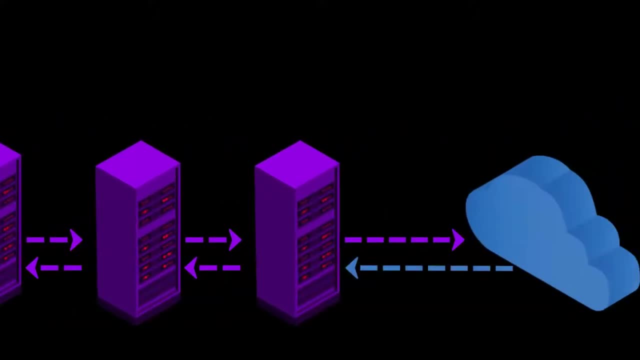 be compromised by the exit node, Because VPN only encrypts the data sent from to you, the entry node. the data sent by websites cannot be encrypted by the VPN while reaching the exit node. In such a case, if the exit node is malicious, it may. 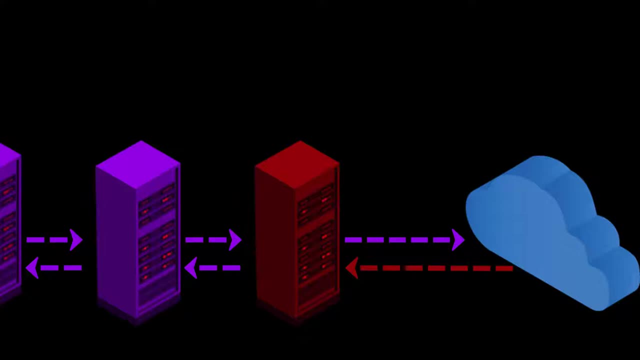 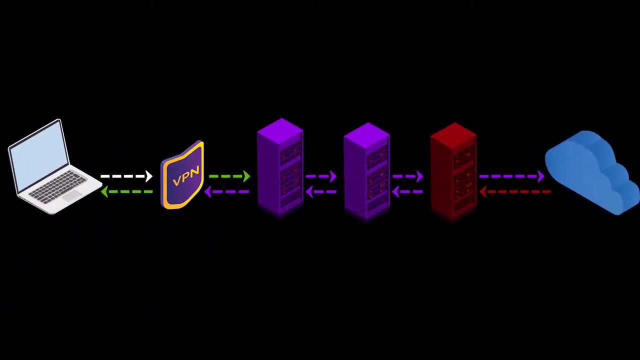 violate your privacy by reading the response sent from the website. However, this applies to any site that doesn't have an SSL certificate. In other words, it isn't a disadvantage of using VPN. I've just added it to this advantage list to indicate. 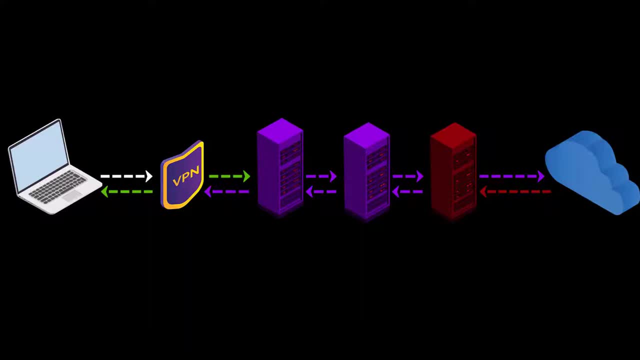 that visiting non-HD TPS addresses with only VPN used can also compromise your privacy. The only solution to this situation is to visit websites that use an SSL certificate. Another disadvantage is that, in addition to the slowness of the Tor network, 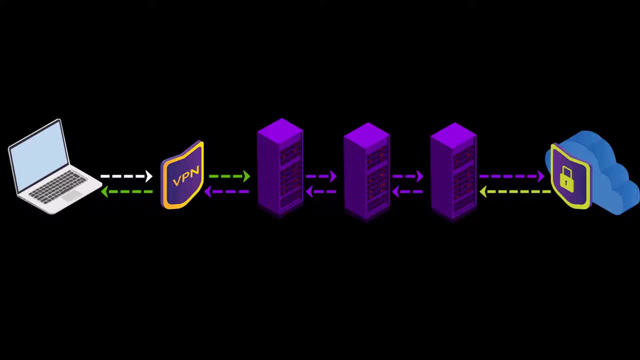 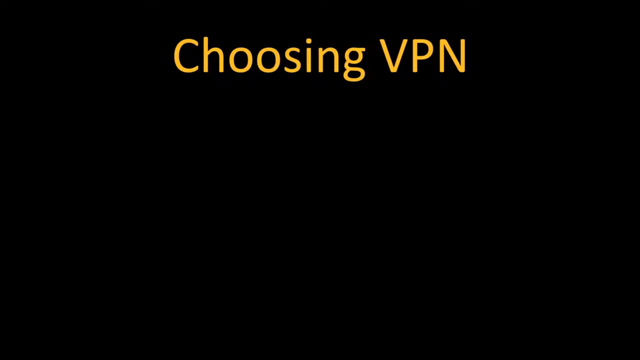 using a VPN will slow the internet speed more. However, considering the security it brings, this is not a big loss. The priorities you should be aware of when using the Tor network over VPN it is to prefer VPN services that provide uninterrupted service. 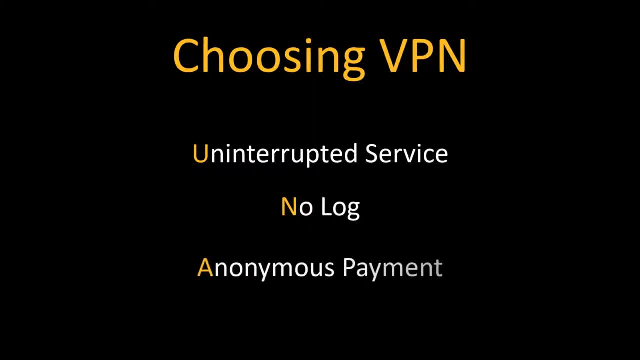 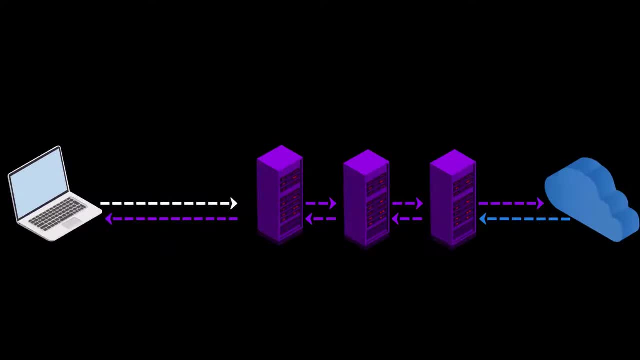 never keep logs and can payments anonymously. If you ask why these are important, if your VPN connections drop, when you connections to the Tor network over VPN, observers on your network can learn that you are connecting to the Tor network. In addition, the entry nodes, which is the 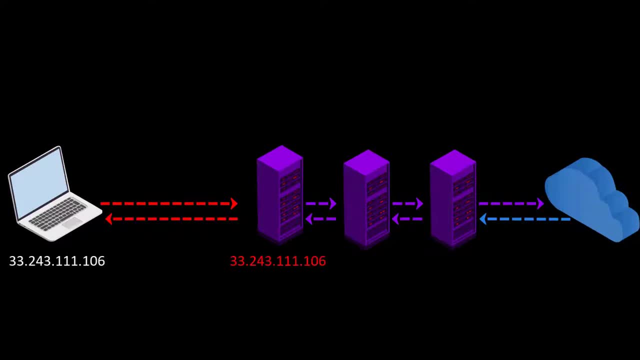 first node can learn your real IP address during the connection drops. If the VPN servers keep logs, all the security and privacy measures you take will be in vain, as the origin point of all activities you do will be known by your VPN servers. 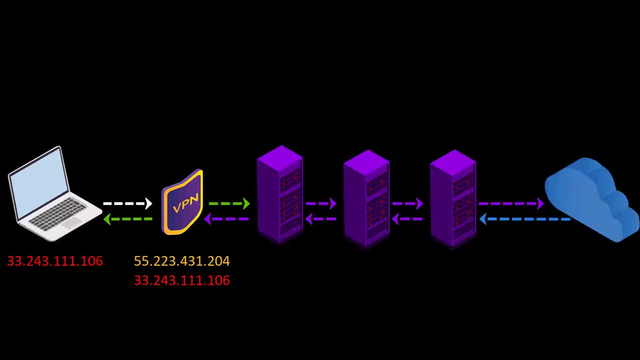 Logging means that your entire internet record is associated with your identifier. In such a case, it doesn't make much sense to be using the Tor network When paying for a VPN service, it is very important to pay in cryptocurrencies to protect your holistic anonymity Thus. 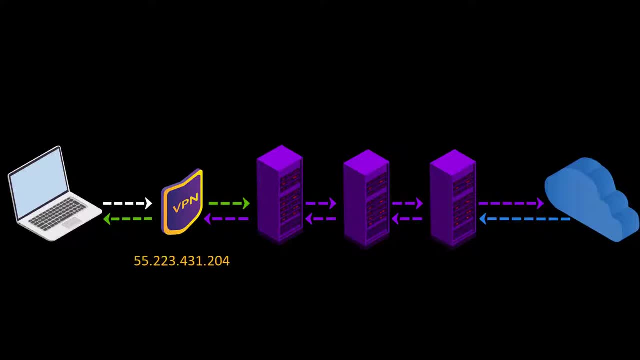 when the IP address of the VPN server, standing in front of your real IP addresses, is surged, it cannot be directly associated with your real identifier. In course, we will also be talking about how cryptocurrencies give us anonymity. At this point, you have to decide. 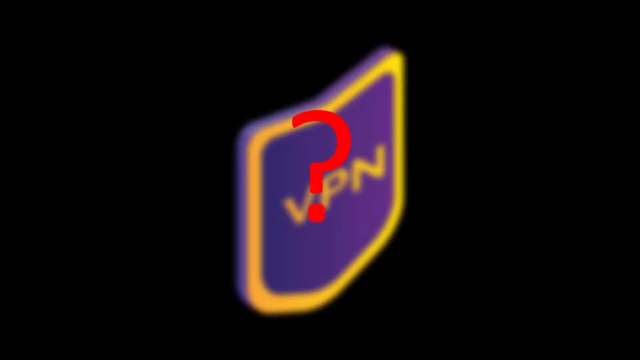 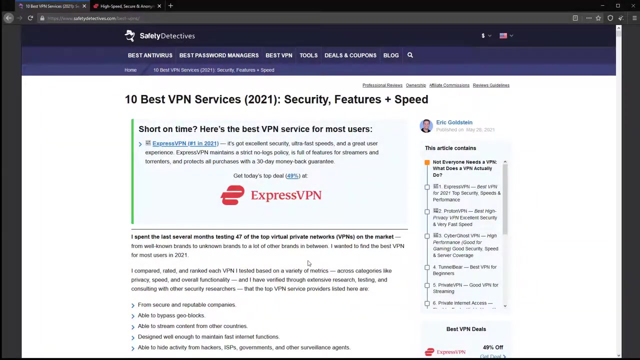 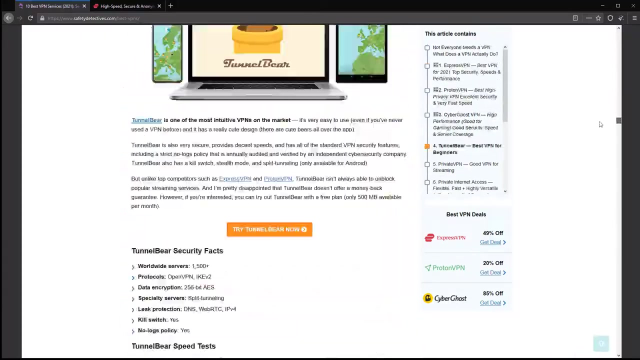 for yourself which is the most ideal VPN service. It can be difficult to determine which VPN service is trusted, So you may want to check out this VPN comparison chart by the OnePrivacy site, which analyzes almost 200 VPN providers based on their jurisdictions and policies. 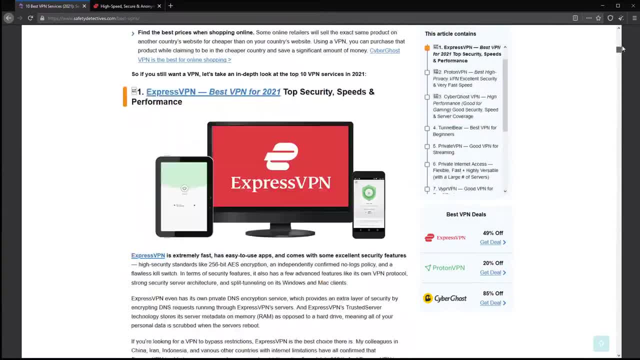 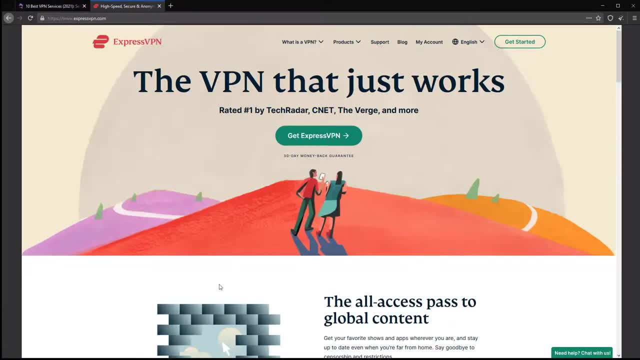 For example, in the period I reviewed the list, ExpressVPN was chosen as the most ideal VPN service. In addition to being on the list, according to my personal experience, I can recommend you to use ExpressVPN. My recommendation reason: it has proven by: 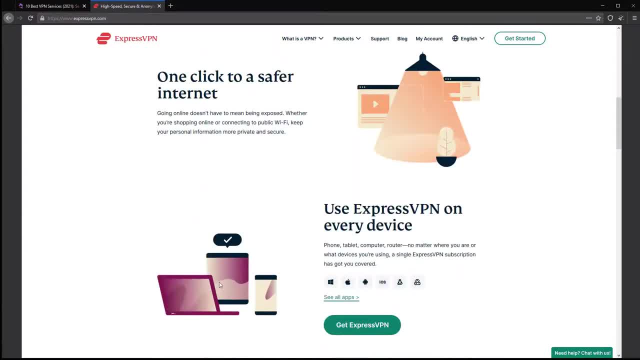 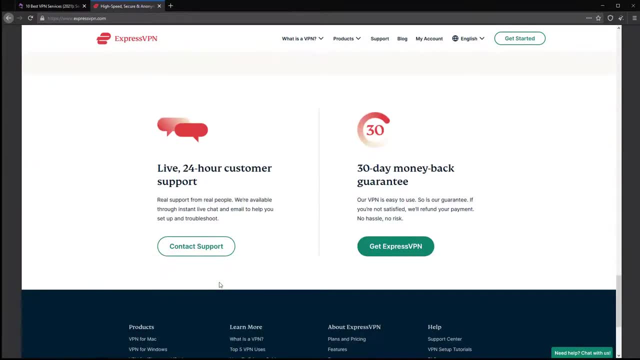 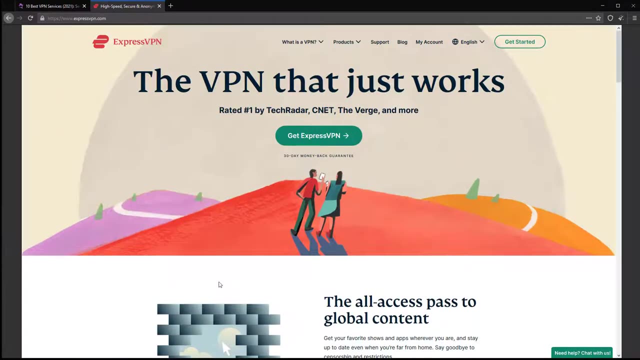 independent organization that it doesn't keep logs and prevents the leak of your real IP address by disconnecting the internet as soon as the VPN connection is lost. You can use the Bitcoin for payments and you can also get a refund if you are not satisfied by trying the service. 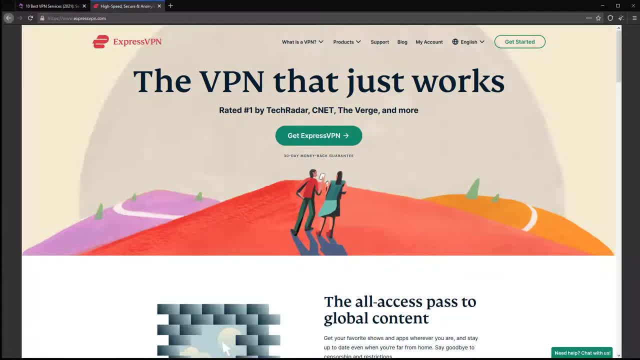 for a month. Although this service is ideal, in my opinion, you can, of course, take a look at alternative services and make your own decision. In addition, what I explain here isn't an advertisement for the service. It is a service that I have specified to share. 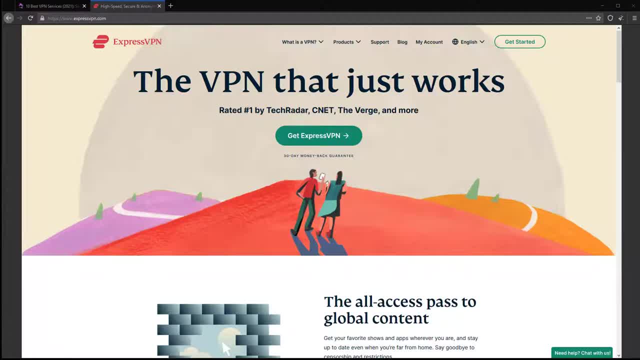 my personal opinion. for suggestions purposes, I've created a special discount link for this course so that only those who want to use it can use it at a discount. I've added the link to resources for this lecture. You can try it if you want to use it. 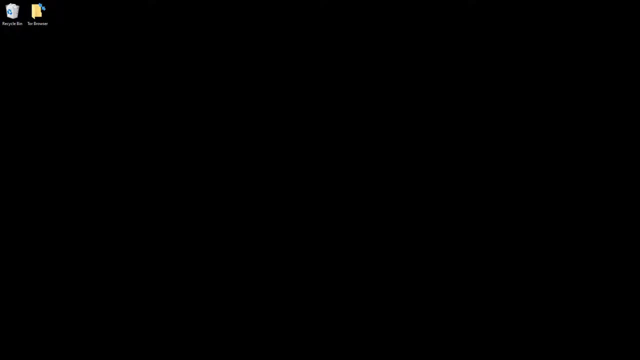 After choosing right VPN service, all you have to do use Tor over VPN is to start the VPN services of your choice before connecting to the Tor network. To connecting to the VPN service, you need to download and install the application of your preferred service on your 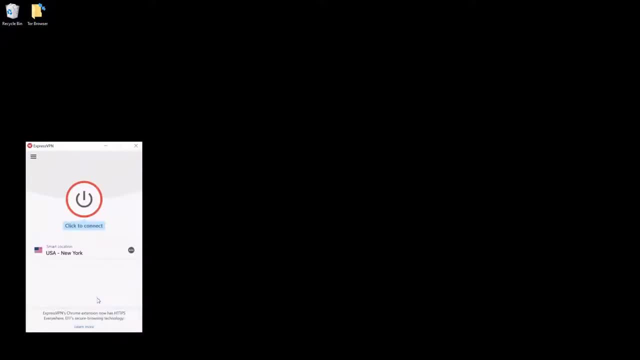 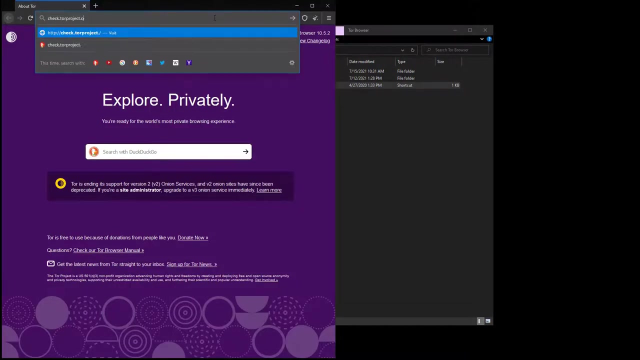 system. After the installation process, you can make the VPN connection very easily. For example, after establishing the VPN connection of the ExpressVPN service, when you connect to the Tor network through the Tor browser application, you can ensure security communication, as anyone who observes. 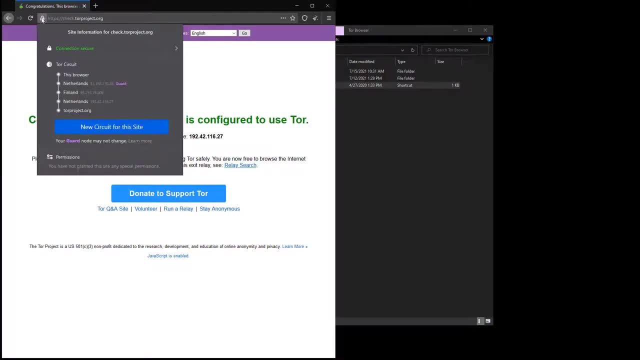 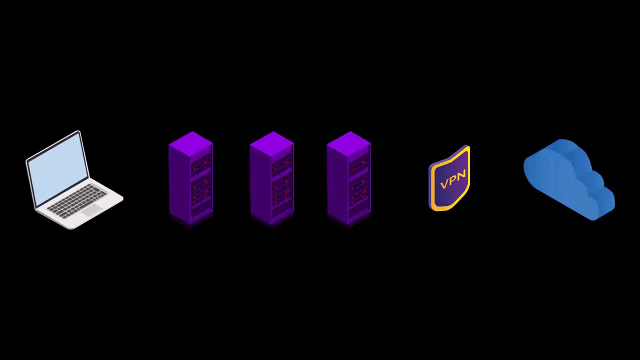 your internet and Tor network can only see that you are establishing a VPN connection- VPN over Tor- In this connection type, in contrast to connection type I mentioned in previously lecture. your internet access looks like this: At the time of preparing this course, there were: 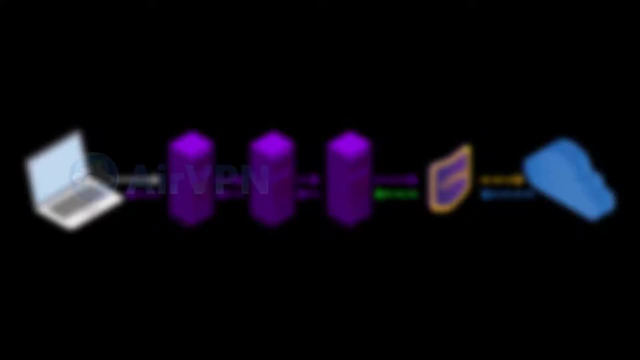 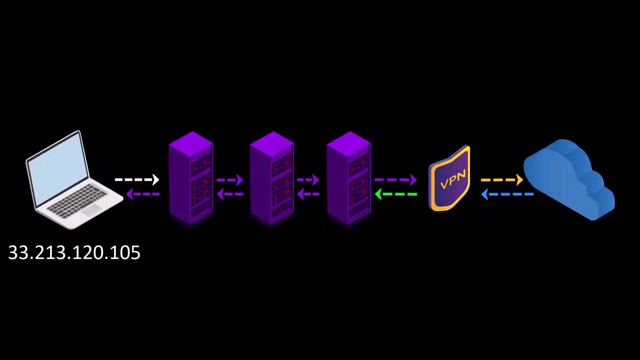 only two VPN service provider, AirVPN and BolehVPN- that provided this service. If we briefly touch on the advantages and disadvantages of using VPN over Tor: Advantages: since you are connected to the VPN server via Tor, the VPN provider cannot see your real 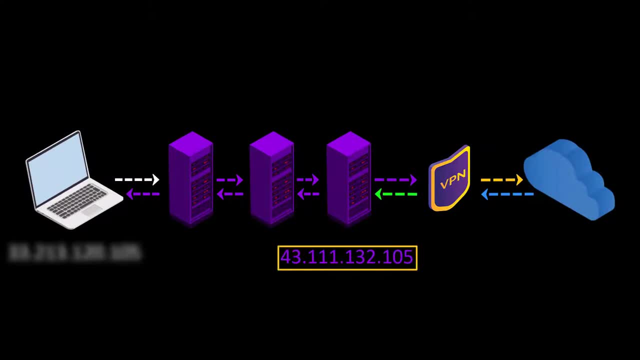 IP address, Only the Tor exit node's IP address. Assuming that you pay for the VPN service anonymously with secure cryptocurrency, your anonymity won't be compromised. even if the VPN service keeps a log, You can use it to visit websites that block visitors from the Tor network. 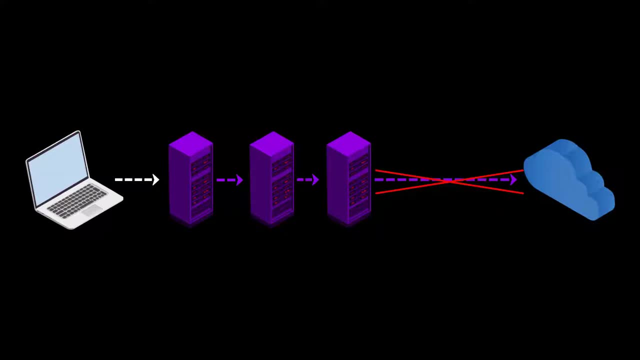 Some websites block users connected to the Tor network for security reasons. When you use VPN over Tor, your VPN connection will appear, so you can overcome this obstacle. However, it would make more sense to use only VPN. to visit such websites Disadvantages your internet. service provider and anyone observing your network can see that you are connecting to the Tor network. Your VPN provider can see your internet traffic. However, because the traffic comes through the Tor network, it can never be directly associated with you if doesn't know your real identity. 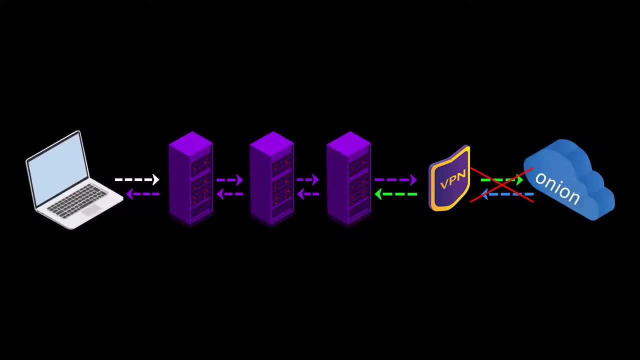 You cannot access websites with ONION services via VPN. The fact that the Tor network connects to the single VPN point can be a disadvantage for the timing attacks I mentioned earlier. However, if you made a payment anonymously, even if the information is leaked from the 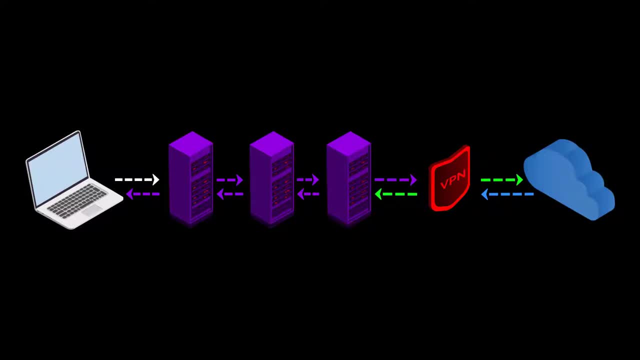 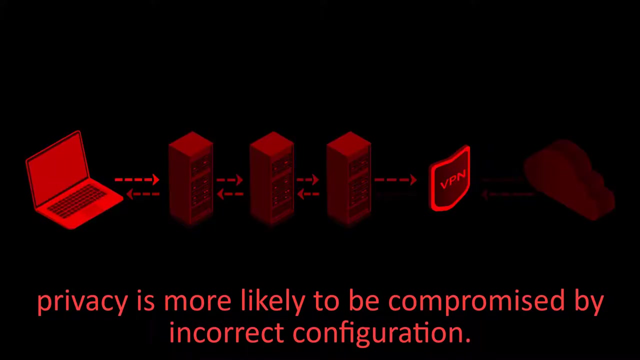 VPN service. it cannot be directly associated with you. In addition, it's somewhat more difficult to configure your internet connection and privacy is more likely to be compromised by incorrect configuration. Configuration settings may vary depending on the service provider used. When we consider all, 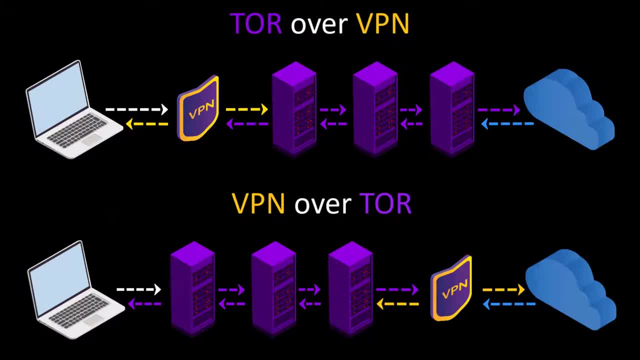 these advantages and disadvantages. it can be said that using the second method, VPN over Tor- is not a good choice for many people. If you are using the right VPN service, the first method- Tor over VPN connection- will meet all your needs. I don't recommend. 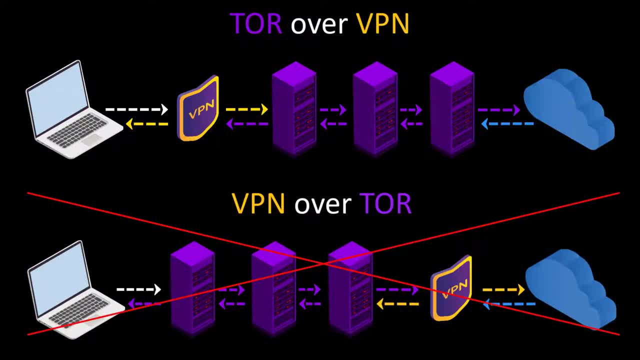 using VPN over Tor method and won't be covered in this course. I just wanted to explain it briefly so that you are aware that such a method also exists. Although Tor alone provides you with very good anonymity, You can decide to use the Tor network over. 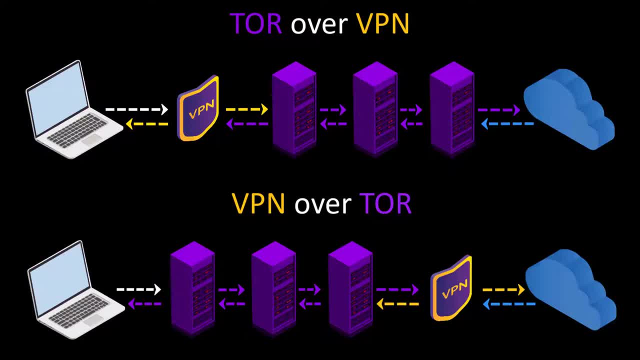 VPN or alone, depending on your needs, considering the advantages and disadvantages of using VPN, For example, if the address you want to connect to has an SSL certificate and you don't want to hide the information that you are connected to Tor network from your internet service provider, or 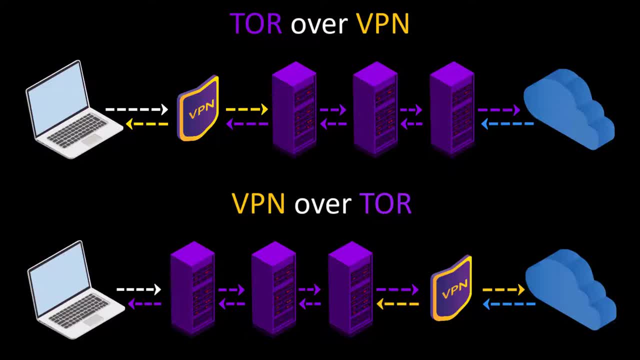 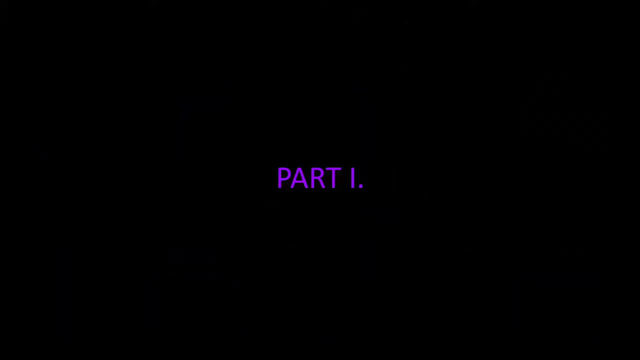 observers, you don't have to use a VPN. Yes, you have finally learned to bypass all obstacles and securely connect to the Tor network via Tor browser. Now let's talk about the Tor browser settings and why those settings should exist. Tor browser settings. 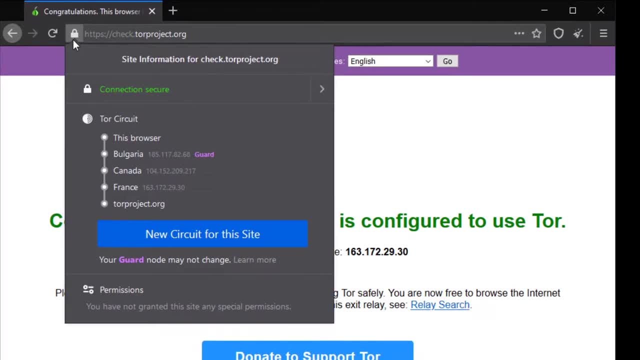 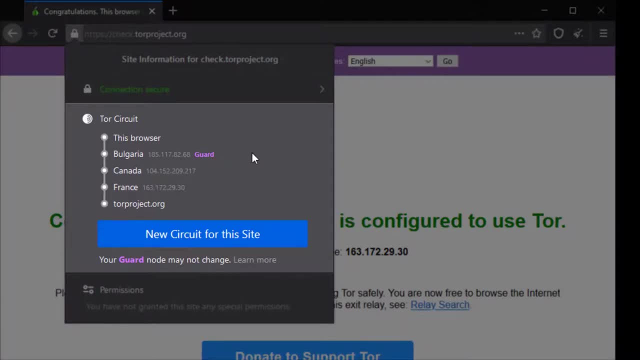 When you visit any website, by clicking this icon in the search bar of your browser, you can see through which Tor services you are connected to the website. Also, if the website has SSL certificate, there is the phrase connection secure here, as you can see. First, 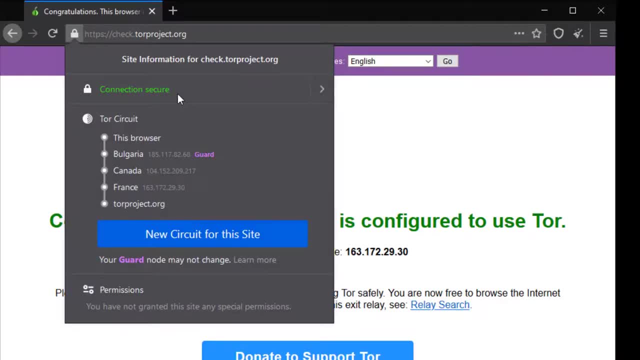 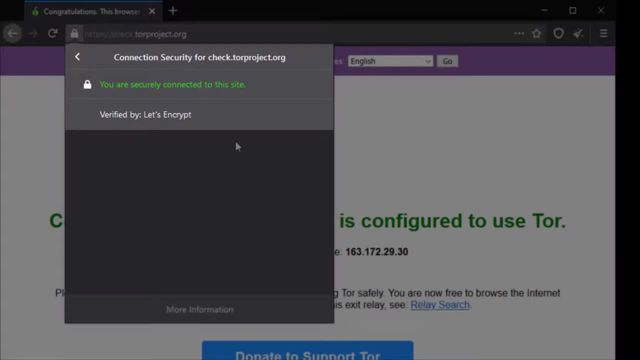 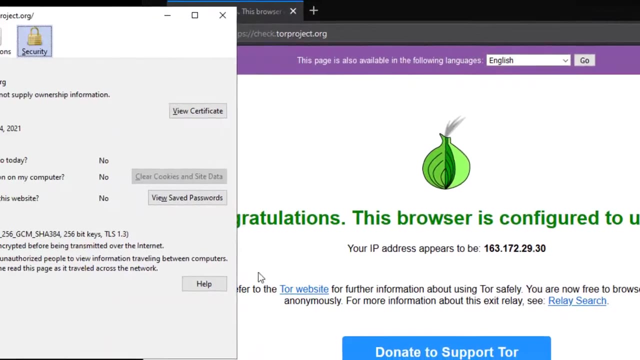 of all if we start with certificate audit. for example, I am currently at checktorprojectorg and can view information on whether this website is safe for communication. Also, I can click the more information button to get more details and assign specific permissions. 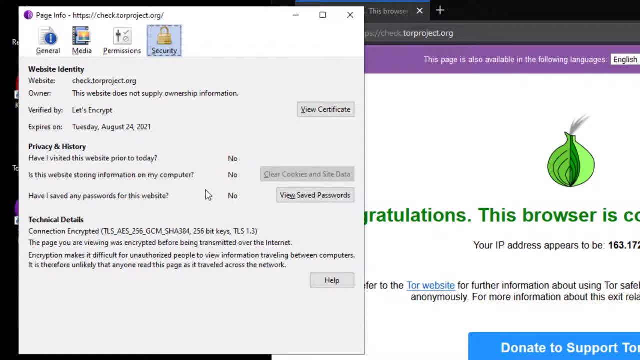 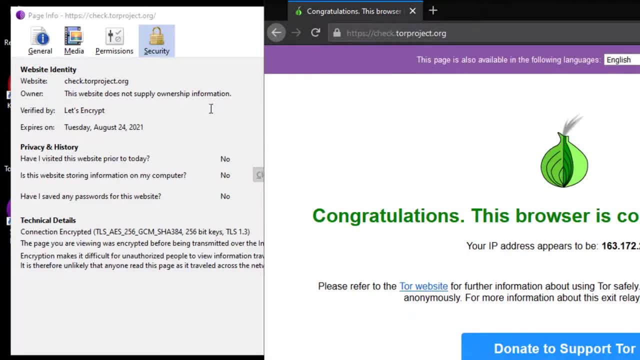 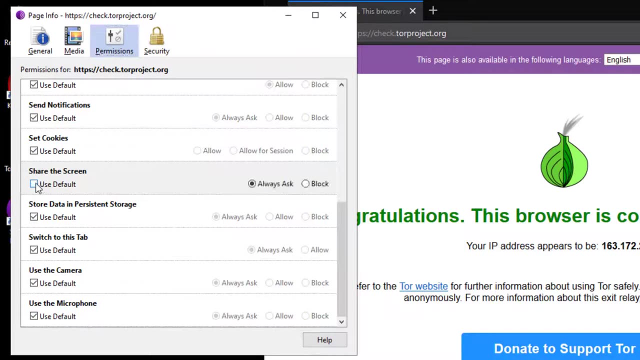 to this site. As you can see, I have received more detailed information about the certificate of the site. Apart from certificate detail, you can set permissions for current website from the permission tab. In order to change the permissions, you need to uncheck the use default. 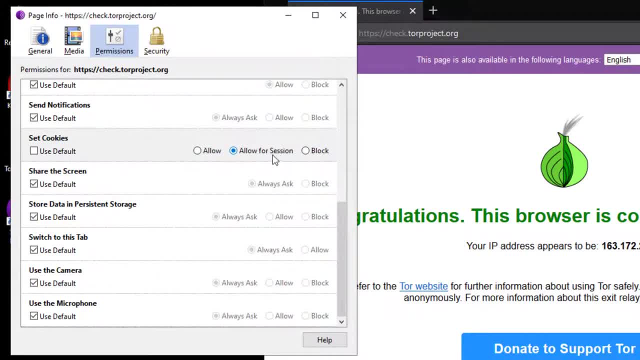 option. As you can see, you can allow the feature you want and block the ones you want. However, for your security, it would be much better to keep the settings here- default, But of course you can change these permissions differently from the default. 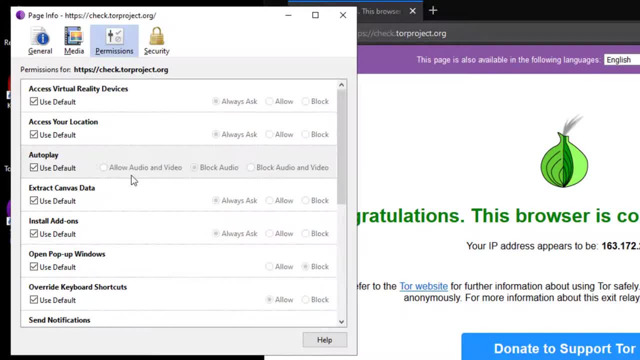 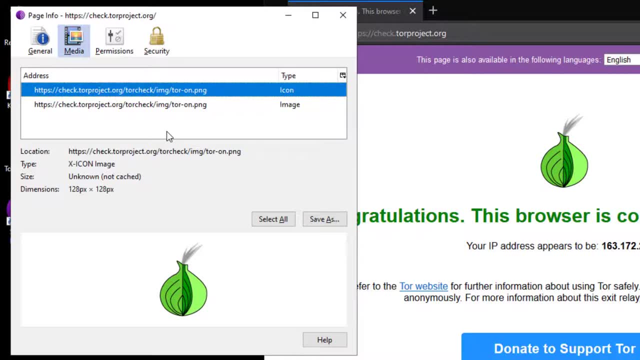 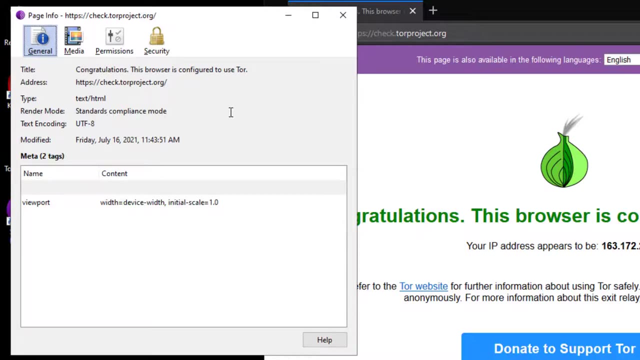 Especially for the websites you trust whenever you need them. For the media tab, you can obtain the information of the materials, such as pictures and videos, owned by website. In the general tab, you can obtain general information such as the title and addresses of the website. I also want. 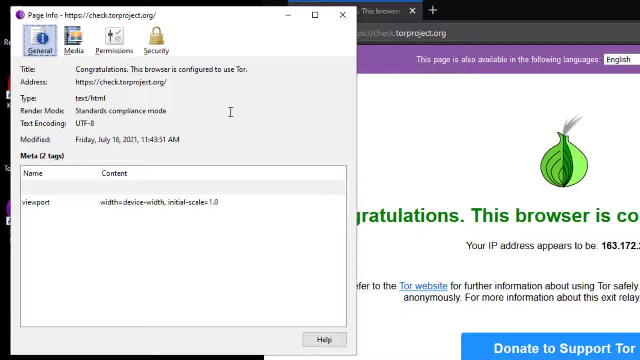 to remind you that this feature allows you to get information about, certificate and manage site permissions- is not only available in Tor browser. I just want to talk about the purpose of use, in case you don't know or don't care if you know, Checking such information about. 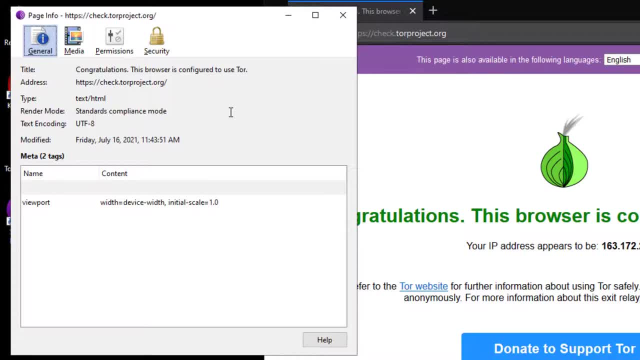 the website you are visiting to and managing its permission is very good habit in terms of security. Even if you haven't paid attention to this until now, you have now learned that it is an important detail to pay attention to this part for your privacy. 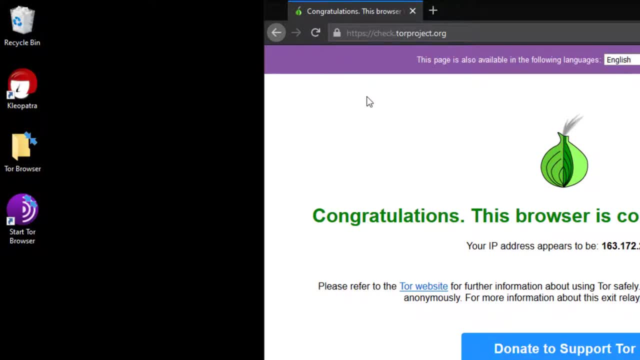 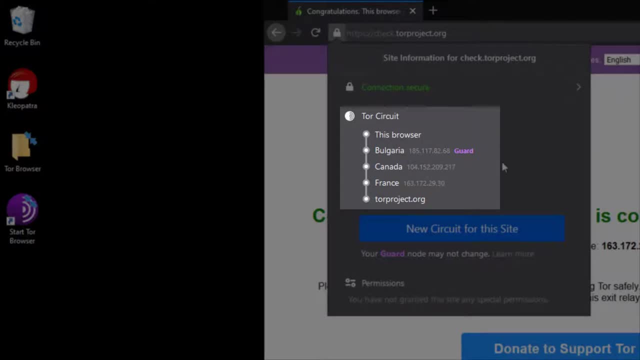 You know, Tor Search Sheets gives the information of the servers you are connected to Tor Network. As you can see, I am currently communicating with checktorprojectorg via this Tor Search Sheet. Except for the first node in the search sheet, the middle, 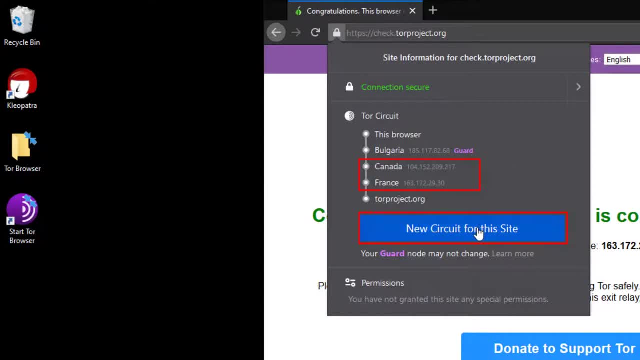 and exit node can be easily changed with the new search sheet for this side button here. In addition, if you don't refresh manually, the search sheet will automatically change itself every 10 minutes, except for the entry node. But why does the entry node? stay the same despite the renewal process. This is because the entry node in the circuit is selected as a guard. It is a fast and stable node that stays the same for 2 to 3 months, as we have already mentioned, to protect against. attacks that could compromise your anonymity. The entry node usually doesn't change for the 2 to 3 months, unless there is a server-side issue. In exceptional cases, when your security is at stake or your server is not working properly, you can witness. its change automatically in short time. In short, the fact that the entry node doesn't change is the most effective security method that can be used now to protect against possible attacks on the Tor Network. contrary to feeling of insecurity it creates in you For more technical. 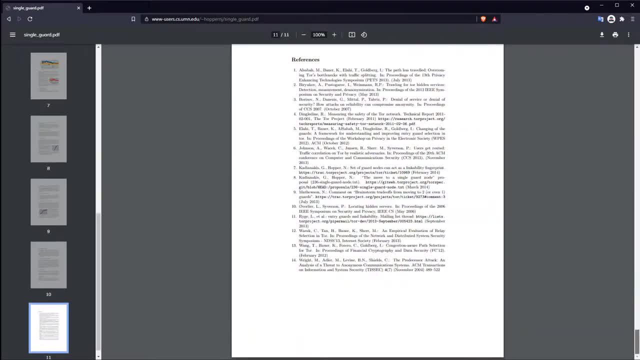 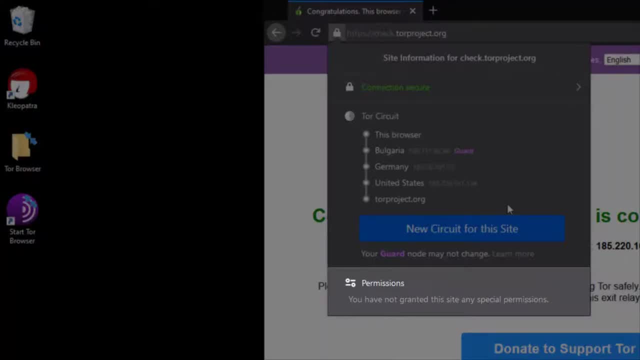 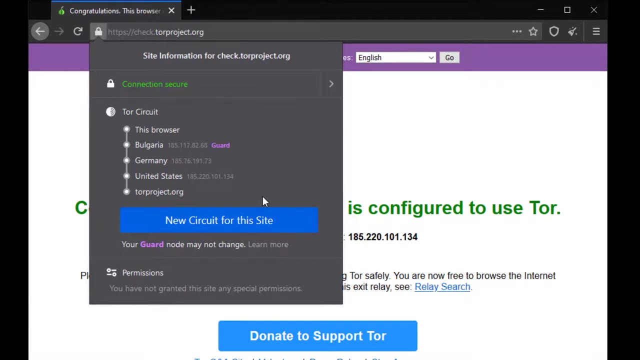 details. you can read the article published by University of Minnesota from the link at this: lecture resources. The permissions section under the Tor circuit shows the site-specific permissions. I will comment the permission issues again. I was explaining the settings in a moment. Now let's talk about the security. 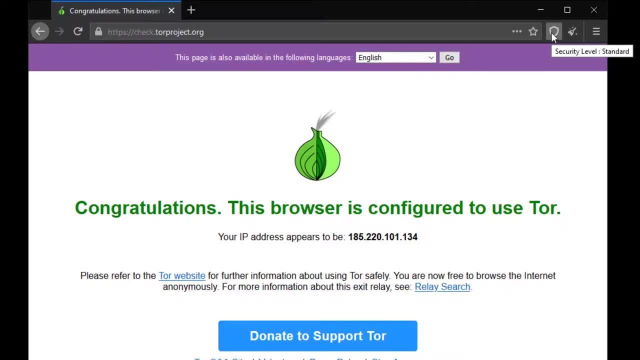 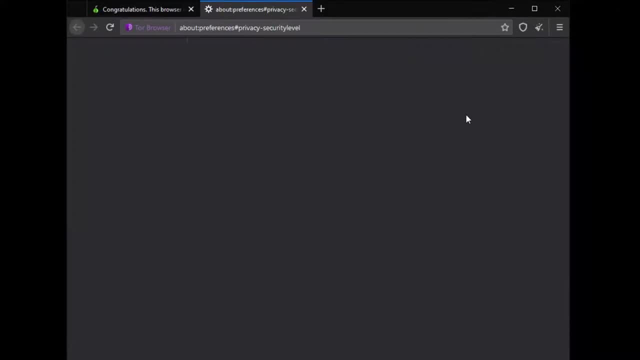 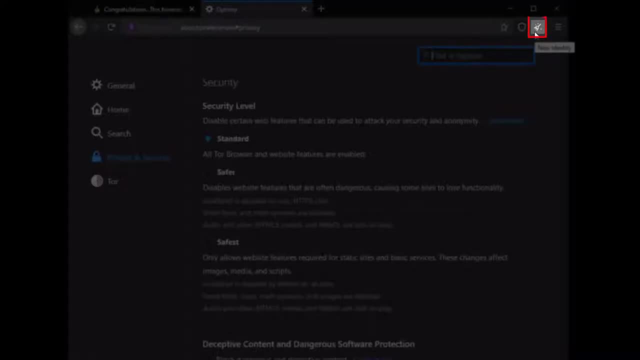 level and new identify buttons. The security level button is shortcut button that shows the security level settings in your browser and direct you to settings when you want to change it. We will talk about this security level settings and details later. The new identify button closes all. 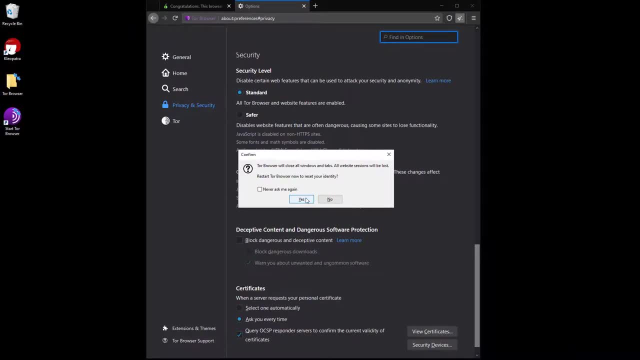 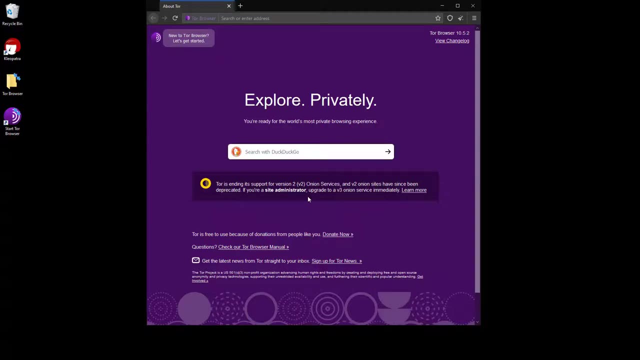 existing tabs and sessions you have opened on the browser and restart the browser by resetting your identify. The locations and functions of these buttons may change with the updates over time, So the browser you are using while following this course may look a little different from mine. 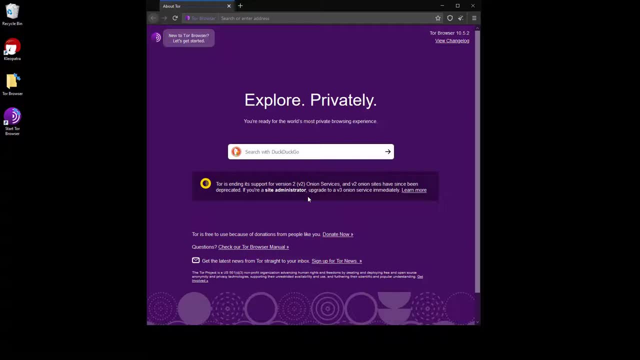 However, please note that such changes doesn't matter at the point of keep going to education. We are basically talking about what is necessary for safety in this course. If the location of the buttons change, you can find their location with a short lookup. If a new feature is, 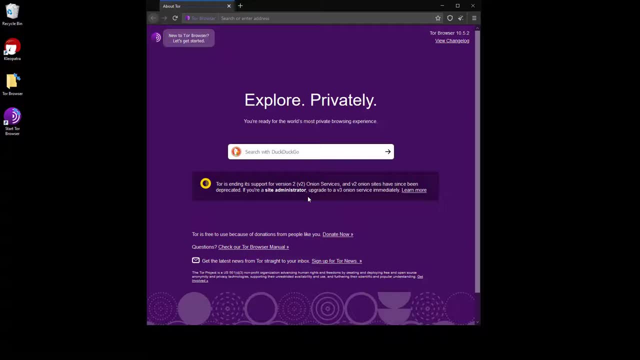 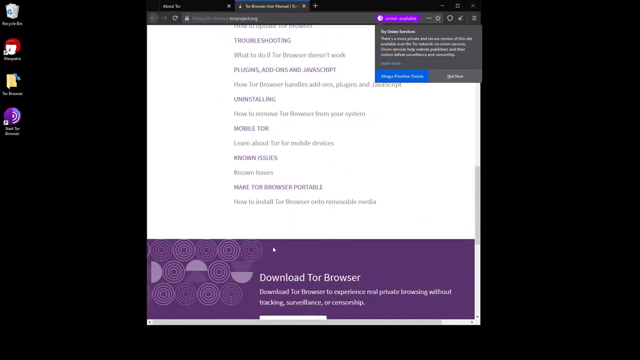 added or existing feature change. you can understand their use by reading short feature descriptions. In short, I want to say that you should always read new documents for the more useful features and constantly focus on what you can pay more attention for your own safety. 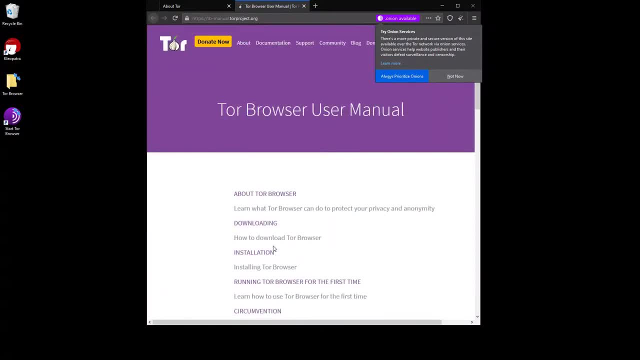 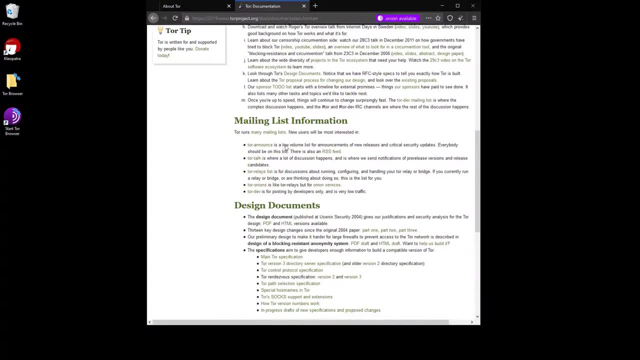 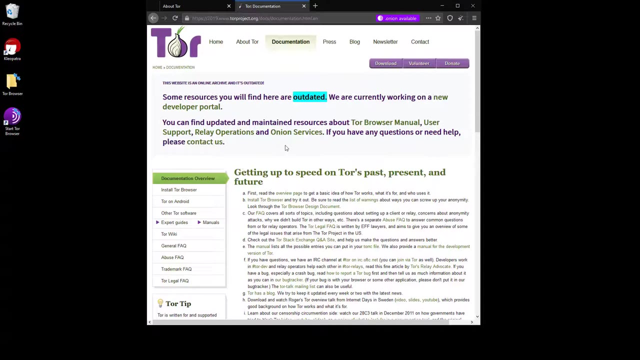 not limiting yourself. that you have learned in this course. Of course, the more we strive to ensure our security, the more those who want to violate our security will do. For this reason, technique use and security methods will be constantly updated and will change. 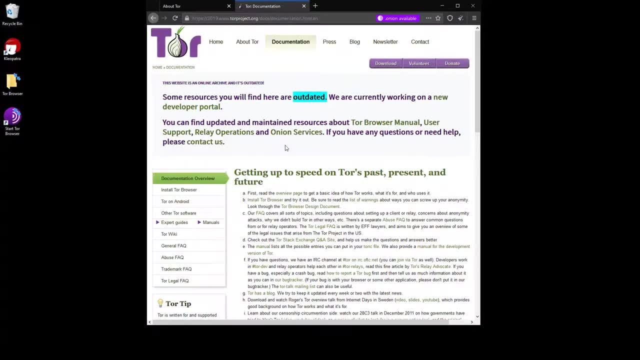 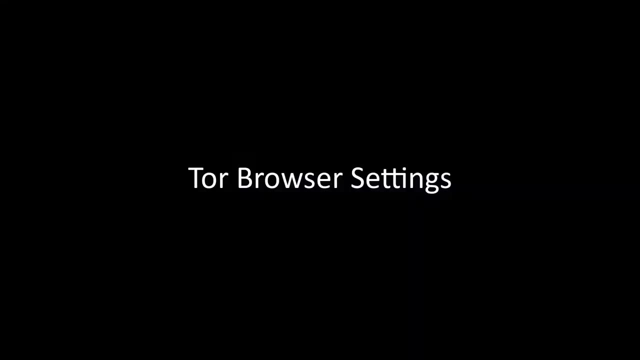 over time. You can only stay safe as long as you are open to innovation. After the brief explanation, let's open our browser settings and click on the Privacy and Security tab to browse the settings that concern our privacy Onion Services With this setting onion available. 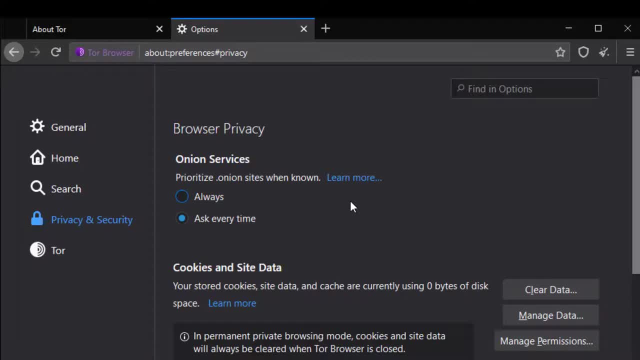 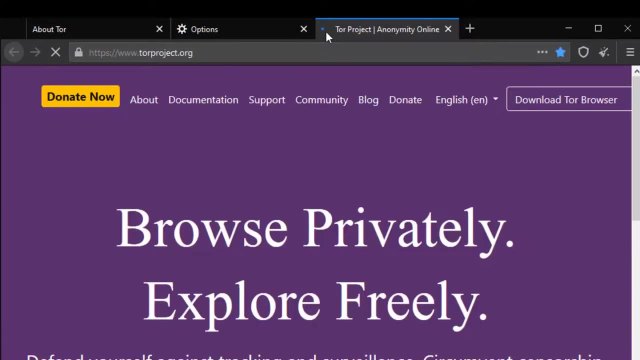 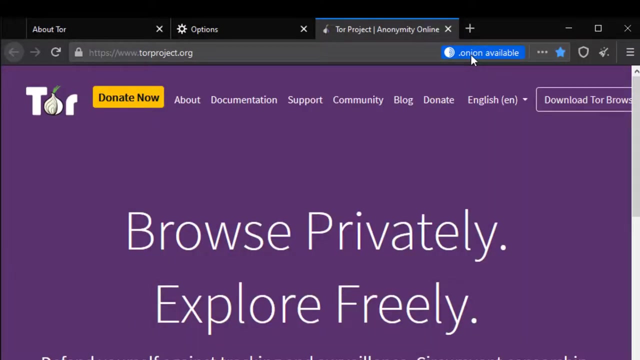 info will appear. if the website you are visiting has a known onion services address, You can visit torprojectorg to try it out. As you can see, it is stated here that the website you visited has an onion address, If you click on it. 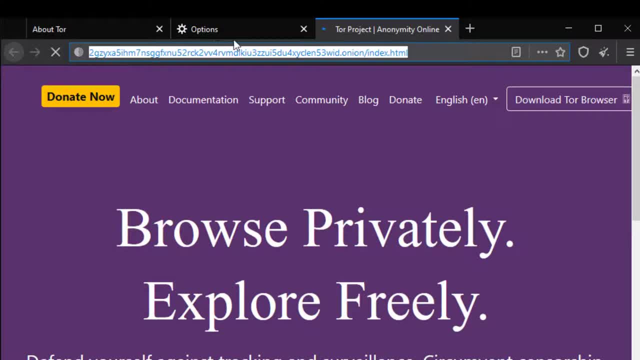 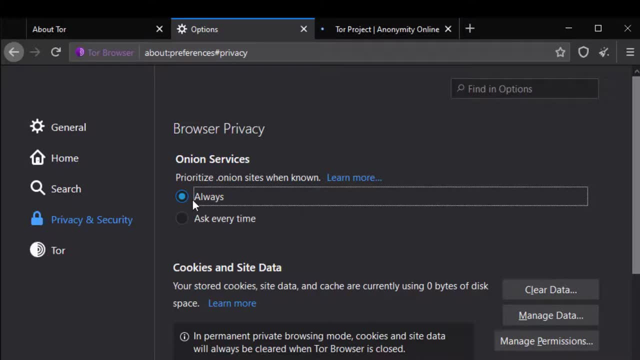 you will be redirected to the onion address If you set onion service settings. always if the website you visit has a known onion address, you will be automatically redirected to the address without asking you. You can visit torprojectorg again to try it out. 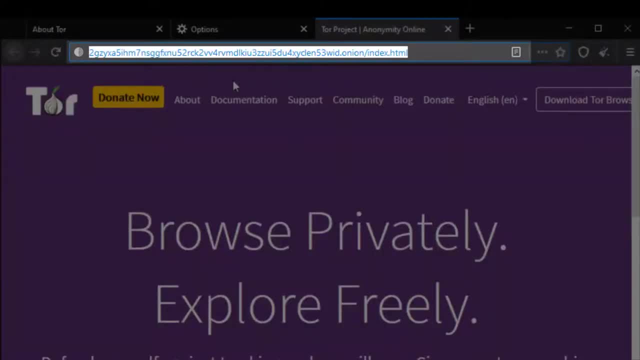 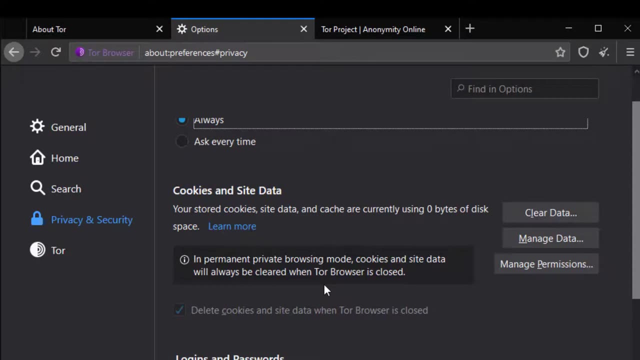 As you can see, you automatically redirected onion address, Cookies and site data. The settings in this section allow you control the cached data of sites. You can perform operations such as deleting and managing from here. However, as you can see, all data. 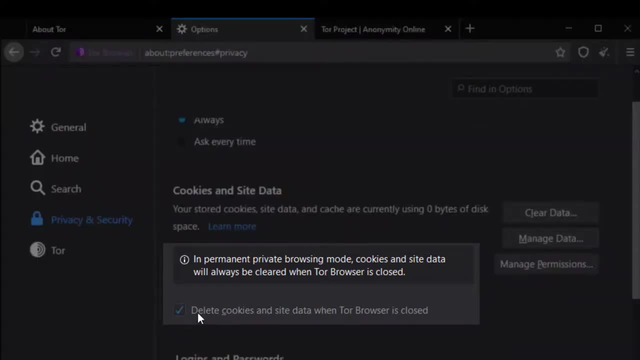 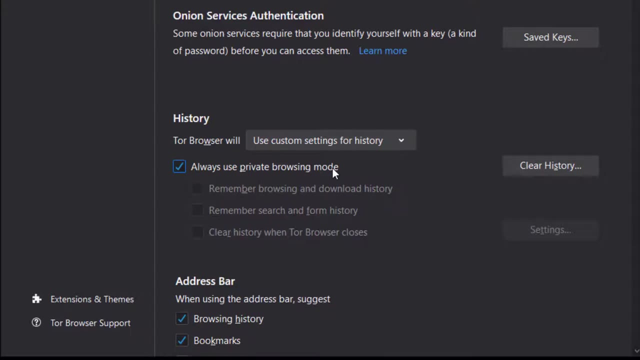 records are currently marked to deleted automatically when you close the browser. This is because the always used private browsing mode of torprojectorg at the bottom is active. With this feature, you can use your tor browser without leaving any traces about any website. My suggestion: 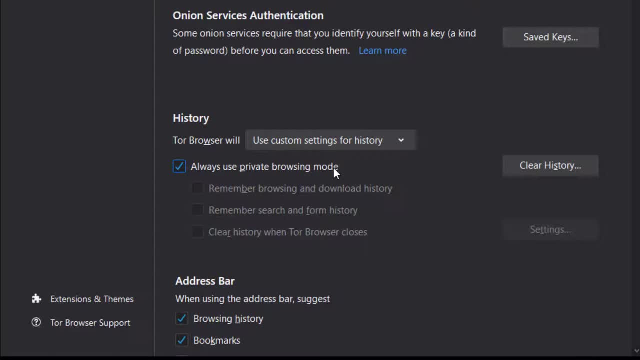 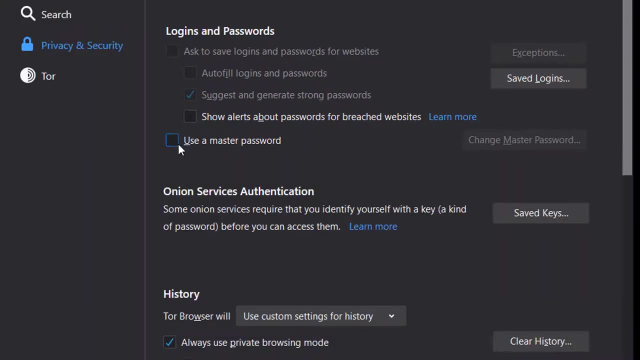 is to keep this setting active to ensure your privacy. However, if you still want to keep your data of your past visits and visited sites, you can customize the settings here as you wish. Logins and passwords: The use master password feature here ensures that. 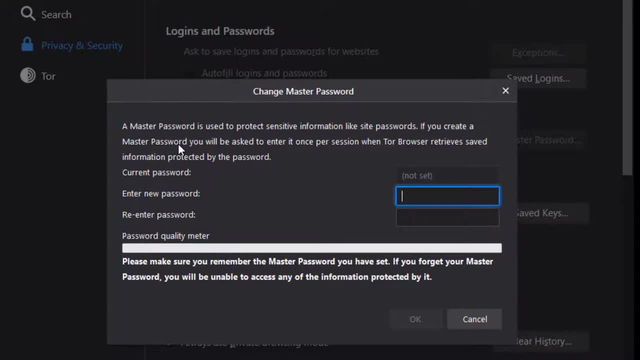 if there are passwords for your logins in the tor browser, these passwords are also protected with a master password. This means that if you create a master password, you will be asked to enter it once per session when tor browser retrieves saved information protected by the password. 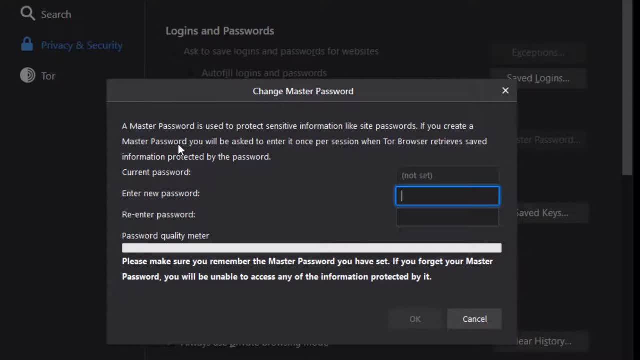 In other words, it provides an extra protection for local security. This feature prevents someone who accessed your browser locally from accessing your information. I mean by accessing locally. it describes situations such as your computer being for inspection or hacking by someone. However, you should note that 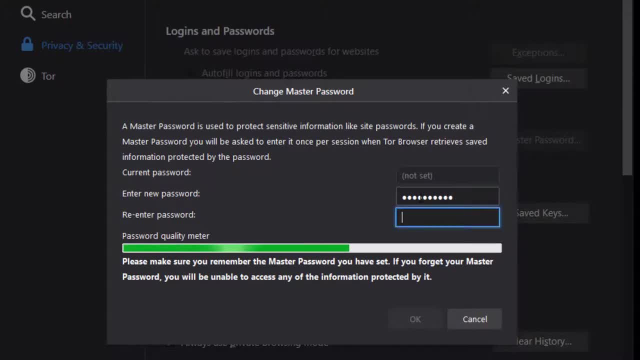 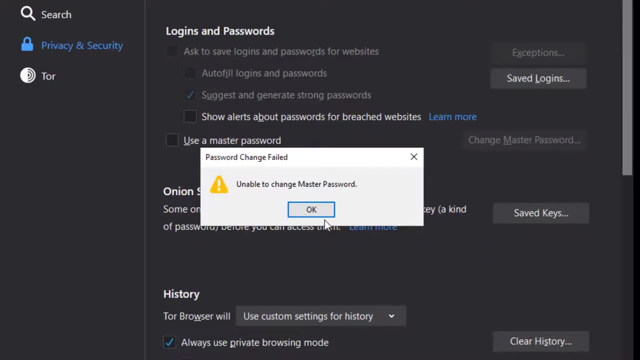 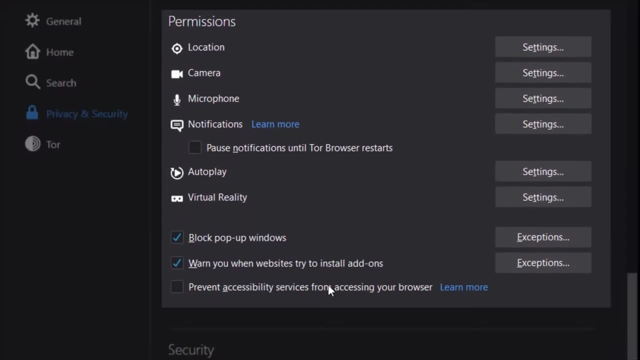 if you forget the master password, you will never be able to access data stored on your tor browser. So, while setting a password, make sure you set one that you will not forget, as well as strong Permissions. While we were talking about permissions earlier, we 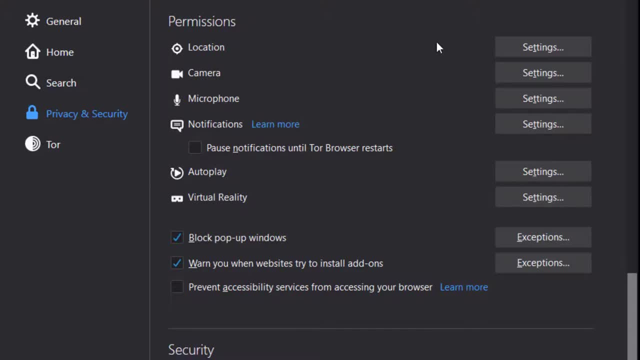 mentioned, that can define special permission settings to website. Unlike the permission settings we mentioned earlier, the permission settings here allows you to define common permission settings for all websites. in the tor browser, For example, if you take a look at the location setting in the window that opens, 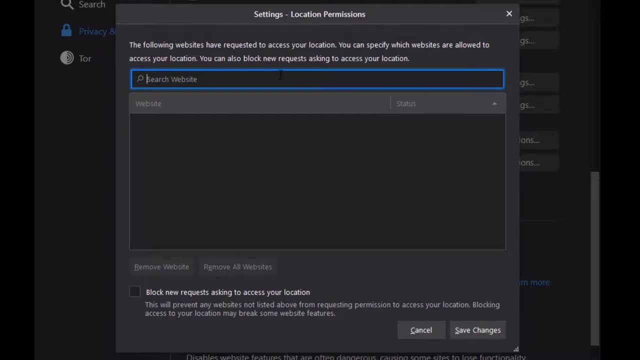 if you have defined a website that can access location information exceptionally, it will appear. In addition, it will be sufficient to check the block new request asking to access your location option below to complete the block location information except for exceptionally websites. I suggest you. 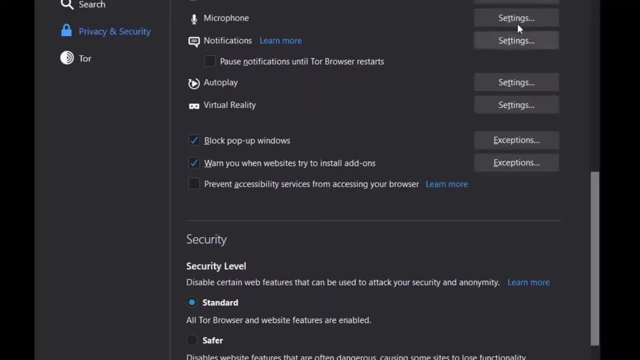 select this option for all permissions one by one, if you not select it by default. Since you can change these permissions specific to website, it would be much better to block these permissions altogether in order to ensure general protection. In addition, I strongly recommend that you 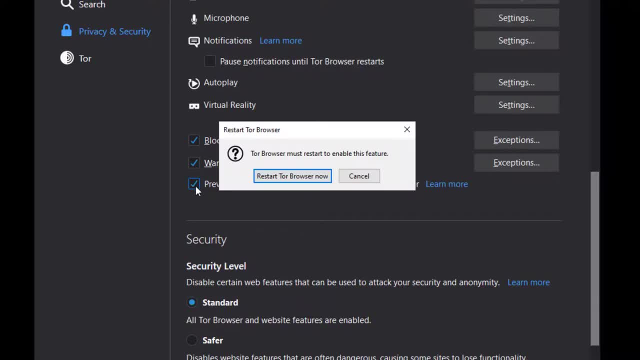 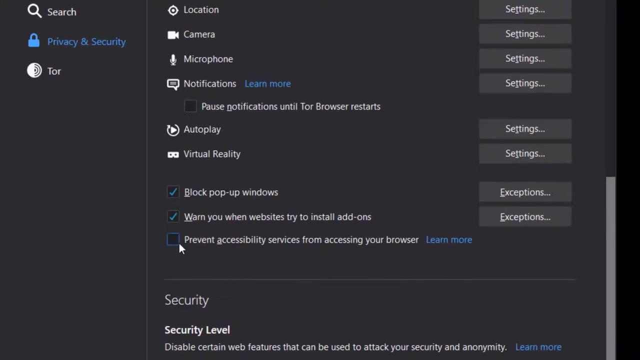 can choose the prevent accessibility service from accessing your browser option under the permission. To fully understand the purpose of this feature. you can get briefly information here. However, as I said, my suggestion is to prevent accessibility services from accessing the tor browser if you don't need to use. 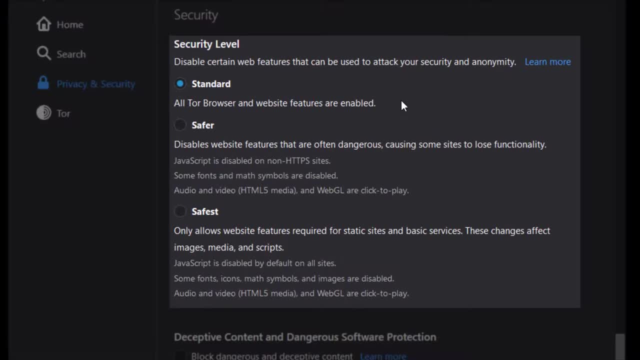 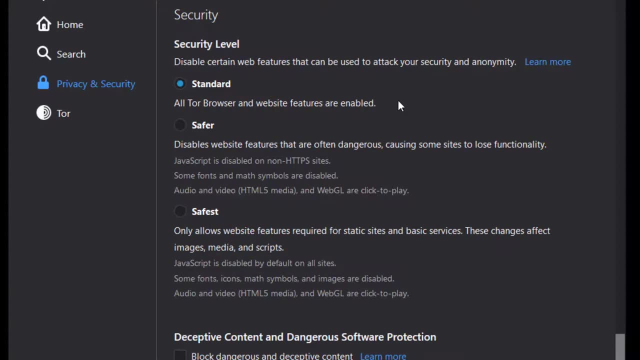 accessibility services Security. In this section, there are security levels that you can use to neutralize possible attacks from all websites you visit or will visit. If the standard security level is selected, your browser will behave just like an standard web browser, vulnerable to many possible. 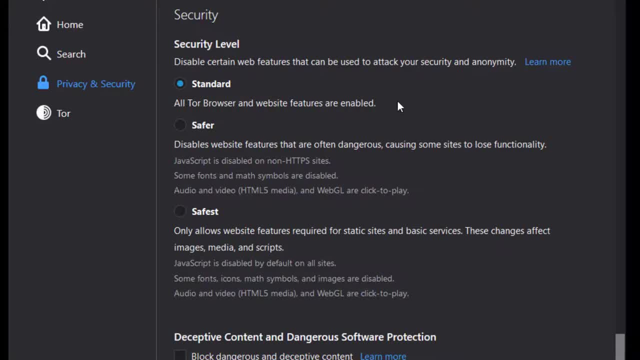 attacks from websites. It has already been stated here that all tor browser and website features will be enabled at this security level, So this option doesn't impose any restrictions. If the safer security level is selected, partial security is provided by disabling the features. 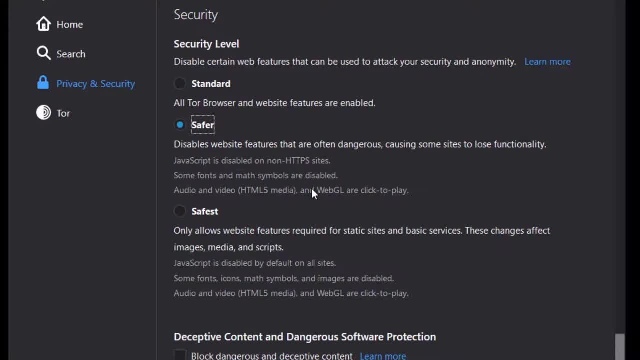 specified in the list. Of course, there may be loses in the functionality of sites used together with the closed features. If the safest security level is selected, many features of websites will be disabled for even more comprehensive security. It is generally used to access the website in much more. 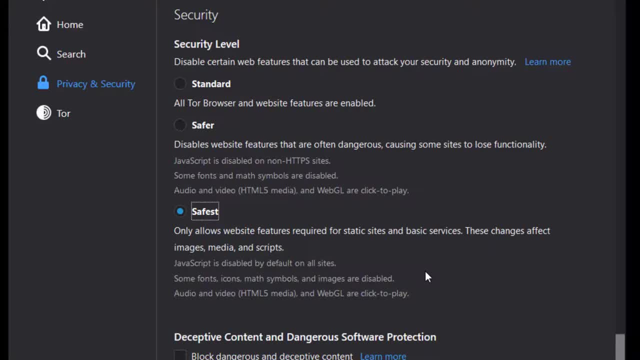 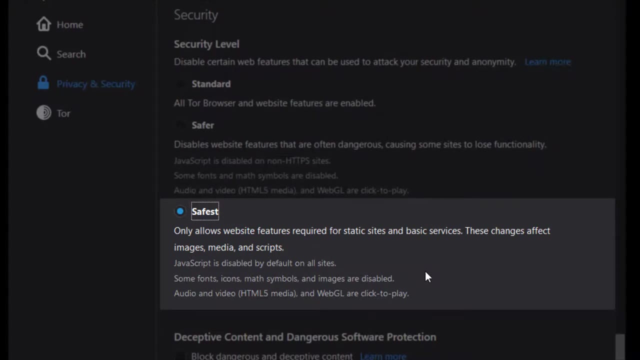 simple and secure way. Please also note that all disabled features may vary based on discovered vulnerabilities over time. In other words, in addition to used features that appear in Minaw, different features may have been disabled in the period you use Ultimately using. 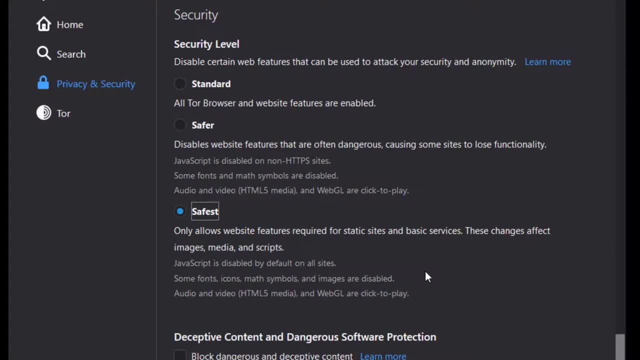 these security levels, you have to choose and consider the status of the website you want to communicate with. If the website you are visiting is unrelatable and you still have to visit it, you can choose safest security level. Or if the surface is one, 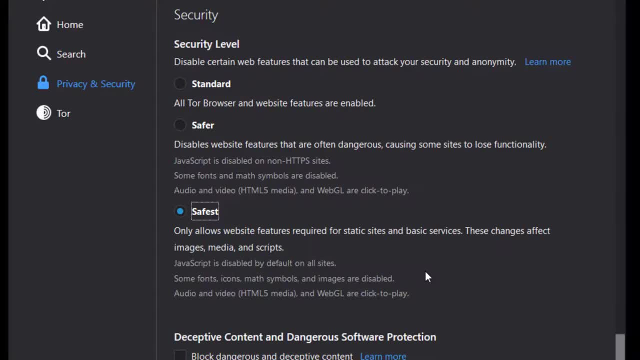 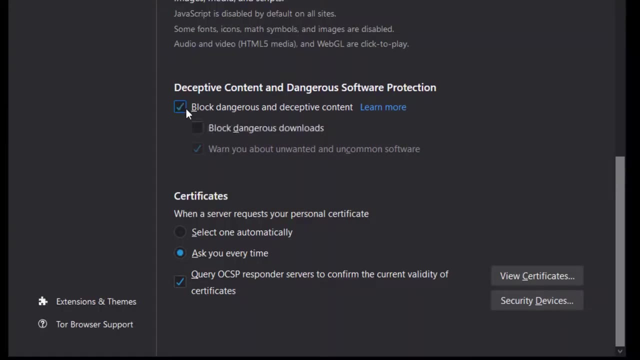 of the reliable servers on the web. you can just select the standard or safer option. It's all about what you can expect from the website and what kind of decide is Deceptive content and dangerous software protection If you activate this feature in this section. 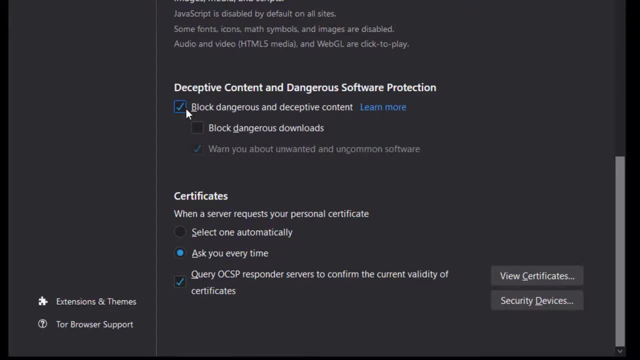 you will be warned before accessing content with a previously reported security risk In. additionally, if you want to block dangerous downloads, you can activate block dangerous downloads option Enabled. this feature can help you avoid unintentional security risk Certificates. It would be more better choice. 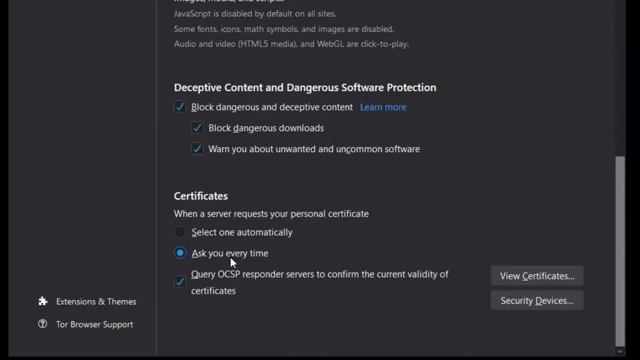 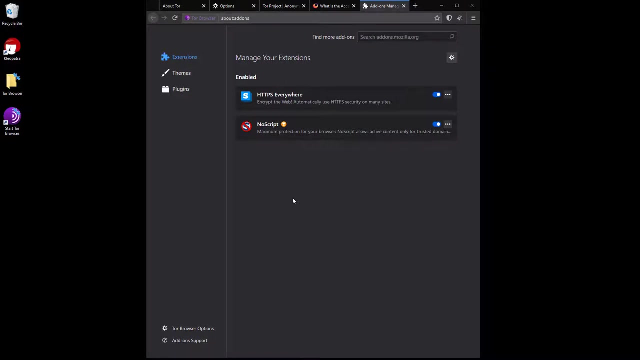 to keep the certificate settings as you every time selected. However, if you have special situation, you can choose the select one automatically. Details for additional security Extensions to secure the browser are already installed by default. Apart from this, it is strongly not recommended. 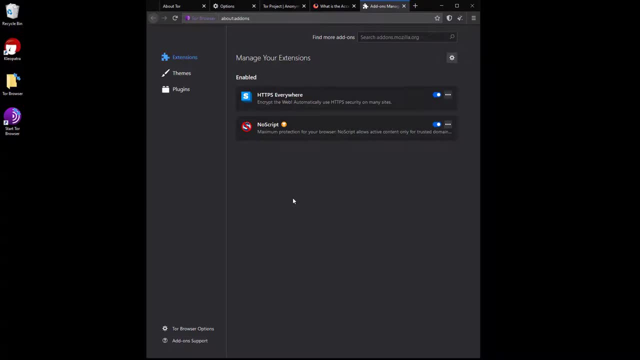 to install new extensions Similar to extensions. I strongly recommend that you don't install new themes and use the default theme among existing themes. It's never recommended to change such default settings for a much more ambiguous user identify. we mentioned earlier Installing new extensions. 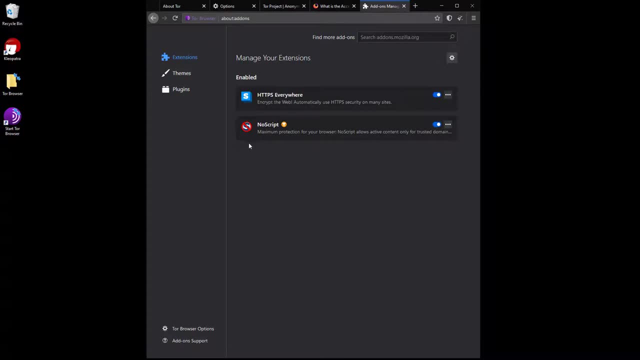 can affect Tor browser in unpredictable ways, causing the Tor browser you are using to create a unique fingerprint. If your Tor browser has a unique fingerprint, that is, if you have a usage habit that can notice among these other users, your action will no longer be anonymous. 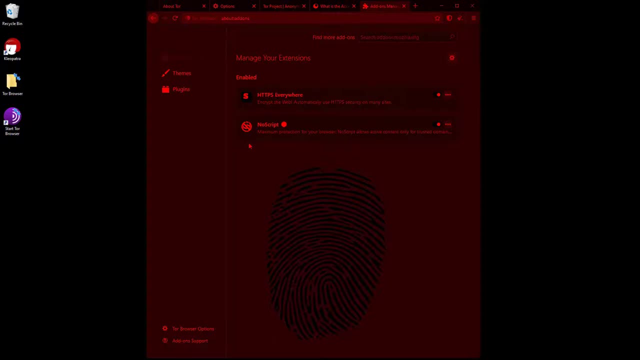 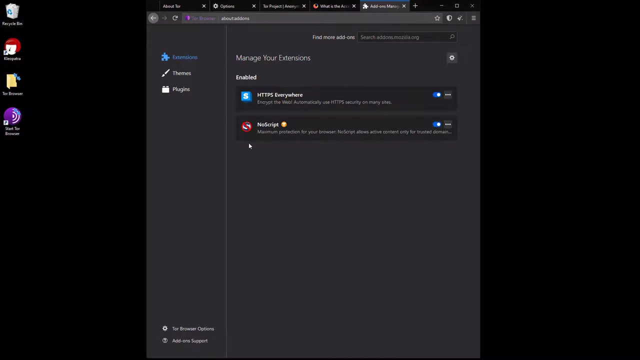 and you can be tracked even if you are using Tor browser. Basically, the settings and features of each web browser create a unique web browser fingerprint. Since most web browsers do not care about this, each user can create a unique fingerprint that can be tracked on the internet. 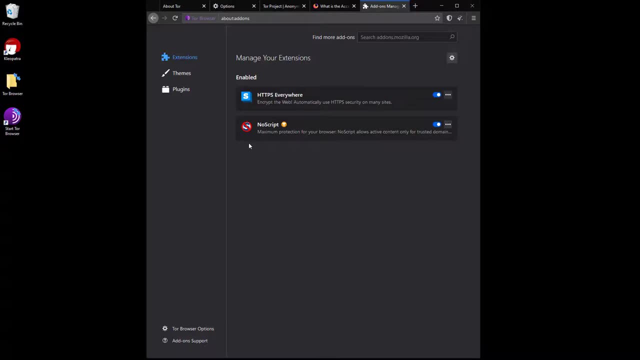 Unlike the standard browsers, the Tor browser is specifically designed to ensure that users fingerprints are nearly same. This means that the fingerprints of all Tor browser users are similar. This situation makes it difficult to track Tor user. Also, each new extension has the potential to increase the. 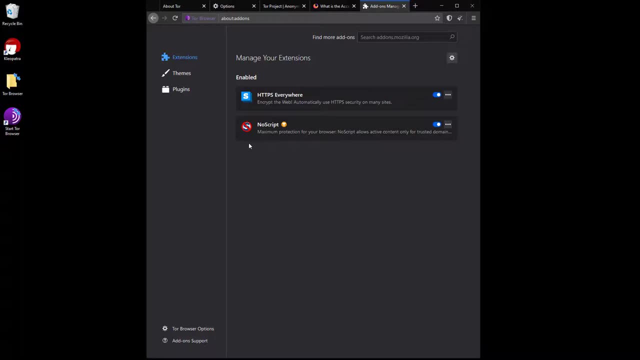 attack surface of the Tor browser application. This could cause personal data to be leaked or an attacker to infect the Tor browser with malware. Even the extension itself may have been maliciously designed to track you. Tor browser application comes with HTTPS everywhere and no script extensions installed. 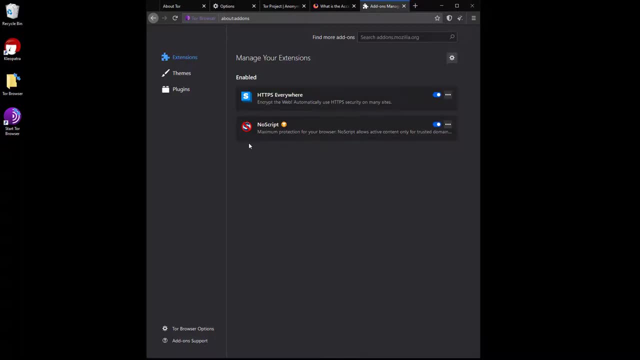 Installing an extension other than that may prevent you from being anonymous. However, over time, there may be changes in the extension used by default, That is, the extensions that come with the Tor browser. If this is the case, the Tor browser has made it. 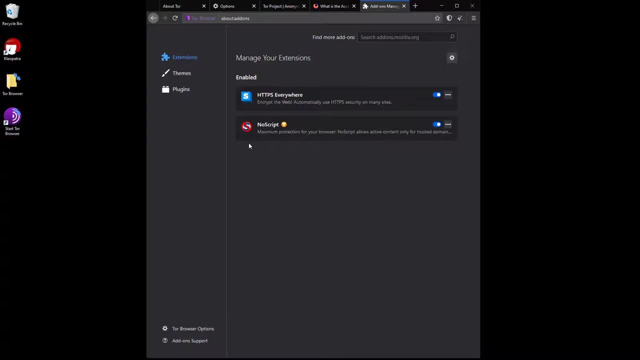 available because it is sure of the security and benefits of extension. However, if you are skeptical about any extension, you can find a lot of information about why the extension is located on the Tor browser and its possible effects by doing a short internet search. 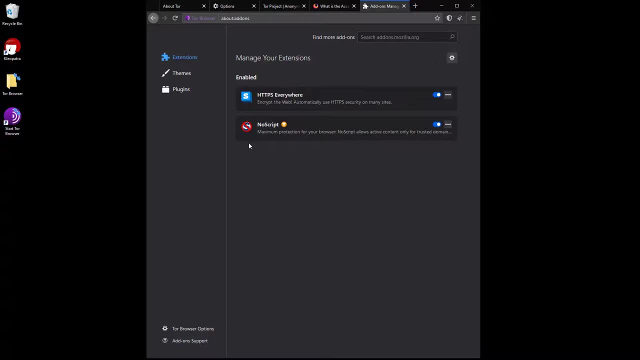 You can also follow the Tor project websites to many such news. For now, adding a new extension is not on the agenda, But this situation may have been changed during the period you follow this course. To stay safe, I recommended you to be a constant user. 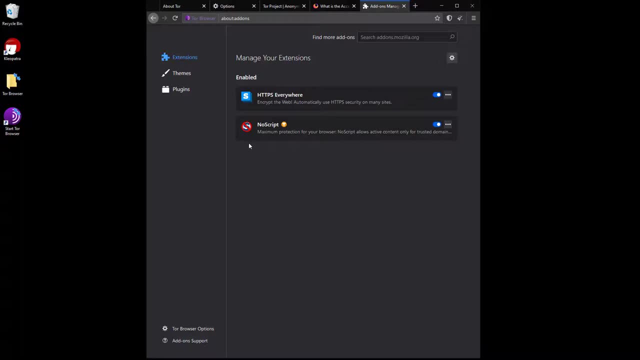 That is the constant question and research. Please note that when it comes to security, you have a very large part of responsibility. Similar to previously clauses, the use of the plugins or language packs should not be used as it may pose a risk to the integrity. 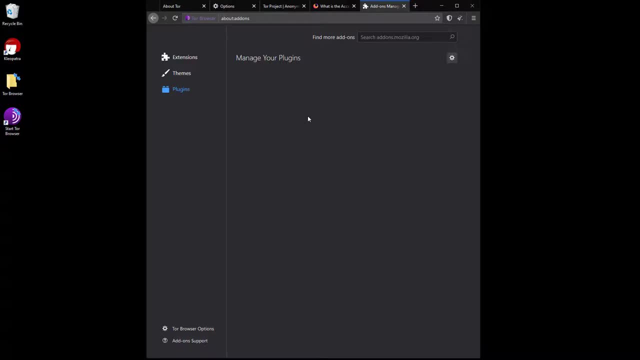 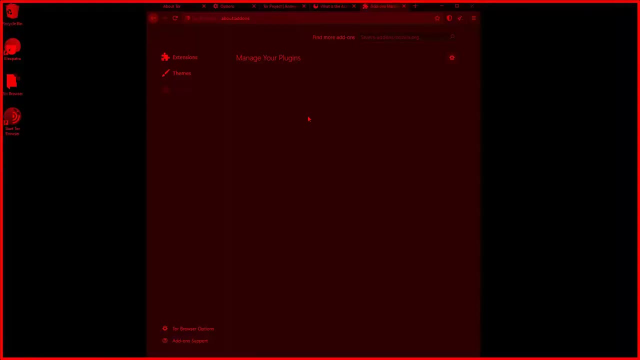 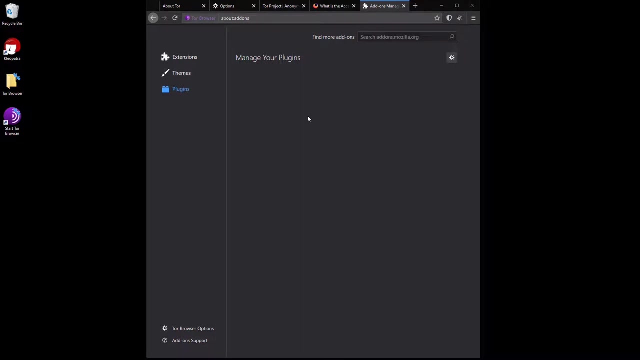 of your privacy. Finally, I don't recommend using Tor browser in full screen mode or maximized mode. If you use full screen, you may leak information about the size of the screen you are using. This seemingly unimportant detail is important and, as a habit, I strongly 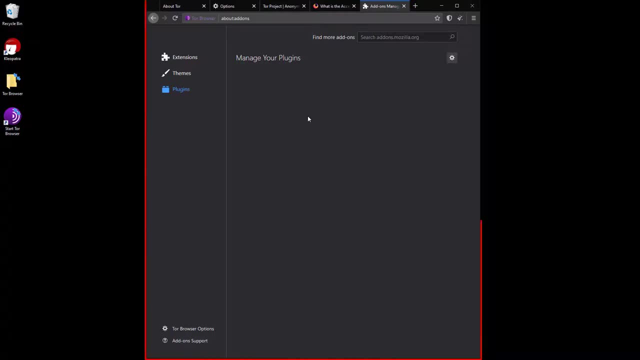 recommend using your browser always with standard windowed size. If all these measures seem too much for you, I would like to point out that security is whole, and the number of details- who should pay attention according to needs of people- must increase at the expense of being 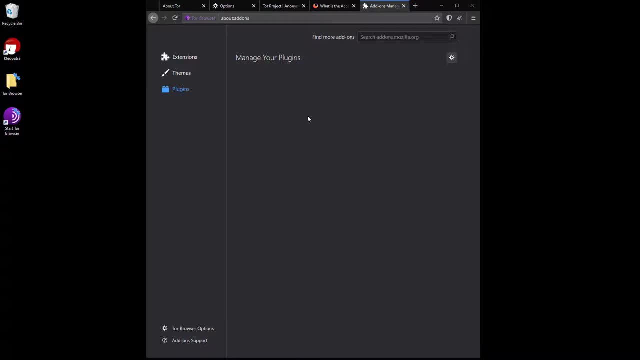 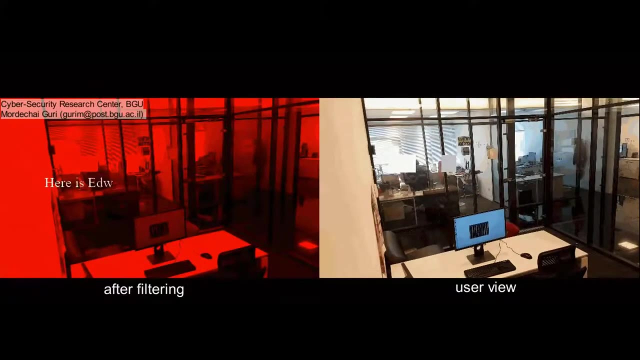 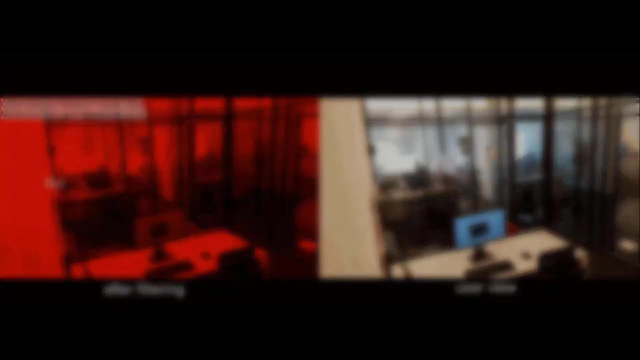 paranoid If I need to give a simple but striking example. for the moment, it's turned out, the data can be stolen from isolated computers without internet connections by changing the screen brightness. So when it comes to security and privacy, it isn't strange to be paranoid. 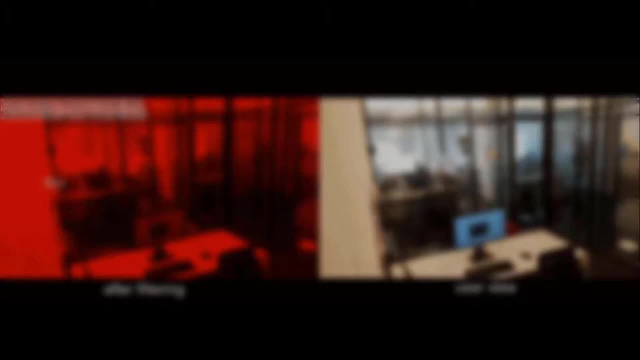 Please keep in mind that security is just a temporary illusion, That illusion. tricks have to be exposed when the day comes. In short, in the real world, security is just a perception. We only think we are safe until it is violated, While the 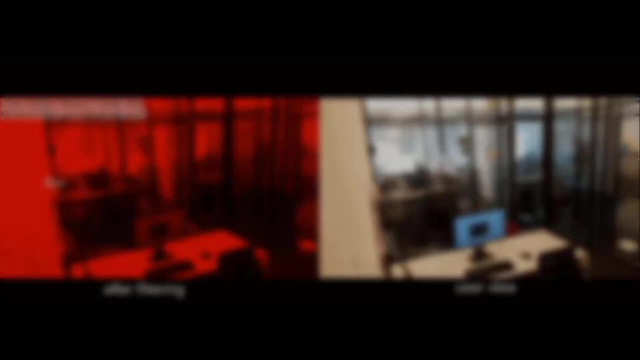 sense of temporary security is good for well-being. in most cases it is the complacency it provides that brings the real security risk. I'm not saying be paranoid, but I always wanted to mention that it will be good habit to research what you can do. 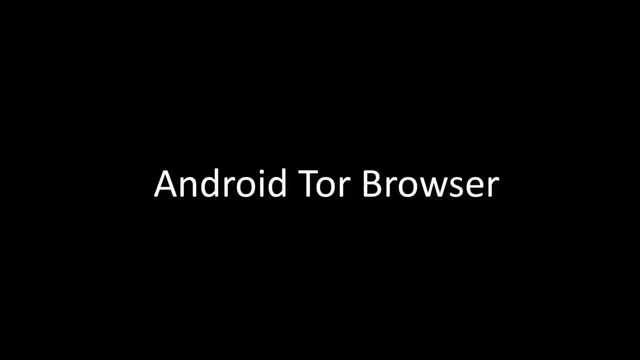 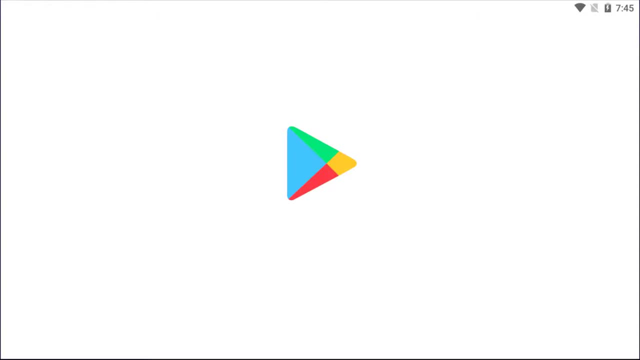 for more security: Android Tor Browser Installation. While you don't have access to your desktop device, you can use the Tor Browser, developed specifically for Android platform, to securely access the Tor network on your Android device. First, let's open Play Store To get the browser simply search. 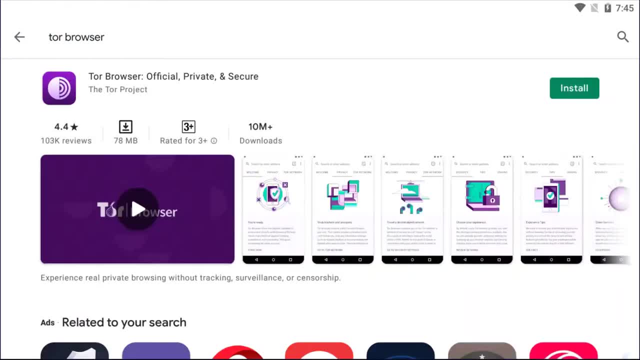 for Tor Browser on the Play Store. Let's install the application published by Tor Developers. Other applications offered by developers other than Tor Developers are not secure, So make sure you download the right application. After the installation completed, let's open the application and click the Connect button. 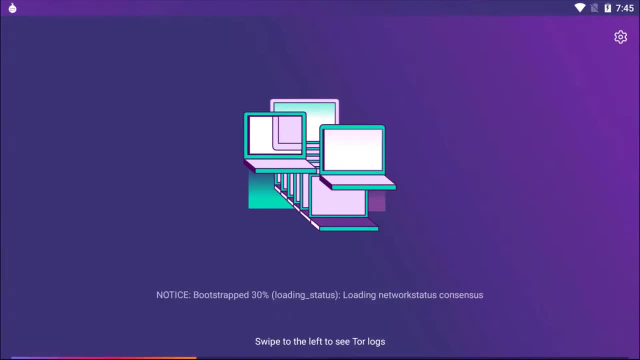 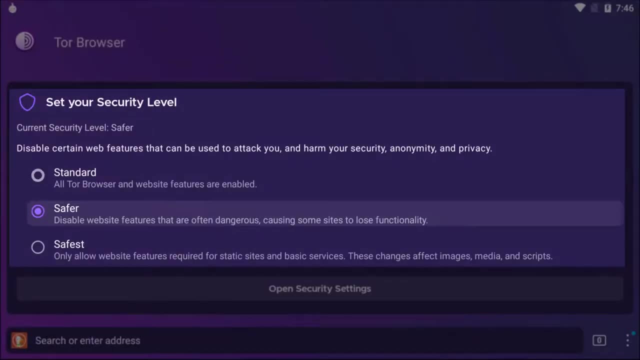 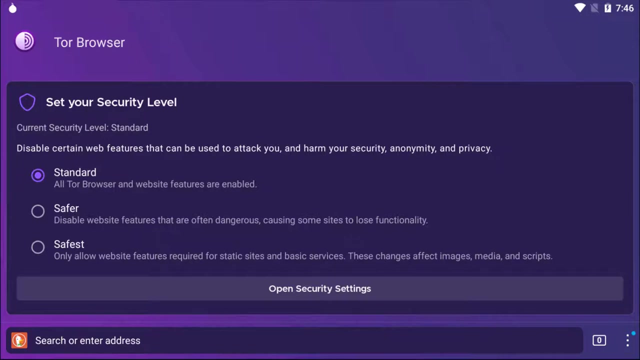 And wait for the browser to connect to the Tor network. You can choose the level of security you want to use the browser from here. Which features are disabled, at what level, is clearly written here. After selection, just type the web addresses you want to go to in the bar. 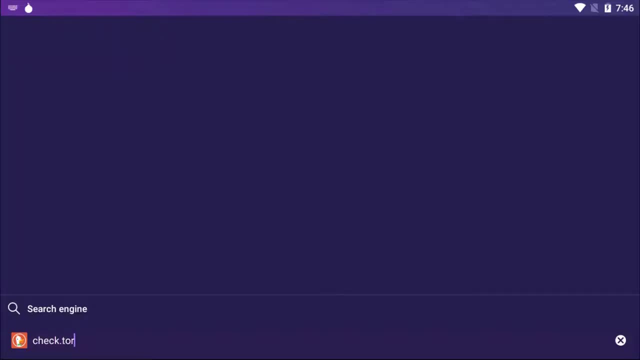 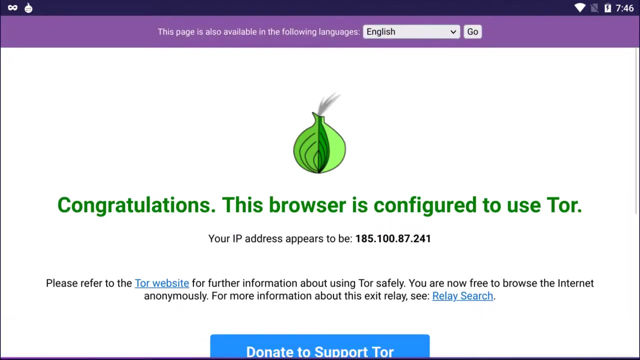 here I visit checktorprojectorg to confirm that I am connected to Tor network. As you can see here, I can confirm here that I am connected to Tor network, So I can use this application to serve the Tor network with my Android device when necessary. 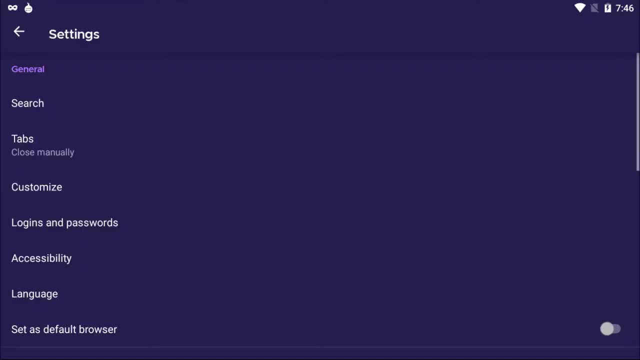 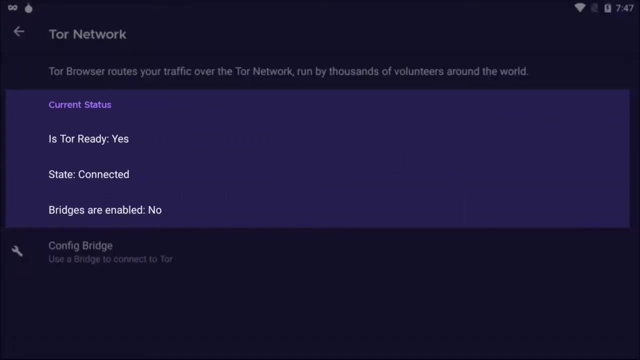 When we look at the settings of the browser, there are settings customized for Tor in addition to settings of standard web browsers. For example, you can change the security level in the security settings. In the Tor network section you can see the connection status. 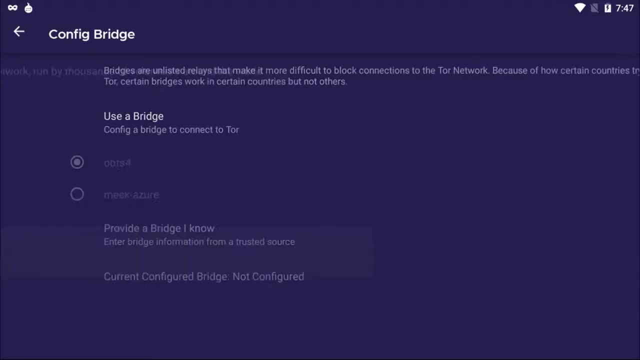 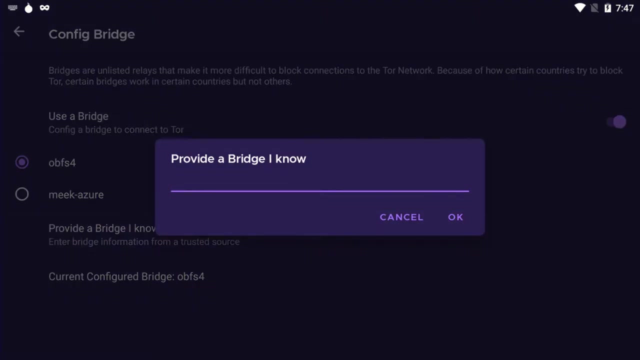 to Tor network and configure a bridge. if you want To use a bridge, simply enable to use a bridge feature. This will automatically provide a bridge connection. Also, if you wish, you can manually enter bridge information from the provide a bridge, I know- section. 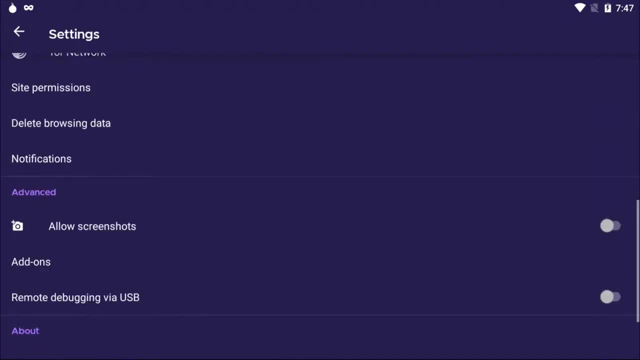 The other settings here are standard settings that you already know. We already talked about all these settings when describing the Tor browser desktop version. The settings we mentioned are exactly the same for this browser, So you can change these settings if you need. About iOS Tor browser. 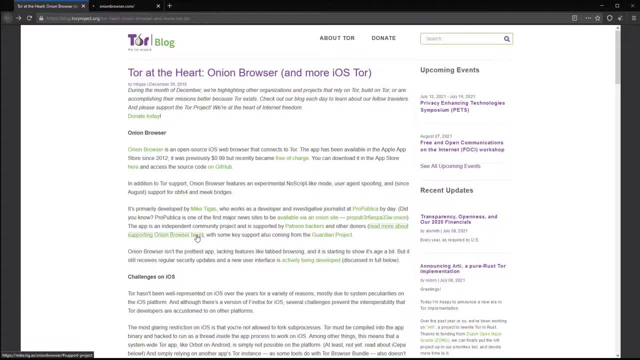 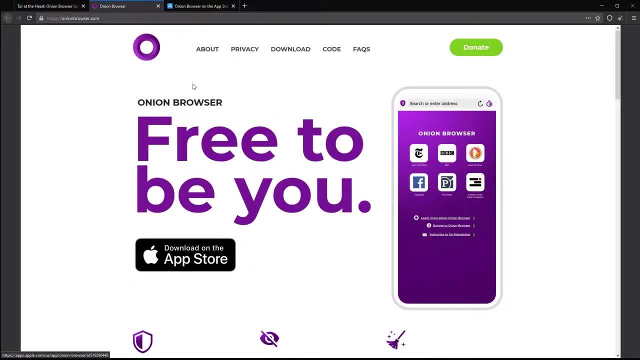 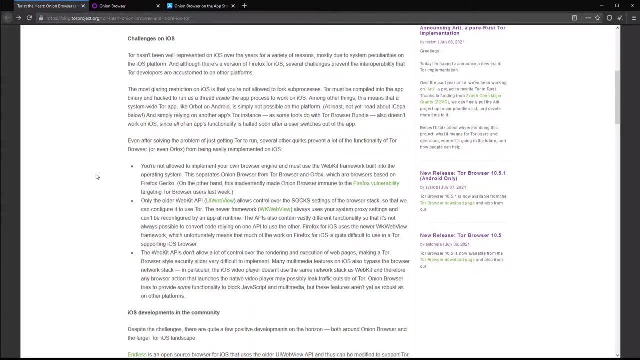 Tor developers recommended an iOS application called Onion Browser, which is open-source, uses Tor routing and is developed by someone who works closely with the Tor project. However, Apple requires browser on iOS to use something called WebKit, which prevents Onion Browser from having the same privacy. 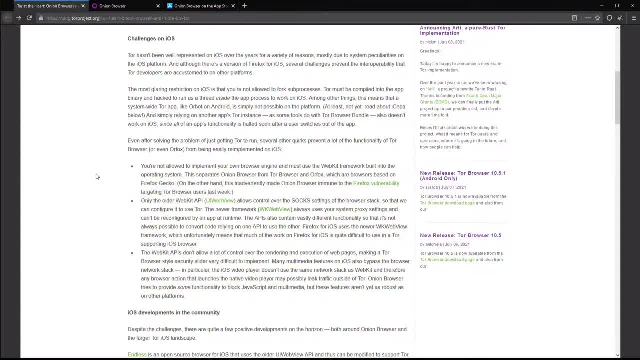 protections as the Tor browser. You can check out the link in this lecture resource to learn more detail. So I don't recommend using it unless it is not have to, as I don't think it's safe. Also, I won't discuss 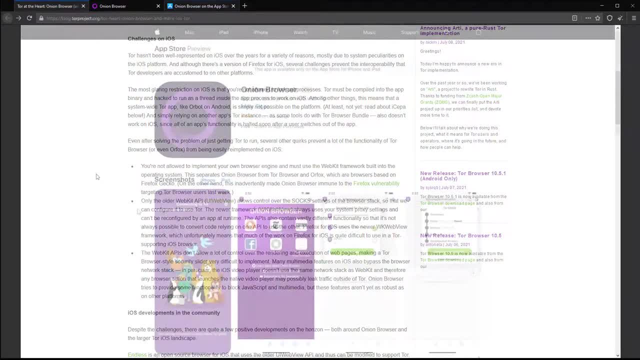 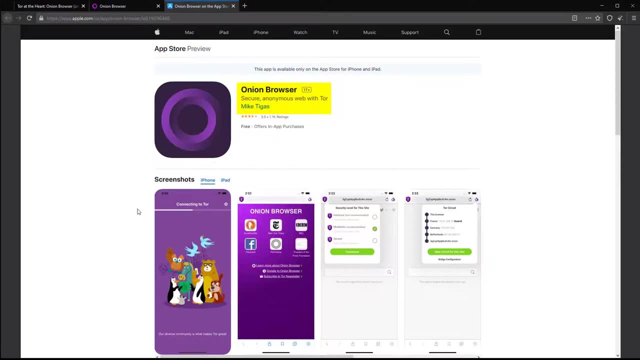 alternative applications and their uses in this lecture Only if you really need it. you can find this Onion Browser, developed by Mike Tigas, by searching through the App Store, but is unreliable about security and privacy If developers of the Tor project release a stable iOS application. 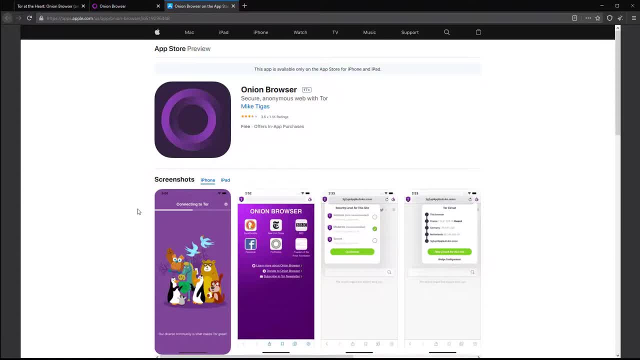 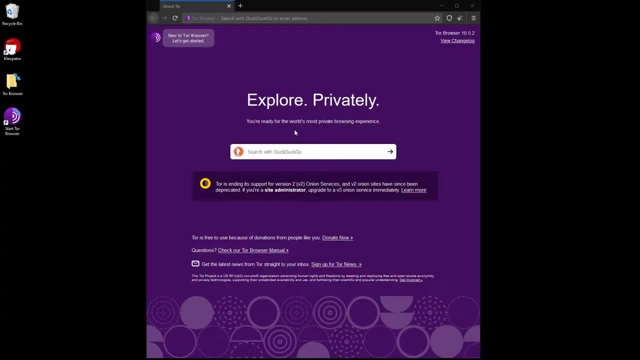 I will have included in this section already Summary. We saw all these settings that concern us on Tor browser and talk about all this configuration required for our security At this point. you might be thinking he is told all this but still hasn't touched on. 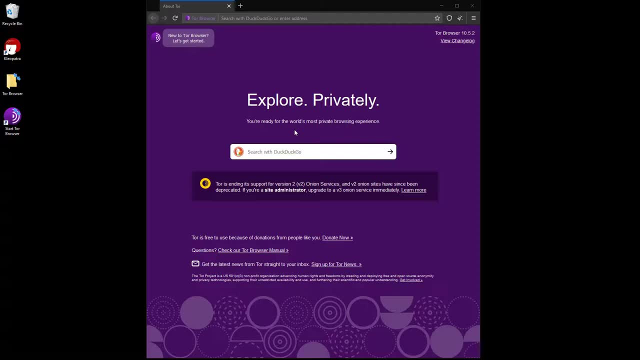 how to serve the Tor hidden services, in other words, dark websites. If so, I would like to clarify again briefly the situation we have explained before and clearly all possible confusions. In this section, you learned how to connect to the Tor network through the Tor browser and how. 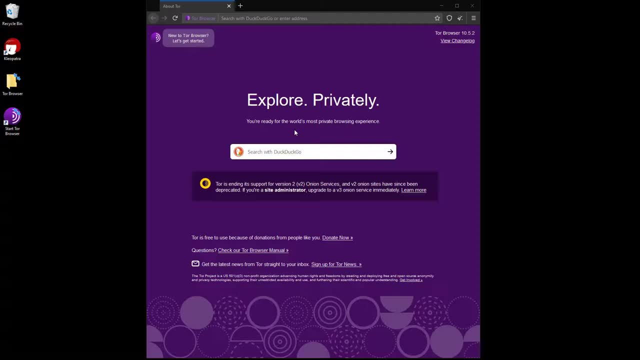 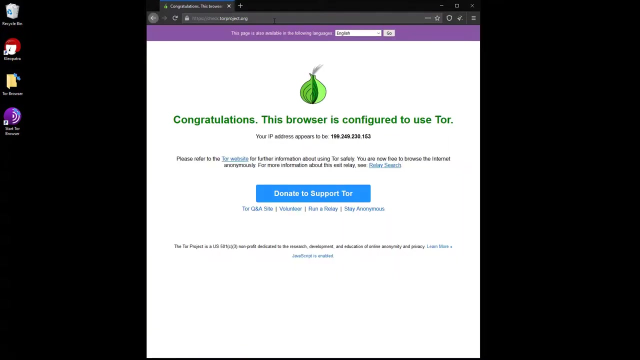 the browser security settings should be when using the Tor browser. So you have seen how you can serve anonymously on Surface Web over the Tor browser. As a matter of fact, the checktorprojectorg address you visit is a standard website in the area. 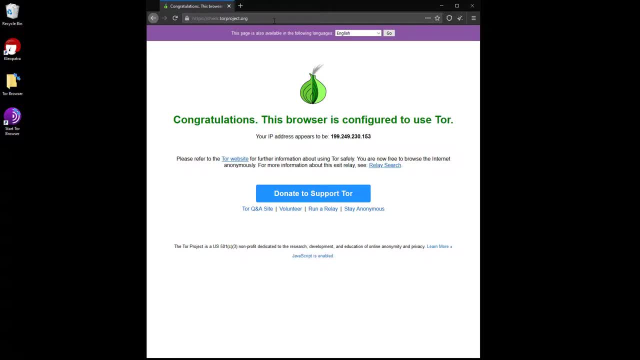 we call Surface Web. In other words, with the information you have learned so far, you can serve the Surface Web more securely and anonymously than ever before by overcoming all obstacles via Tor browser. Apart from that, if you are wondering how you can access onion hidden services, 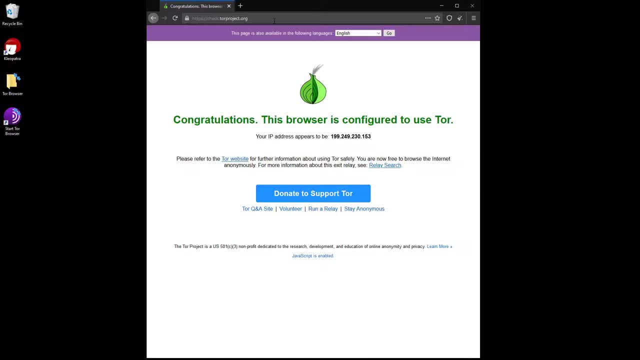 namely dark websites on the Tor. we will discuss this issue in detail in the future. For now, you have just to be a little more patient and continue the study by adhering to course curriculum, being aware that all course content is interconnected. At the end of course, you will realize. 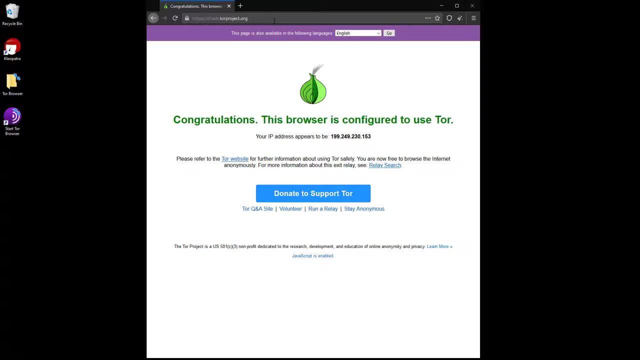 yourself that all course curriculum are prepared in a way that will make it easier for to learn by progressing in conjunction with each other. In the next section we will continue explanation with Tail Operating System, which is considered to be much safer than using only the Tor browser. 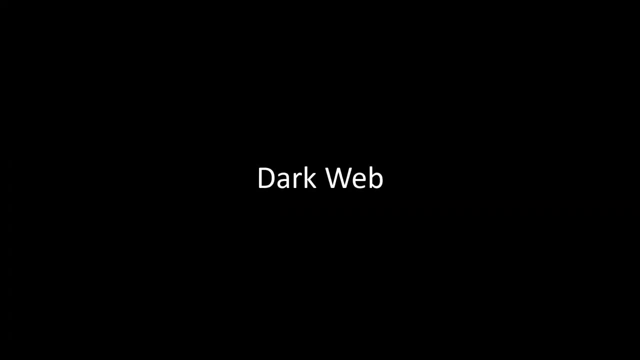 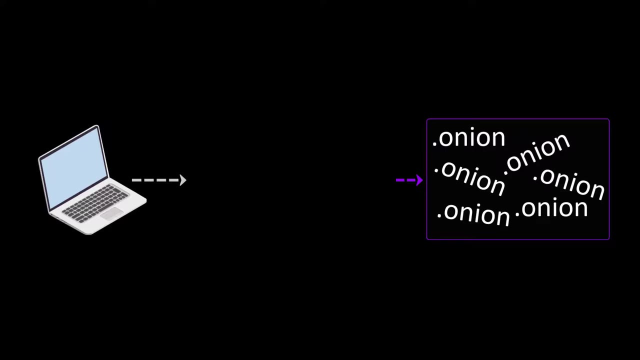 Tor Hidden Services- Dark Web. At the beginning of the course we mentioned that there are Tor Hidden Services that can only be accessed over the Tor network, And the web states where these services are located is called Dark Web. In this section, we will be discussing how to. 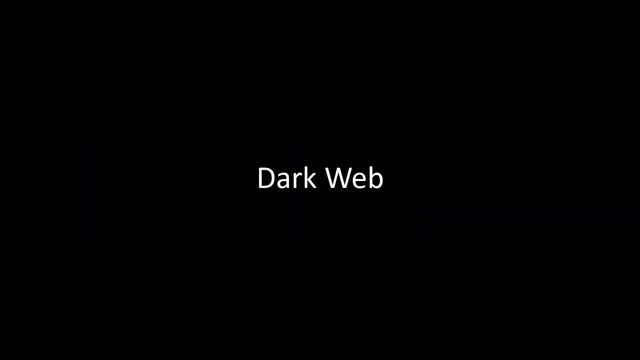 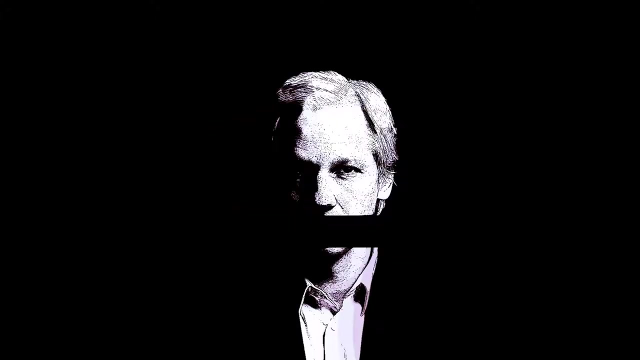 access websites on the Dark Web. If you have prejudice of these services because of the Dark Web name, investigating the reason Tor Hidden Services born may change your mind. The main purpose of the Tor organization from the very beginning to ensure that people can use their right to communicate. 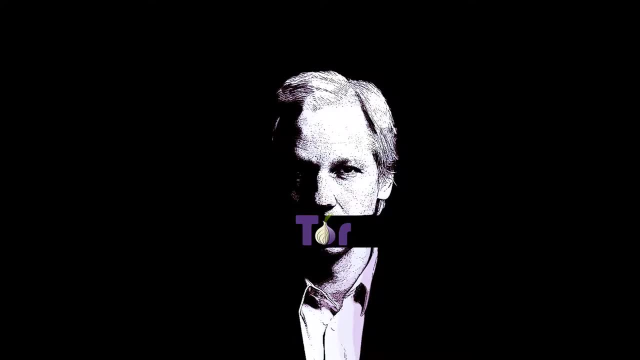 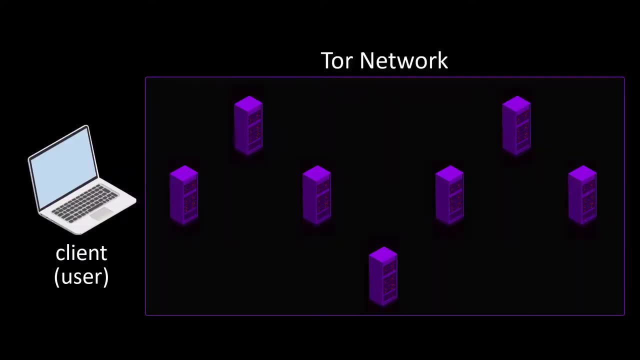 and receive information against all forms, operations and censorship restricting freedom. Therefore, realizing that it won't be enough to provide security and freedom on the user side, Tor Hidden Services have been started to provide a secure publishing environment for publishers. Tor Hidden Services work within. 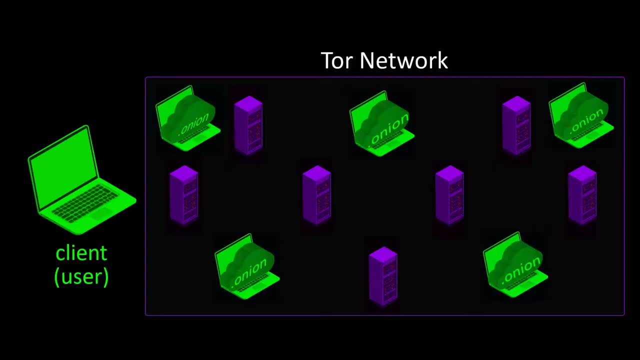 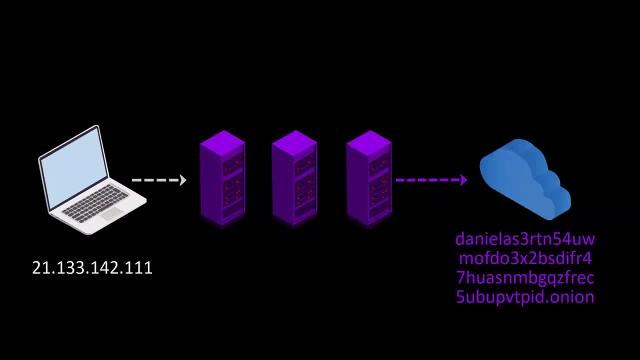 the Tor network and allow you to register an internal Tor-only servers that gets its own onion hostnet. When visiting connect to the Tor network, Tor resolves those onion addresses and directs you to anonymous servers sitting behind that name, Unlike with other services, though. 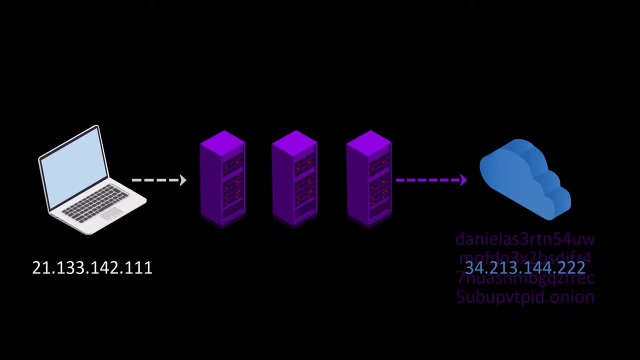 Hidden Services provide two-way anonymity. The server doesn't know the IP of the client, like with any servers you access over Tor, But the client also doesn't know the IP of the server. This provides the ultimate in privacy, since it's being protected on both sides. 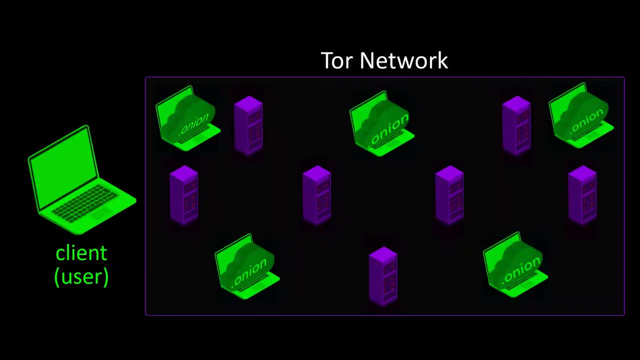 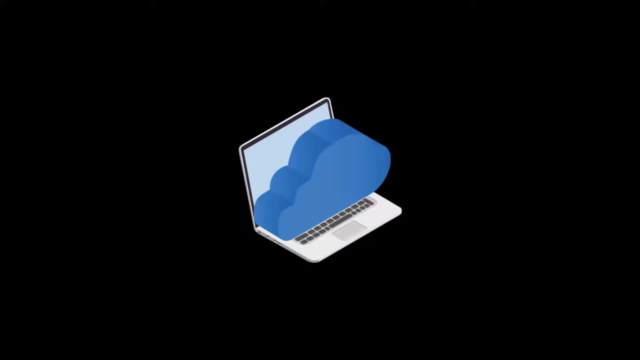 Thus, a free and highly secure publishing ecosystem has emerged for all publishers with restricted freedom, such as journalists under pressure. When publishers want to publish via Tor Hidden Services, in other words the onion service, they can publish the content they want anonymously, without being dependent on any company. 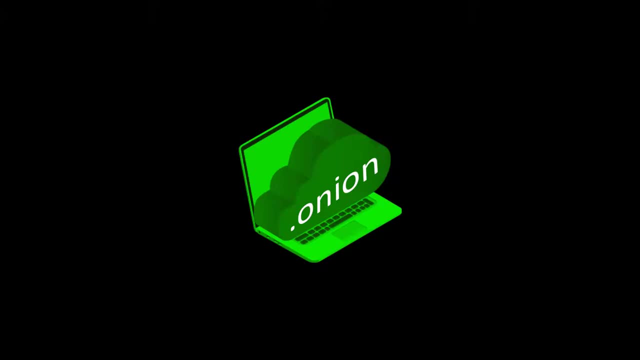 for things such as domain name registration. Normally, when registering a domain name, the credentials required for registration must be shared with the registrator and a fee must be paid for registration. In order to register a domain name with the onion service, there is no need to provide. 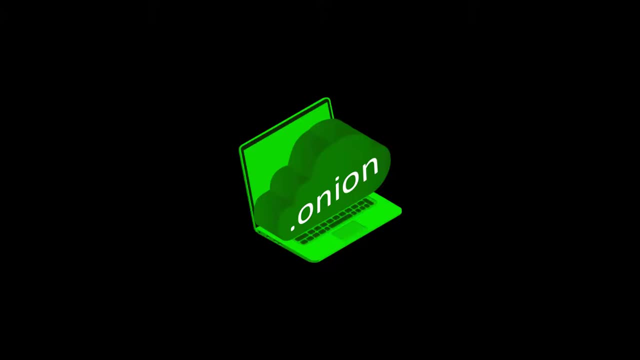 identification information or pay any fees. In this way, it provides free and anonymous publishing that can be accessed by anyone. You can even use your computer to host your website files. In this way, you can freely publishing over the Tor network without having to share information. 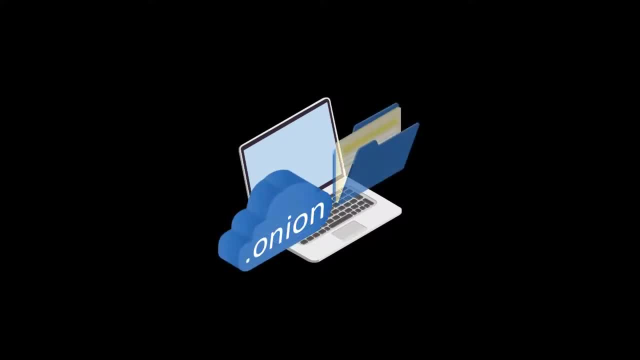 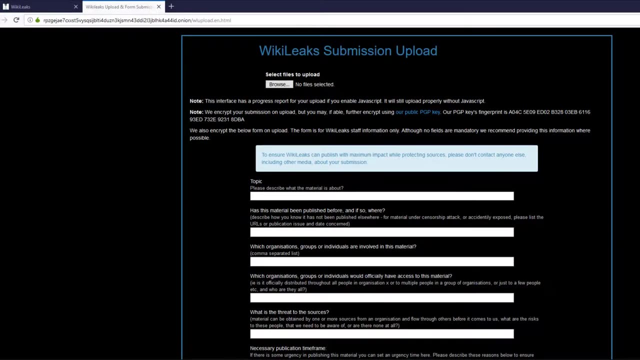 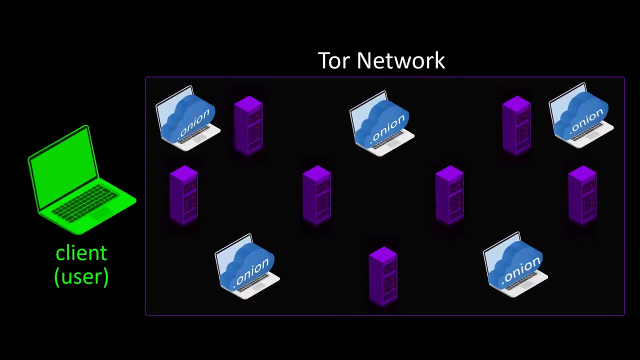 with anyone, both domain name or host service. As the clearest example of the freely publishing I can give example: the Wikileaks documents moved over the Darknet As the websites established with the Tor Hidden Services are located on the Tor network named on. 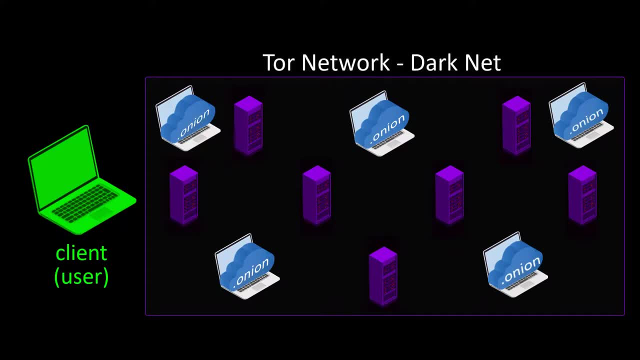 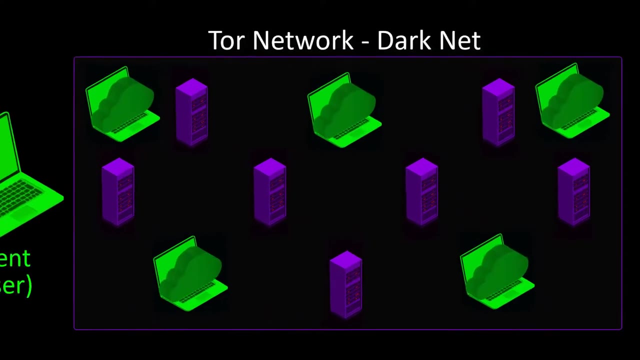 the Darknet, your real IP address as a publisher is also hidden. In addition, since you don't register domain names with your credential, no mechanism that wants to prevent your information sharing activities can directly interfere with you. By looking at the previous explanations, 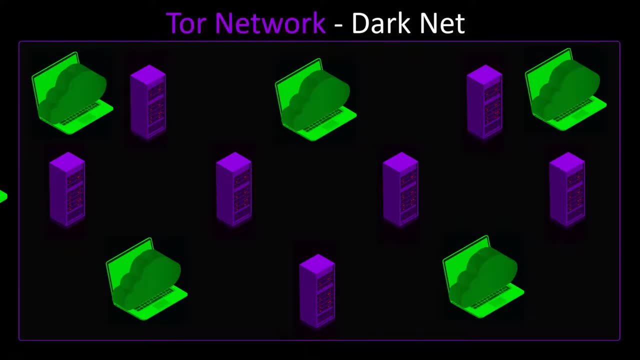 you may have been noticed that the Tor network can also be called Darknet. This is due to the notoriety of the Tor project, which we mentioned earlier. In other words, by using the expressions Dark instead of Tor, the phrase Darknet can be used. 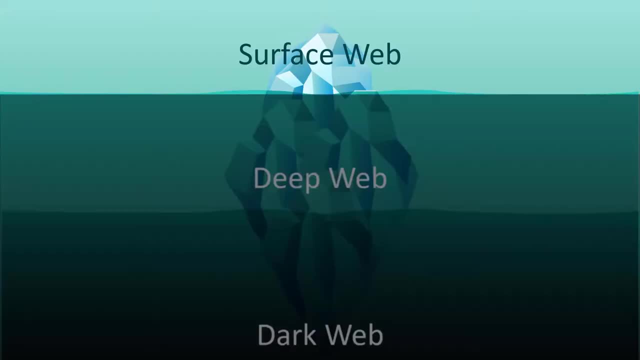 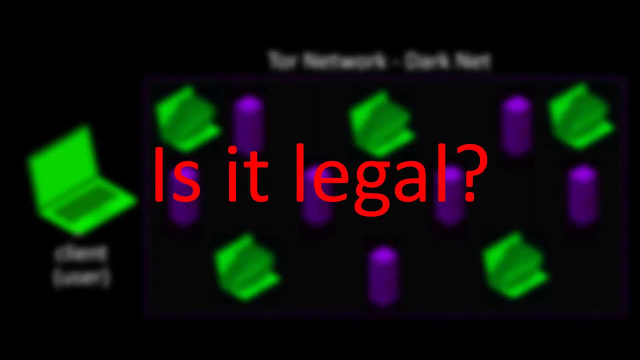 instead of Tor network. Similarly, the web space that you can reach with standard browsers without connecting to the Tor network can be called Clearnet. that is, open, clear network. If, at this point, you have a question about whether it is illegal to browse and publishing, 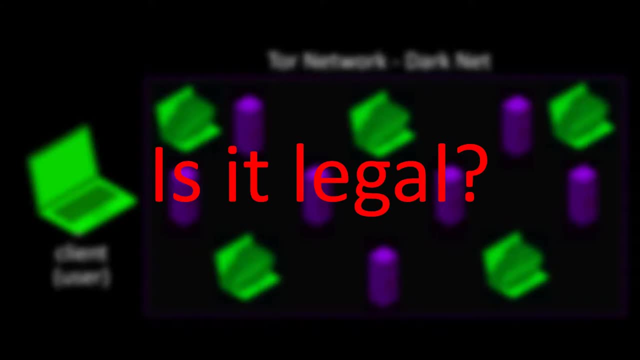 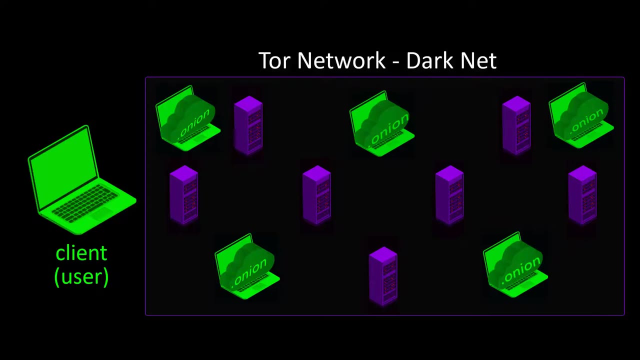 on Onion services, that is, Dark websites, my answer will be the same as using the Tor network. In other words, whether the use is legal or illegal is completely determined by the activities of the people. While legitimate content is not a problem, access to and publish of 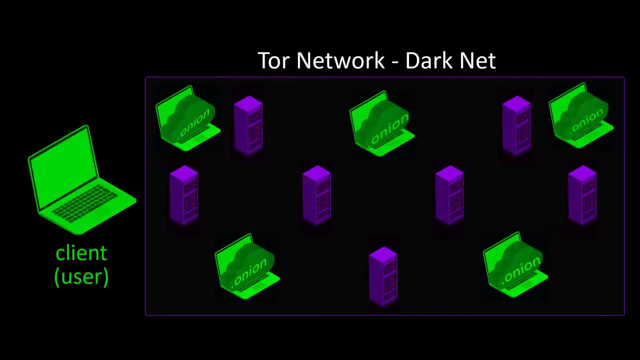 illegal content is criminalized. Although the anonymity of both sides allows people to circumvent the law temporarily, I would like to remind you once again that these security measures don't provide 100% security. There is a possibility that your real identity will be revealed. 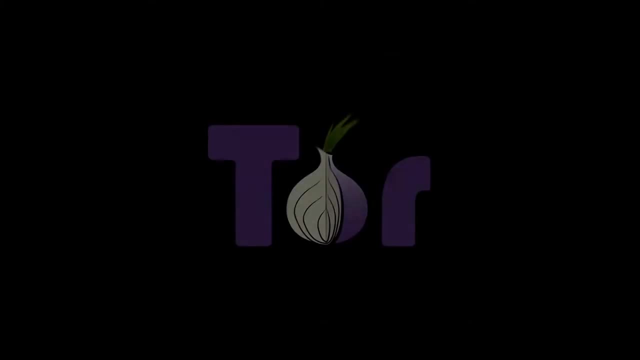 when the necessary resources are allocated. However, as long as your activities use Tor or for your own personal information security, you will have no problems, Be aware that the concept called freedom is a concept that can be valid as long as it doesn't restrict the freedom. 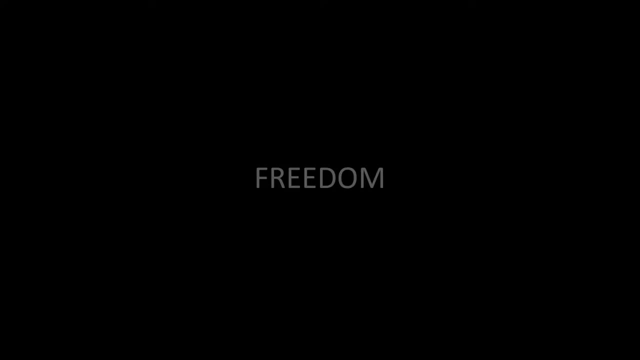 of other people and risk lives. Otherwise, all the anonymity measures you take will only keep you anonymous for a certain period of time. As the clearest example of this, I can give the quote of the founder of Silk Road, which has been publishing on the dark web for. 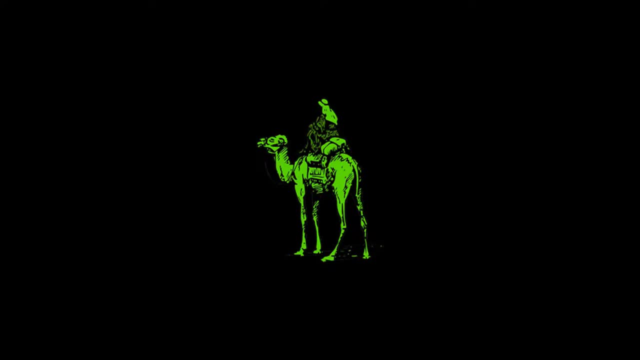 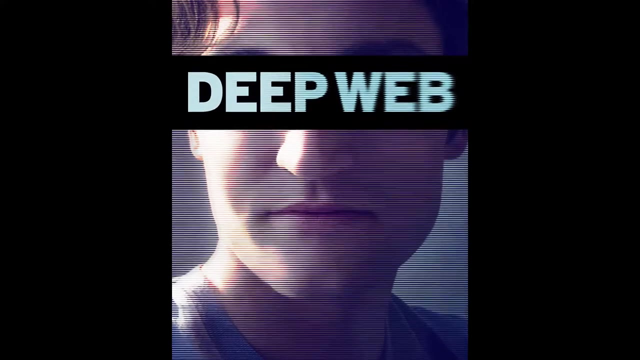 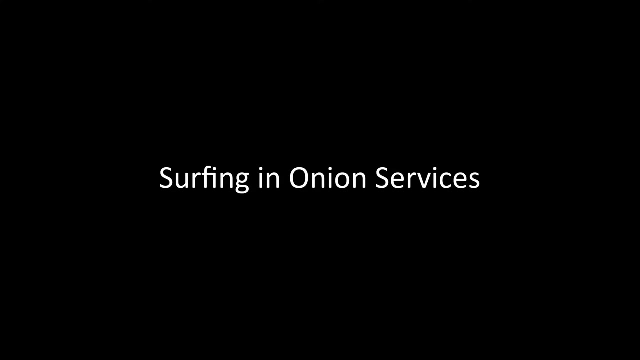 many years and is the biggest illegal trade site of its time as a result of meticulous work. If you haven't watched it before, I strongly recommend to you watch the documentary Deep Web in order to learn more about this subject and gain awareness. Surfing in Onion. 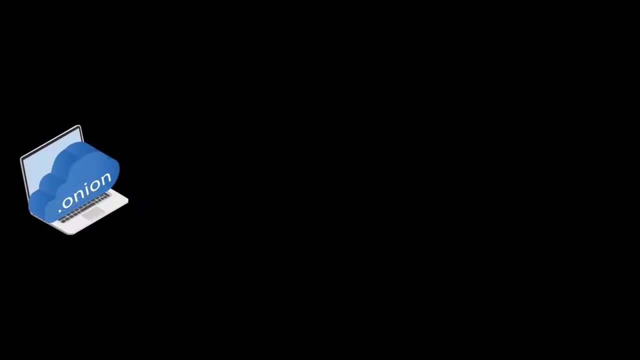 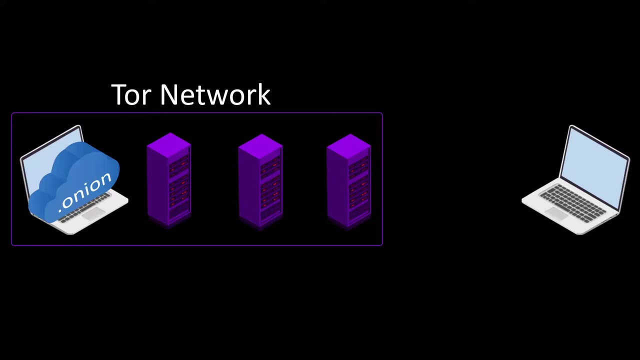 Services. Since websites publishing on the Onion servers are located on the Tor network, you can only access such websites through tools such as Tor browser that can access the Tor network. In other words, it is not possible to access the web area called dark web with ordinary browser that. 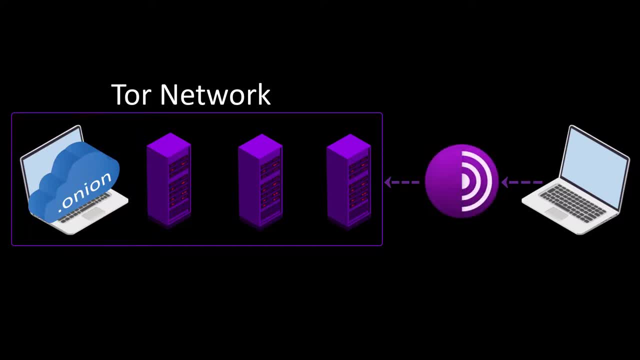 do not use Tor network. Once you are sure you have access to the Tor network, all you have to do is use the domain names of the website you want to go to. However, the domain names of websites in hidden services are often very difficult. 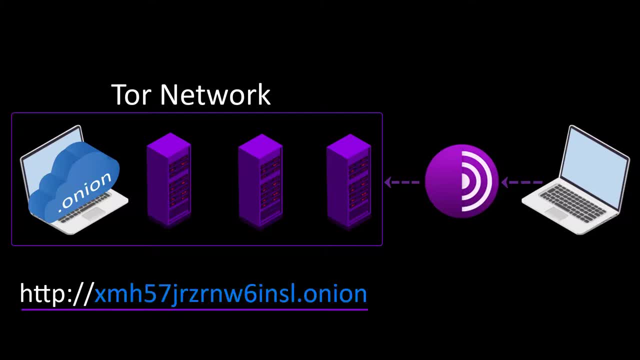 to keep in mind, as they don't contain meaningful words As such, you usually need to learn addresses of websites you want to go to using darknet search engines or lists shared by other peoples. Now let's talk about both: darknet search engines and shared. 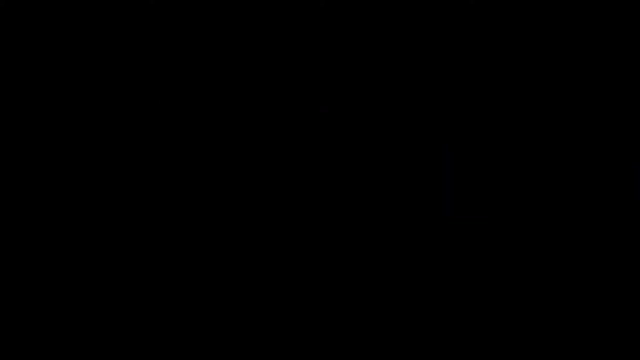 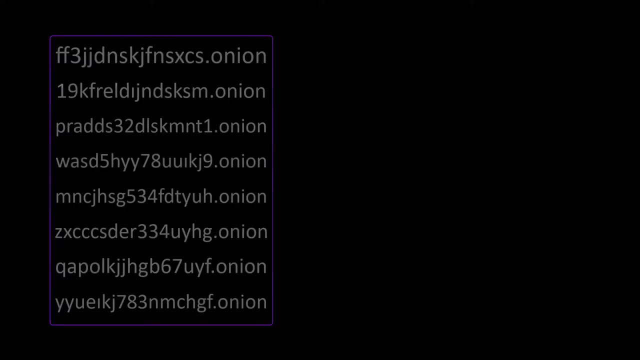 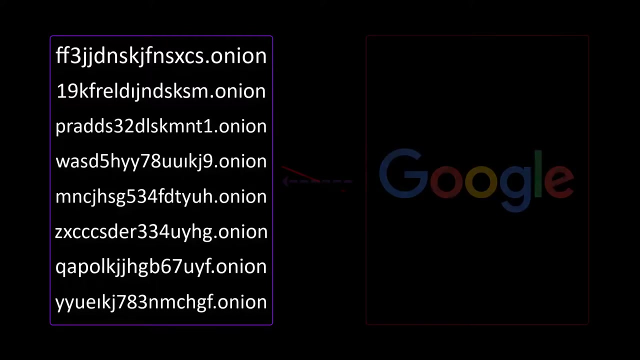 lists respectively: Using darknet search engine. You can't access the link addresses of websites on darknet with search engines working for surfing. You can't access the link addresses of websites on darknet with Google, Bing or Yandex, Although not working as efficiently. 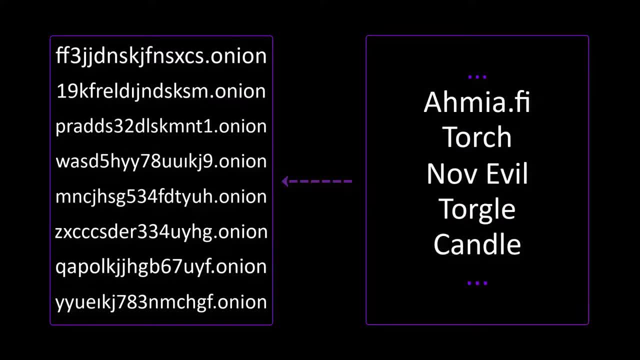 as Bing, Google or Yandex. there are also darknet specific search engines that can search on the darknet and provide you with consistent results. However, it is worth mentioning that these search engines aren't as effective as the search engines you are used to. 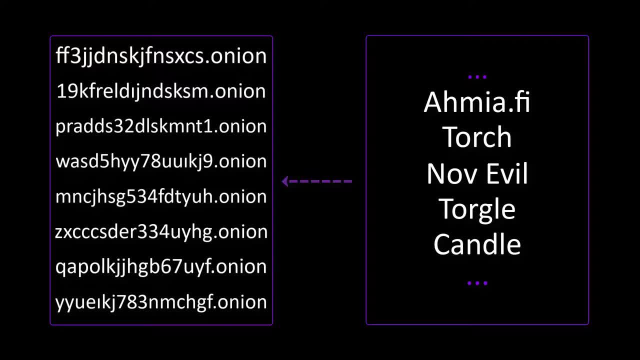 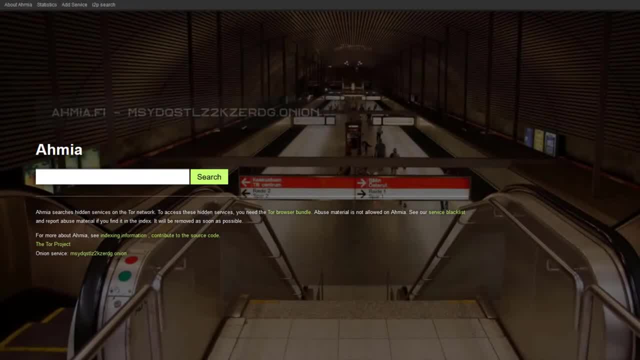 In other words, it would be better to see darknet search engines, as you can get help without keeping your expectation hikes. Thanks to this search engine, we can search the websites on darknet via clearnet. The biggest advantage of this search engine is that has a easy to remember. 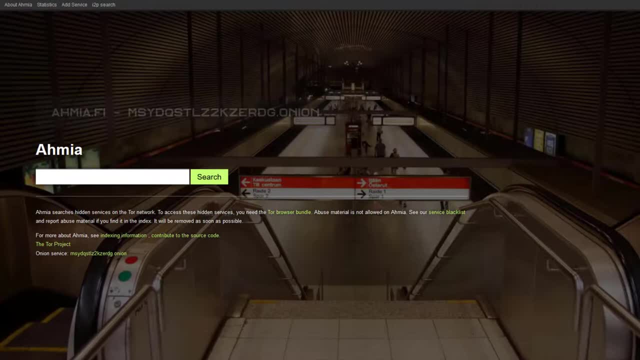 domain name that also publish on clearnet. For example, when you don't have an address of any website, you can easily find the address information of many websites on the darknet through this web address, Even if you are not that satisfied with the result of this. 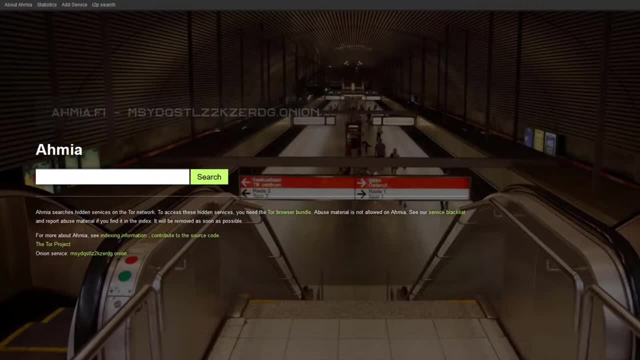 search engine. you can use this tool to find addresses of any other darknet search engine that you find useful. In short, you can use the Amiafee search engine as an easy to remember and easy to access gateway to start searching on the darknet. 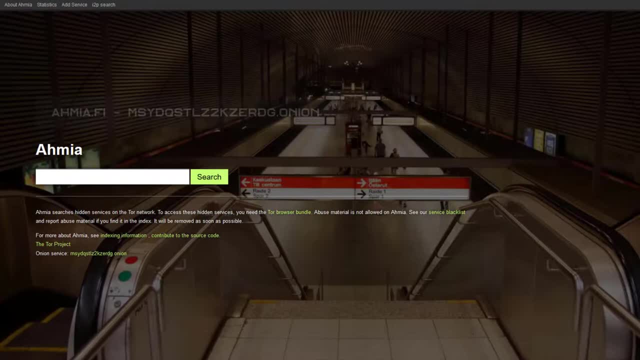 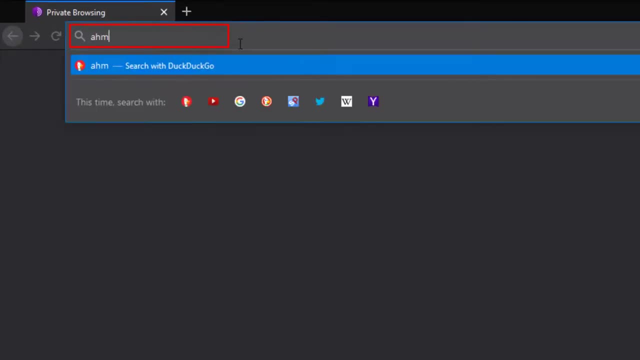 Let's go to the addresses on clearnet to give an example of its usage. I go to its addresses on clearnet because it is easy to remember. I type Amiafee in my browser address bar and confirm it. As you can see, we have come. 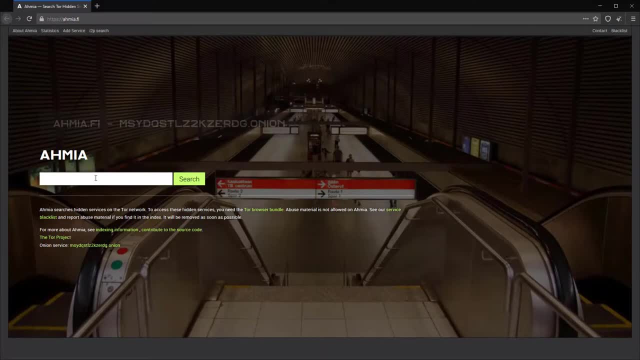 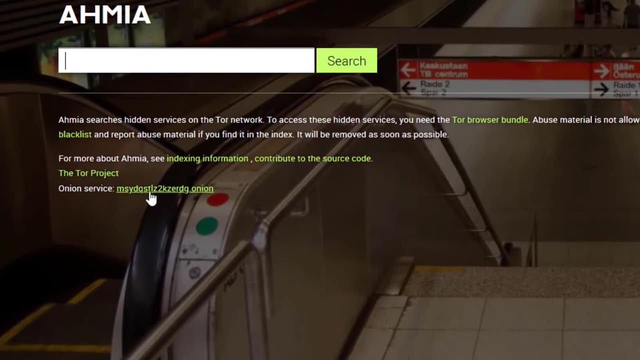 across a very simple web page. Just enter the keywords of the website you want to find in the search bar and search. In addition, as you can see at the bottom, there is the onion service address of the search engine on the darknet and you can use this address if. 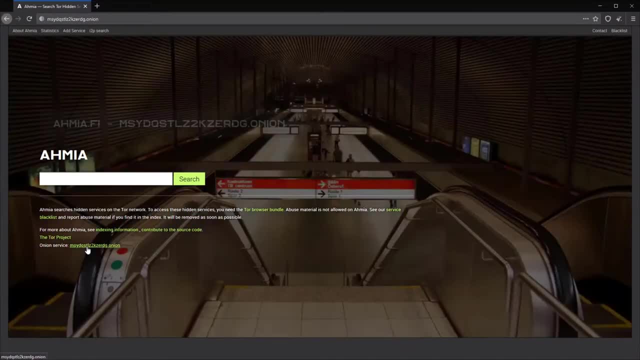 you wish. As I said before, I first visited its addresses on clearnet, just because it is easy to remember. Now, to try it, let's search by typing the name of another search engine Torch in the search bar. As a result of my search, many 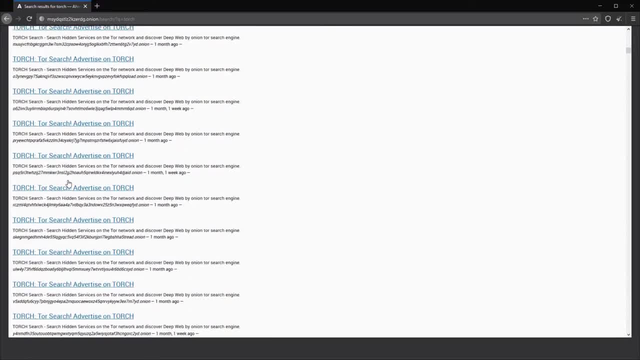 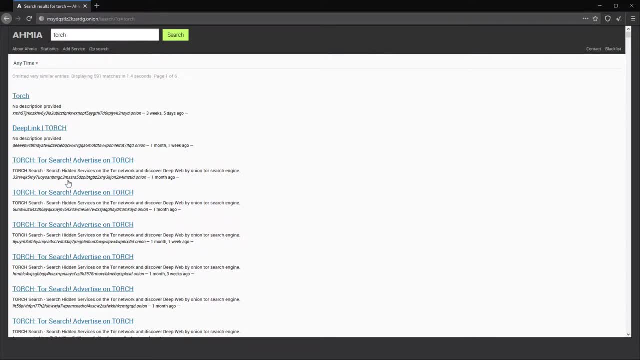 links with the same name but different addresses have been listed. Unfortunately, there is no sure way of knowing which are these are real and which are fake. All users can report the malicious addresses if they are want. If the number of report is high, the address is. 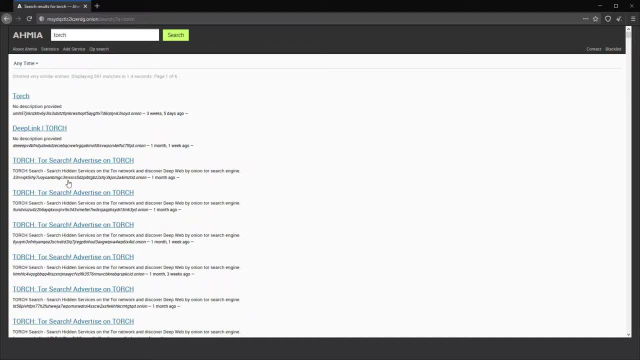 removed from the list. However, don't rely too much on this feature, as the abuse reporting system works quite ineffective. To visit real addresses, you need to keep your own address list. This way, you will have a safe list of addresses over time. 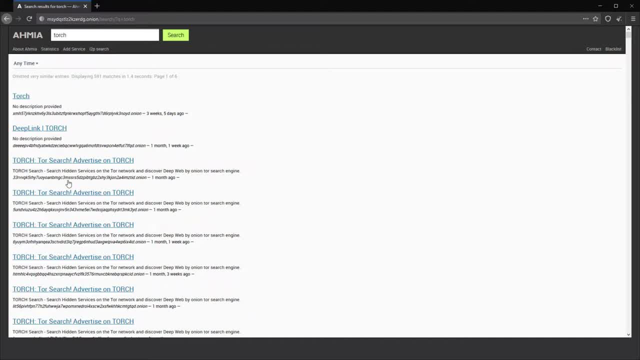 You can use search engines for new discoveries. When you discover a new secure address, simply add it to your own address list. Since I already know the address, I click the relevant link when I see the address. Frankly, I don't find other search engines. 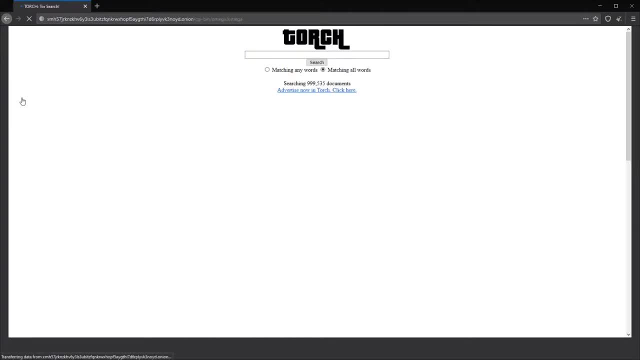 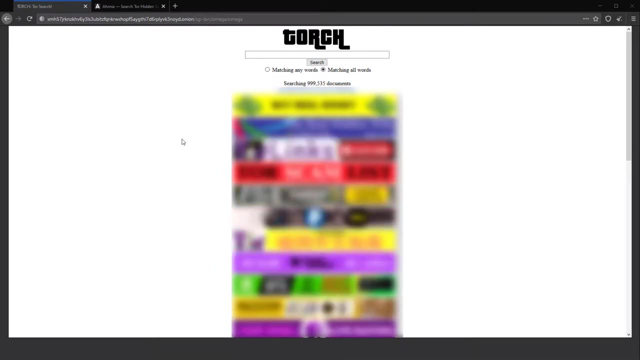 very useful compared to a MiFi search engine. However, you can still experience various search engines and decide which one works better for you. For example, let's try the Torch search engine. Torch, It is a search engine that has been active for a long. 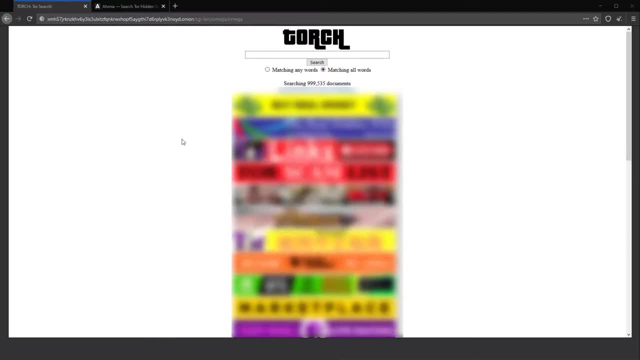 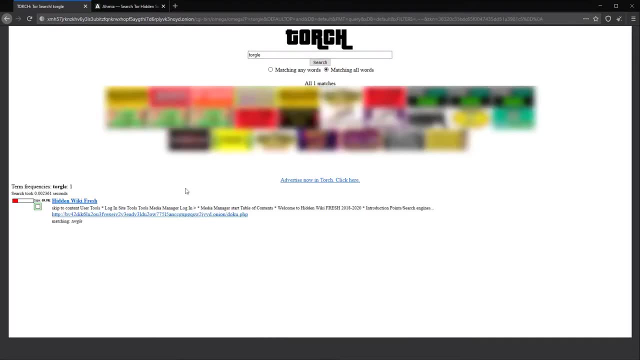 time, and it claims to have researched over about 1 million documents To test this engine. let's search another search engine, Torgl. this time, As you can see, I couldn't reach the result I want to search for, which didn't surprise me. 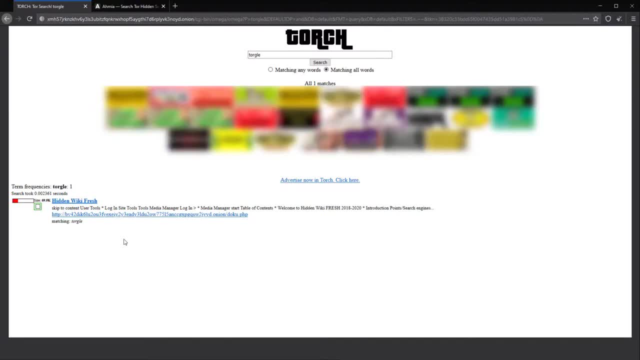 at all because in my personal opinion, Torch can use the excess number of addresses it has correctly. It is not very good at indexing addresses correctly and it also contains a lot of advertisements. Although it is not my favorite, it is wide addresses potential causes it to be preferred by. 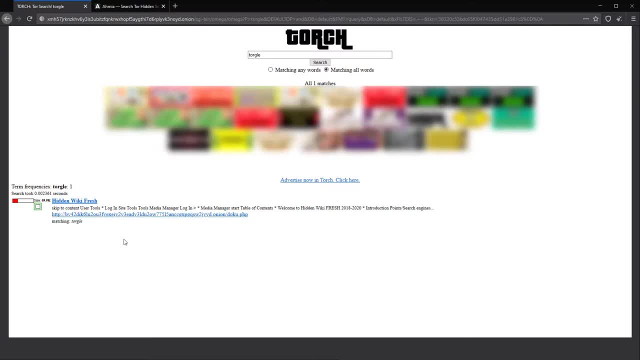 many users. People often use the Torch search engine to discover new addresses rather than popular websites. I wanted you to know because it is frequently used search engine. Although it is not my favorite search engine, you should definitely experience a little bit and make your own. 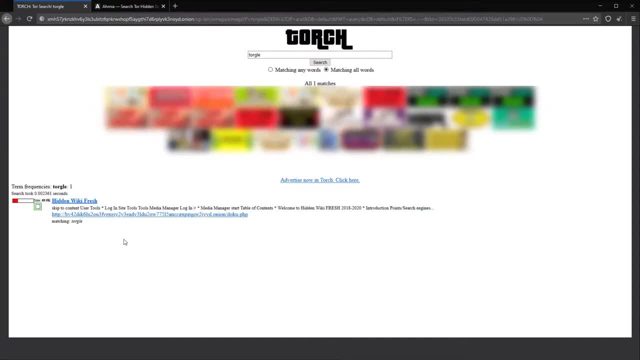 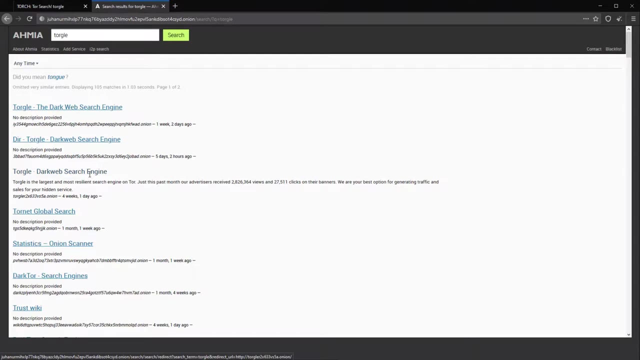 decision. I am not saying that it is absolutely useless. I just wanted to point out that it gives an efficient result for me, according to my personal experience. Now let's do the same. search again over AMF. As you can see, many addresses have. 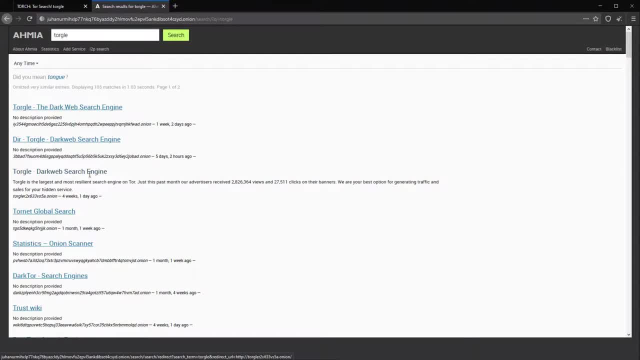 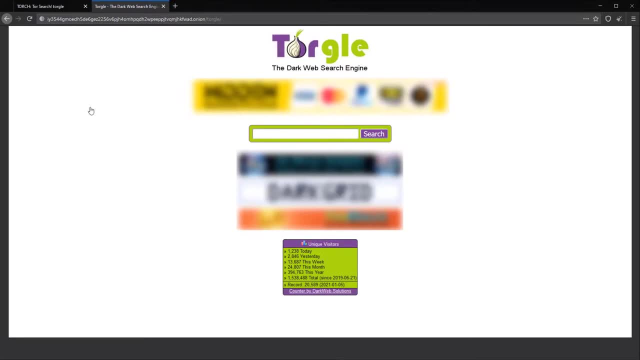 been listed. That's why the AMF search engine is my favorite search engine. I click this because I know this is the correct address, Torgl. Unlike the others, this search engine also displays the page content of the website in the listing stage. In this way, we 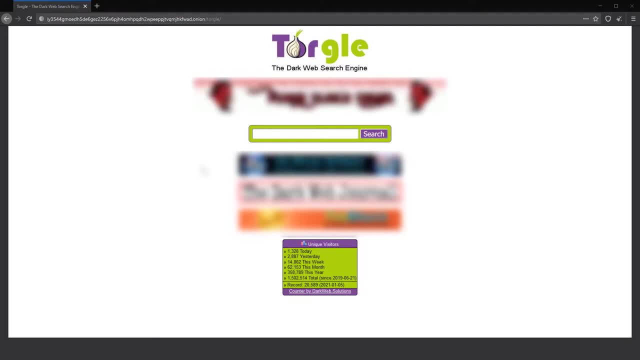 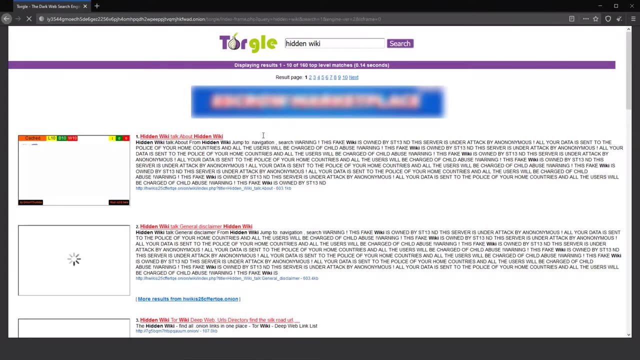 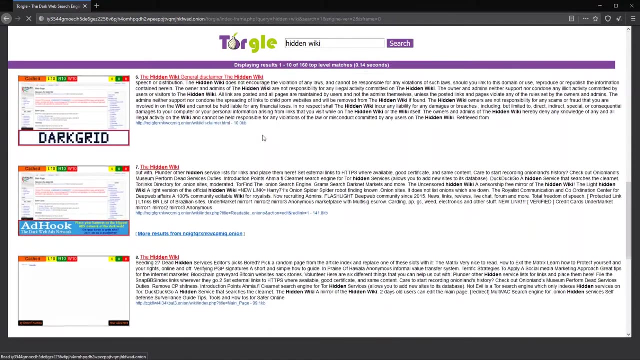 can avoid unwanted website visits to some extent. Let's search HiddenWiki to trade out. HiddenWiki is a useful web address that keeps a listing list of onion addresses. Later we will also be talking about the HiddenWiki. The results have been listed, together with the images. 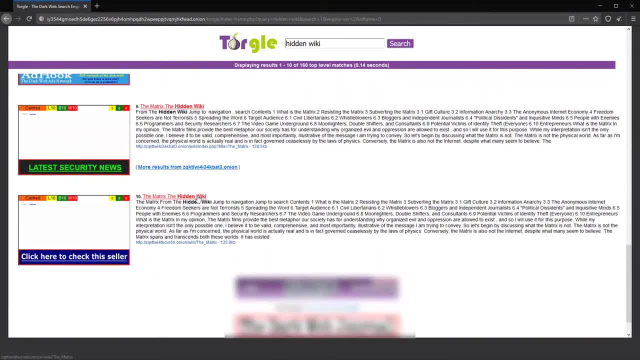 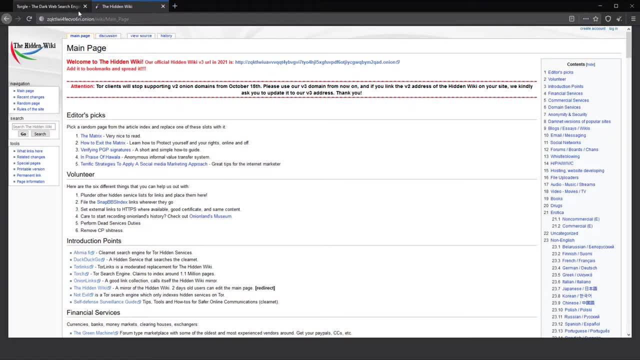 of the websites. I go to the link I am looking for from the list with the help of screenshots. You can use this engine for links and new discoveries that you are often not sure about. Nevertheless, it is an engine that I prefer very often as it contains: 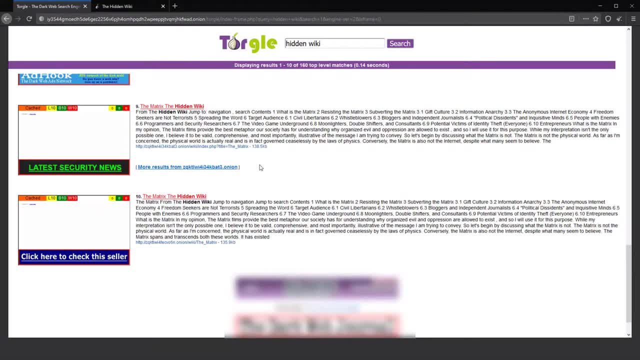 too many ads and doesn't give results with high constancy. We have dealt with a few basic and most frequently used search engines with their general use. The websites here may be shut down over time or replaced by different search engines, But don't worry this situation. 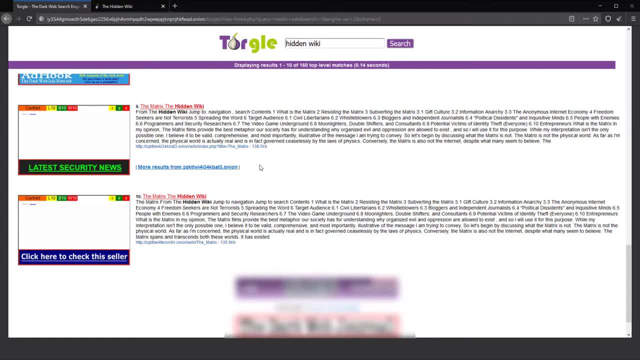 won't be a problem for us, Because in this section we will see how you can access addresses on the dark web without search engines. So, when necessary, you will be able to obtain the information of new search engines through alternatives. In addition, there are many dark 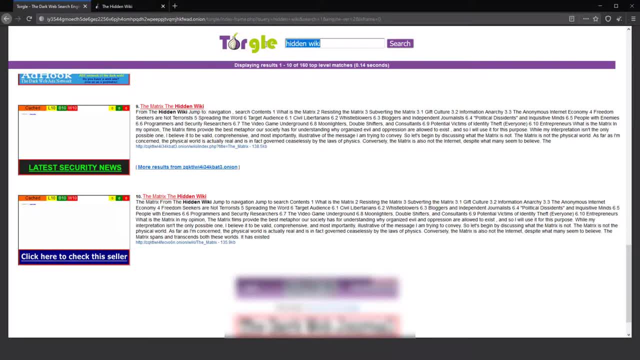 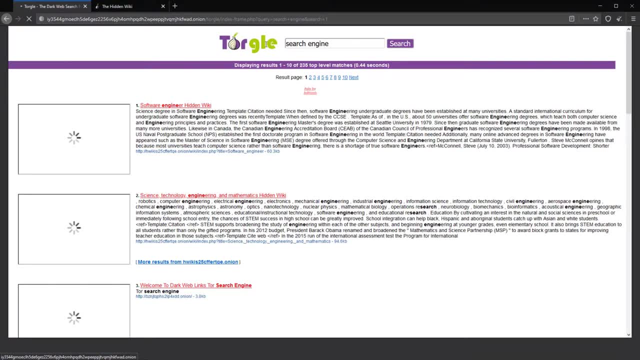 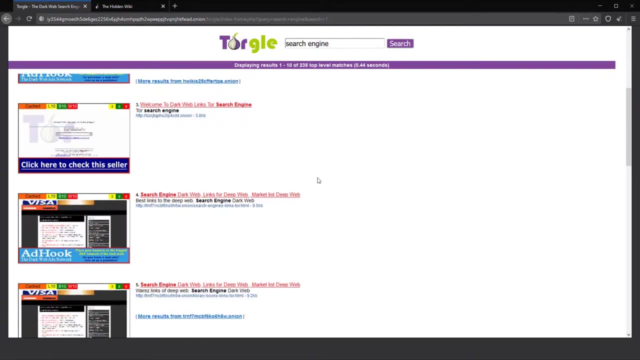 web internet search engines other than the ones I mentioned here. You can search the keyword search engine in the current search engine to discover alternatives. I suggest you try out many services and discover which one is useful to you. The search engines I have covered are just. 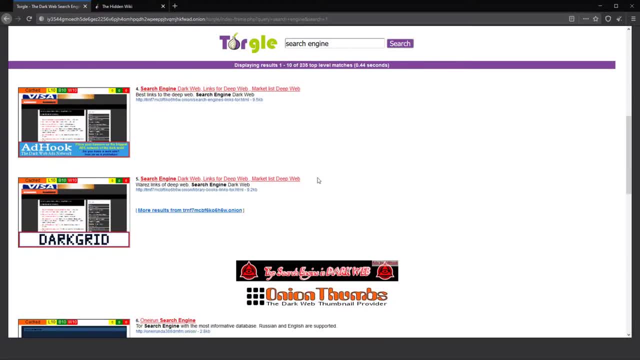 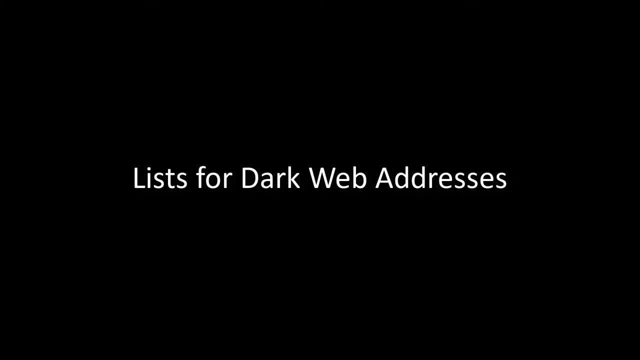 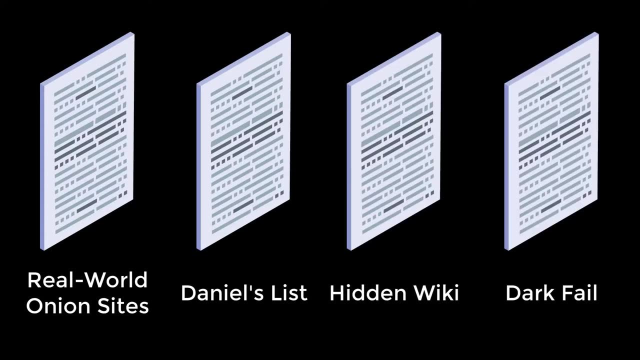 the engines. I have chosen to give you a start point: Always be open to discoveries for more and please search constantly. List for Dark Web Addresses. In this lecture we will be talk about a few of the main list resources you can use. Of course, 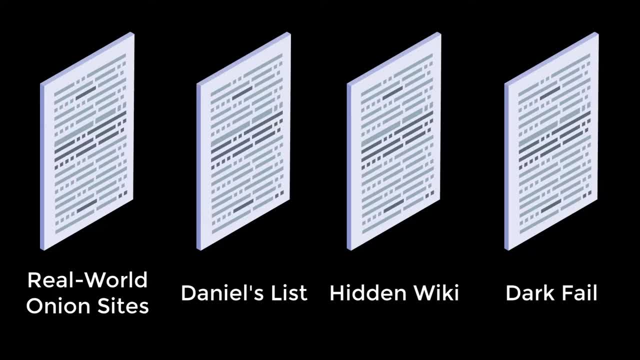 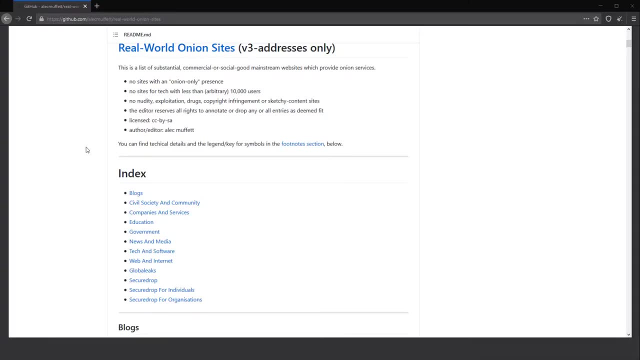 apart from the resources here, you can also get new addresses on various forums and blogs according to your interests. So please see this list only as reference sources for a start. Real World Onion Sites. This is a list of substantial commercial or social goods mainstream websites. 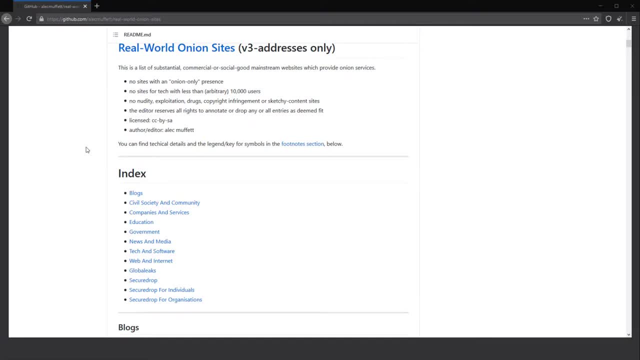 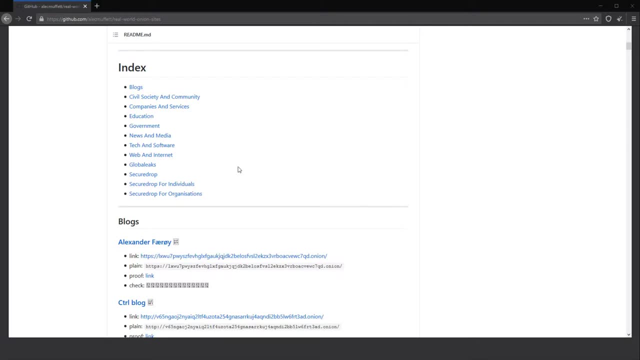 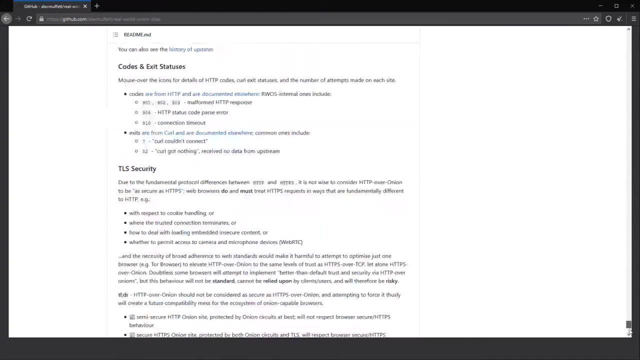 which provide onion services. This list contains public address information that is voluntarily updated regularly. The address of many widely used websites in many categories is available here. As you can see, you can learn onion address information of many popular services If you want to. 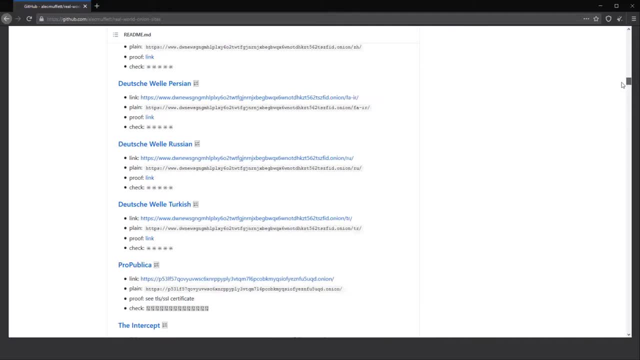 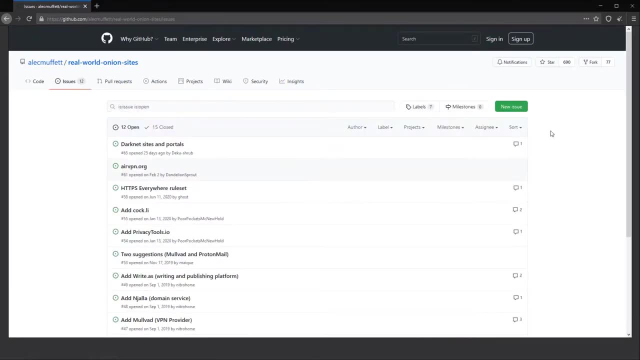 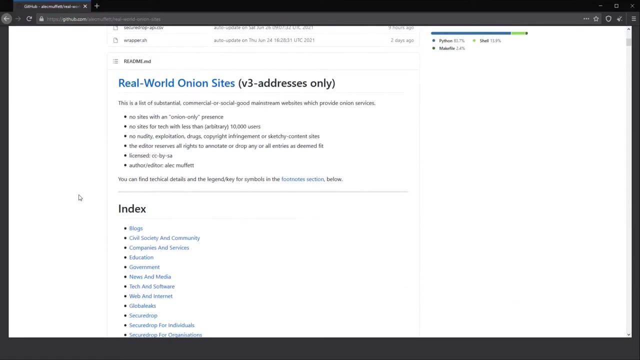 browse these websites anonymously. the list here will help you access real onion address information. If you want to contribute to this list, you can create new issue on the issue tab to add new address or correct existing mistakes. You can also see that there are 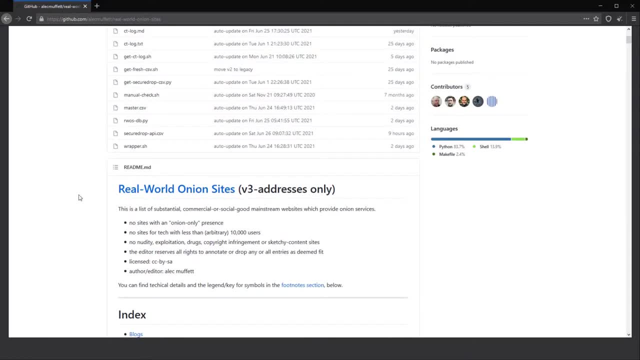 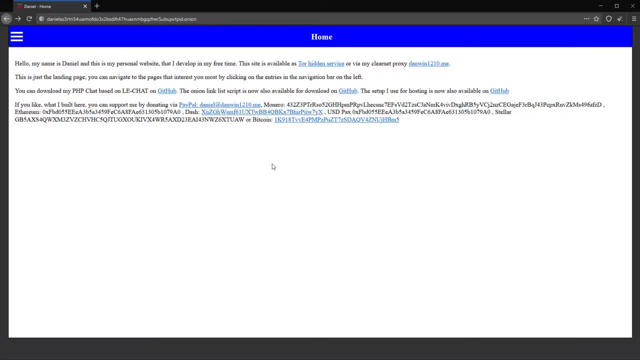 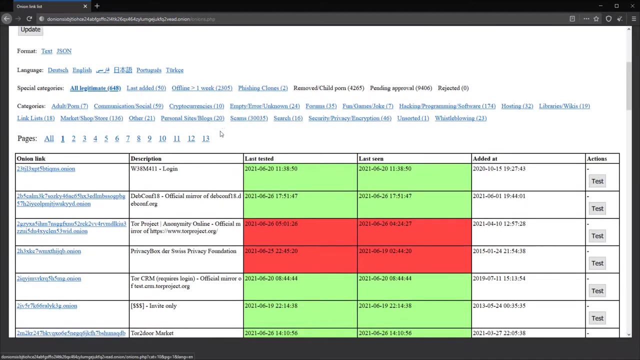 many addresses that have already been shared. You can, too, contribute to the project through your Github account. Daniel's List is an useful resource to help you discover various onion service links. I think this list really helpful compared to its alternatives. These websites list a lot of. 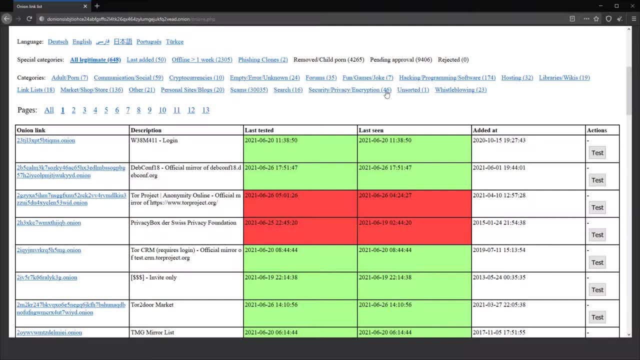 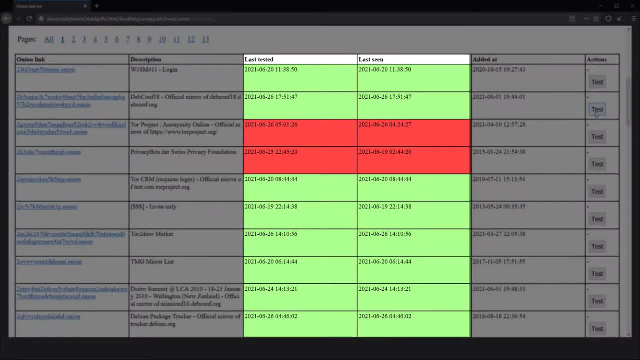 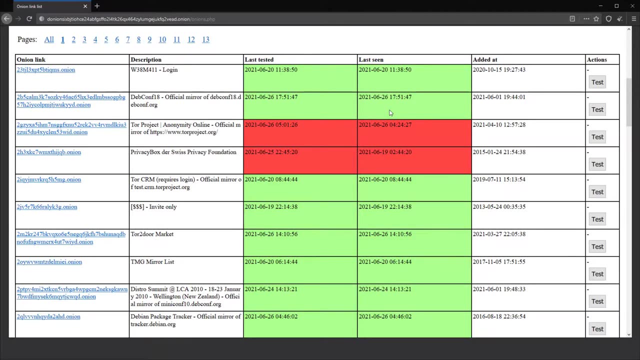 onion links which are categorized to make browsing easier. Moreover, it has a very useful built-in functionality which lets you know whether a particular website is online. This is very useful as it means you don't need to click and load every dark web link listed to see. 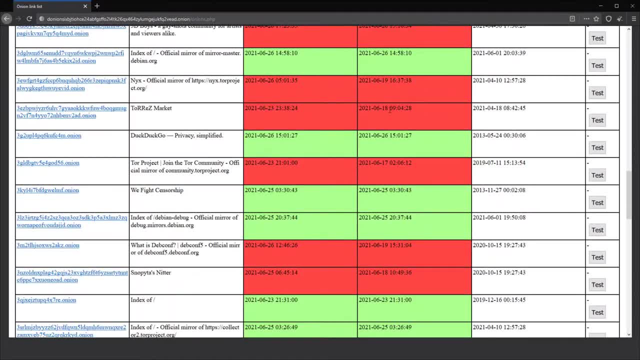 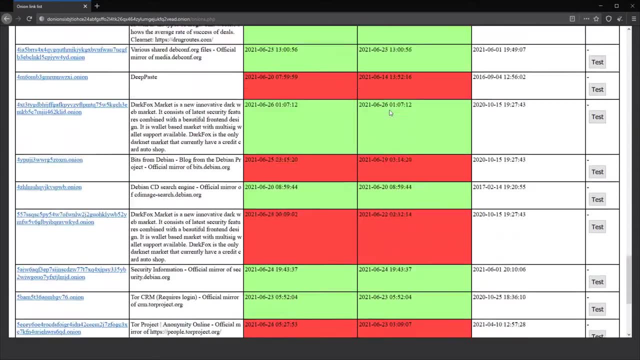 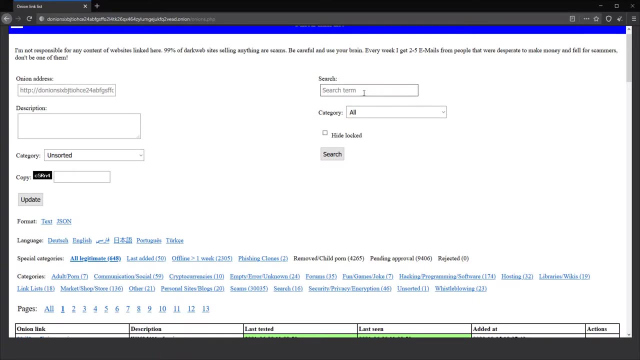 if it is working, Especially with the potentially long loading times of the Tor browser. this is a great feature: To see how many addresses are on the list. just take a look at it. If necessary, you can also search websites you want from the search bar here. 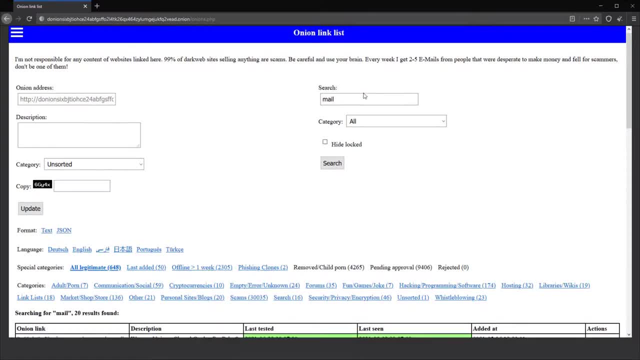 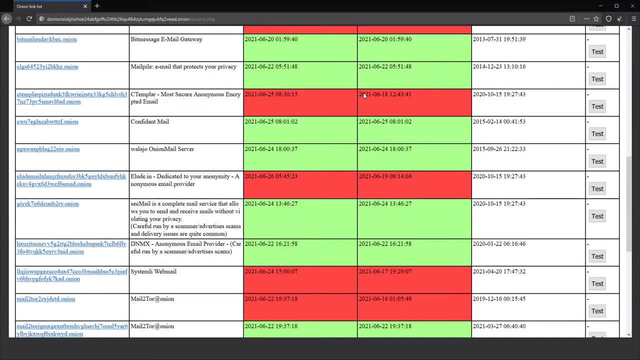 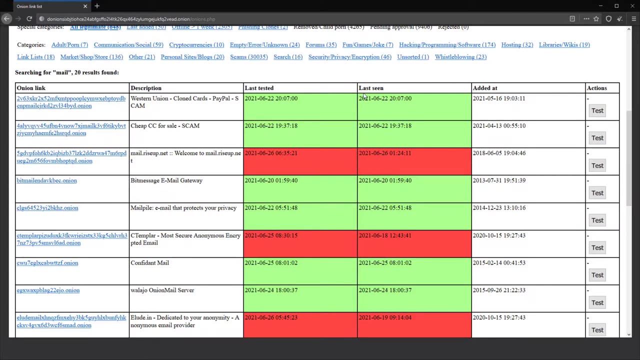 For example, when I do search mail, email services are listed, as you can see. Also hit the warning here: be careful about dark websites. Many of them can be scams. The fact that web addresses are on the list doesn't mean that these websites are safe. 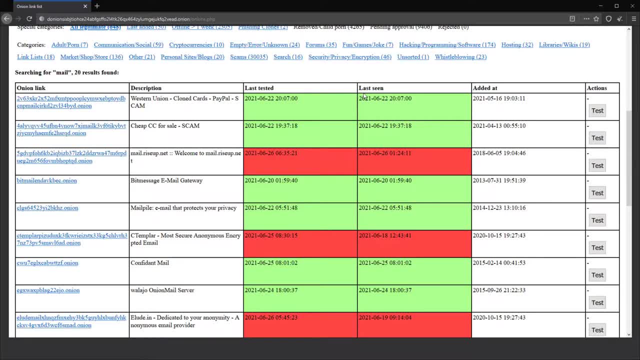 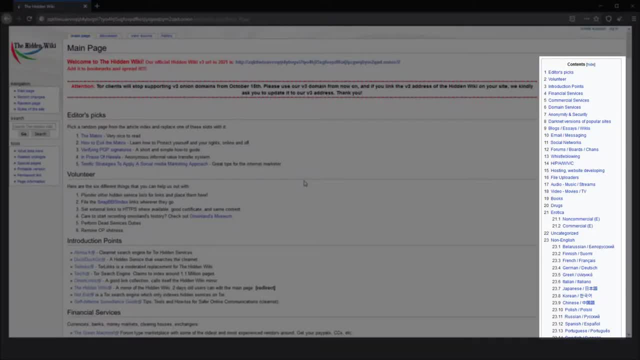 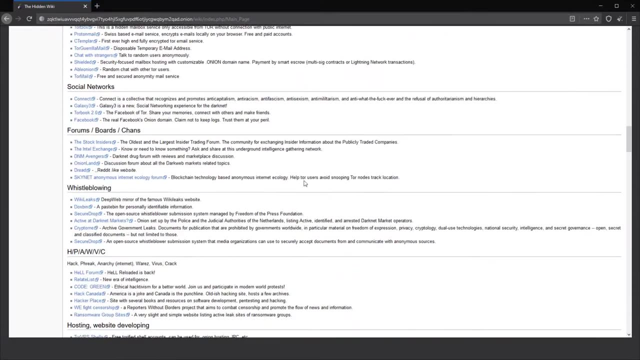 For this reason, you should always act carefully. Hidden Wiki: You can use the Hidden Wiki resource for the main link addresses that are categorized. Although most of websites in the list have to up to date information, it may be that some links don't work for various. 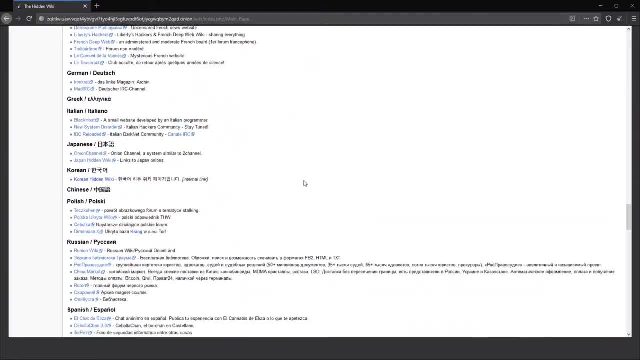 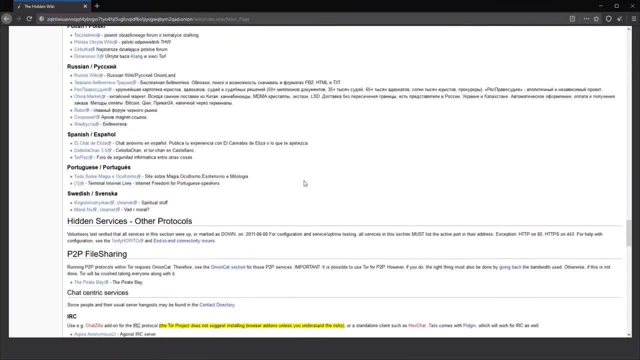 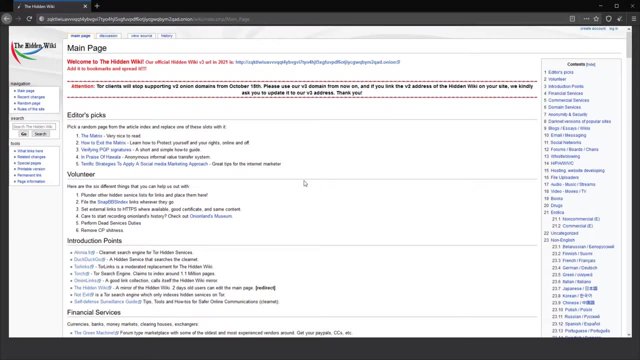 reasons. Nevertheless, we can say that it is the source that provides the most information among the alternatives. Also, please be aware that the addresses listed may not be legal or secure. Only the most frequently used ones are on the list, So it wouldn't. 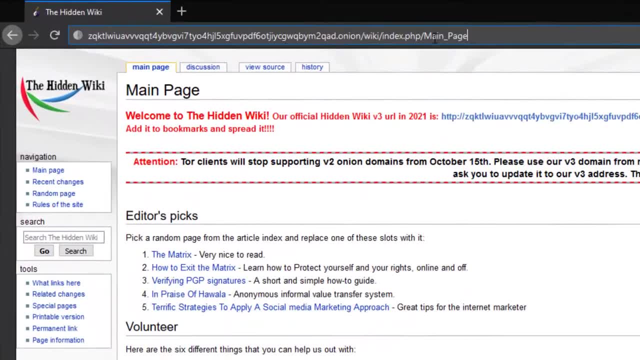 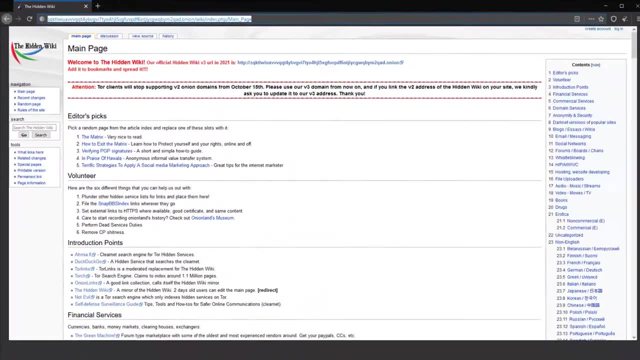 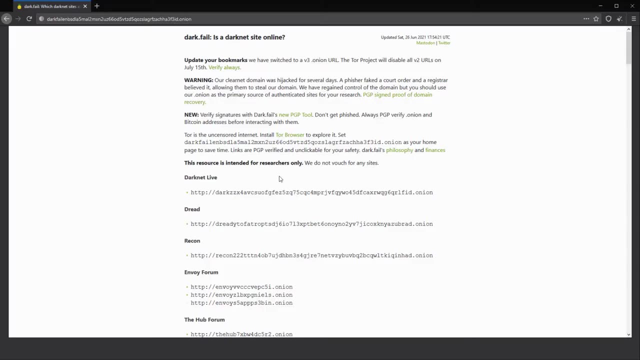 be right to blindly trust the list here. Also, make sure you are visited to the real Hidden Wiki address, as there are many malicious copies of the Hidden Wiki address. Using fake ones can put your security at risk. Dark Vale- After the Hidden Wiki resource, this is the most. 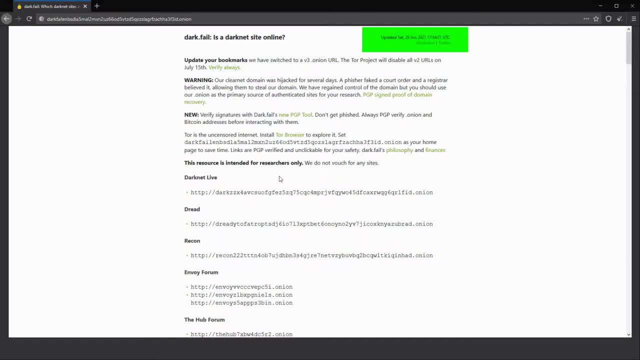 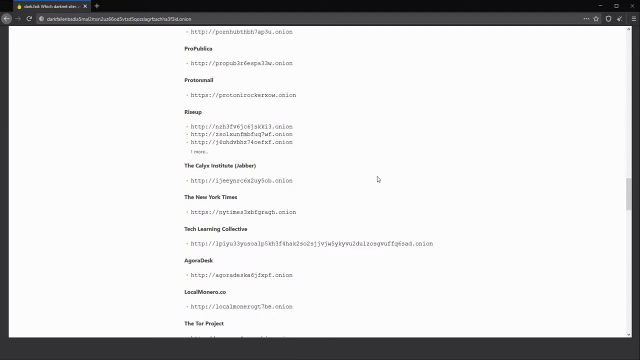 preferred list. Moreover, since it is updated frequently, it provides much more up to date address information compared to Hidden Wiki resources. You can also use these websites to confirm the addresses on the Hidden Wiki. when necessary, You can test real web address with the. 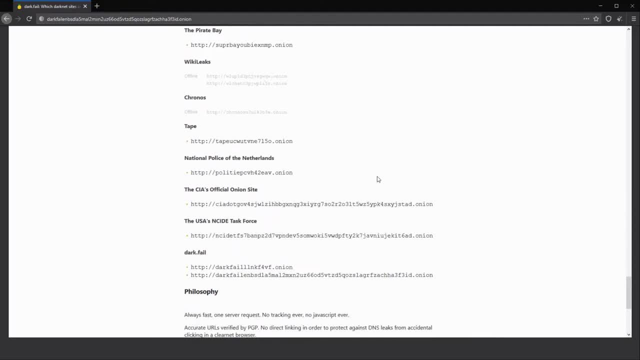 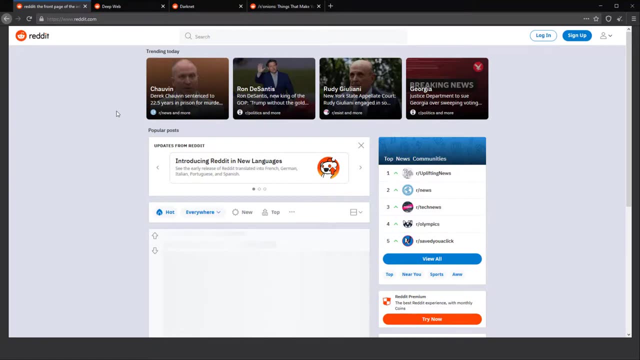 simple comparison, as fake or outdated address information won't be the same in the two lists. Apart from these addresses, you can also browse the list shared by people from platforms such as Reddit and add the links to your own list if they are the kind of addresses you will. 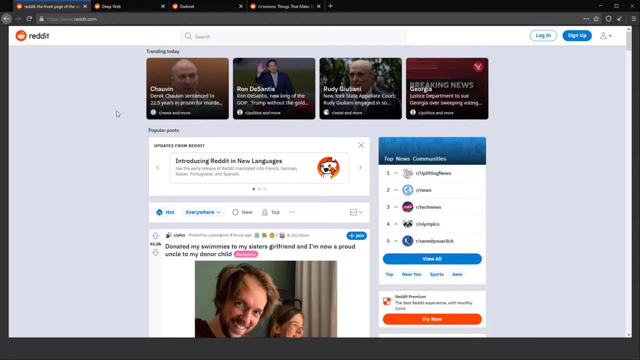 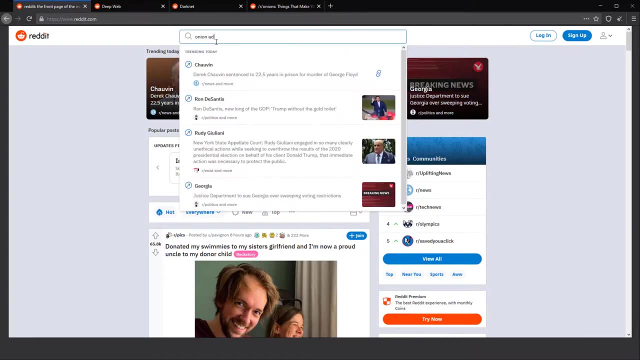 often use. There are many information sharing channels about Onion services on Reddit. If you haven't used Reddit before, you can see how easy it is to use. with a short glance and use it as a resource you will benefit from. You can access a lot of address. 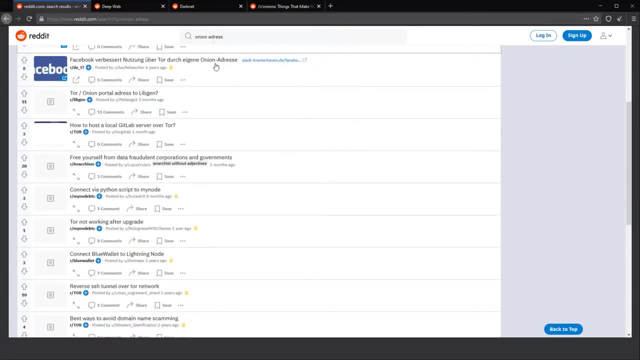 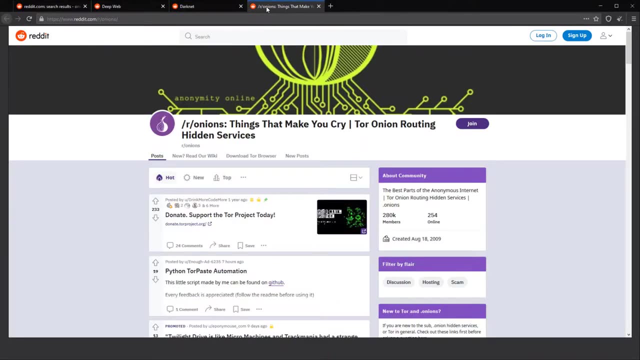 information by using the search bar on the Reddit platform or by joining communities such as Deep Web, Dark Web and Onions. You can also get new addresses in many different ways, apart from platforms like Reddit and Hidden Wiki. However, unfortunately, due to Tor's security architecture, 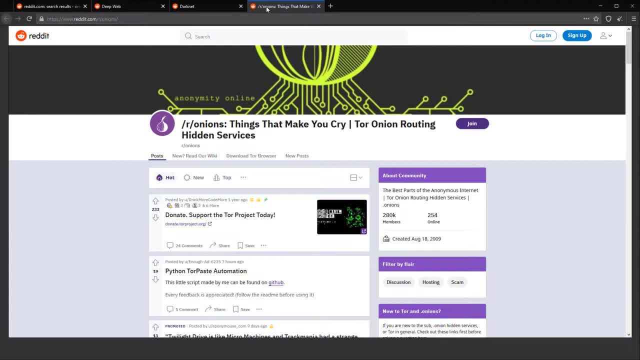 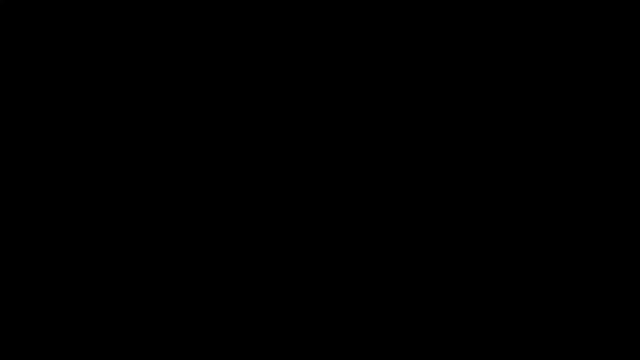 it is not possible to find resources where everything is collected in one area. Anyway, Tor doesn't want all Onion addresses to be easily exposed, So the reason why Onion addresses are hard to find it is purely for security reasons, According to your interest, you. 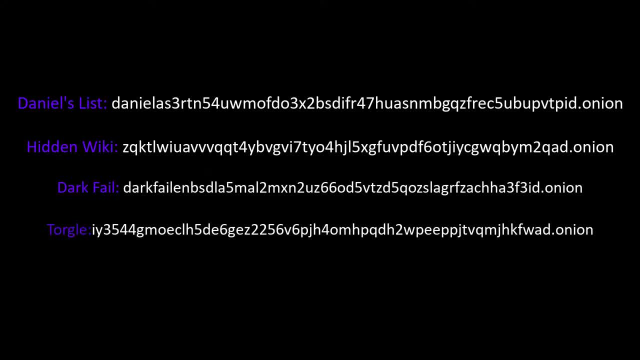 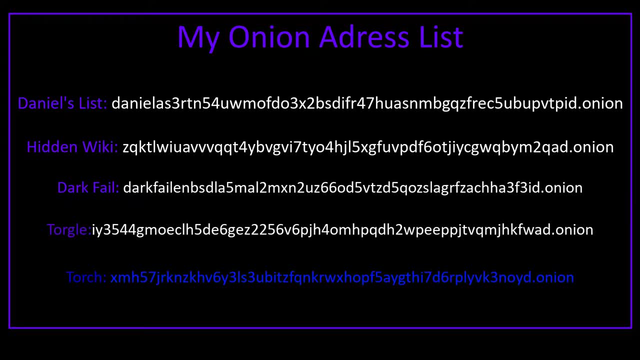 need to discover these web addresses by yourself over time and write them in your address list. What you need to be careful about with the new addresses you find is to confirm whether this address is original address from more than one source, if possible. In this way, you will have a clean. 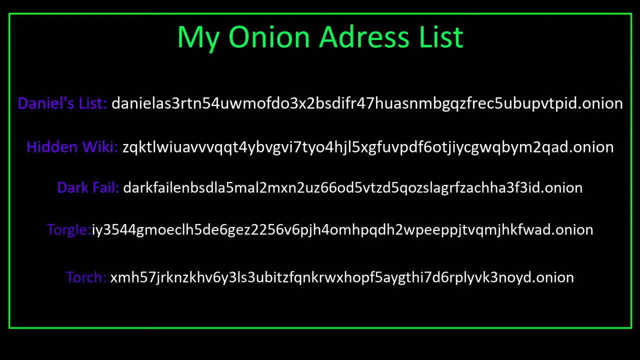 list of the addresses you use frequently. over time, However, you may need to update your list frequently due to changing addresses and unprofessional intermediate services on the Dark Web. This is one of the main reason why browsing on the Dark Web is cumbersome About Onion addresses. 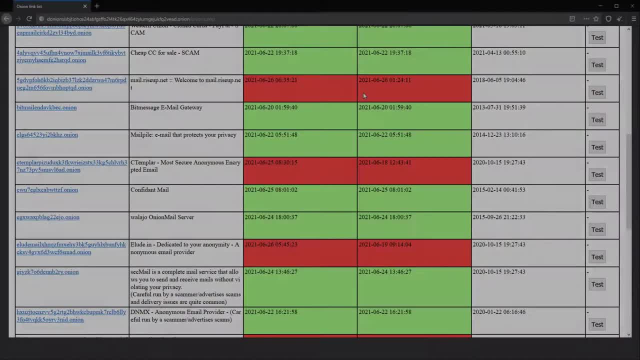 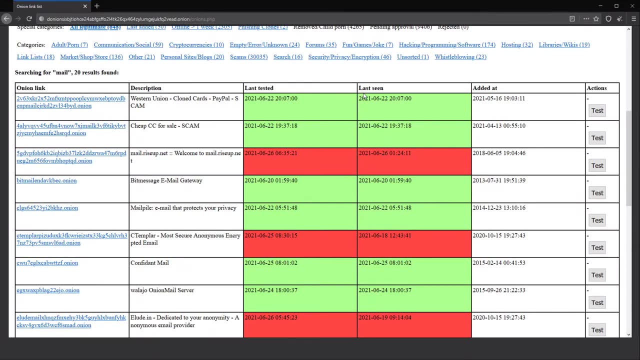 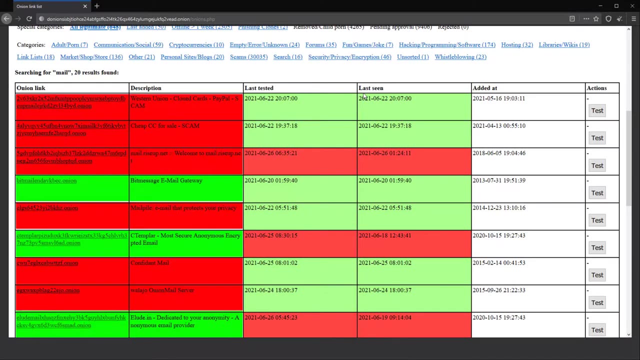 with meaningful and meaningless. While browsing the Tor hidden services, we witnessed that, with some exceptions, many Onion services have domains with full meaningless characters. What is the reason for the existence of both meaningful and meaningless domain names and the imbalance in their number of the character length? In fact, 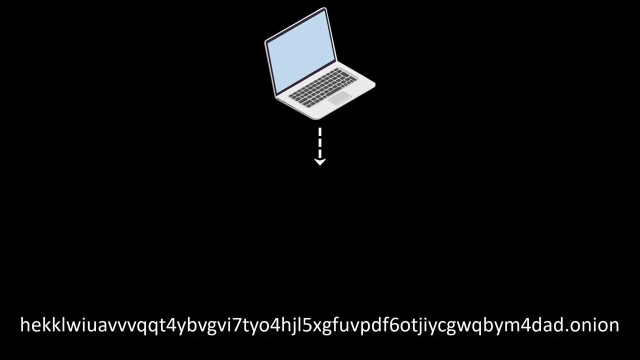 normally, these domain names are randomly generated by applying the method determined by the Tor service, depending on security reasons. In other words, nobody has the opportunity to choose in the domain name. Still, if we want a vanity domain name, we can create. 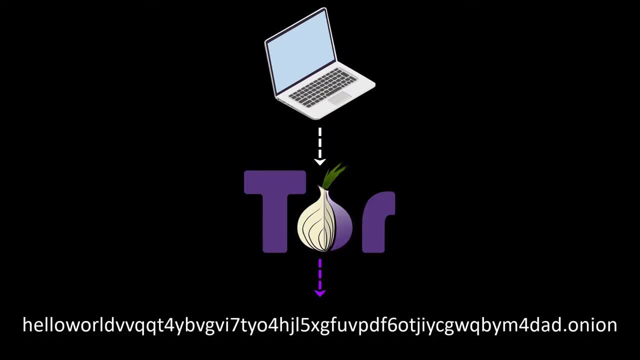 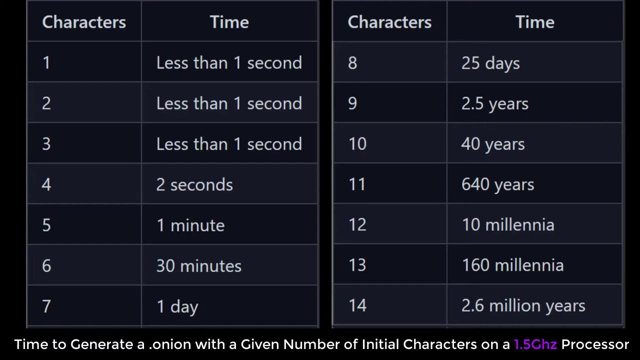 a vanity domain name by generating it over and over again. However, since this number of retires required very high processing power, it isn't an operation that everyone can do. You can see how much processing power it may require by looking at the list. 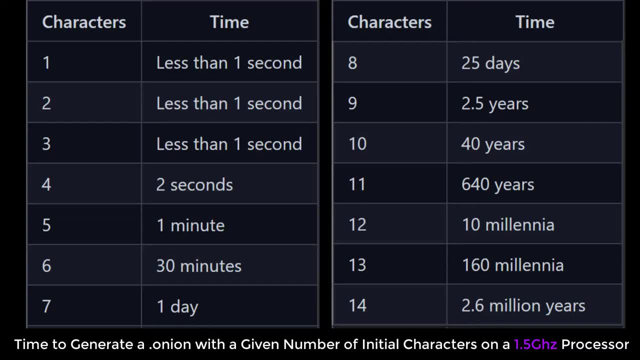 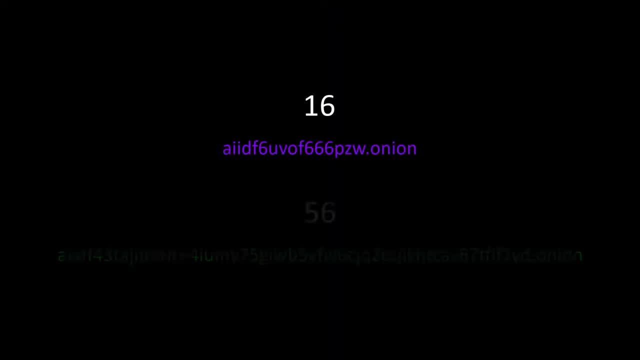 It's also unreasonable to try to produce a full meaningful domain name, as a Tor developer has increased the domain length from 16 characters to 56 characters in the new version. We explained the reason for meaningful and meaningless domain names. Now let's explain the reason for different. 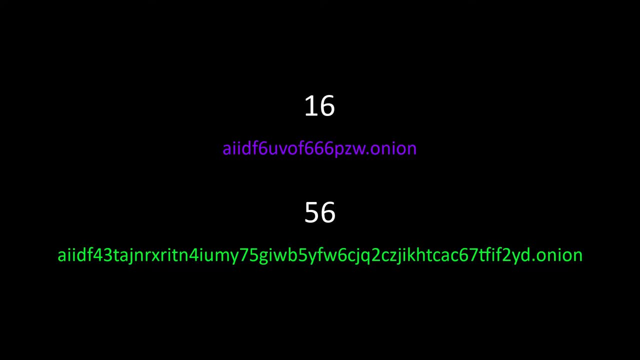 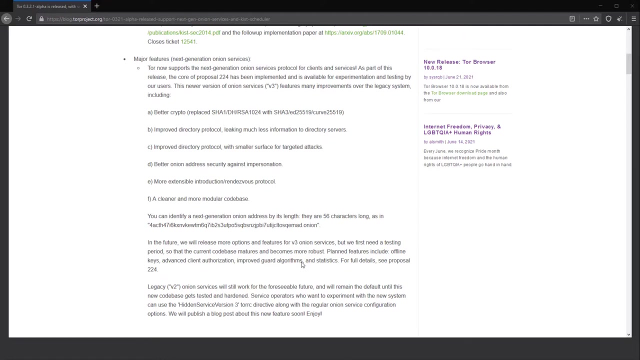 character lengths in domain names. For security reasons, Onion domain names are produced with a complexity and length that cannot be found by fuzzing methods. If you are curious about the technical details of this topic, you can read the official documentation from the link in: 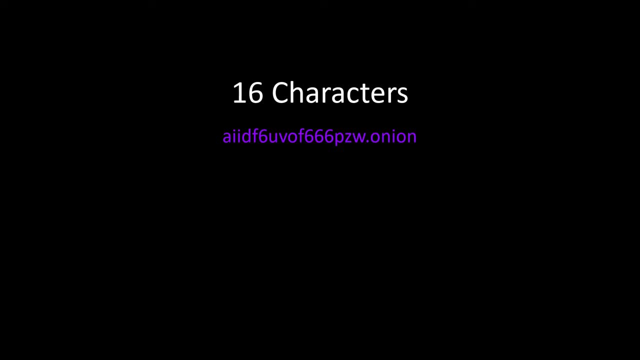 the lecture resources. Domain names with 16 characters are referred as the version 2,, while domain names with 56 characters are referred as version 3.. Although version 3 is recommended by the Tor as it provides an extra security measure compared to the, 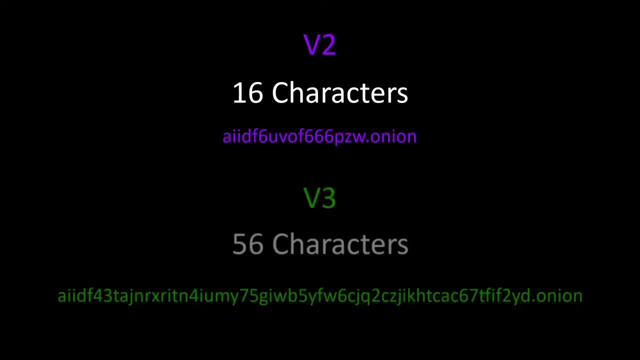 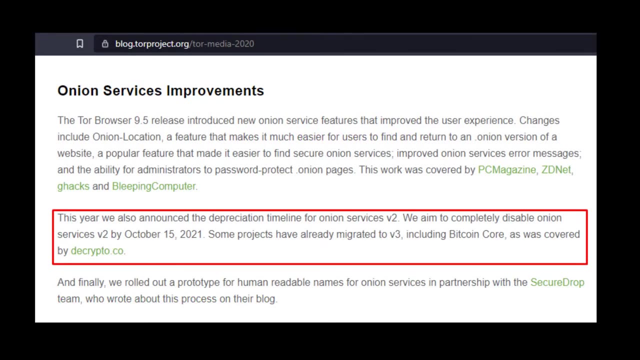 old one. It's possible to use the old addresses system, namely version 2 system, but Tor developers have announced that they won't support version 2 from October 15, 2021 release. Therefore, domain addresses generated with version 2 will no longer. 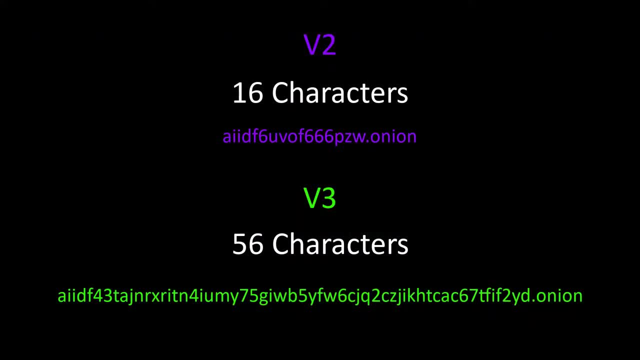 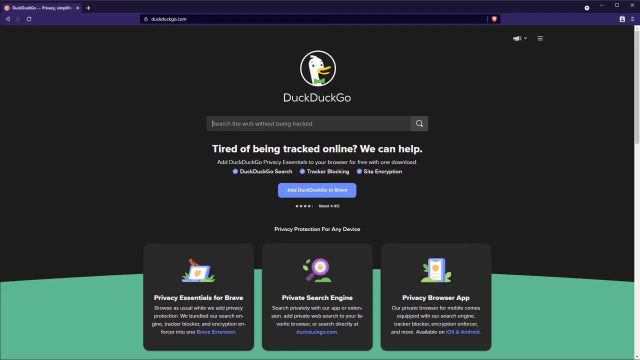 be in use. So if you encounter version 2 addresses and this link address doesn't work, the reason is that version 2 addresses are no longer supported. How to create your Onion site on Tor. In this lecture I would like to briefly show for those. 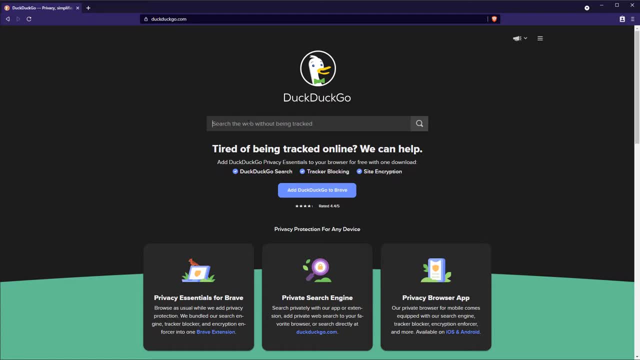 who are curious how they can create their own Onion website. I said for those who are curious, but since I will refer to what I will tell in this lecture in the future, I strongly recommend that everyone follow the lecture here. In this lecture I 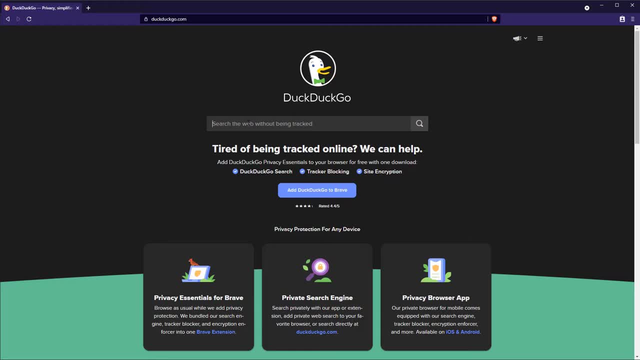 will only show you how to use your computer as a host, But of course your website won't be accessible when your computer is turned off, as the host that is hosting site files will be your computer. If you want to establish a constant active website, you can. 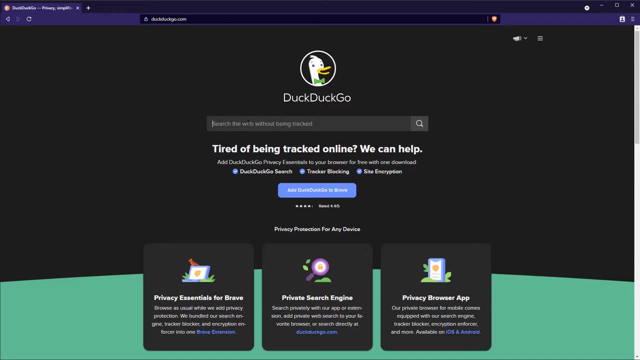 rent a server and have it hosting 24x7. via this server, You can also use of hosting services that offer services over Darknet, Since the installation process will be similar. in any case, I will show you how you can host on your computer so that everyone. 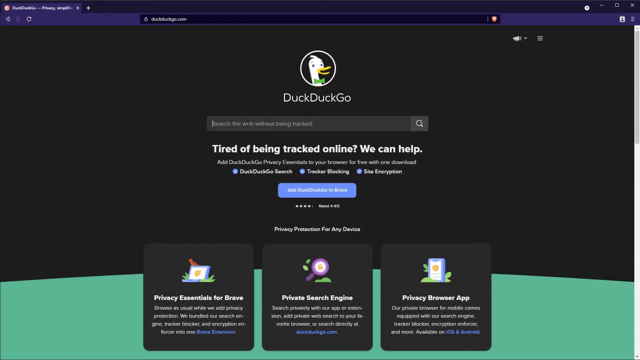 can test it and see how the structure works. Since the professional website setup and details will be outside of the discourse curriculum, I will only be discussing hosting a simple web page. In other words, you need to have necessary infrastructure in order to set up. 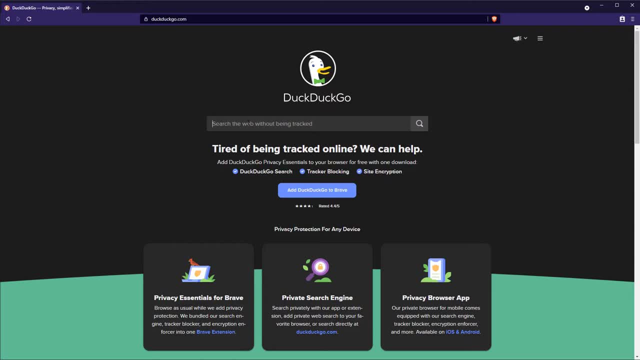 a website that offer a comprehensive service. Here we will be covering basics of onion service hosting. to get an idea of how the system works, I will be doing the explanation over Windows, as they are more widely used. Nevertheless, the tools I will use during the 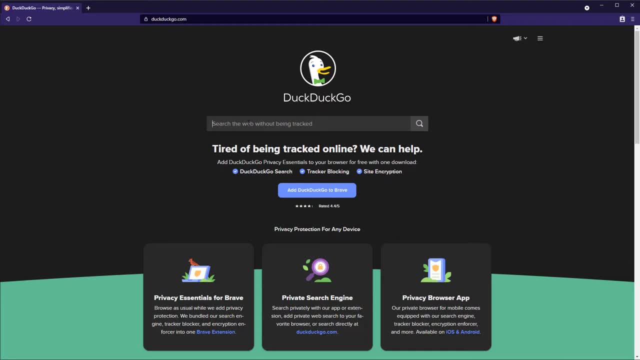 lecture are those that can be used in common on Linux and Mac operating systems. In other words, you can easily follow the steps on operating system you are using. First of all, to use your computer as a server, you need to download and install. 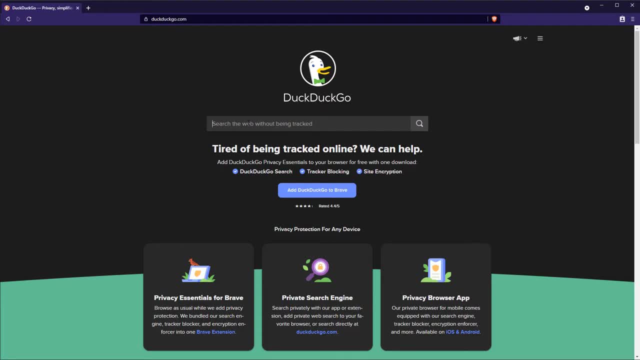 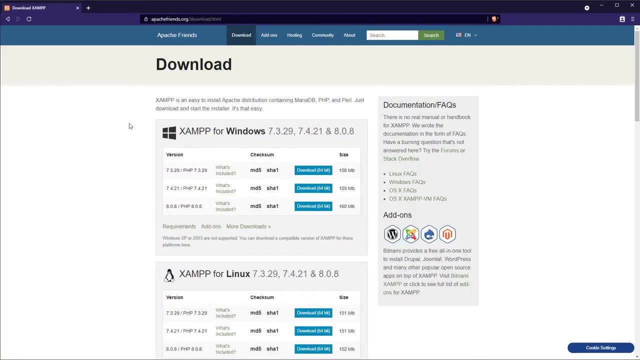 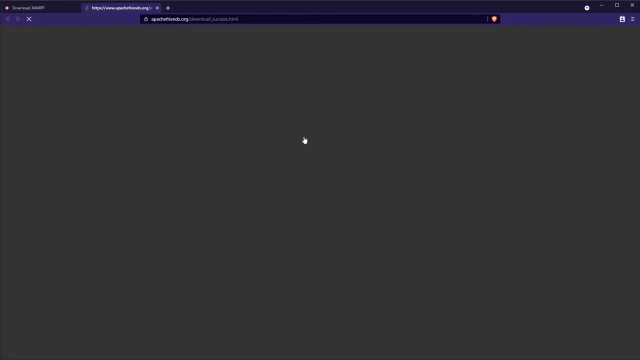 the XAMPP tool that helps you create a local web server. Let's visit the website to download tool From here. you should download the setup file suitable for your system. Since I am using Windows, I am downloading the setup file for Windows. 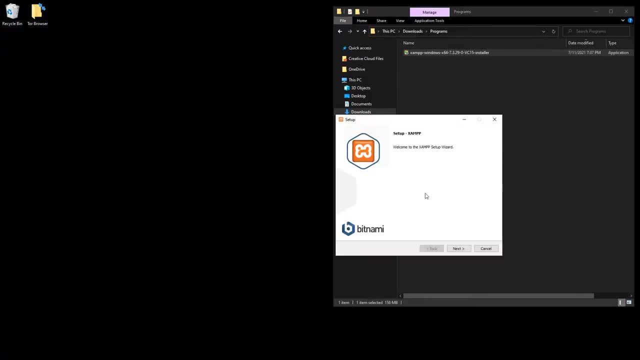 After downloading setup file, let's run setup and complete installation steps. I am not talking about the installation details, as all the installation steps are very easy and standard old systems. You can easily complete installation steps. After completing the installation steps, let's run the application. 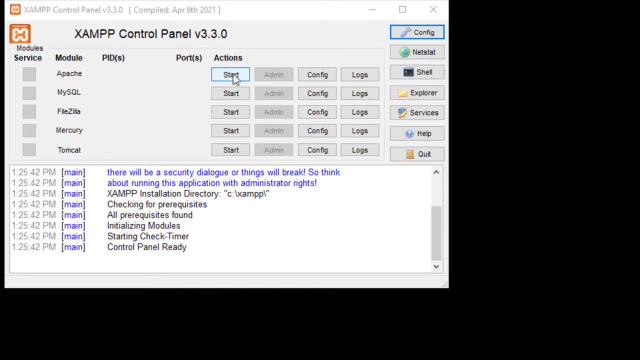 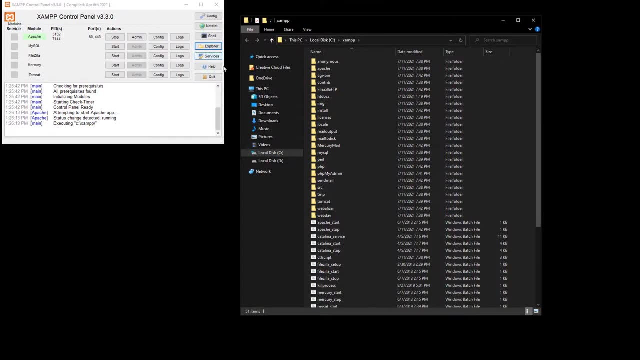 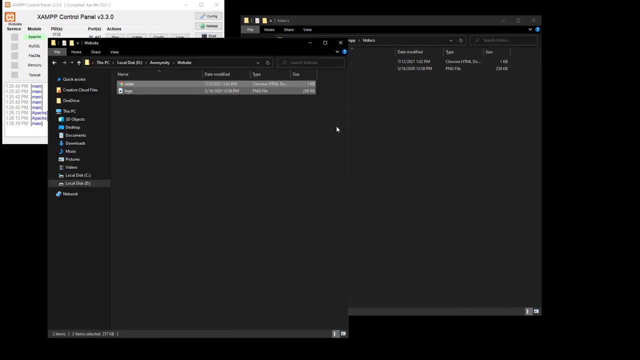 When the application opens, click the start button to start the Apache service. After the service is started, click the explore button to add the files of your website to the required location. Now you should go into the hddocs folder and add the files of your website. 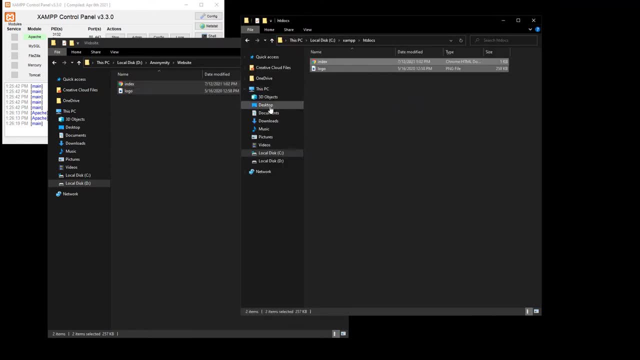 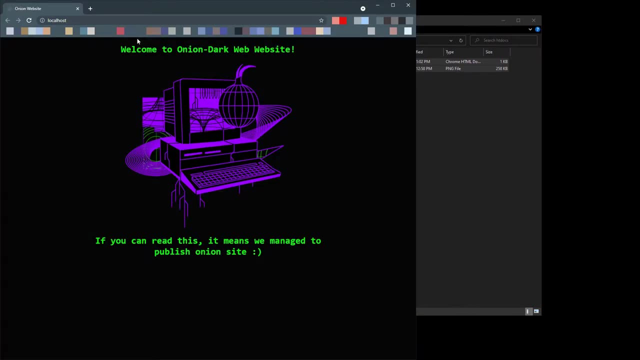 after deleting the files here, After adding your website files, go back to the application and click the admin button to test your website. From the page that opens, you can see that you have managed to host your website locally. Now you need to make a few adjustments. 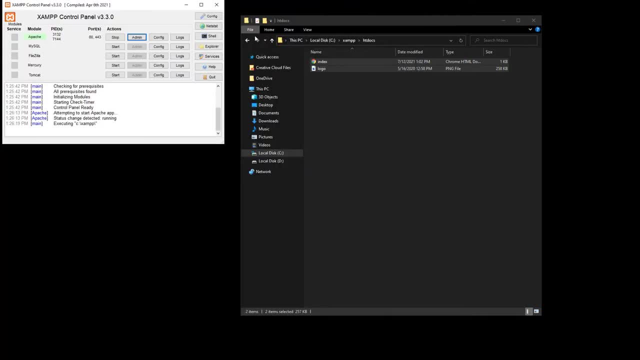 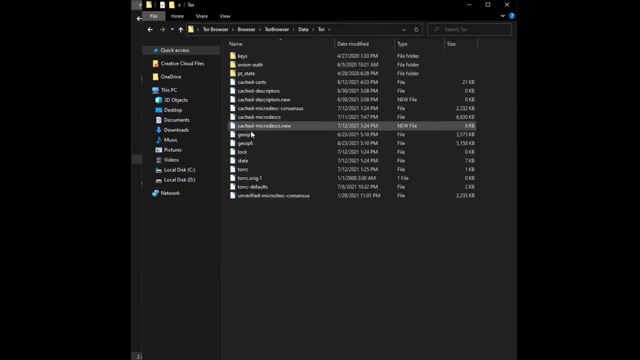 to get this site, which you have hosted locally on the Tor network. First let's switch the Tor Browser Browser. Tor Browser Data. Tor Folders. Let's right click on the file name Torch here and open it with any text editor. 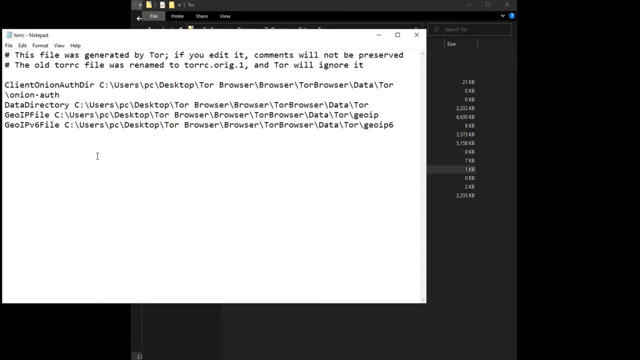 The file location is similar on the Linux and Mac OS systems. You can easily access Torch file by going to the location where you installed the Tor Browser. Let's come to the bottom the line of opened file and specify the hidden service directory of website and the address of. 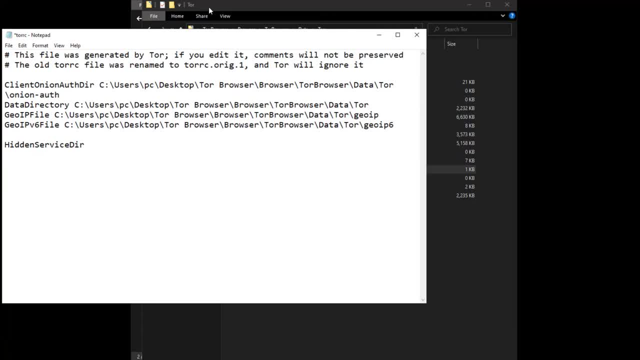 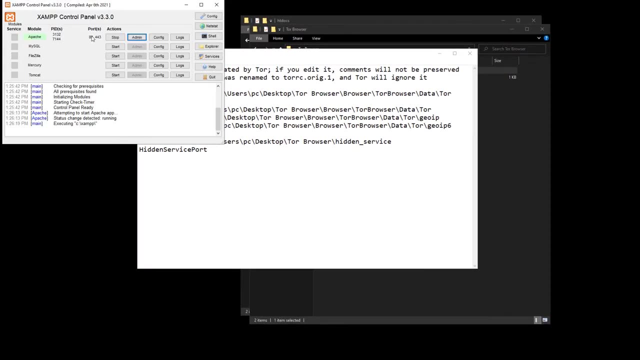 your local server. In the first line you need to specify the location where the configuration files of your onion service will be located. I specify that it should be saved in a folder called hidden service in the Tor Browser folder. As the service port, I specify port 80.